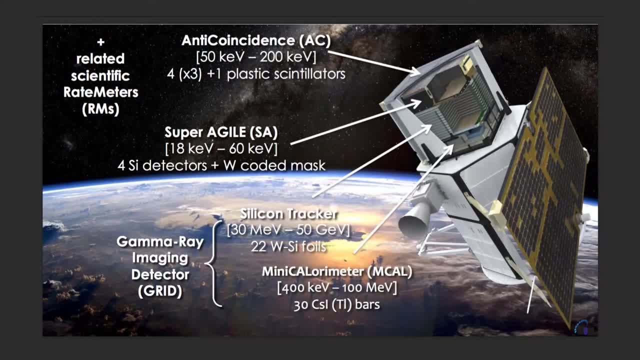 is composed of a silicon tracker with imaging capabilities here, sensitive up to 50 GV, and a minicolor emitter. Yeah, And the other thing that we'll start with here is the silicon tracker Just to an all-sky monitor with no imaging capabilities, sensitive up to 100 mev above these two detectors. 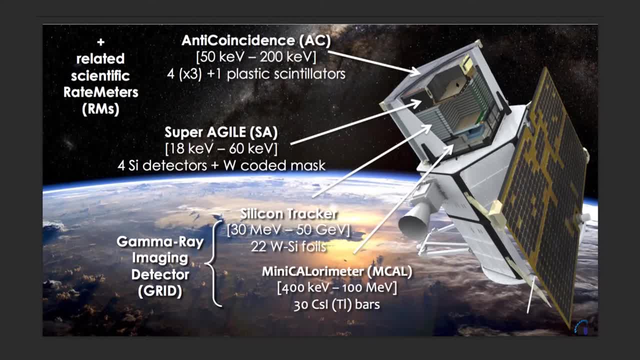 there is an x-ray for the mask, super agile, which is sensitive in the x-ray energy range, and all around we have plastic scintillation panels acting as an anti-coincidence modulus. so it's usually it's important to remark here that we have also scientific red meter data. 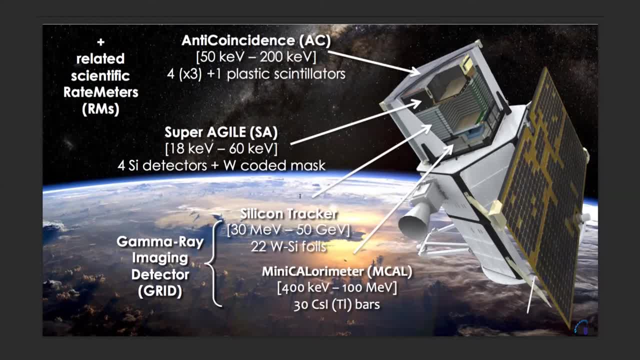 which are basically the same data acquired by each detector here, but sampled with a rougher time resolution of about half a second or one second. so they basically serve to monitor the background rate, the background modulation, but of course they can detect transients as well. so, um, some of the most important results of agile. of course it's a it's a high energy mission, so 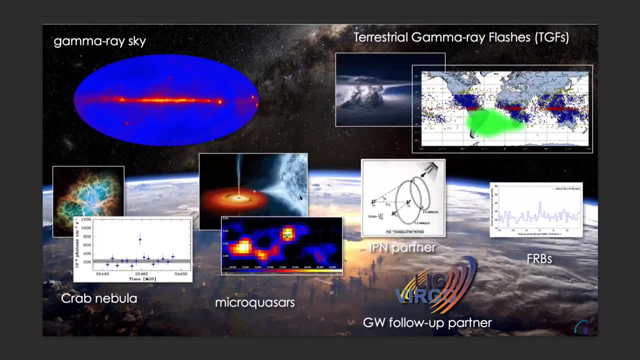 it investigates the gamma-ray sky detecting sources, and it discovered the crowd nebula variation, which was thought to be a very stable source in the high energy range. it discovered an emission above 100 mev from jets of micro quasars, especially in the sickness region. 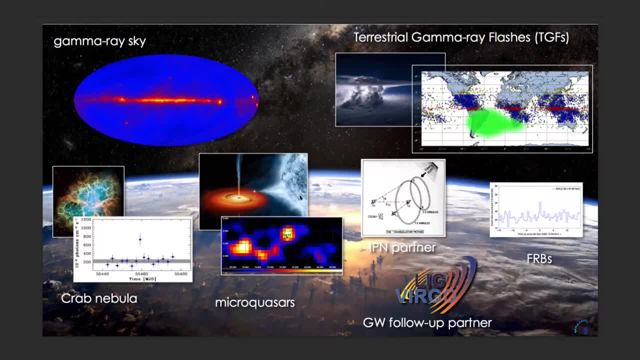 and it detects gamma-ray bursts. so it's an active partner of the ipn network for triangulation and for sharing data about your beast. it has been a very active follow-up partner for what concerned the detection of gravitational waves during the lago virgo campaign for two and all three brands. 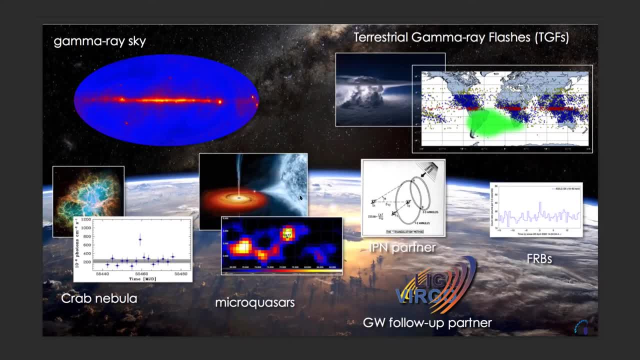 and it's one of the major players in the detection of terrestrial gamma-ray flashes, which are these high energy emissions produced during thunderstorms on the earth and escape into space. and more recently, last year, it detected, together with integral insight and comes wind, an x-ray pulse coincident with the fast rated birth. so actually, 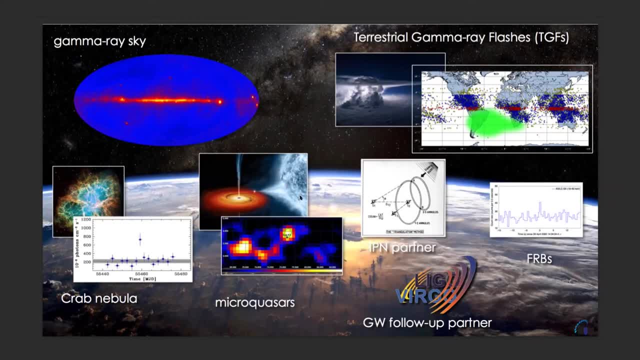 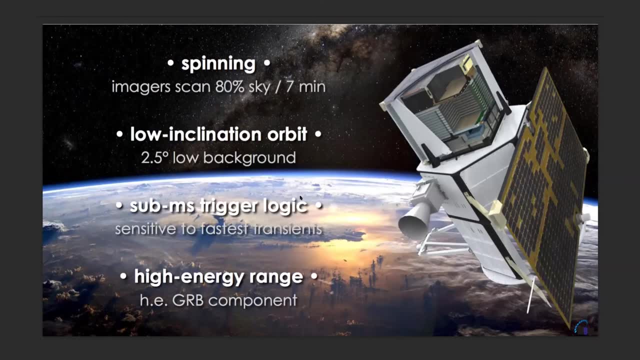 opening up a new way of investigating this: this radio policies. so just a few points about agile. after the first two years, in a nominal phase, we lost the possibility to point sources in the sky. we are spinning around our sun point in axis, scanning about 80 of the sky every seven minutes. 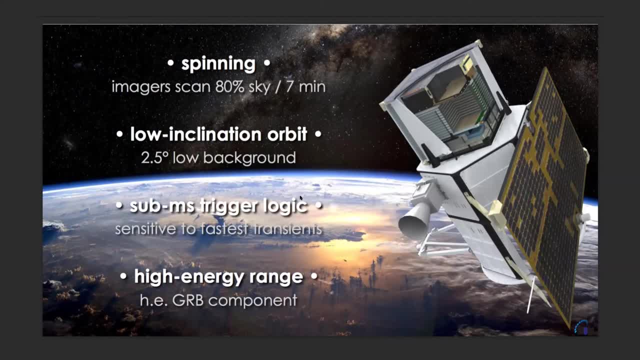 back when dealing with fixed sources in the sky, but it's not much of a drawback when dealing with isotropic events, isotropic transients such as GRPs. It experiences a low charged particle background modulation because of its very low inclination orbit. The mini-calorimeter has a 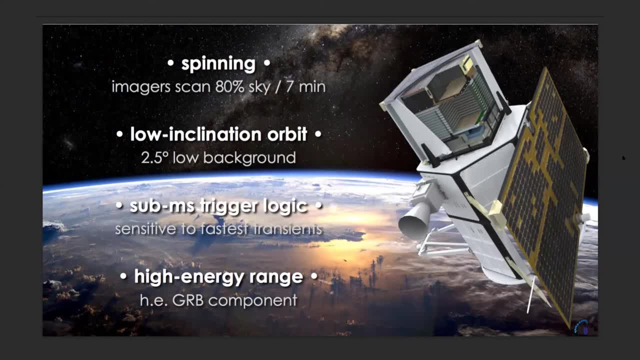 sub-millisecond trigonologic time scale, which makes it very sensitive to short duration transients. And, of course, Agila is a high energy mission, so it's mostly focused on the detection of high energy gamma-reverse. So just a few words about high energy gamma-reverse, Simplifying, if we take 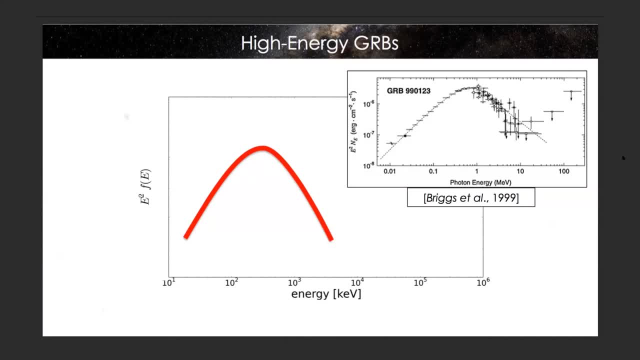 a look to the spectral energy density. here we can describe a typical spectrum by means of a band model, for instance a smoothly joined broken power law. And so what happens when a mission sensitive, let's say in the x-rays, hard x-ray energy range, detects something coming from a GRP? 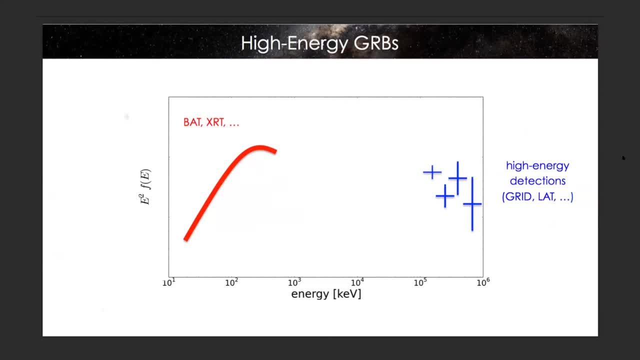 and together another mission. another detector detects some high energy photons coming from the same GRP, So it's interesting to see what lies in between. And this region is the one investigated by the mini-calorimeter, And it's also a region. 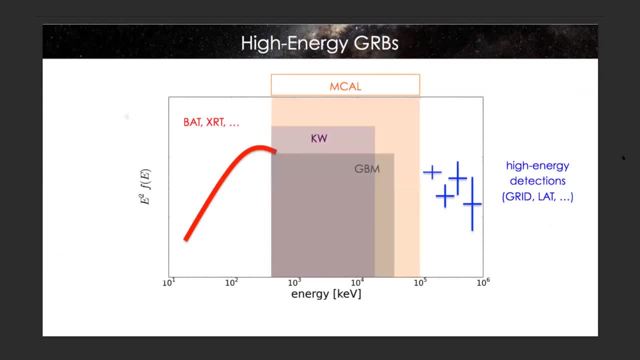 spectral region which is poorly investigated by other space missions. So we have GBM, we have Conoswim, but it's a very important region of the spectrum, of course. What could MCAL see in this context So, for instance, it could detect just the right part? 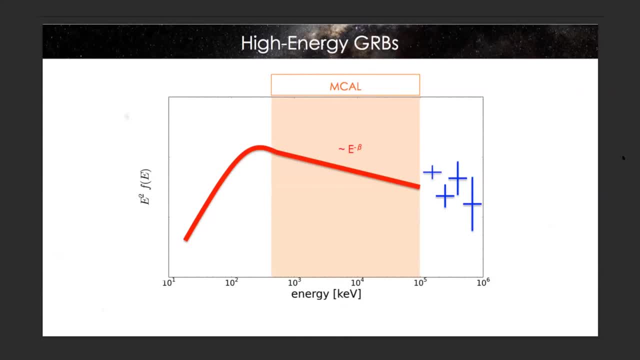 let's say the high energy part of the band model. So we can just observe a single power law, in this case extending up to the highest energies, Or we can observe the high energy component of the band model plus an extra component, an extra power law or an extra power. 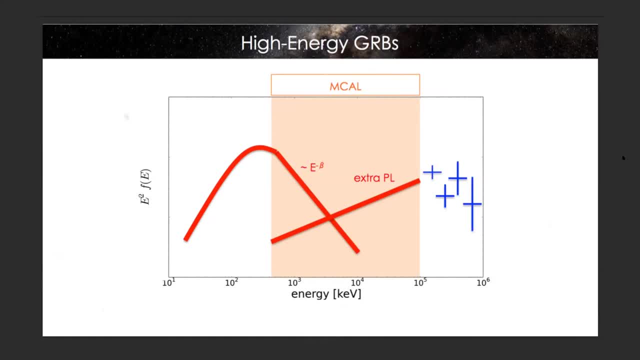 law emerging at a certain time or during the prompt phase, extending the spectrum up to the highest energy, Or we can just detect a very energetic band model with a peak energy about our lower energy threshold, So let's say about 400 kipi And, as I said before, all these extra. 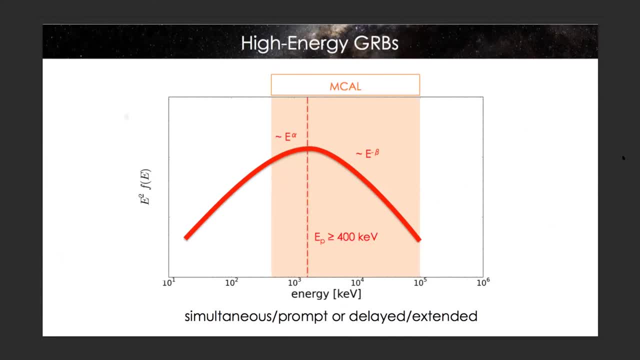 components could arise simultaneously during the prompt, So suggesting sort of inner origin in the inner core from inner shocks, or a delayed, extended emission resembling a sort of high energy afterglow, So something which is more like outer shocks interacting with the surrounding medium. 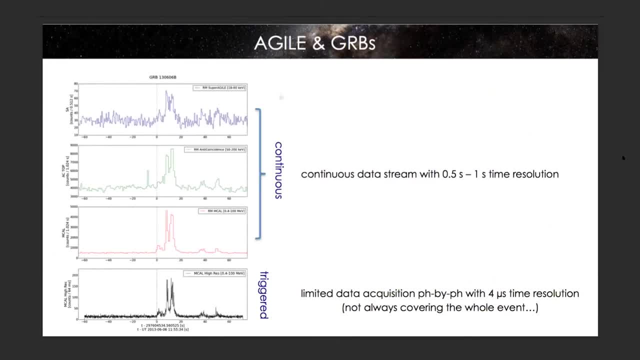 So here I focus on the detection of the GRBs with MCAL and the rate meters. As I said before, rate meters are here rate meters of the supra-ragile index rays, anticoagulants in the X-rays, and MCAL. So these two are the same energy range. 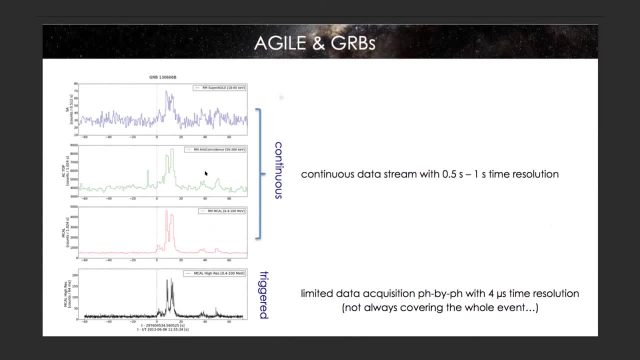 The important thing is that these data are a continuous data stream with, let's say, half a second or one second time resolution. On the other hand, we have MCAL data, which are basically, in principle, photon by photon data with four microseconds time resolution, but they are. 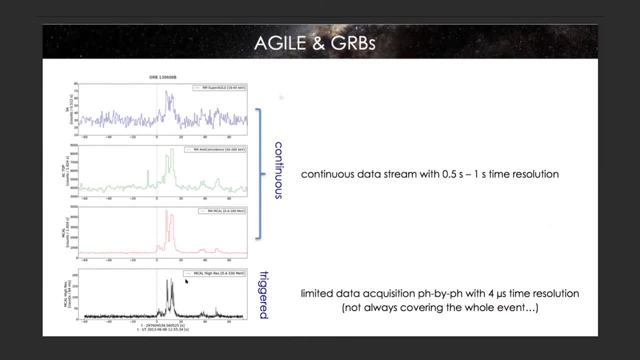 acquired after a trigger is issued on board And, of course, the data acquisition acquired on board. the duration of this data acquisition depends on the trigger time scale and depends on the onboard configuration. I say this because in recent years, we underwent a lot of telemetry restrictions, which makes us 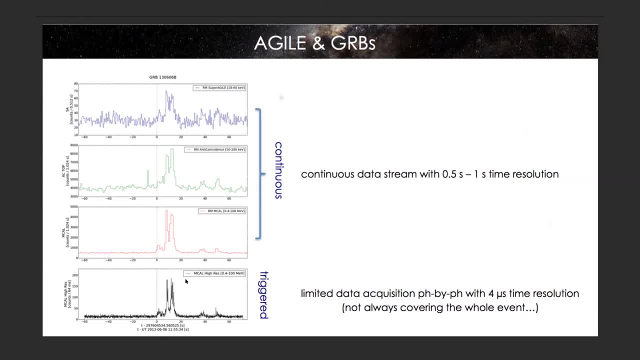 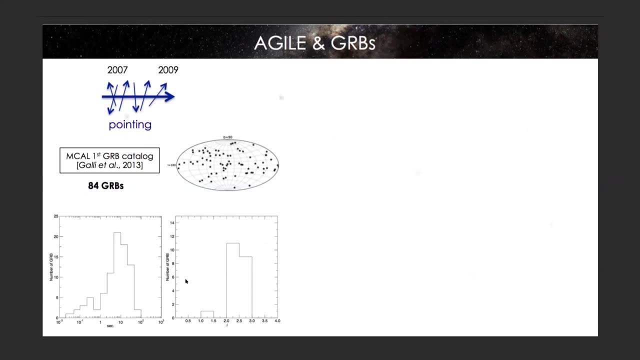 less sensitive, let's say less capable of detecting very long GRBs, because we had to reduce the amount of mass memory dedicated to these acquisitions here. So about GRBs detected with MCAL? we have the first catalogue released in 2013 concerning the 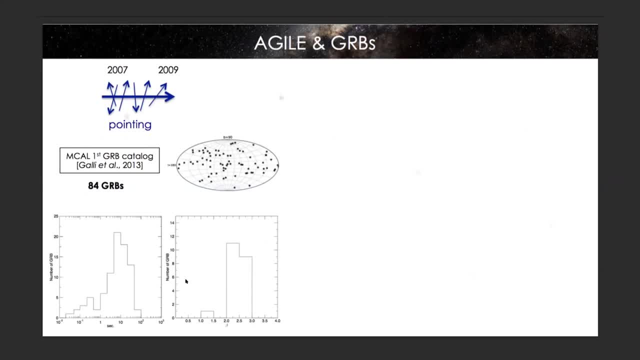 first two years during the so-called point-in-phase, 84 GRBs. Here you can see the T90 distribution and here, assuming that we are just observing the high energy component of the band models. basically a single power law, a simple power law. here we have a distribution of the photon index speaking between: 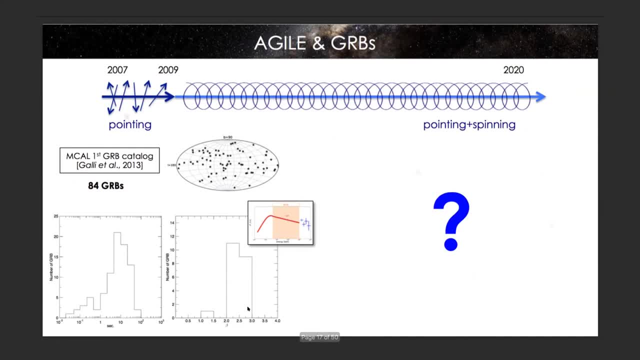 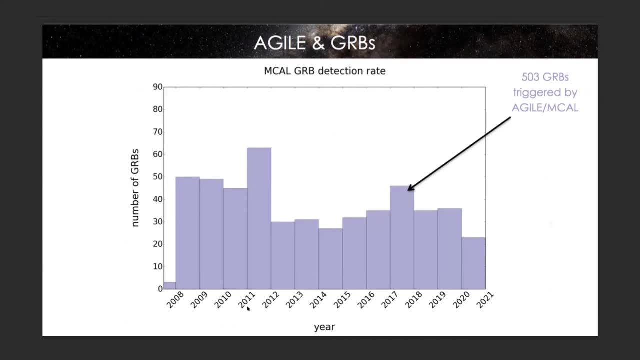 minus two and minus three. so what happens in the in the last years up to november 2020? let's take a look to the mcal grb detection rate. it's not constant in time. so after this first four years, let's say with what i call the golden age, we have, of course, a reduction. 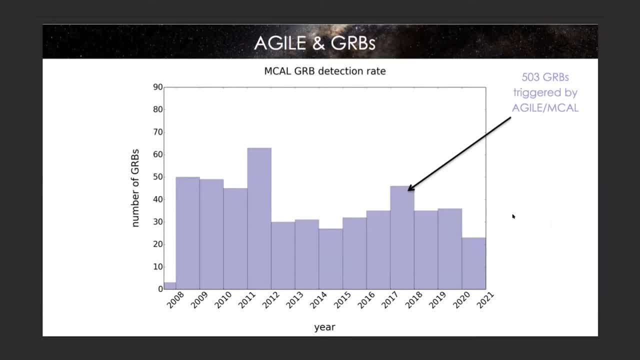 of detected grbs it is. this is due to telemetry reductions. as i said before, we had more third passages during 2017, during the the life of ergo ram and, unfortunately, last year. we have this lack of data due to the provide pandemic, which is very affected our our number of served passages in 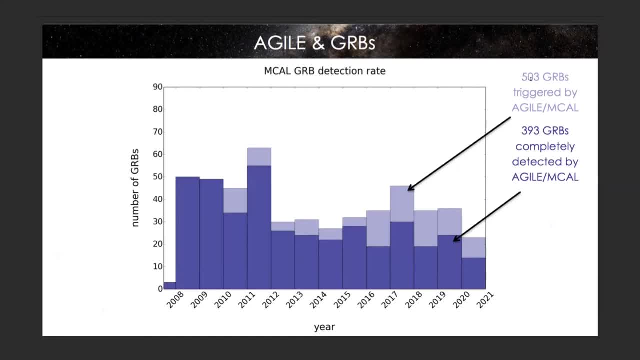 malindi. so, as i said before, out of 503 grbs triggered by mcal, we completely acquire only 393 grbs. so in this case, these are the grbs that are completely acquired. um the other 110 grbs are not useless, of course, because our 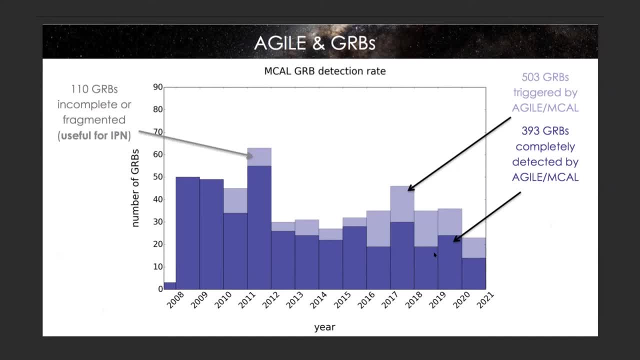 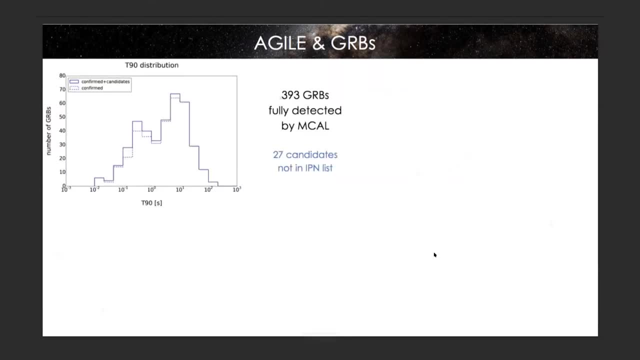 partial detections, but our partial detection with a four microsecond time resolution, and this case could be useful for improving triangulations or sharing data with the ipn. uh. this is the distribution of 393 grbs, the t90 distribution by model distribution. here i i show also 27 candidates which are not present in the ipn list and as you can see here, um, if we 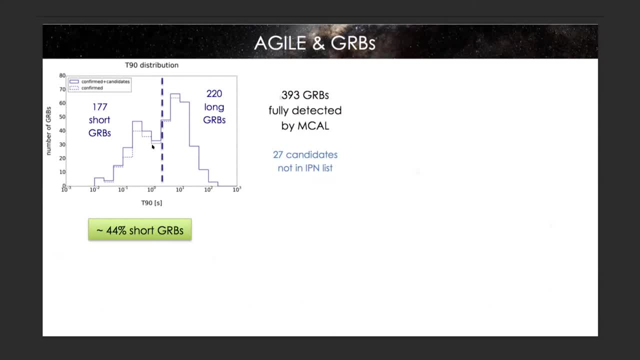 take a look to the this distribution, we see that our rt90 is mostly biased toward short grps. so this is because of several reasons. uh, if we take a look to the grb duration as a function of the detection here, here and here blue dots represent events that triggered mcal and were completely 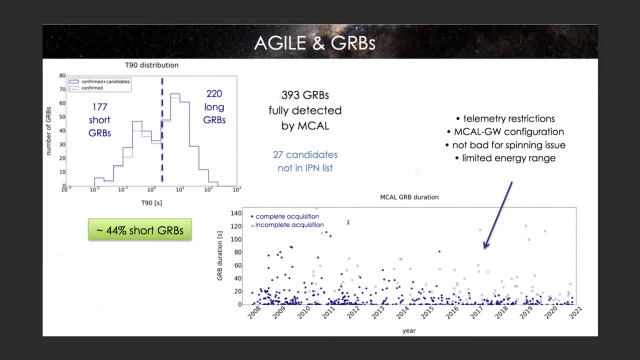 acquired on board, whereas the hollow dots- here white dots- represent events that triggered them but were not completely acquired on board. so you can see here that we didn't lost our sensitivity to uh, also to long duration grbs, but we lost the capability of detecting, of acquiring data. 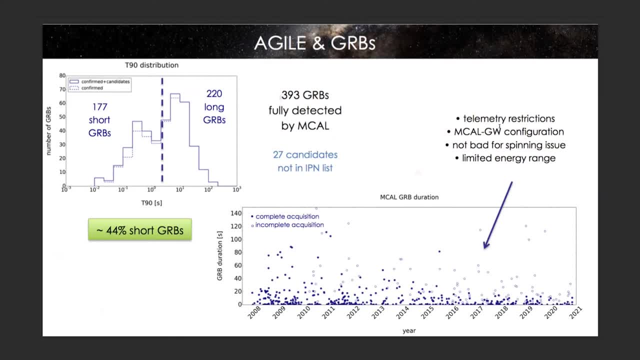 for the whole duration of these events. due to telemetry restriction, we had to to reduce the amount of available mass memory. uh, we exploited this drawback by improving our detection algorithm and mostly focusing on the detection of short-term reverse. and this was done especially in view of the ligo virgo campaign because, of course, short grbs are the most promising candidates to be. 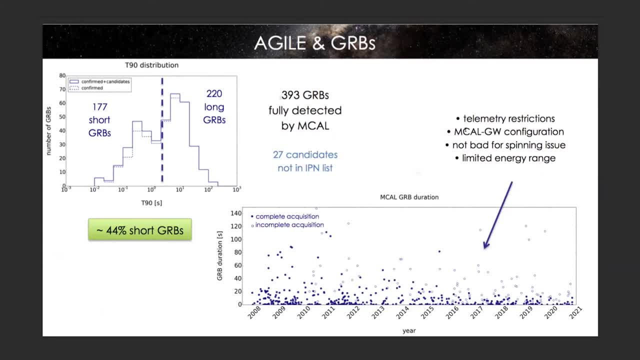 counterparts of the gravitational waves, electromagnetic counterparts, of course, and it's not so bad also for spinning issues, because, as i said before, we are spinning and so if we're observing a very long event, we would observe that under different angles, and this requires an interaction with different response matrices, which is not susceptible to perform. 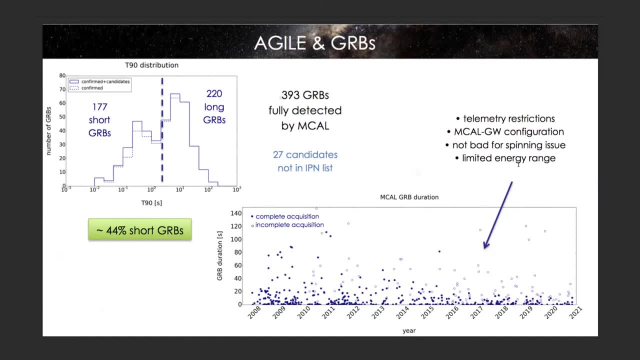 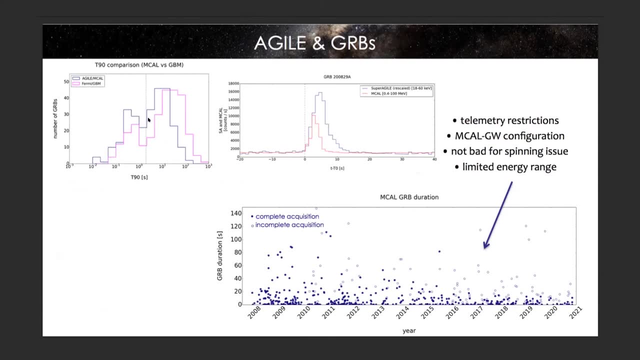 another important point is the limited energy range of mcal, about 400 kg. so if we take a look to the t90 distribution of the same sample, these are about 200 grbs detected both by mcal and gbm. and If we take a look to this distribution we see that MCAL detects T90s which are slightly shorter than the ones of Certifier by GDM, for instance. 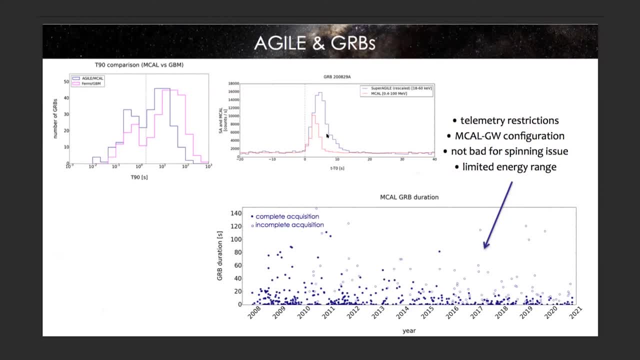 And this is normal because we are just observing a limited portion of the spectrum. So here, in this case, I show an event where SuperAgile detects this GRB in the X-rays and has a certain duration, And you can see that the same event with the same onset here has a very shorter duration in the MCAL energy range. 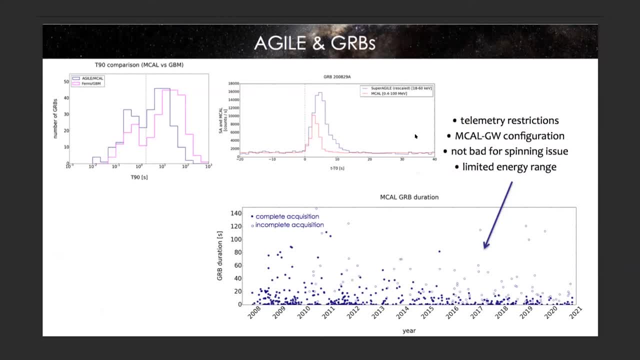 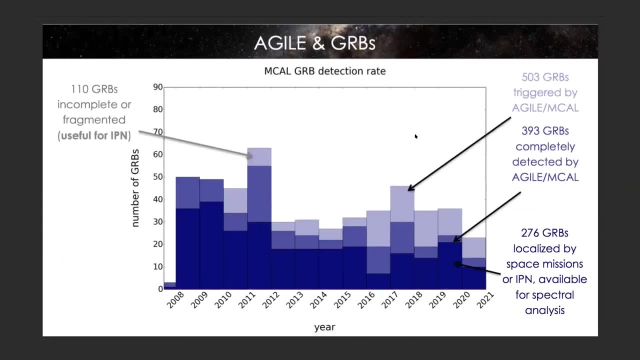 So this is completely normal, that we have T90 distribution mostly biased toward short duration events. Out of these events, we have 276 GRBs which have a localization, of course, an external localization, because I'm talking about the MCAL, which is a non-imaging detector. 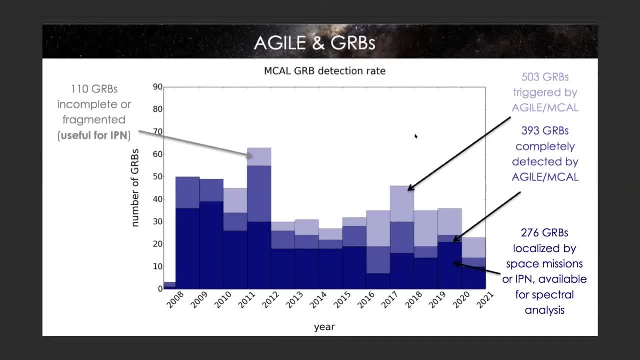 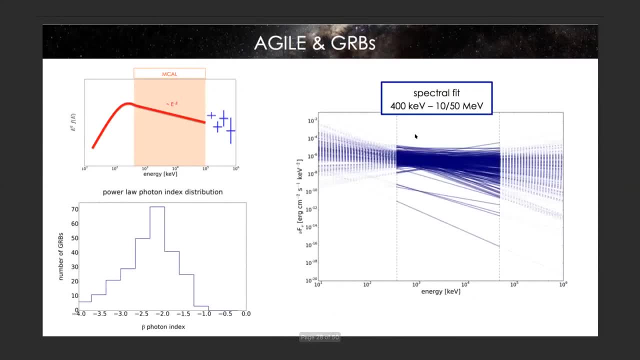 And this localization could be provided by external space munitions or by the IPN triangulations, So we can perform, out of these events, spectral analysis. So, again, assuming that we are just observing the high T90s, we perform an automatic analysis fitting by means of a single power law with a beta for the index, and you can see the distribution peaks at about minus 2.3 here. 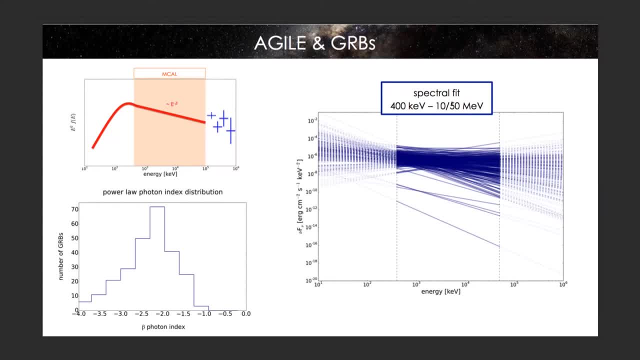 Fits were performed up to 10 or 50 MeV, depending on the statistics, And what is interesting here is that we have about 77 GRBs with a beta which is greater than minus two, So something which, in the new spectrum, has a positive slope. 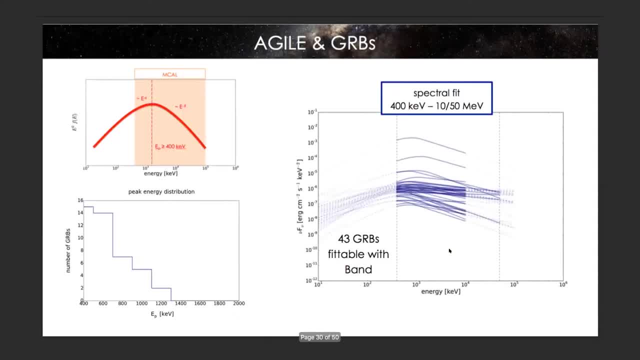 So something that should All the very hard spectrum. Moreover, this is not so simple for us because we start from 400 MeV, but we could also perform a spectral fitting by means of a band model up to 443 GRBs, with a peak energy above 400 MeV. 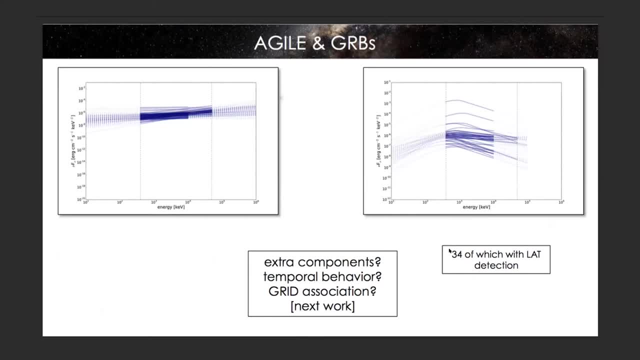 And, of course, these two data samples represent the highest energy GRB sample of MCAL. And this is the object of our forthcoming study here, because we are investigating these events one by one, investigating the arising of extra components. When do these extra components arise? in the temporal behavior, in the temporal and spectral development? 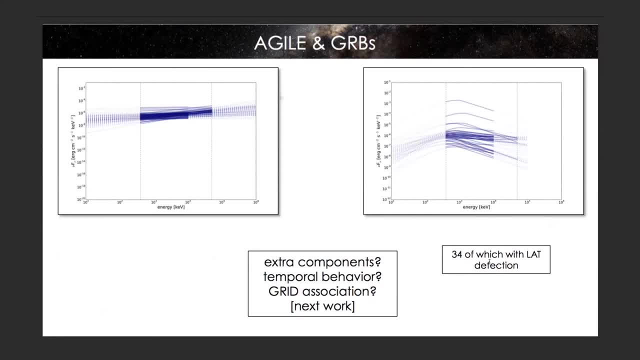 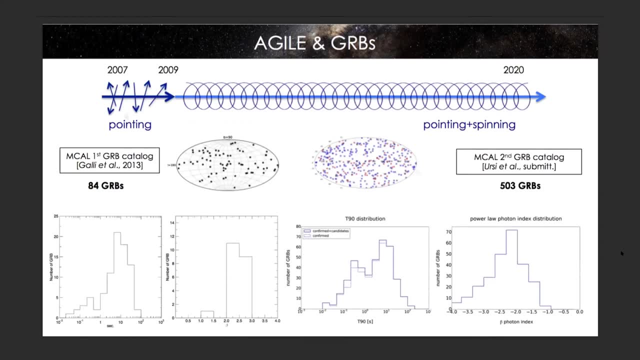 And we also found out that 34 of these events are also observed by LAT, So we have LAT-LAT detection. So they are very interesting. So this is just a final picture of what happened here, with the final distribution of this 400 of these events here in the new catalog which has recently been submitted. 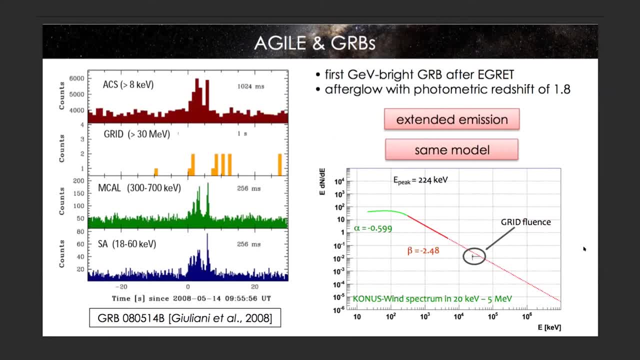 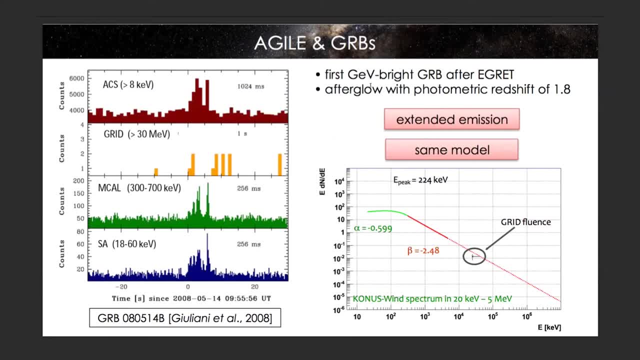 Here we have the first event, 08.05.14b, where the GRID instrument detected a GEV photon, the first event after YGRET. And this is describable by the same model here, by the same band model. As you can see, we have here a joint detection by Conoswind. 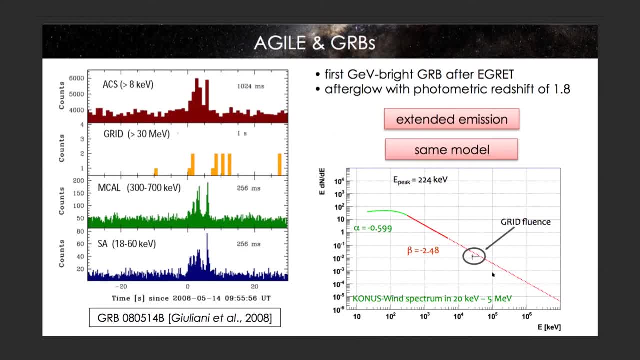 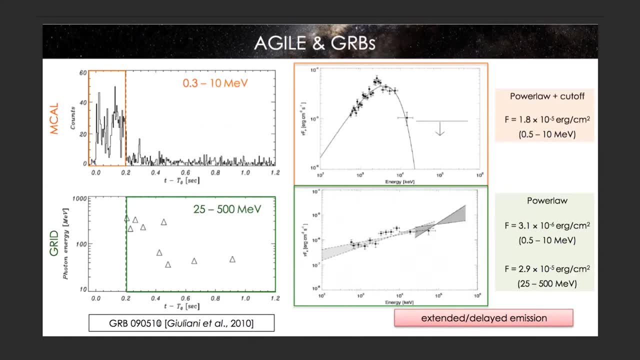 And the GRID fluence perfectly fits with a single band model here. Another very interesting event is this: 09.05.10,, which is the historical GRB thought to be originating. Another very interesting event is this: 09.05.10,, which is the historical GRB thought to be originating. 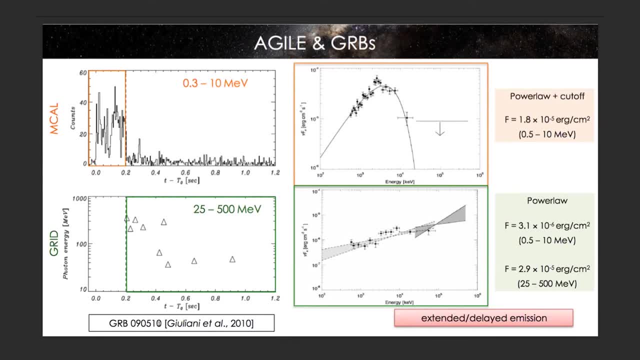 Another very interesting event is this: 09.05.10, which is the historical GRB thought to be originating, And in this case we have, after this very first stage of the prompt phase here detected by MCAL up to 10 MeV and describable with a cutoff power law. 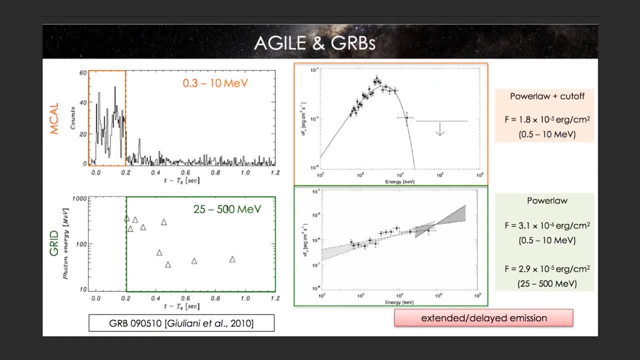 we have the arrival of GRID photons up to 500 MeV with a harder spectrum which is fitable with a power law extending up to the highest energy, So a delayed emission up to the highest energy, And this is a very important event. 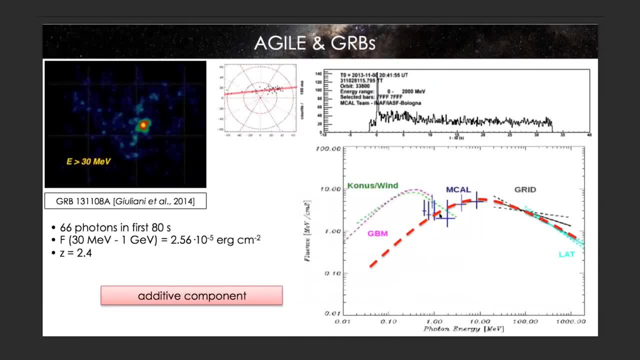 Another event where MCAL data are very useful, with this big shape, let's say, is this one, 131108A, where NCAL links very well the common-screen and GBM data in the X-rays to read and LAT data in high-standard Gs. 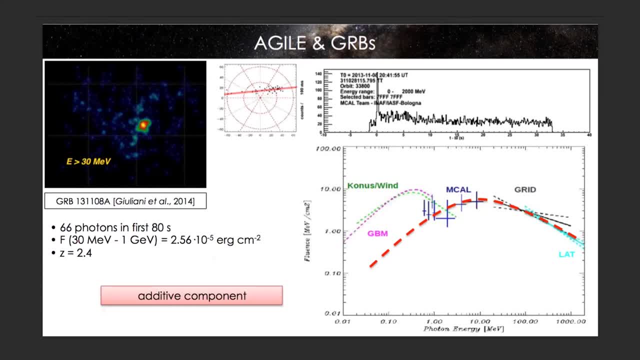 And we also had the localization by means of superagita. here, Of course, we are in 2013,. so, as I said before, we were spinning, so we have here a strip rather than a bunch of photos, but we could provide localization. Another interesting event was this: 180914B. 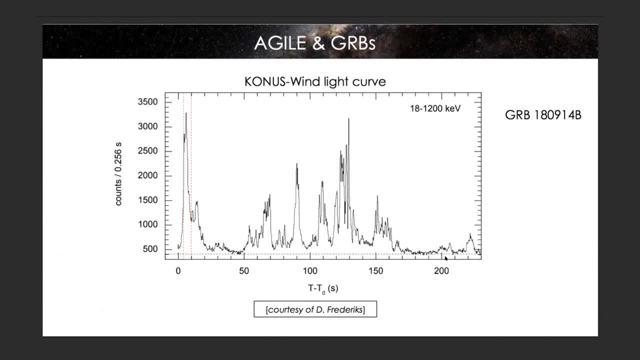 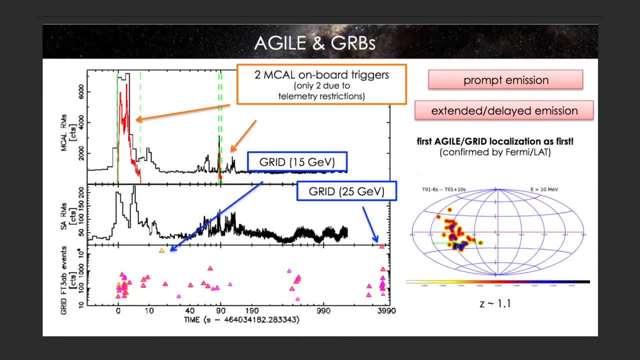 very long, one of the longest GRBs that we observed, more than 200 seconds. This is a light queue of my icon swing because, as I said before, NCAL is not capable of detecting the whole duration. so we just have two limited portions, two limited triggers here, But it's. 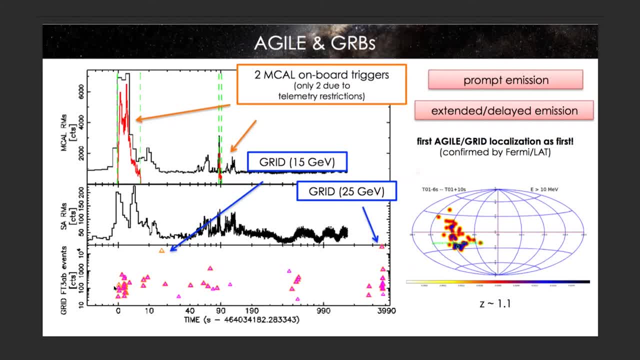 not NCAL, who is very interesting here. It's the grid, because we have a bunch of photons arriving exactly at the TZ work here, which allowed also localization. We arrived as first with localization. This is very peculiar for us, so it was very good. 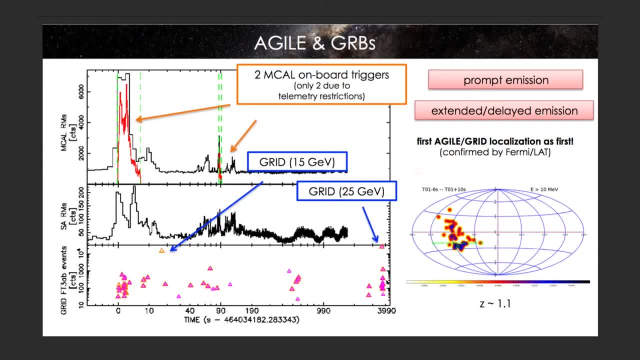 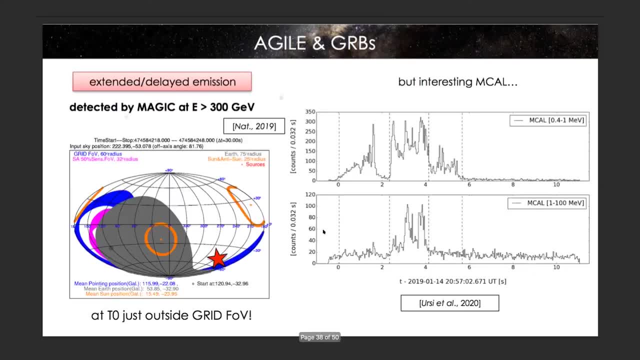 And also these photons arrived for thousands of seconds after up to 25 GB. So this is a very, very strong and intense GRB with the grid detection And the last important GRB that we detected is the magic GRB in 2019.. Unfortunately, it was just outside the grid field of view. 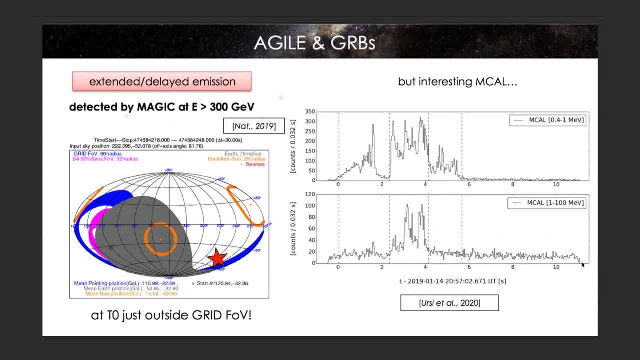 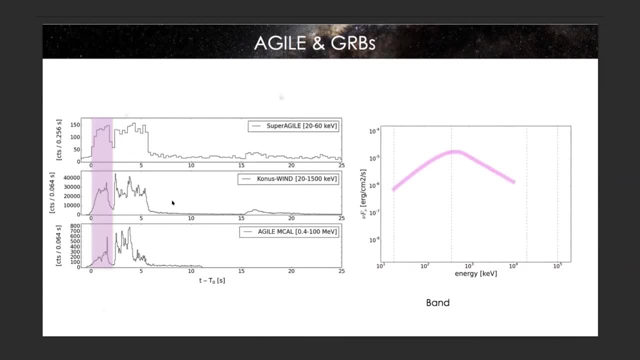 but we have very interesting NCAL data here. an NCAL trigger here lasting 11 seconds, hovering the first five, six seconds of the prompt phase, And we studied this together with cono swim here down to 20 kV. Here you can see also the superagilirate meters down to 20 kV. 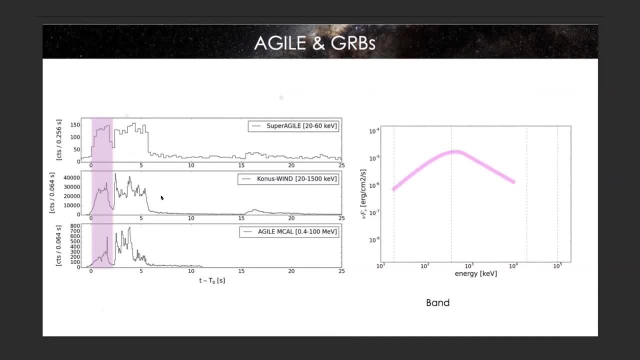 up to 60 kV and, as you can see, this is completely fitable with a band model here. so a typical synchrotron emission. but already during the first stages this is very rare. At early stages we have the rising of this extra power law component which could be the manifestation, for instance, 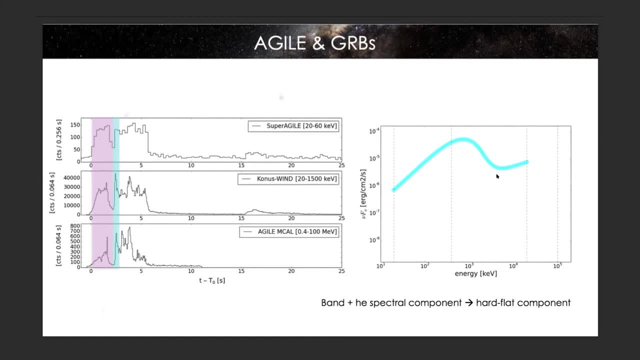 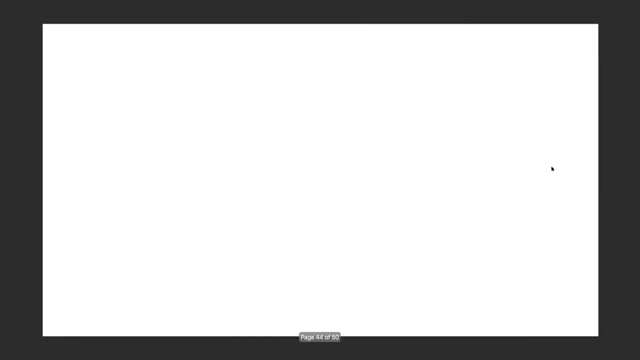 of a different population of accelerated particles emitting synchrotron or inverse quantum here, and this evolves in a sort of very flat component here, very hard component, until we reach a v shape. so there is a separation between the synchrotron component and this flat power law. Here we, we, I inserted here also a spectrum from fermion sweep which fits very 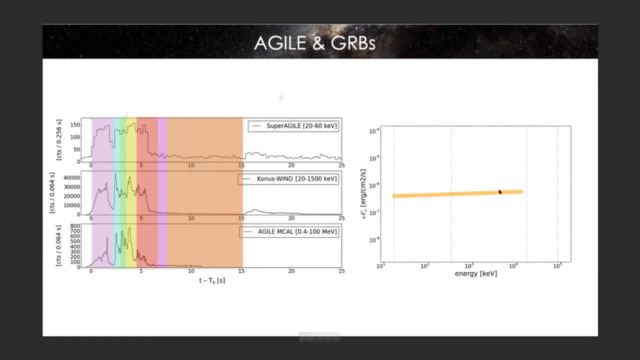 well inside this transition to the early afterglow. and then we have the decreasing, a small reflaring here, observable just in the x-rays, as you can see, by rather than from swing, but not really triggered by M Kalamath 400 PV. so there's no trigger here. 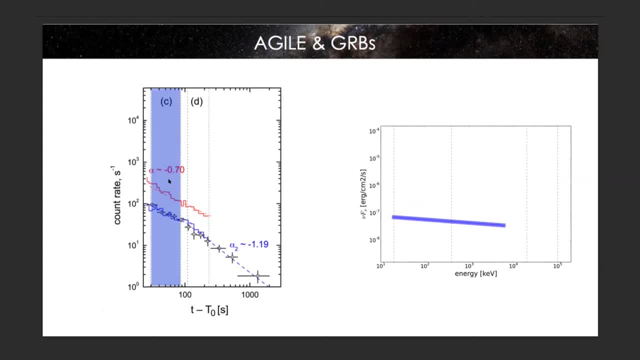 And again we have also this decrease at the very longer times with a break. Here we have a break at about 90, 100 seconds, which is also observed by the spikes of integral here with these three dots, And this is compatible with a fireball. 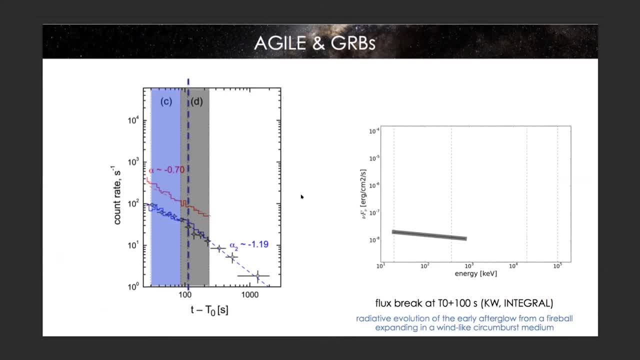 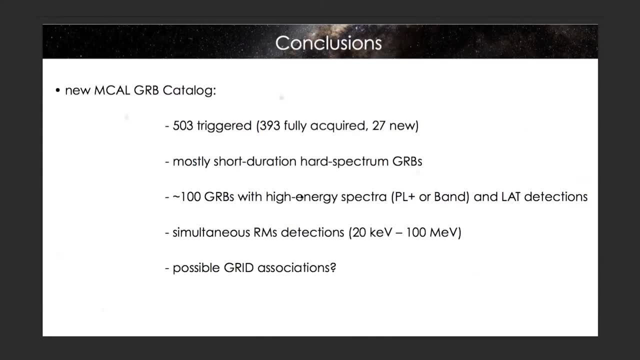 which is expanding and not in a constant density medium, but in a wind-like circumverse medium with decreasing with R to the minus two. So this is just. this was just a brief review about the M Kal GRBs, the Agile GRBs. 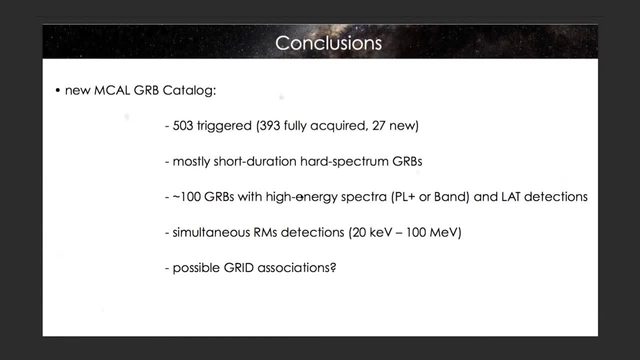 So there is this new catalog, now submitted, with 503 triggered GRBs and 393 fully acquired GRBs. There are 27 new events that should be started without emissions. Of course, our sample mostly consists of short duration high-spectrum GRBs. 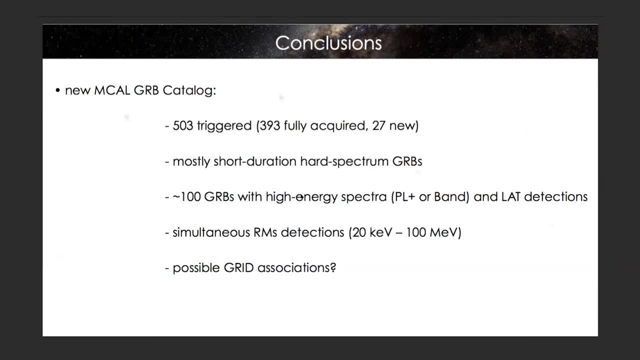 And we have also, as I said before, about 100 GRBs with high energy features. So high energy spectrum, so a power load with a positive slope in the new spectrum or a band model, together with associated LAT detection. So this is the object of a forthcoming study. 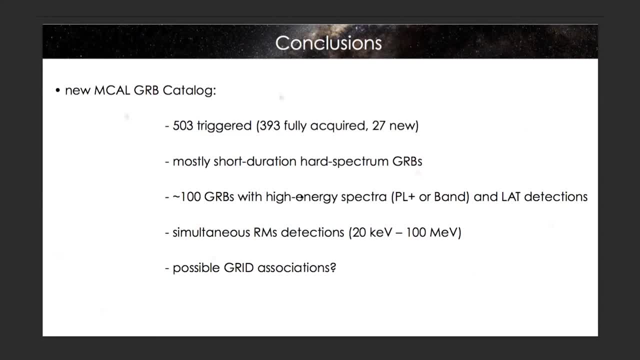 We have also simultaneous rate meter detections which allow to perform a sort of broadband observation of these events, down to 20 kV, up to 100 mEV, And of course we are also studying grid to see whether there are some high-energy photons. 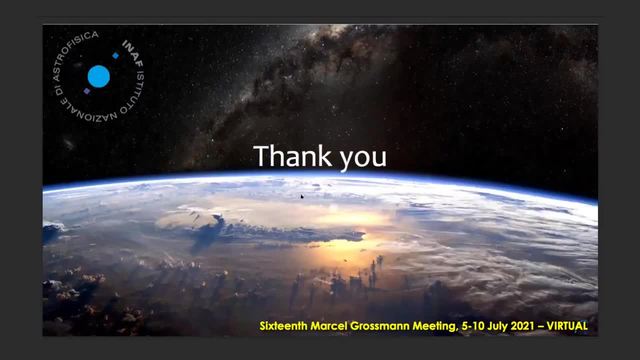 associated to these events. So, thank you, I hope I wasn't on time. Yes, Alessandro, perfect, You stayed up to in time 16 minutes or something. Thank you. I have some minutes for a question to you, So are there questions to Alessandro? 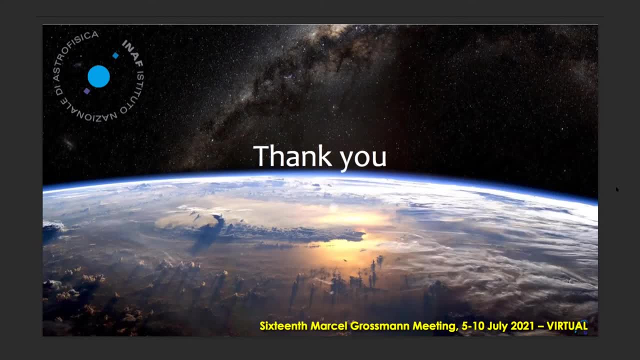 So, Fabian, please, Ciao, Alessandro, Thanks a lot for this nice talk. I might have missed it, but maybe you can say a few words about the time scale you need to produce alerts, so from the detection to the submission of GCNs or things like that. 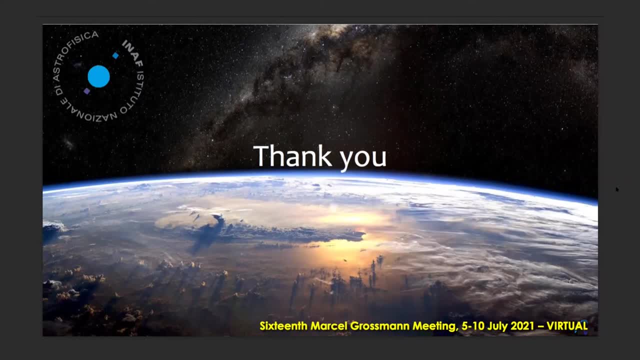 Yeah, actually it depends on the third passages. Actually, in the best case it could be something all about, let's say, 20, 30 minutes, because if we detect a GRB just before the passage over Malindi, over the telemetry ground station, 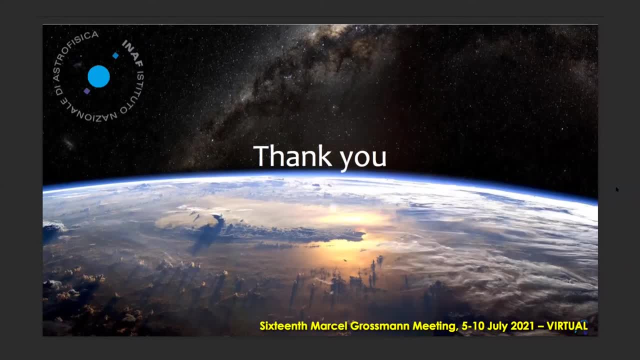 of course, there is just the time due to processing, And it's about, I guess, 15 minutes or something like that. Yeah, So it's very fast, But, of course, if we detect something just after the passage over Malindi, where we downloaded the data, 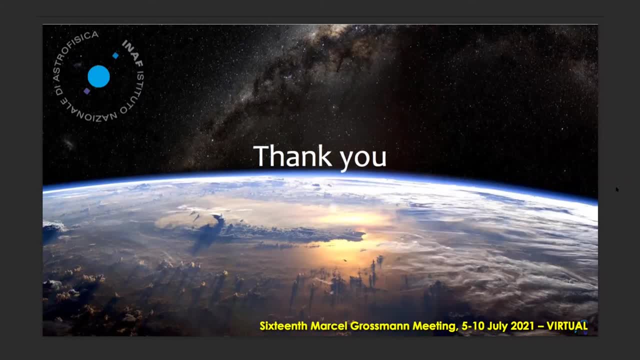 we have to wait another 90 minutes, 94 minutes, before we download the telemetry to the ground station. So it's variable, unfortunately, But in the best case, yes, something like 15 minutes just to process all the data, the raw data. 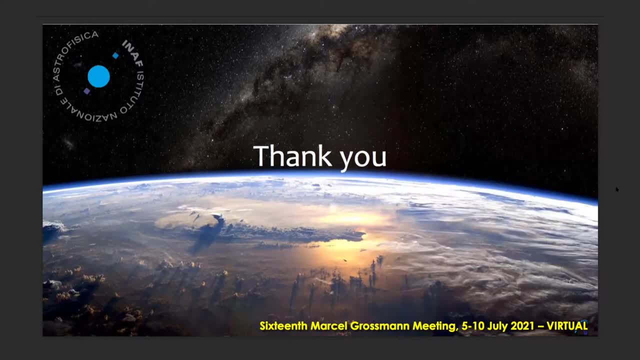 and produce something and deliver something to the community. OK, thanks a lot, You're welcome. OK, thanks, Alessandro, for the answer as well. So is there time for another question? if any, OK, so if not, we thank the speaker again. 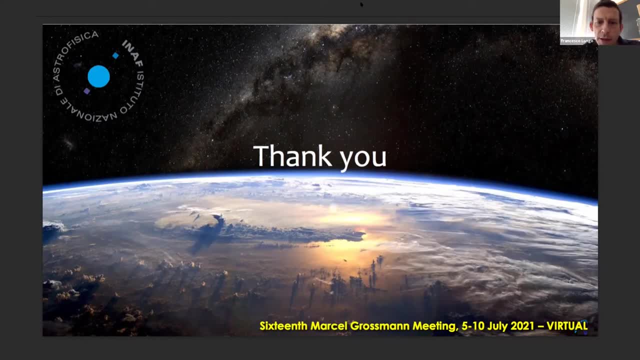 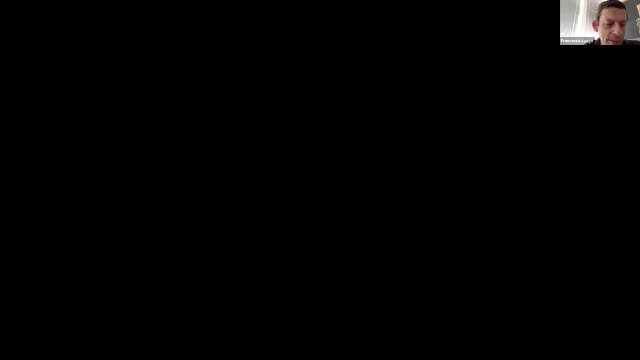 Thanks, Alessandro, for the nice talk, And then we move to the second topic of today. So Elisabetta will discuss about Fermi, GBM and LAT results about gamma-rebbers. So, Elisabetta, please, OK, can you hear me? 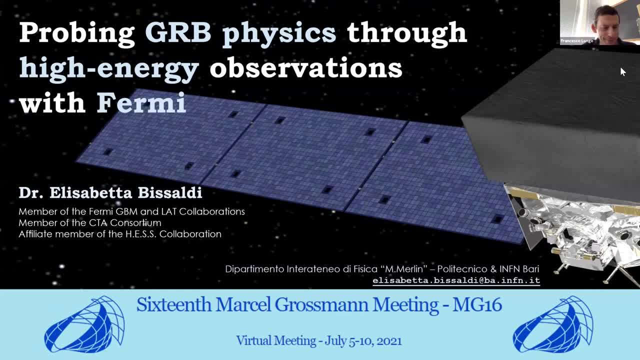 Can you see my screen? Perfect, Go ahead, Oh, OK. OK, so I will talk about high-energy observation of gamma-rebbers with the Fermi telescope. I will talk on behalf of a pretty large collaboration because I will include the results by both the GBM. 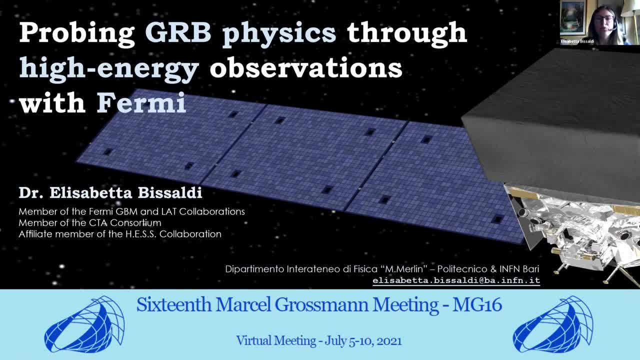 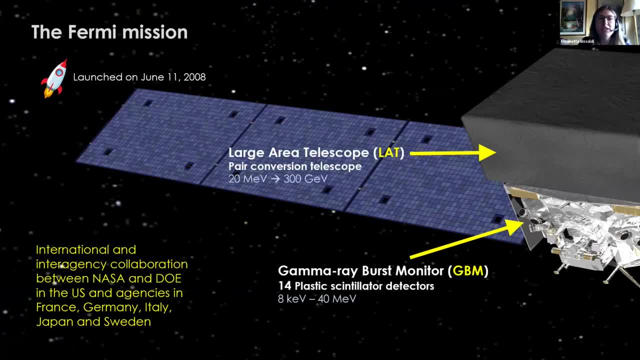 and the LAT instruments. So let's move forward. OK, If my slides are OK. So you all know what the Fermi mission is. It's taking data since 13 years now And you know we cover the lowest energies with the gamma-rebbers monitors, scintillator detectors. 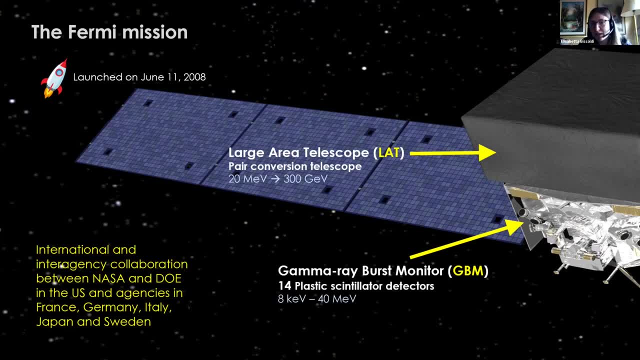 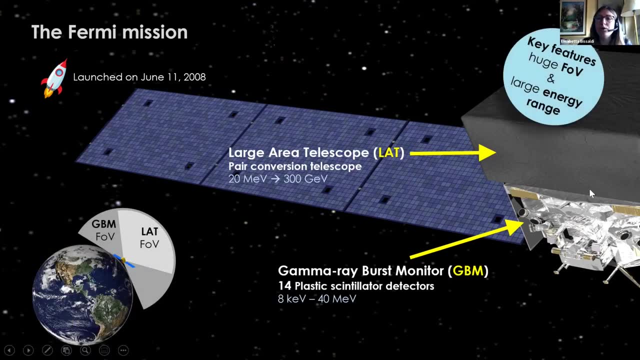 between 8 kV and 40 mEV and the highest energies. with the large-area telescope from 20 mEV to more than 300 gV, We have a very large field of view which is ideal for catching transient events like gamma-rebbers. 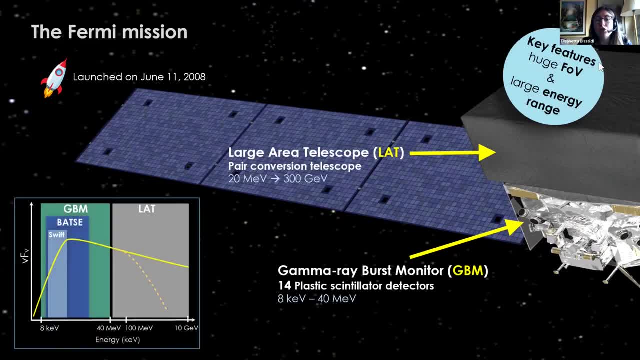 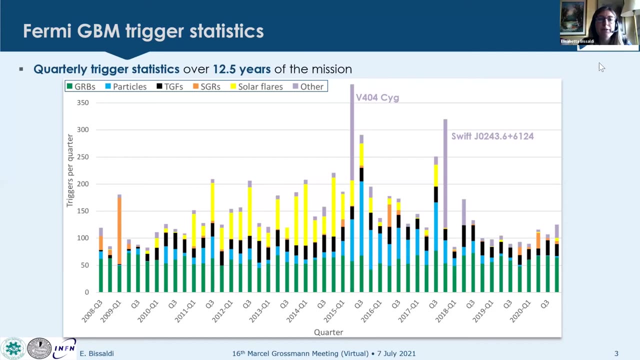 apart from the large energy range, which is also very nice because we can cover the spectrum of a typical GRB in a very nice way, as it is shown in this cartoon in the bottom left. So, starting from the GBM, let's say highlights. 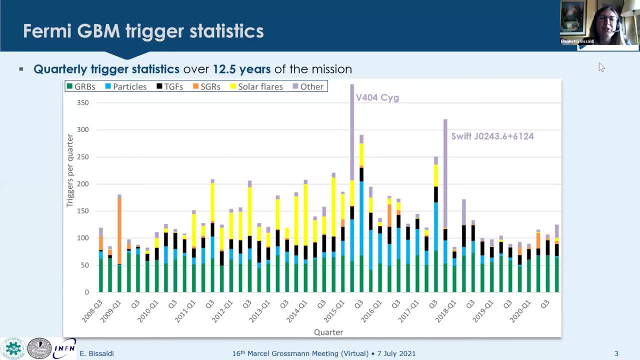 you can see that GBM does not only trigger on gamma-rebbers. Here you have the trigger statistic over the past almost 30 years, and all of the different different colors tell you that there are different transients that are triggering GBM. 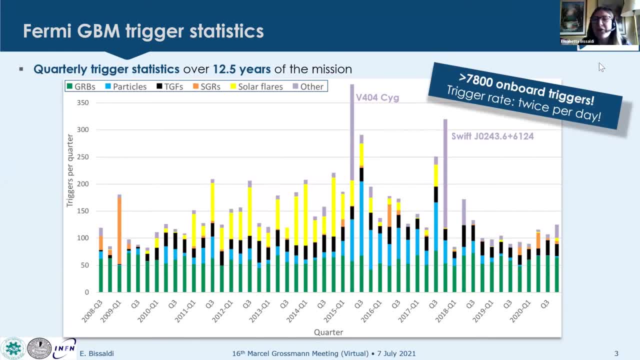 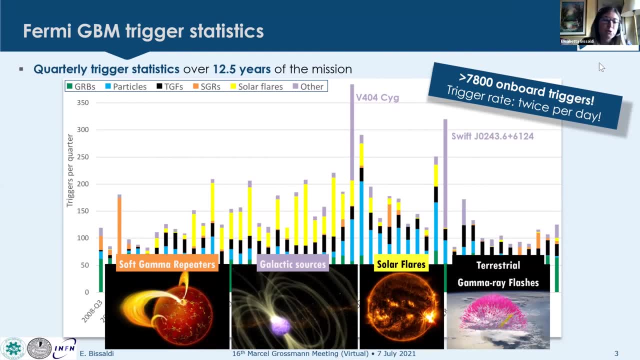 So we had more than I mean at least almost 8,000 or more triggers, which means almost twice per day, And we trigger on also soft gamma-repeaters, like in the last couple of days. galactic sources, solar flares. 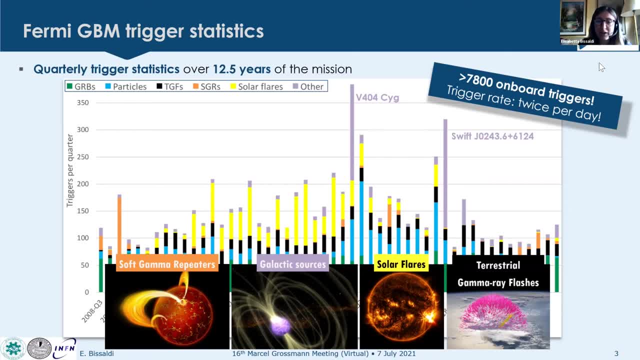 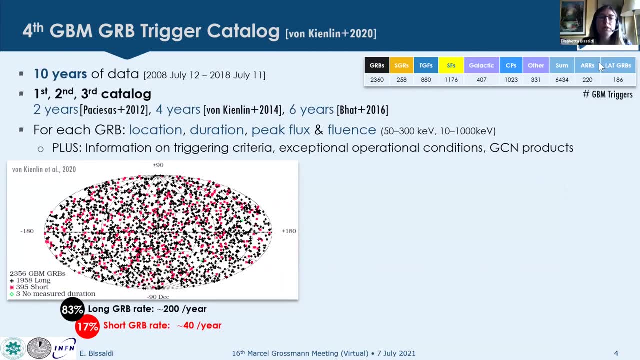 TGFs. So we have really lots of transients populating our trigger statistic. But let's move to gamma-rebbers. So the last catalog that we published this year it's the 10-year trigger catalog, following the first, second, third catalog. 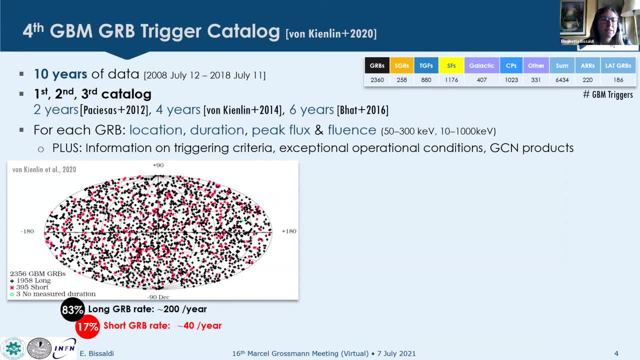 So in this kind of catalog we, let's say, we put the location, the duration, the peak flux and the fluence for each event, Plus we have all of this information on triggering criteria, exceptional operational conditions and all of the other things that you might be. 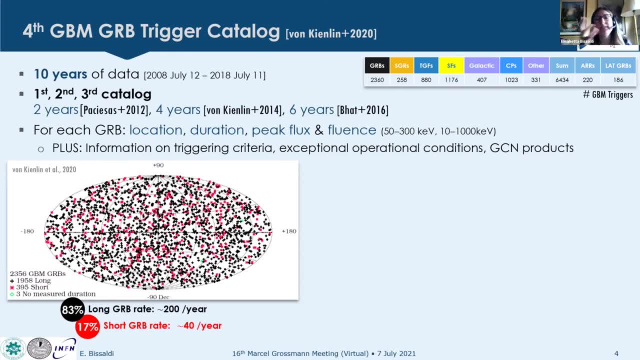 let's say interested in. So here you can see the sky map of all the events. Red and black are short and long gamma-rebbers. You see, if you simply divide the gamma-rebbers as usual with the two seconds, let's say rule as we know it. 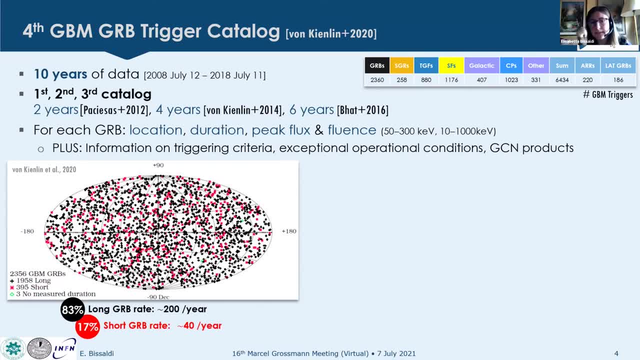 we have about 83% of long ones and 17% short ones, which means almost 200 long and 40 short gamma-rebbers per year. As of today, we have 3,100.. GBM- Actually, I think it's 3,099.. 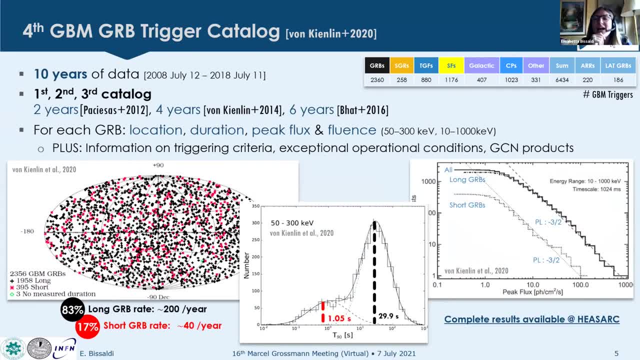 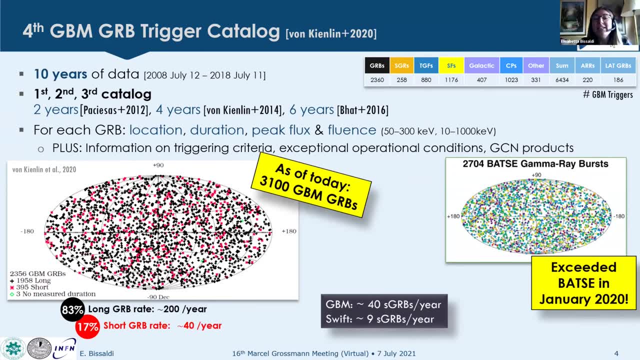 But, OK, I rounded it up at 100.. And it's worth noting that, OK, we exceeded BATSE already in January 2020, so it's been a long time, And I want to stress that GBM is a very nice instrument. 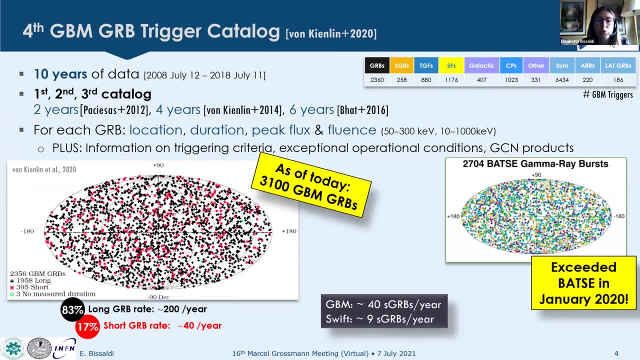 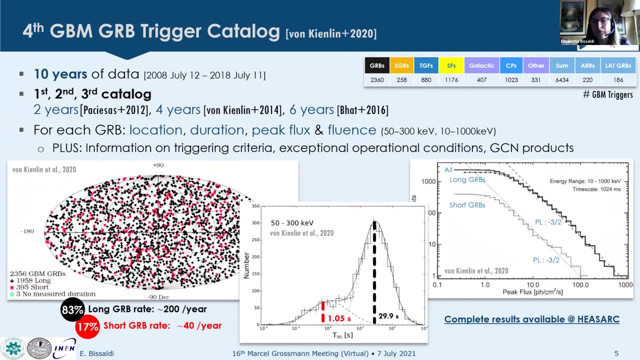 for short gamma-rebbers detection because, for example, with respect to SWIFT, we detect almost three, four times more than this. In the catalog you can find all of the short gamma-rebbers And if you look at all of these, let's say distribution. 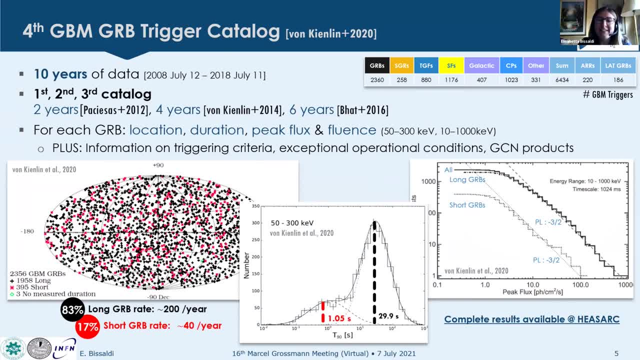 like, for example, the duration distribution which we already saw from the Agile results a few minutes ago. you see, these are the median values, one second and 29.9 seconds for the long and the short, And it's very interesting that if you look at the intersection, 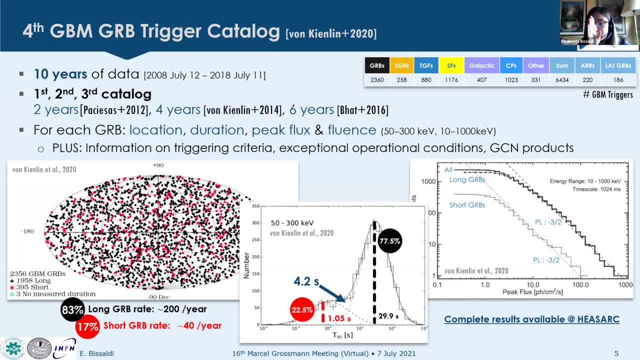 so the intersection is more or less at about 4.2 seconds And if you divide the long and short at this intersection you get a higher number of short ones, I'd say a higher percentage of short gamma-rebbers. The short ones are up to 22.5%. 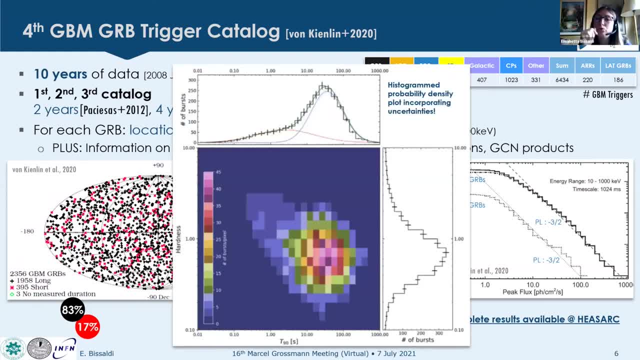 And if you include also the uncertainties. so if you do a histogram probability density plot incorporating the uncertainties, then you get an even higher percentage, let's say, of short bursts, And we go up to 26%. If you are interested, please go to the catalog. 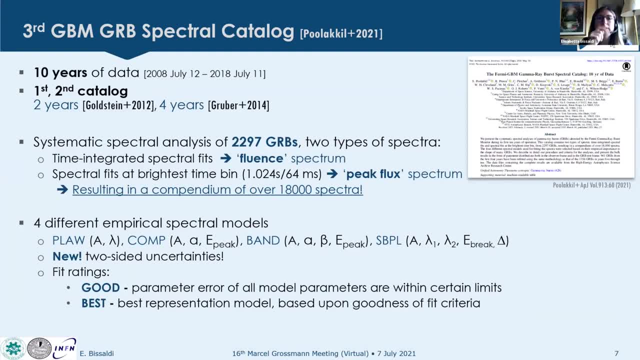 and look at the details. So, moving to the spectral catalog that was also published this year, so we have it's the same Time period, another 10 years following the first and the second spectral catalog. It's a systematic analysis of almost 2,300 gamma-rebbers. 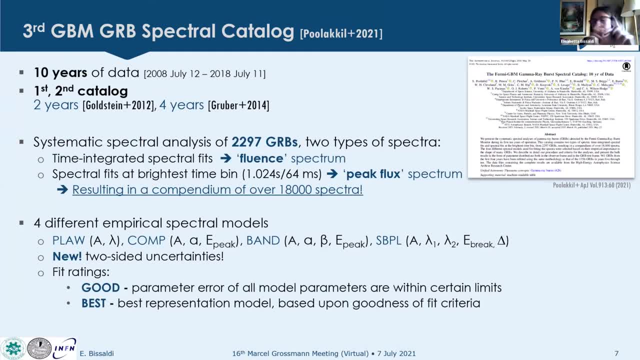 And there are two types of spectra: the fluent spectrum, so the time-integrated ones, and the peak flux spectrum of the brightest time beam. They are always fitted with the four, let's say, empirical spectral models, power law, Comptonized band. 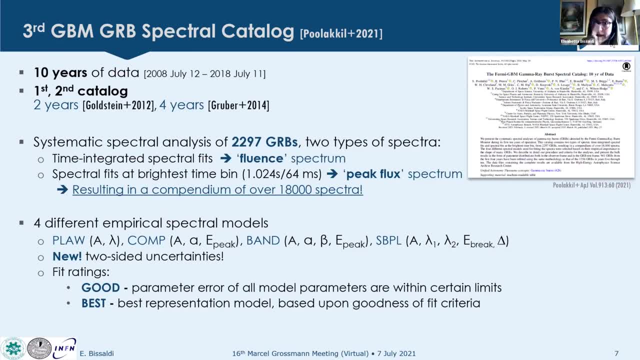 and the smoothly-broken power law. We have two-sided uncertainties, which is new. We respect to the older catalogs, And then you have always this division in a good and best subsample, so to say, regarding the goodness of the parameters that you get by fitting your data. 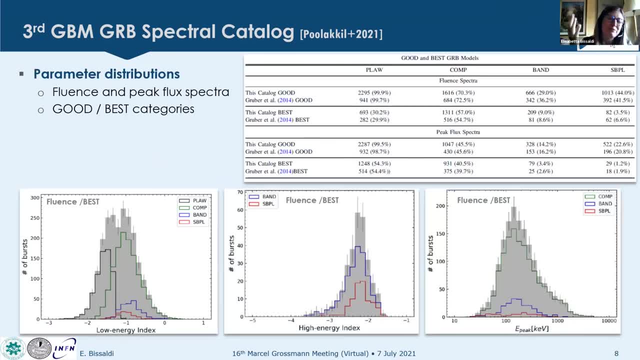 So here there are lots of distribution, lots of plots. I just made a very, very small. let's say: you have a selection, let's say, of results, because there are really really many results. So you have a selection of results because there are really really many results. 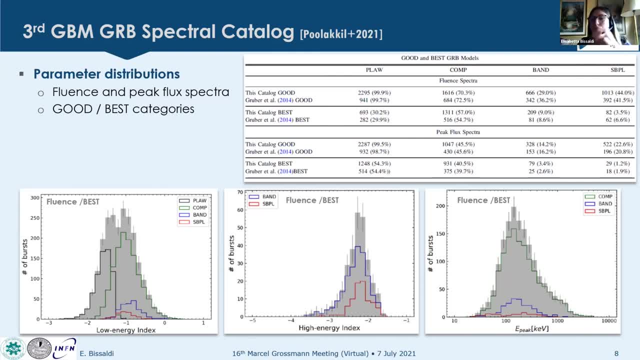 So you have a selection, let's say, of results, because there are really really many results Here. in this table, for example, you can see the main results for all of the four spectral models, for the fluent spectra and for the peak flux spectra. 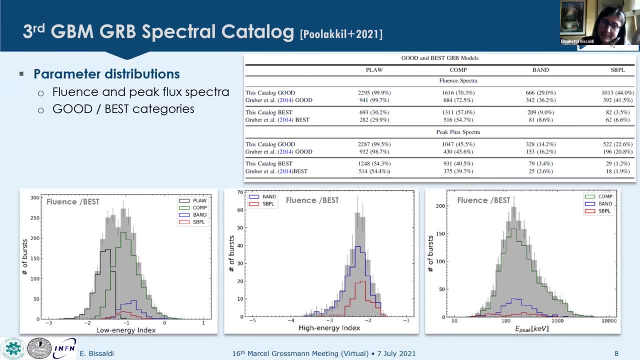 The plots here just show the fluency and for the best category, not the good one. So I mean you have all of the other distributions in the paper if you are interested in. It's nice to see what the medium values are of this distribution. 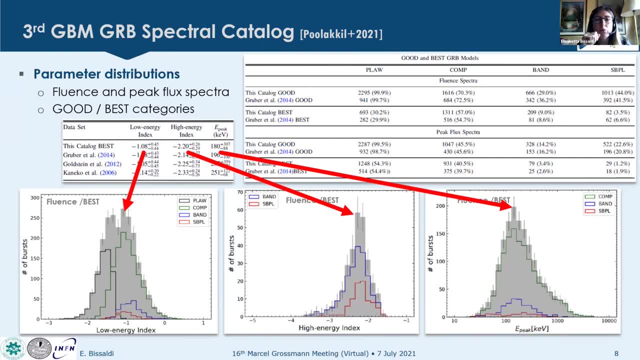 You see alpha around minus one, beta around minus 2.2, and epic this is for, let's say for for all of our models. You see, here you have the different components that are in color, and then the gray is the full distribution. 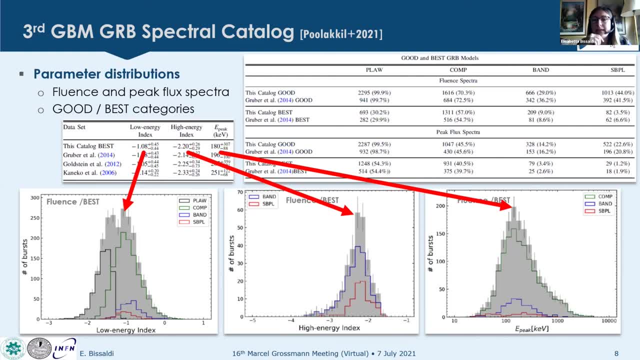 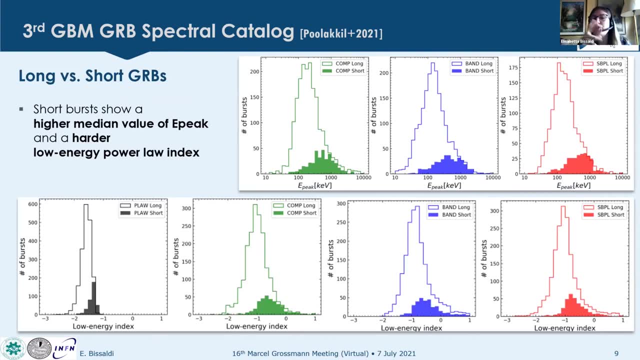 Epic is around 180 kV. It's also interesting to see what is the difference between long and short gamma-ray bursts to see, And we find again I mean something that was found also in the literature, So to say that short bursts have higher medium values of epic. 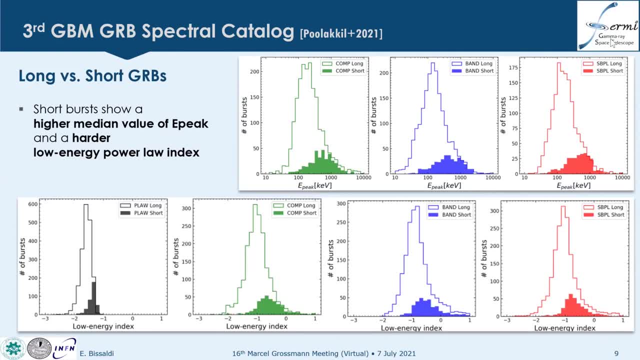 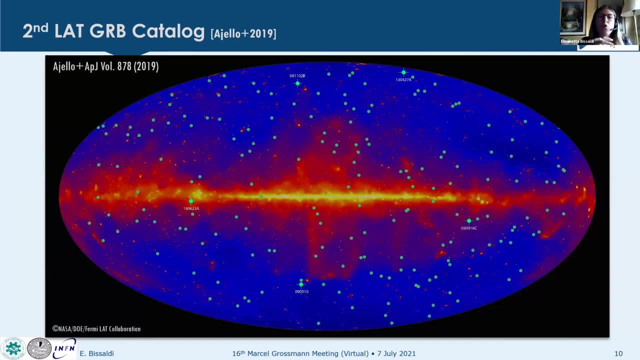 and also show harder low energy power law Indexes. so I will flash these very, really fast And let's move to the higher energies. So let's switch now to the Large Area Telescope. We published our second GRB catalog in 2019.. 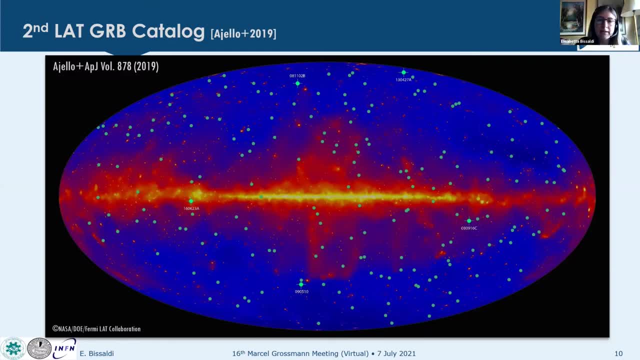 Here you see the very nice sky map that was produced by the NASA Goddard Media Group showing all of our detection in green. These are 186 GRBs, 169 long and 17 short. also is divided with the data, So you can see here. you can see here. you can see here. 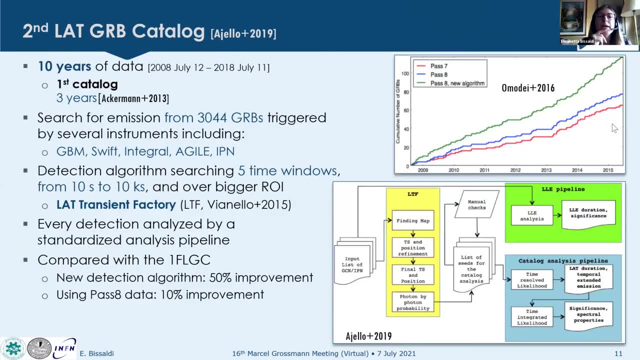 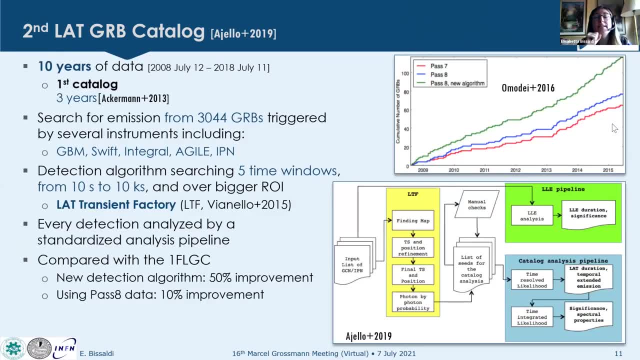 So this is the standard two-second rule. So it comes after the first catalog, which just had the three years of data, So it's a much bigger increase. We checked, indeed, not only GBM triggers, but also triggers coming from Swift, from INTEGRA, from Agile, from the IPN in general. 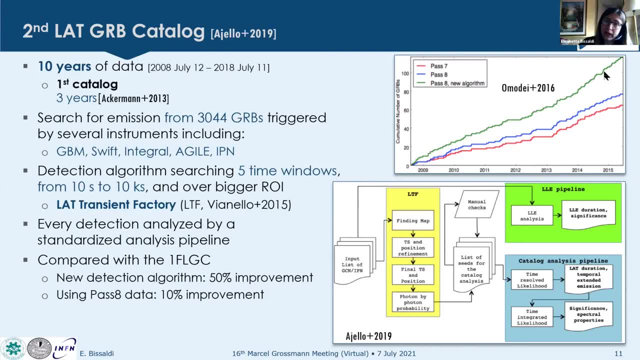 We performed the analysis with an improved algorithm with respect to the first catalog and we got a much higher improvement in the detection rate, as is, As you can see in this graph here on the top right, getting up to a 50% improvement. with the new algorithm and also using, when we switched many years ago now to the past eight data, we also gained another 10% of improvement. 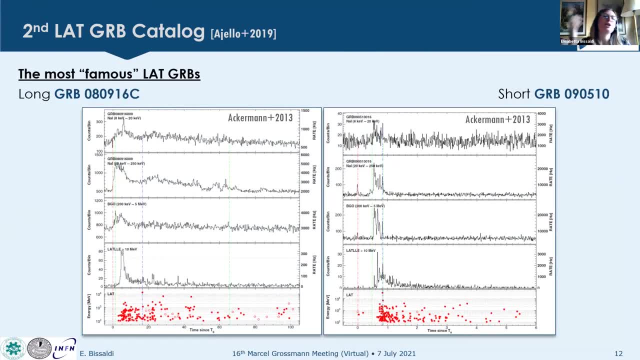 And so we arrived to a much higher number of detection. Okay, I wanted just to put the most famous GRBs- Alessandro already mentioned them- the most famous long one, which also- I mean all of these bursts- happened at the very beginning of the mission of 8.960C, which was published in Science, and they're also the very famous 9.510.. 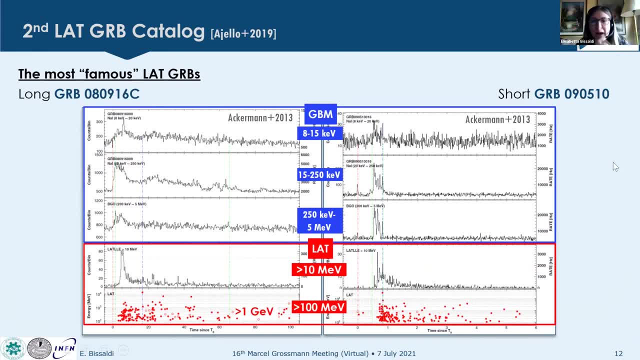 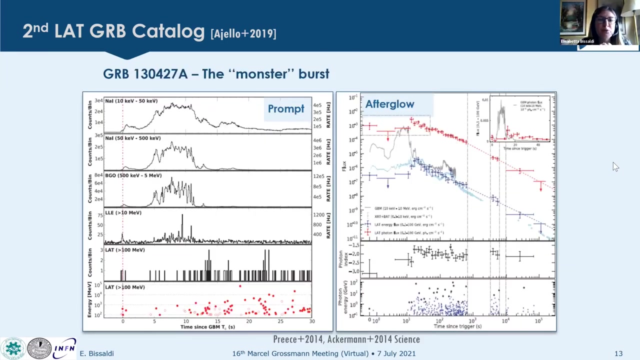 And usually we always, when we publish these nice bursts, we always include the gamma reverse monitor light curves on the top so that you can see really how the gamma reverse evolves In every energy band, from the lowest ones to the highest ones, as I said. so, one was published in Science, the other one was published in Nature, and then the super famous 1304278, the so-called monster burst, which was until recently our best, let's say our best candidate for very high energy detection, because it had the famous 95GV photons. 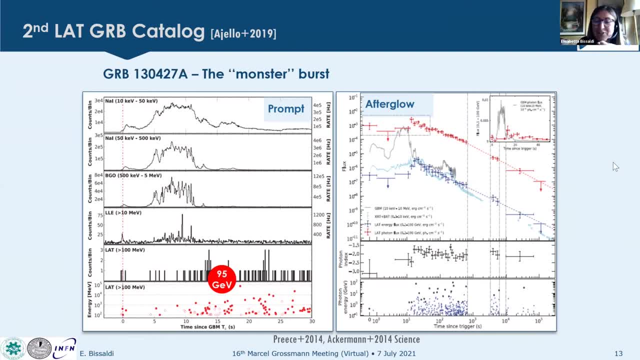 And, as we know, Veritas was almost there in catching this burst, Unfortunately, because it happened. I mean it lasted almost 20 hours, the Latte afterglow, so they were almost on target and it was really a pity that it could not be seen by Veritas at the time. 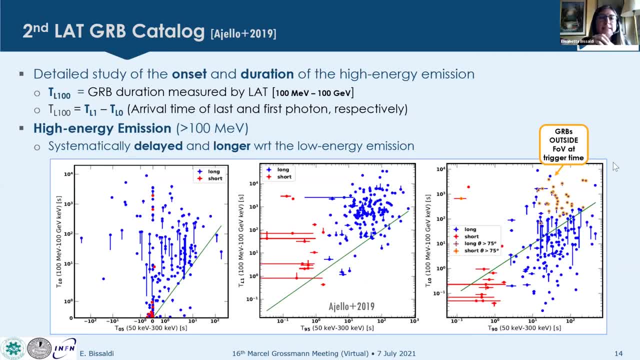 So let's go a little bit into the Latte results We present again. this is just a very small subselection of plots and of results. It's very interesting to study the temporal properties of gamma reverse at high energies. So we did a very 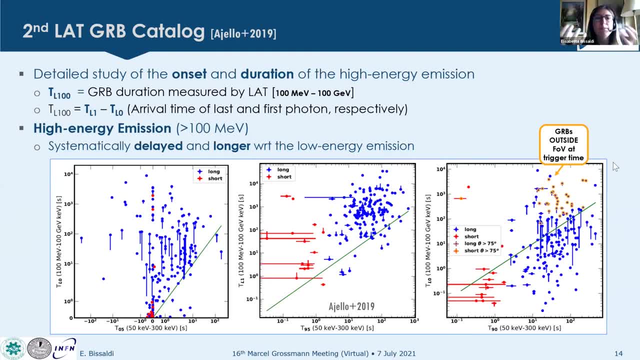 We did a very detailed study of the onset and of the duration of the high energy emission in the typical Latte band, So from 100 MeV to 100 GeV. we see, as we already saw in the first catalog, but here we saw it even more- I mean that the high energy emission is always systematically delayed and it lasts much longer with respect to low energy emission. 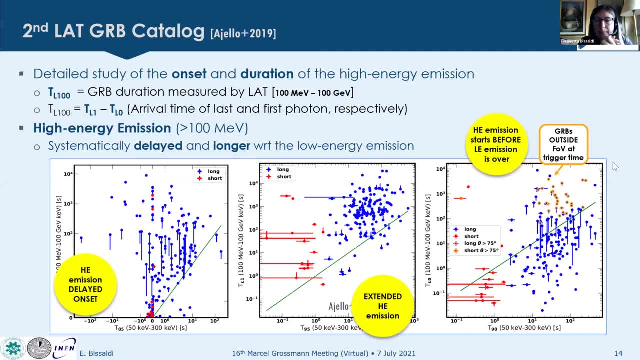 So I put here a subsample of plots, let's say, highlighting this process. It's also interesting to note in the very last plot on the bottom right, that the high energy emission usually starts before the low energy emission is over. So it's not always that you have the GPM and then the Latte comes at some point, but for many bursts we have the high energy emission that is kicking in while the low energy emission is still there for really many bursts. So we compared the properties ofísimo spruts, where at the very beginning there was a lot of particulate rage in the high energy emission and the very last plot. we can write that the high energy emission is now starting before the 내�ggie emission enters the low energy emission. We compared the properties of the high energy emission following the low energy emission. So those are the missing forests. So we compared the properties of the low energy emission that have been lost Also. so again we tried to find out what were the only possiblefyament for these huge numbers in the pop up. 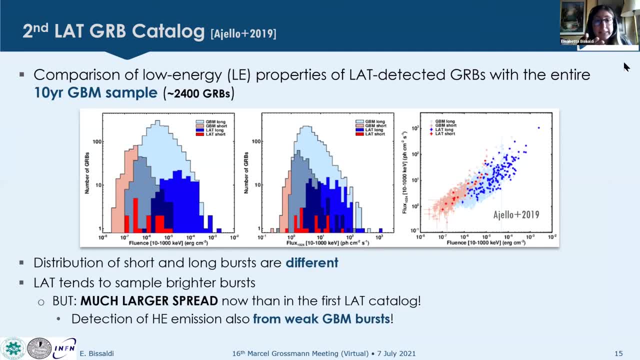 the properties of the lat burst with the 10-year GBM sample. and what I want to stress is that, with respect to the first catalogue, we do not only catch, let's say, the brightest GBM burst. so once you say, okay, this is a bright burst in GBM, we have to see it with lat. 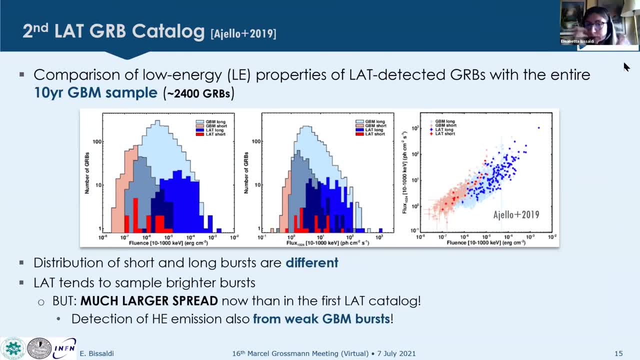 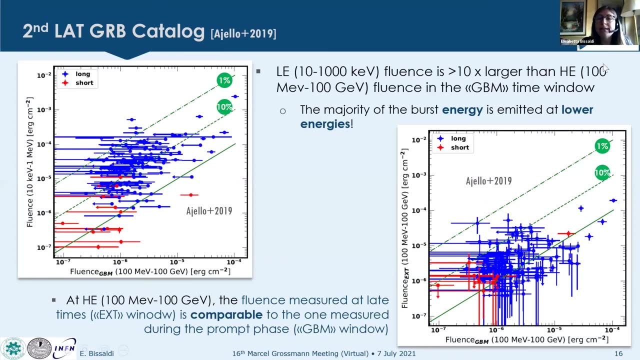 We also saw the afterglow of very faint GBM bursts. so also high energy emission from weak bursts is not something, let's say, that you can simply rule out. Also, regarding the, let's say, the energetics of lat gamma-ray bursts, it's interesting to see that if you study the emission, 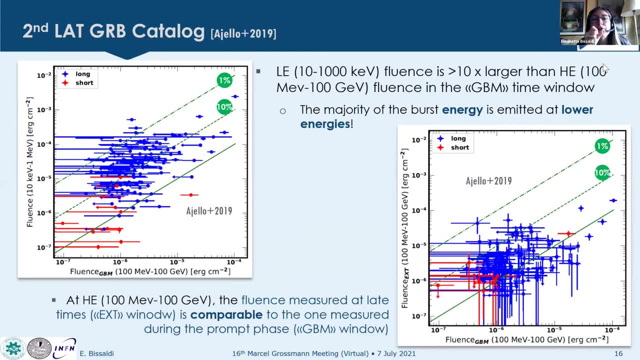 the fluence, so to say, in the energy band of GBM. so 10 kV to 1 eBV in the GBM time window. you see that the fluence at low energies is 10 times larger than the fluence at high energies. so most of the burst energy is emitted at low energy. 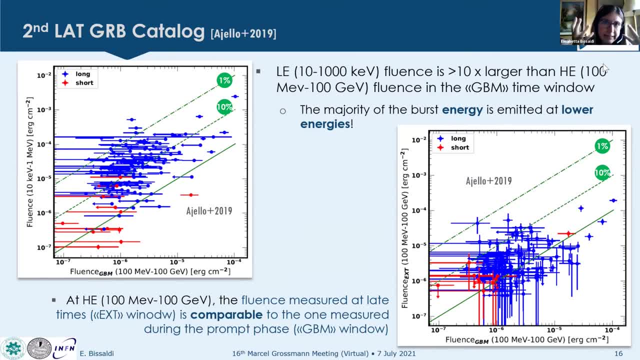 in the window of emission of the GBM, let's say in the T90 window, while if you move then to the so-called what we call in the catalogue, the x-th window. so if you move to, let's say, 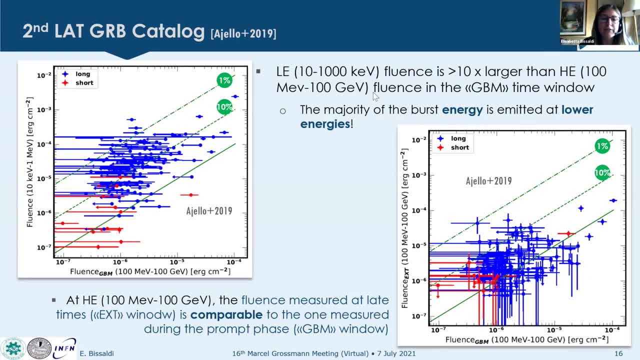 longer time scales, so the time of the extended emission of the lat. then you see that the fluence measured in this time window is more or less similar, comparable to the one that was emitted during the GBM time window. You have many more of these results. I mean, this is just a super short selection of highlights that I wanted. 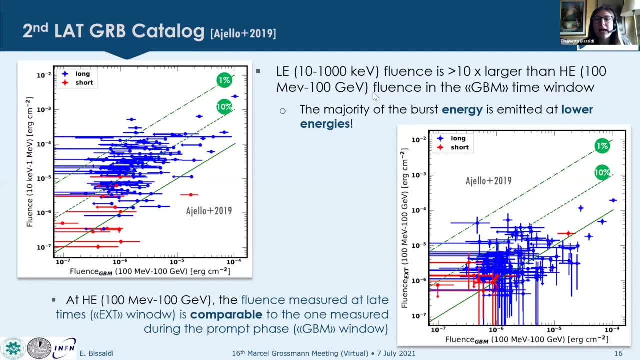 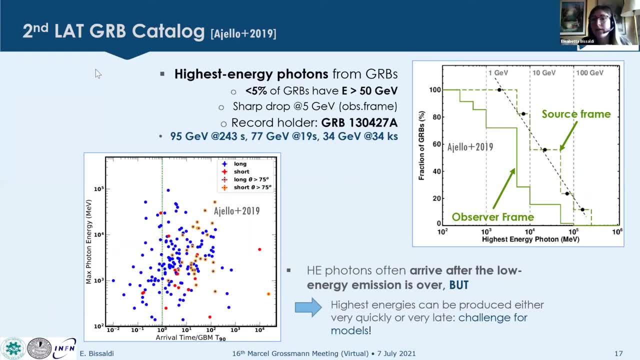 to show you here If you are interested. you have all of the full results in the catalogue. The last thing that I wanted to mention is the fact about the highest energy photons. As I told you, our record holder in Fermi is still 130427A, with the. 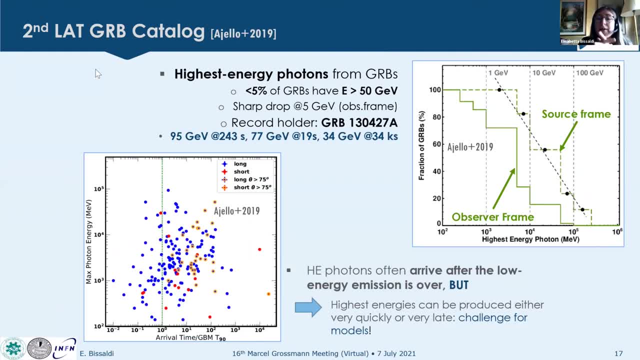 95 Gb. but we found also other very high energy, well, very high energy- for lat photons, always coming from 13427A, so 77 Gb. Then we have all of these photons at around 30 Kb that were seen also. 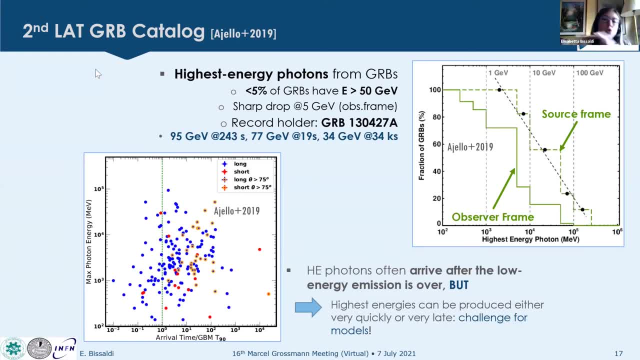 in the famous first burst, and so we made several distributions about this event, and we did not find a clear path. I mean that these high energy photons can arrive often when the low energy is over, but it's not always the rule, because sometimes they can be also produced very quickly. 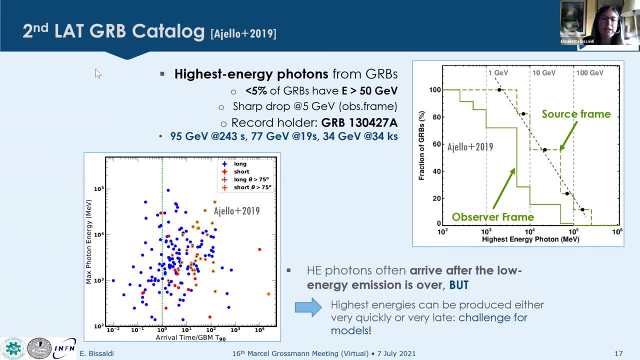 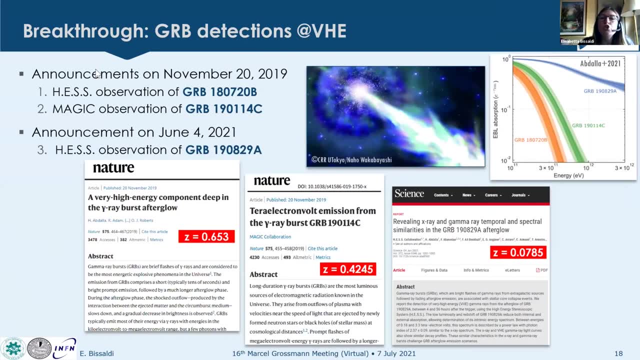 or sometimes super late. So I mean, this is really a challenge and I think that Yoni will discuss this in the next talk even more in detail. So, moving to something that we already discussed largely on Monday, so the very high energy detections of gamma-ray bursts. So the breakthrough came with these very beautiful 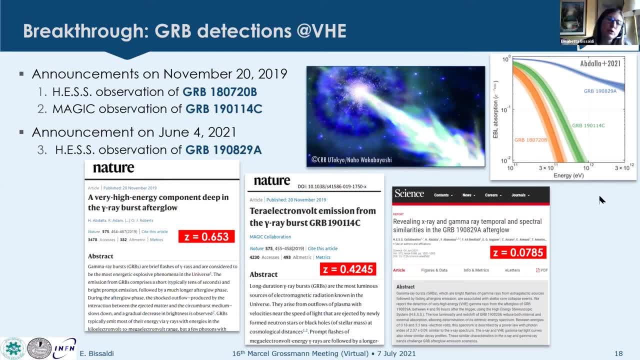 bursts Seen by Hess and by Magic in 2018 and 2019.. And I just wanted to stress, let's say, the role of Fermi, in particular Fermilab, but also Fermi GBM- in the detection of such nice events. Obviously, 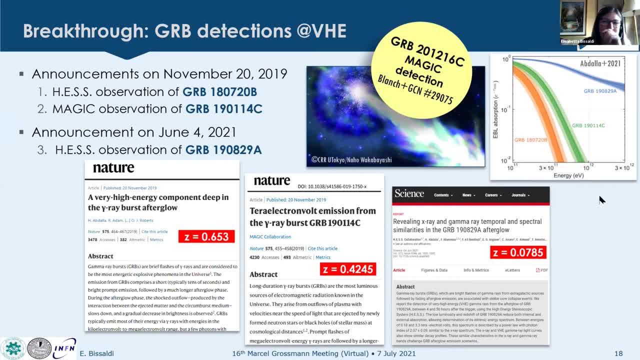 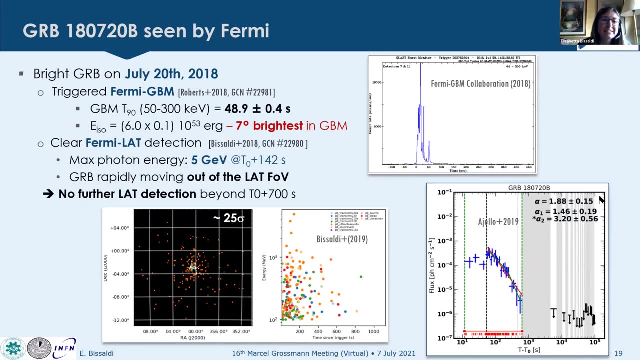 there is also that we already know. there is also the other detection that is still not, let's say, published, but there is the GCN about this event that was seen in December last year. So, starting in chronological order from 1807-20b, So this was a very bright GRB and it was super bright. 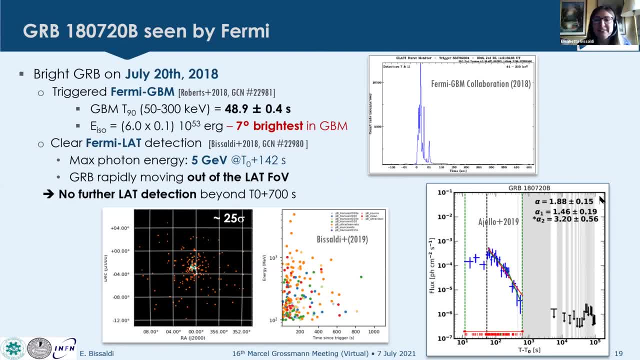 for GBM. It was one of the brightest among all of the GBM bursts ever recorded. It was a very nice and clear Fermilab detection. Actually, this is a burst that is in the catalogue. It's one of the last bursts of the second LAT-GRB catalogue, Unfortunately. the photon, the maximum photon. 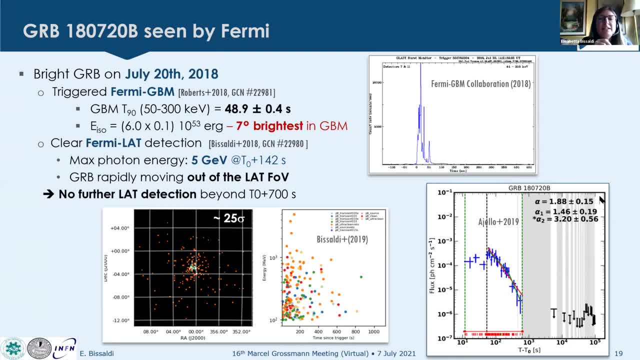 energy was only 5 Gb, So the maximum photon energy was only 5 Gb. Unfortunately, the maximum photon energy was only 5 Gb, So not spectacular, And even more unfortunately, the GRB was rapidly moving out of the LAT field of view. 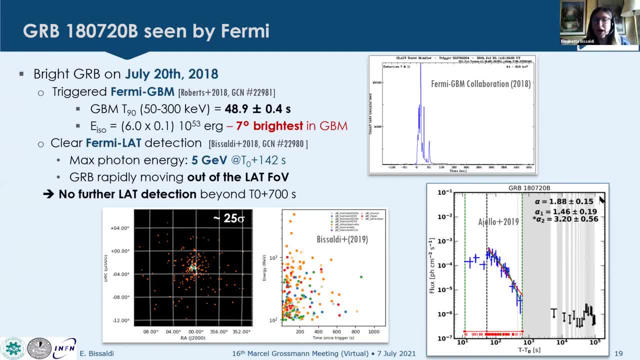 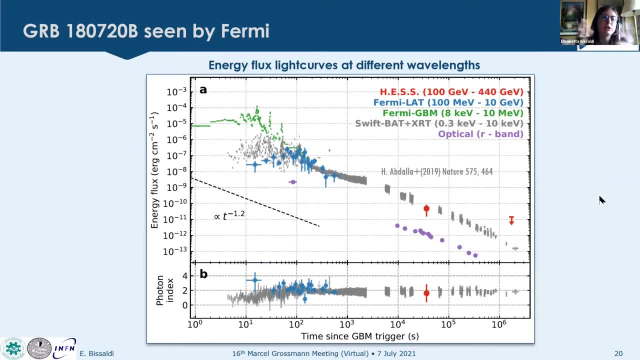 So after 700 seconds, there was no other detection of this event. And here you probably- I mean you already saw it on Monday- you have the LAT and the GBM data superposed on the, let's say, multi-wavelength light curve of this event, And here you see that the GBM 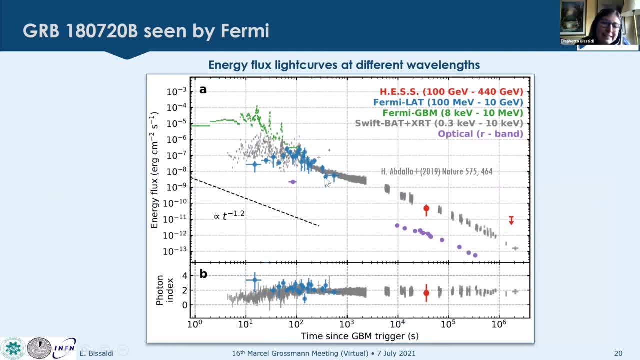 on top in green and the LAT in blue, And unfortunately the GBM data is not so spectacular. The LAT data only lasts until 700 seconds, because afterwards the GRB goes out of the field of view And it never- I mean it is never- seen in the subsequent time windows. 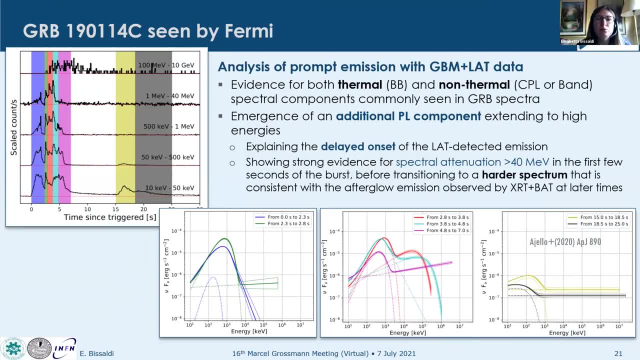 I am almost done, Franz, Just very few last slides. You already saw this in the talk by Alessandro 1901-14c, So I want to discuss it even more. the whole power law component that is popping out in the GBM plus LAT data. 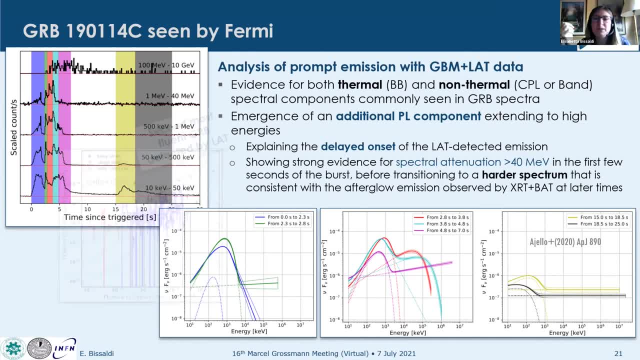 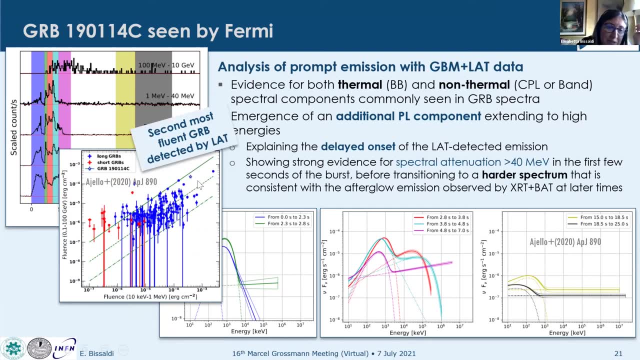 I mean it was the second most fluent GRB detected by LAT. I mean it's very small, but maybe here you can see there is a very small star just superimposed on what we published in the catalog, just to show you how bright this event was And again, I think you already largely 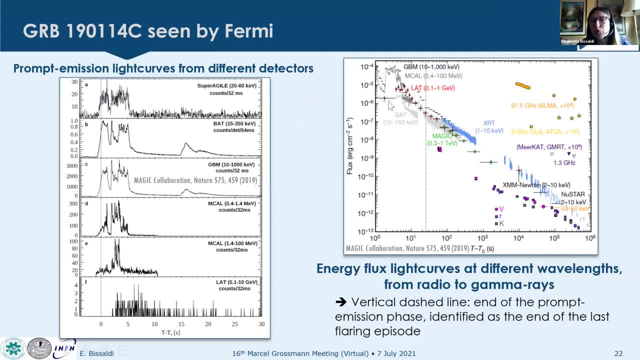 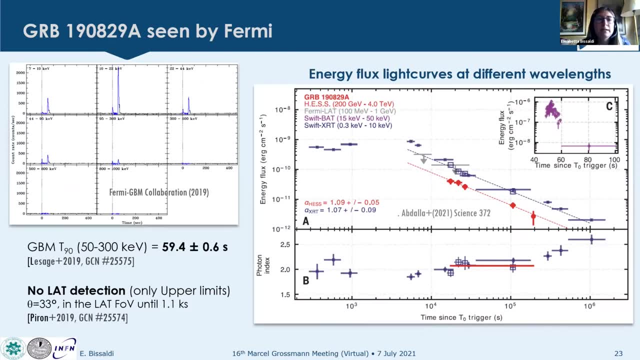 discussed it on Monday. You have the multi-wavelength light curve with also the LAT and GBM results here. A last word about the last published GRB 1908-29 by the Hess collaboration. So it was a long burst, You see in GBM. 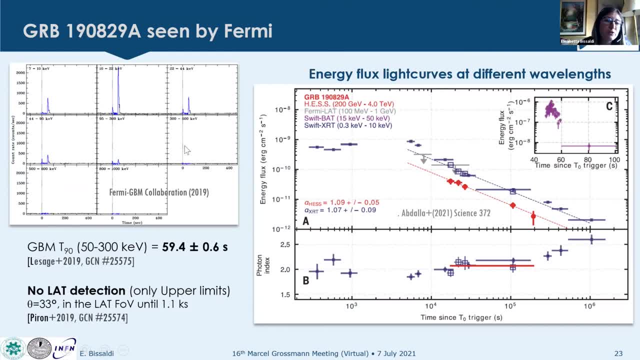 it was not particularly bright at high energies. I just put here an example of all of the energy ranges covered by the GBM And there was no LAT detection, only upper limits. that are also visible here in the multi-wavelength light curve published in the science paper. 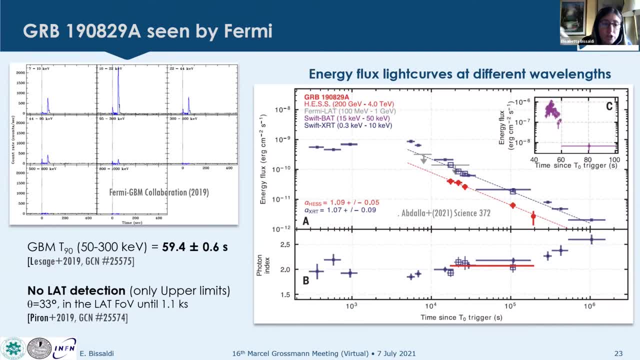 Unfortunately, I mean the LAT, sorry, the GRB was in the LAT field of view. I'm going to run until 1,000 seconds at the nice data angle, but it was not seen. And I want to stress that the last detection, the 20 by magic, again unfortunately, here the GRB was not in. 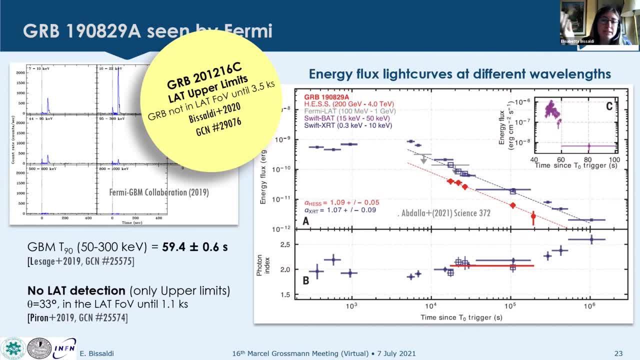 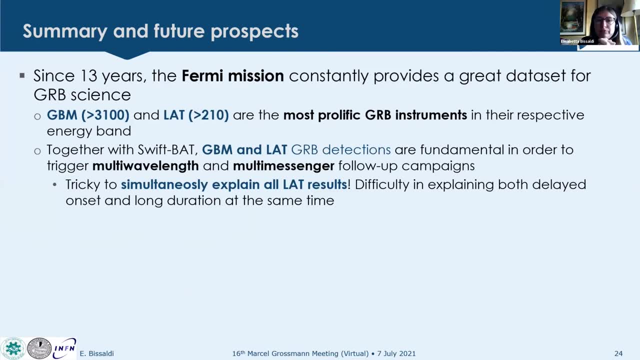 the LAT field of view until 3,000 seconds And there are just a few upper limits afterwards in the first time window to my conclusions. so since 13 years, the Fermi mission is constantly providing a great data set for GRB science. so we have I mean GBM and LAT with this number of of verse are the most prolific. 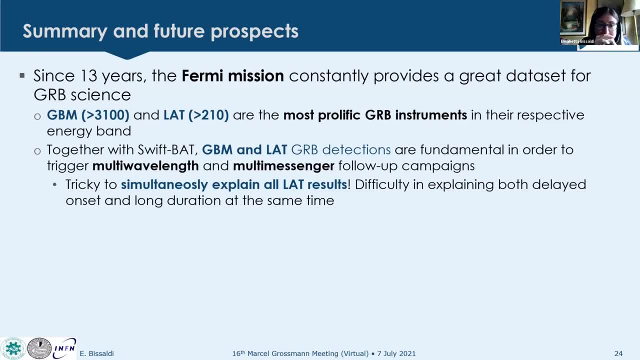 prolific GRB instrument in their respective, let's say, energy band and together with all of the other, I mean with swift back. they are really, I mean, and also agile that we heard before. they are really fundamental in order to trigger the multi-wavelength and the multi-messenger follow-up, so not only for 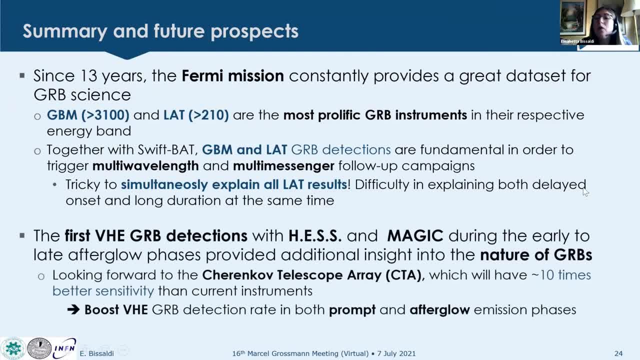 gamma-ray bursts, but also for for GV. obviously we are very keen on CTA coming up, so we are really now playing together with SMAGIC and we know that with CTA it will have 10 times better sensitivity than the current instruments. so we really hope that this will boost the very high GGRB detection. 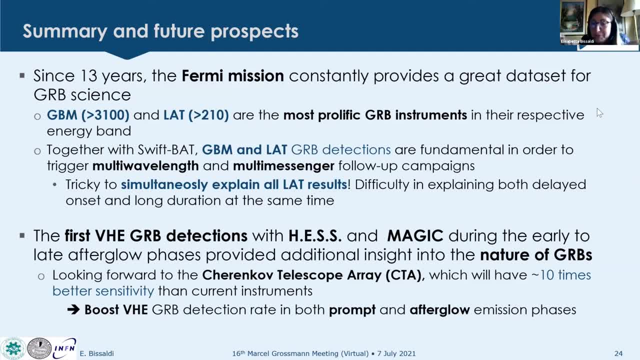 rate in the prompt and in the afterglow, and what we hope is that Fermi will still be there once CTA will be online. so this is the greatest hope that we have right now and I will go. I will finish with that, Thank you. 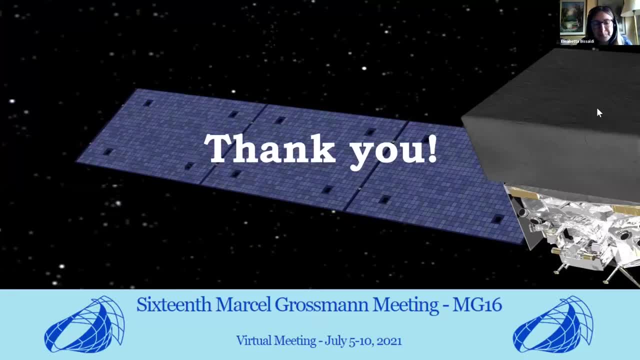 I will finish here and thank you for the attention. Thanks, Elisabetta, also for keeping in your time slot. so are there questions to better? otherwise, I have one. Okay, don't see any other questions. I will ask you one, one, one point, Elisabetta. you mentioned about 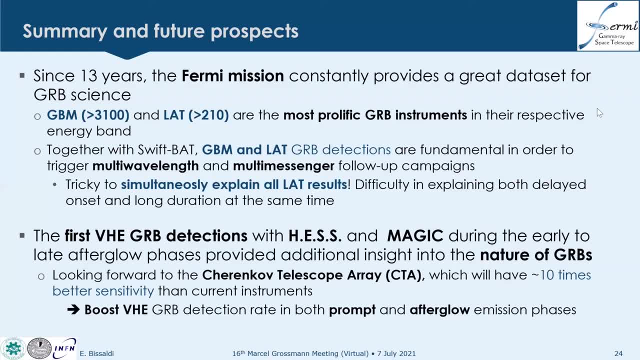 CTA. so the prospect of CTA, Yes, The prospect of joint detection. so let's say, do you have any? let's say, for forecast, for how much Fermi will be prolonged, so to keep active? while, how is the community we can support in case of this? 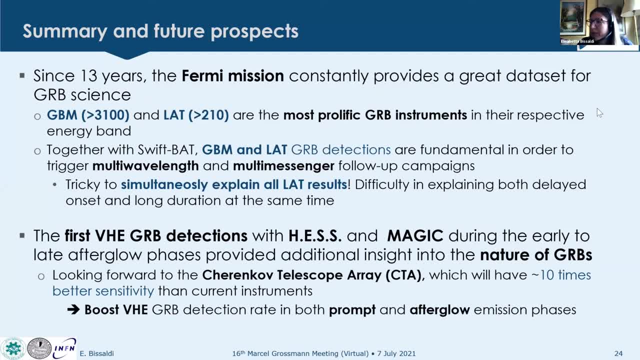 decision. Well, well, I mean Fermi, as we know, is undergoes a senior review every two or three years now, I don't remember the next one. Yes, one is coming up soon. so i mean, if fermi proves to be, uh, i mean uh- always so important for, as i said, 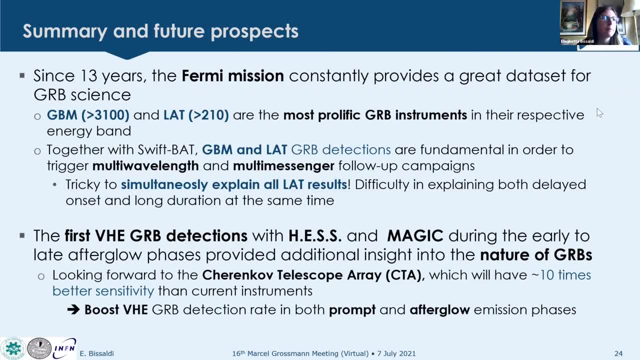 for uh as a multi-wavelength player, a trigger for gamma rebirths and for other interesting transients. now this year we had the famous magnetar giant flare from an extra galactic. uh, i mean from an extra galactic event, and i mean if the, the fermi mission proves to be uh, let's say, vital. 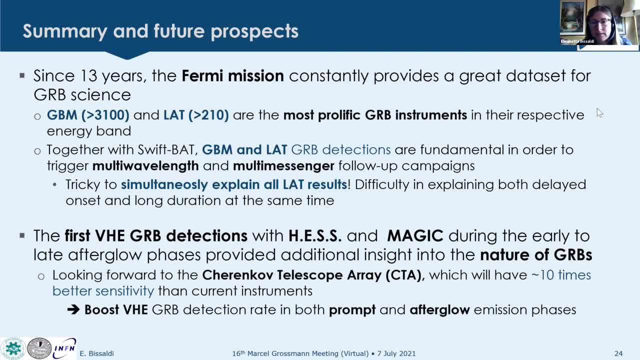 for uh in the multi-wavelength and multi-messenger context, then it's easy to write this kind of uh, let's say proposals during the years, and we- and i mean there are no consumables on board- fermi. so until the uh, all instruments perform nicely and they are. 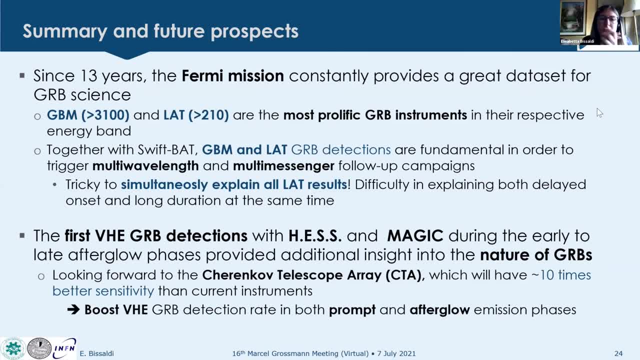 i mean, they are not, apart from the solar panel problem we had a few years ago, there were no mother. i mean, the instruments themselves are performing greatly, really. so uh, i, i, i assume that we will hopefully pass this review every uh thought years, and so we will be able. 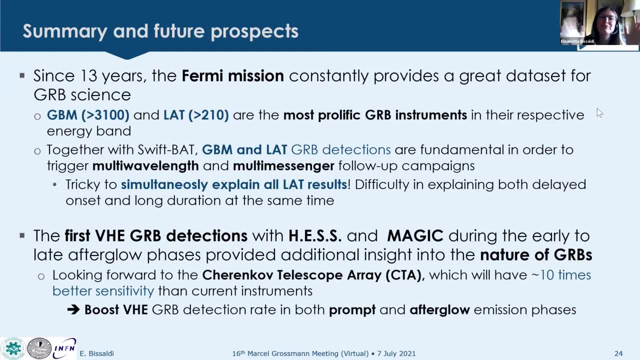 to be there at least for a few other years. i mean, we should have already been over somehow and we are still there. so i really, let's say i really cross fingers that this will continue for the next many years to come. okay, should i stop my screen share? 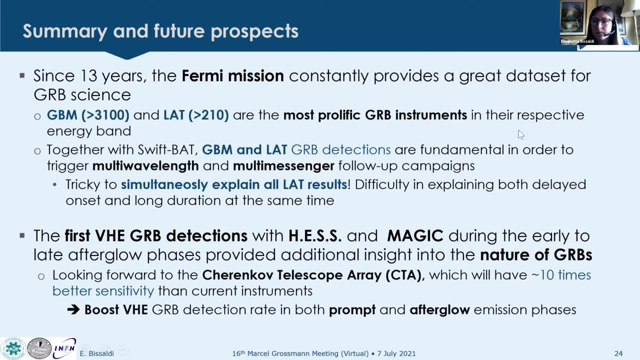 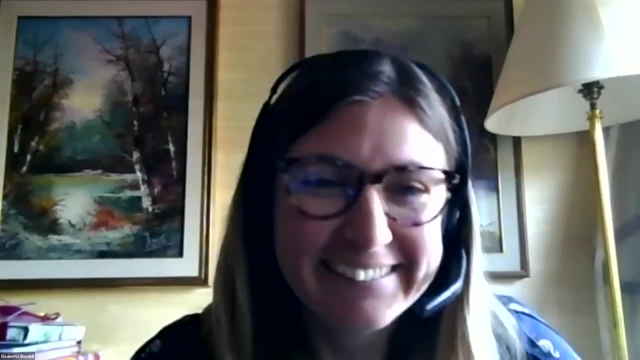 i can't hear france seems like. it seems like we lost france. yes, okay, so let's okay. okay, thanks a lot elizabetta. okay, thanks a lot elizabetta. okay, thanks a lot elizabetta. and uh, yeah, let's move on um, while waiting for france to to reconnect. 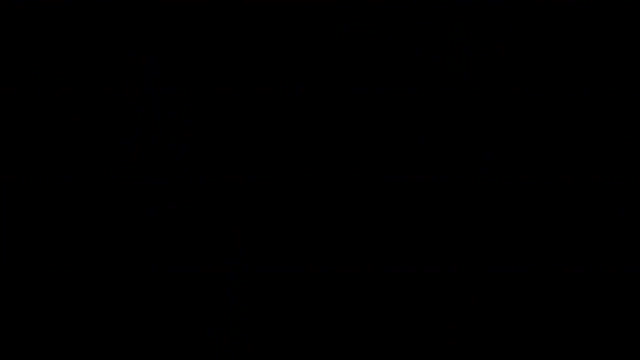 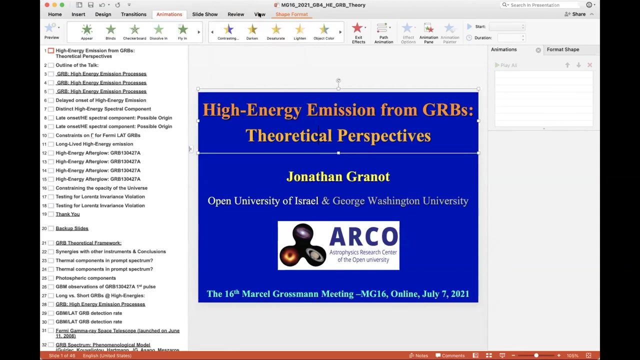 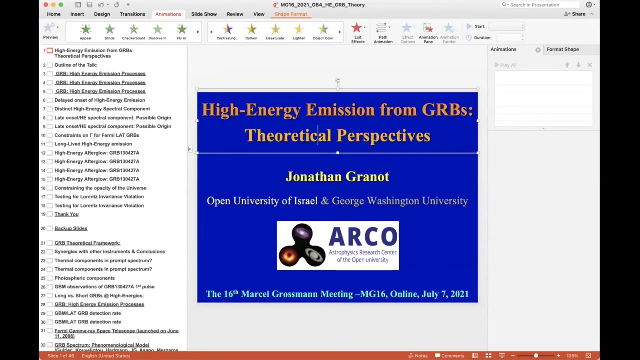 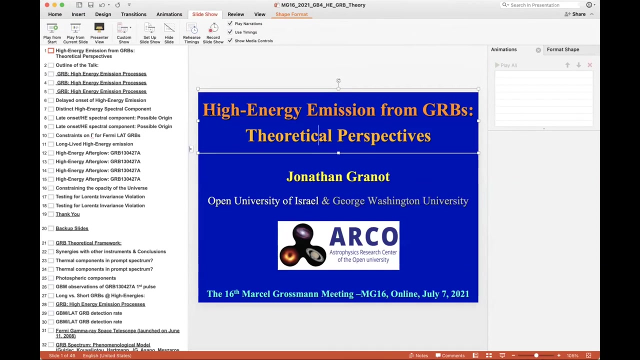 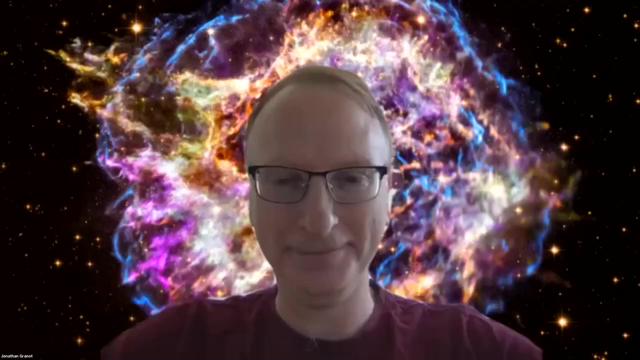 uh, we have a look at the, at the theory side now, and then this is your screen. yes, and go ahead. okay, okay, sorry, okay, it was looking fine just seconds ago, yes, but i was on mute and without the camera, so i will try to share again and then i couldn't do anything about it. okay, okay, okay, otherwise you. 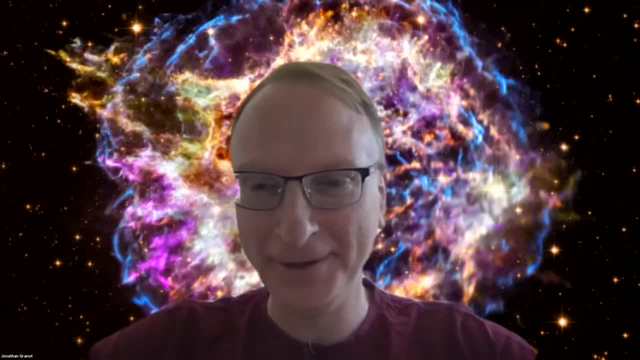 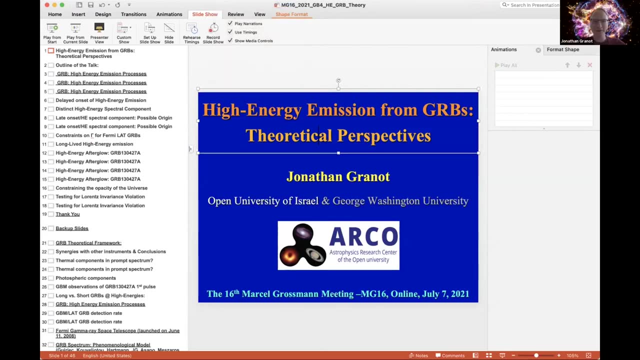 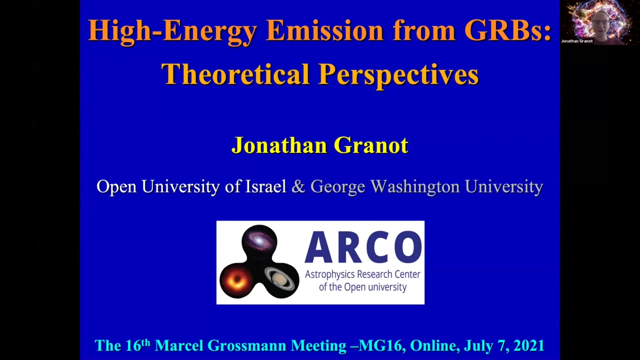 wouldn't hear me. so can you see that's yeah, i can't hear you, i can't hear you, i can't hear you. it's okay, yes, okay. so thank you very much for giving me the opportunity to talk here. i will give a theoretically oriented overview of the high energy emission. 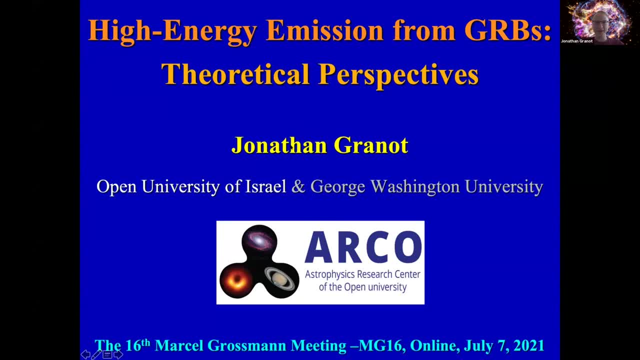 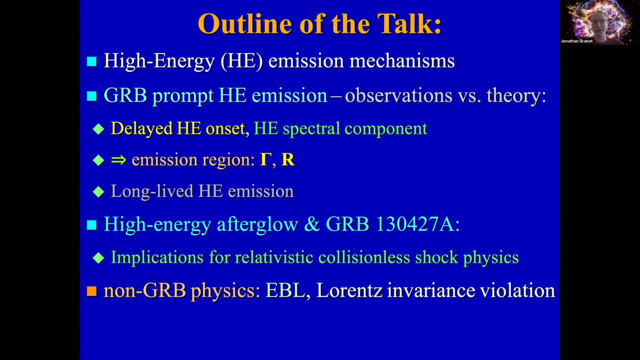 from gamma ray bursts, and the outline of my talk is as follows: i'll first discuss potentially relevant high energy emission mechanisms. Then I would discuss Trump-GRB high-energy emission observations versus theory. in particular, I would rely on previous talks in this session that gave a very nice overview on some of the most relevant observations. 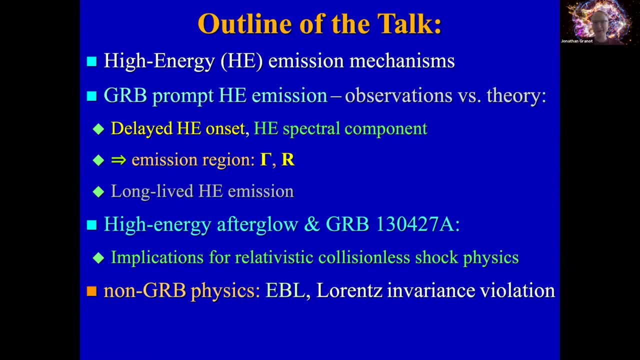 I would discuss the delayed high-energy emission onset, the high-energy spectral component that was shown already and what we can learn from high-energy emission about the Lorentz factor and radius of the emission region in the Trump-GRB. and what can we learn from the long-lived high-energy emission that can last for very long. 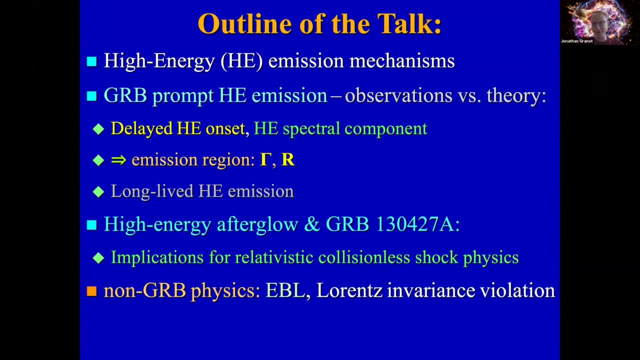 Then I would give a case study of high-energy afterglow: the case of the very bright GRB 1304-27A. that was already discussed partly. So what can we learn from it and, in particular, implications on relativistic conditions as shock-fitting? 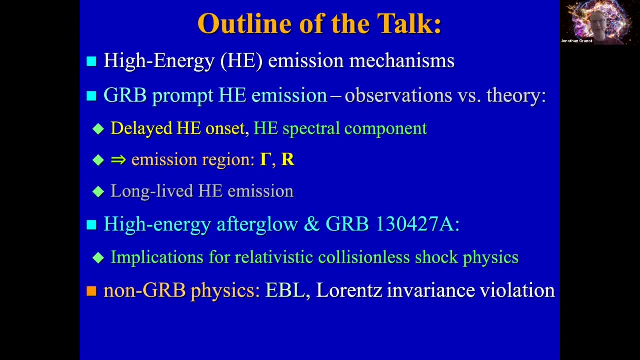 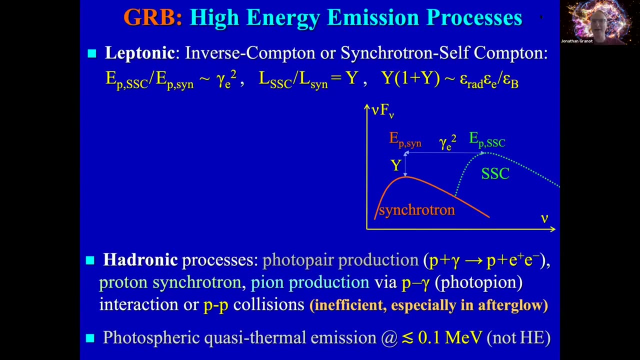 and at the very end, I would discuss two things that you can learn about from this high-energy GRB emission that are non-GRB physics, essentially about the exogalactic background light and Lorentz invariance violation. Okay, so high-energy emission processes. 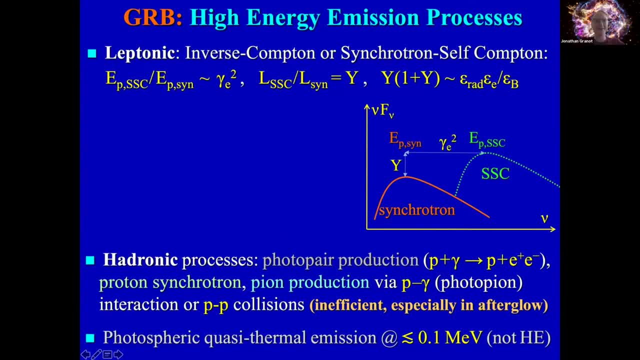 So the two most relevant types of emission processes are leptonic and hadronic. In the leptonic processes you typically can see here that you have that you expect a synchrotron component by relativistic electrons gyrating in magnetic fields within the emitting region. 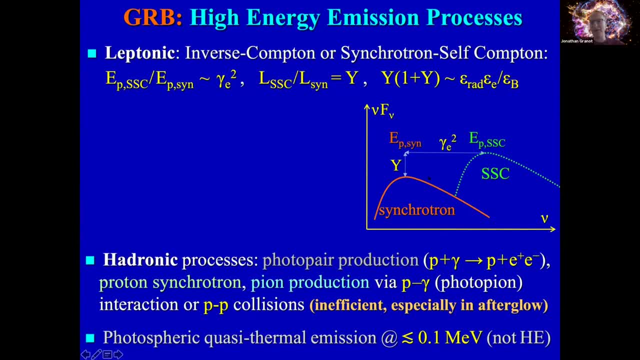 And those same synchrotron photons can be Compton upscattered by the same population of relativistic electrons into higher energies, and then you get the so-called synchrotron self-Compton component that peaks at higher photon energies. Now this SSE, or synchrotron self-Compton versus synchrotron component have some interesting relations directly related to the underlying physics. 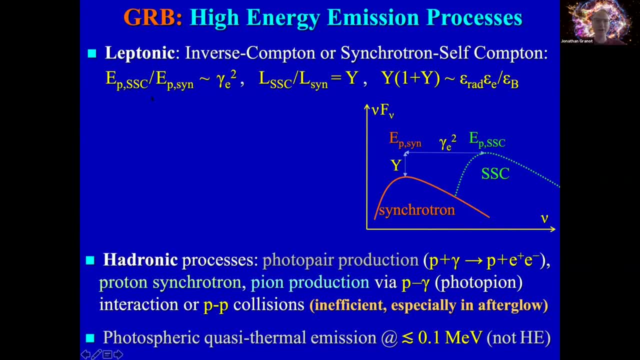 Essentially, the ratio of their peak nu of nu photon energies is the square of the typical Lorentz factor of the emitting electrons, gamma e squared, And the ratio of their luminosities is the famous Compton y parameter. here that you can see is related in a fairly simple manner. 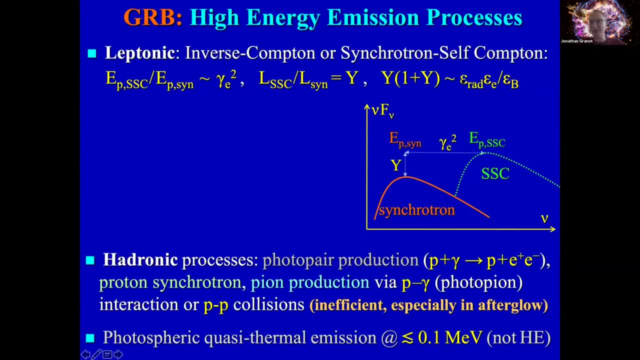 to both the radiative efficiency, epsilon rad and the well-known epsilon e and epsilon b, the micro-physical parameters, the fractions of the internal energy in the emitting region that go into these accelerated electrons, and the magnetic field, respectively. Okay, now, on the other hand, we have hadronic processes. Sorry. 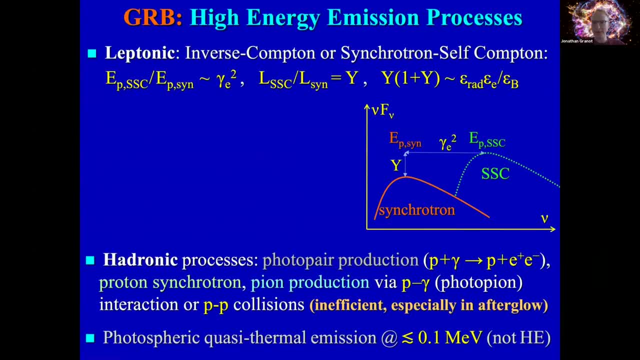 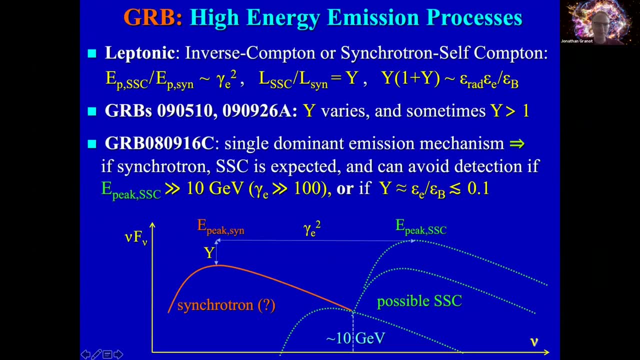 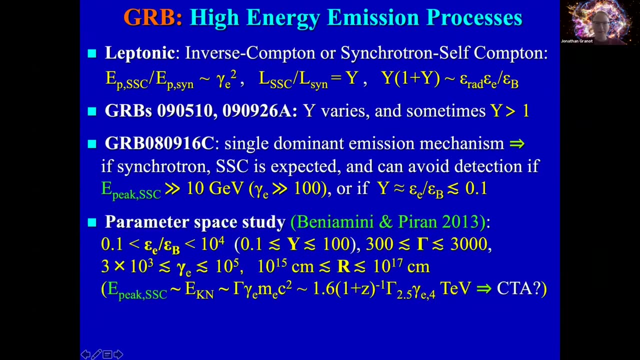 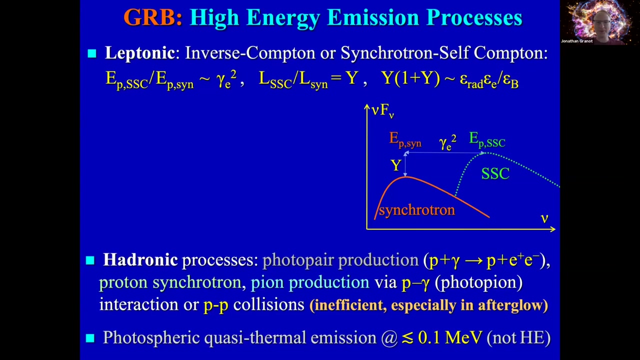 Okay, Oops. In adronic processes we can have: Oops, What's happening here? Okay, Transitioning along, We can have photoperiproduction, proton-synchrotron production via P-gamma or P-P interactions, et cetera, et cetera. 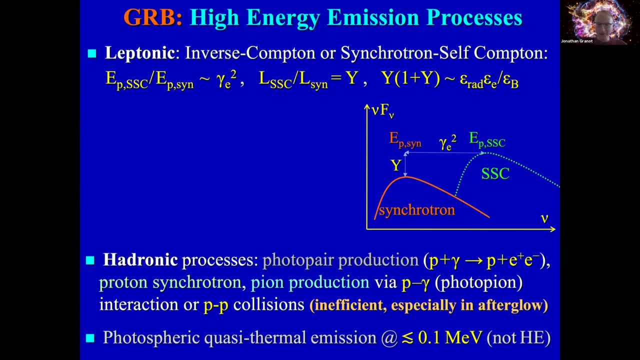 Hadronic processes are generally inefficient. In particular for the afterglow they're even much less efficient. This is because they require high densities. so a small emission radius You can have that under certain circumstances. for the prompt emission In the afterglow it's very hard. 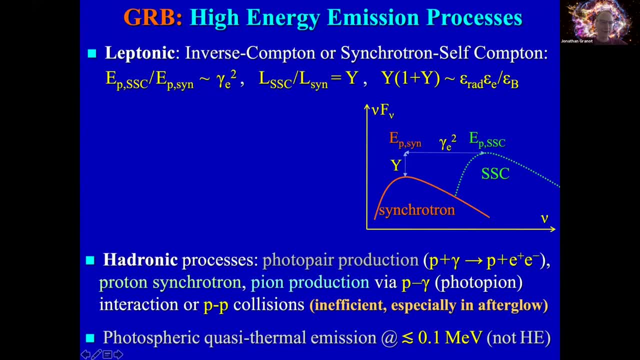 And finally, we can have photospheric quasi-thermal- Okay, Photospheric quasi-thermal emission, but that is relevant for low energies under MeV, so not high energies. So I would not discuss this much further in this talk Now. 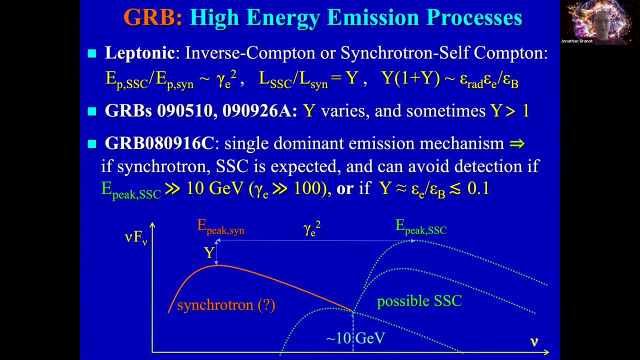 Why is it not switching? Okay, So from observations of high-energy emission from actual GRBs it appears that this Compton-Y parameter varies And sometimes even exceeds unity. So sometimes you can have more energy in the energy component. Usually you have somewhat less during the prompt emission. 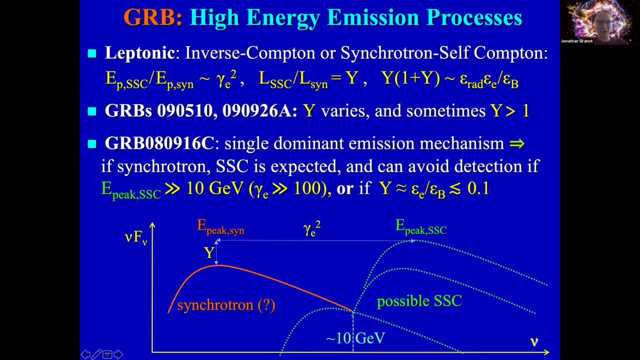 And in particular in the famous GRB 080916C, we have a single dominant emission component up to the highest observed energy, which means you should hide the SSE component. So either the Compton-Y parameter is below or above 0.1,. 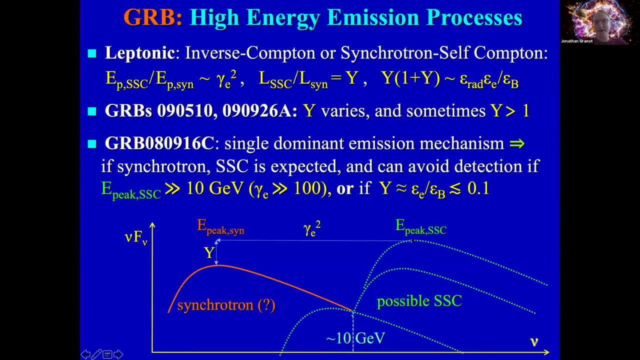 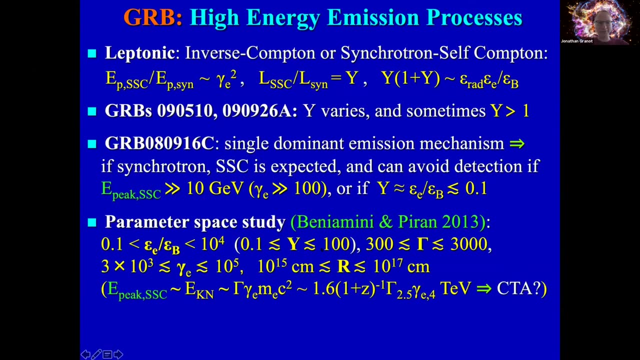 or it peaks at very high energy, Okay, Very high energies, TV energies, So above what Latt could see, but still very interesting for TV instruments. And finally, if you take the observational constraints and these two components, you can really constrain the relevant physical parameters. 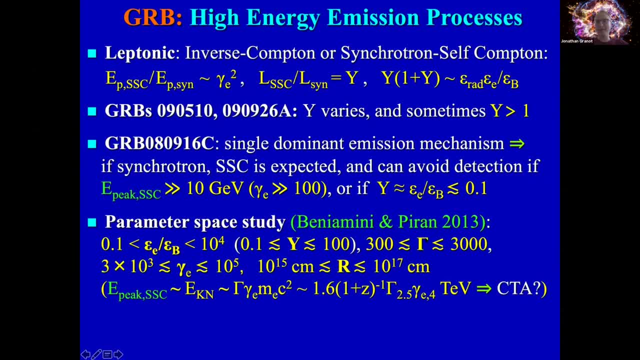 in particular the ratio of epsilon E and epsilon B, the bulk Lorentz factor, the typical Lorentz factor of the emitting electrons and emitting radius, And you can have emission that's limited in the highest energy by Klein-Ishina effects. 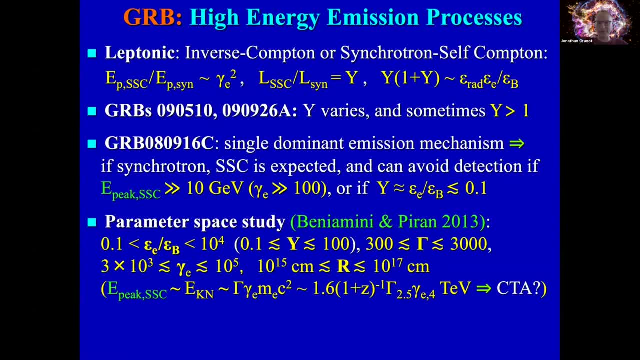 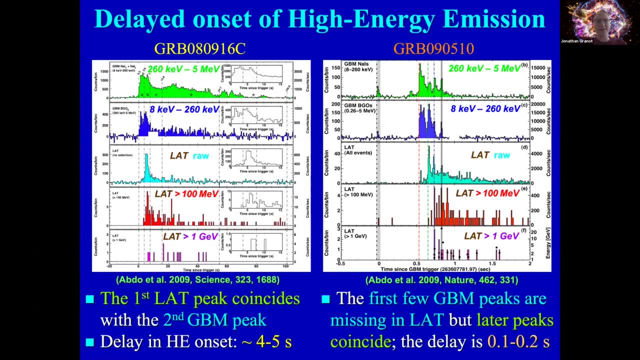 but it can reach TV energies potentially, which is very interesting for CTA and other instruments. So here you see two well-known bright Fermilab emission GRBs, the long GRB 080916C and GRB 090510 that I showed before. 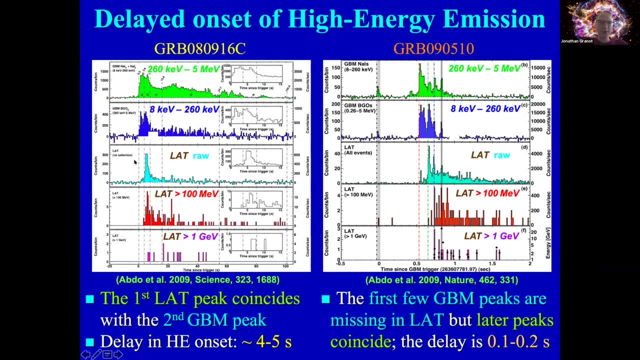 They both show delayed emission, And what I want to show you here is that essentially what this delayed emission means is that you miss the first spike, as you can see here in this long GRB, causing a delay of four or five seconds, And in this short GRB, you miss the first few spikes. 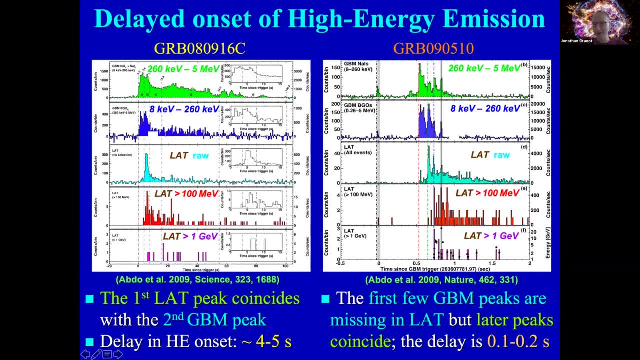 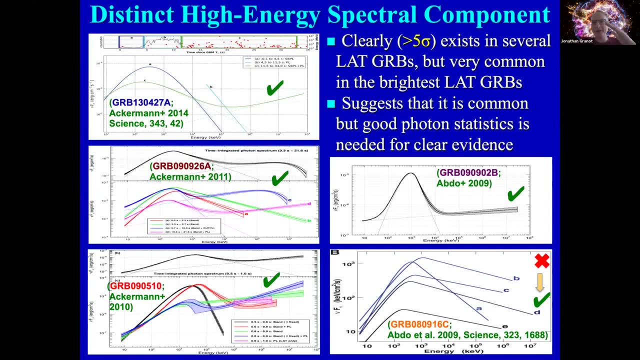 but then later spikes really coincide in all energies. So this so-called delayed emission is truly missing the first spike or a few spikes at high energies. So we can see here that also in most of the brightest GRBs at high energies you see this distinct high-energy spectral component showing as a power law. 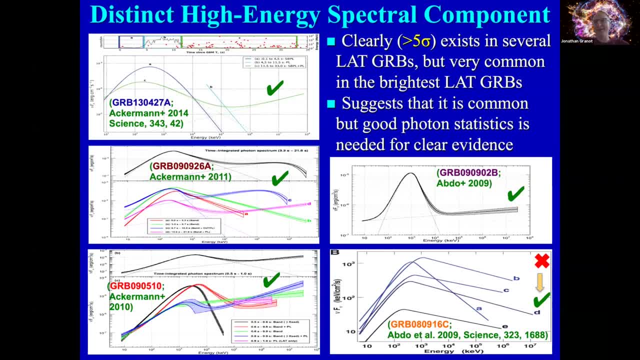 which is usually fairly hard, And the fact that it's very common in the brightest bursts suggests that it's intrinsically very common and you just need the good photon statistics to detect it with high significance. And in addition to that we see some time-resolved. 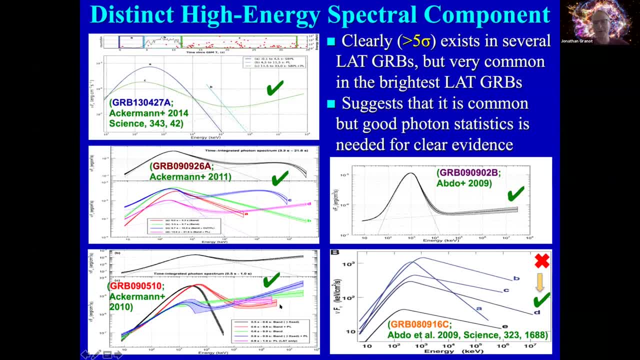 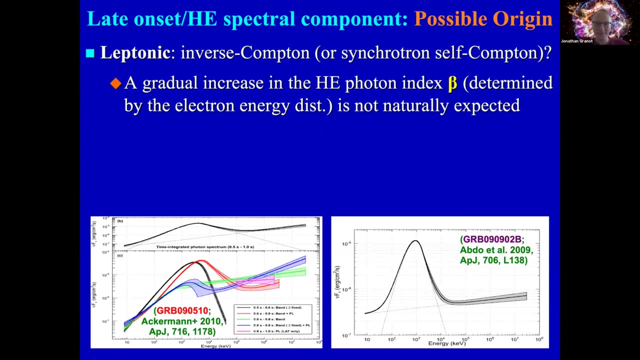 the spectra here. it tends to become harder throughout the duration of the GRB, which might partly explain why at early times, when it's less hard, you miss the first spikes at the high energies. So can you still hear me? Yes, yes. 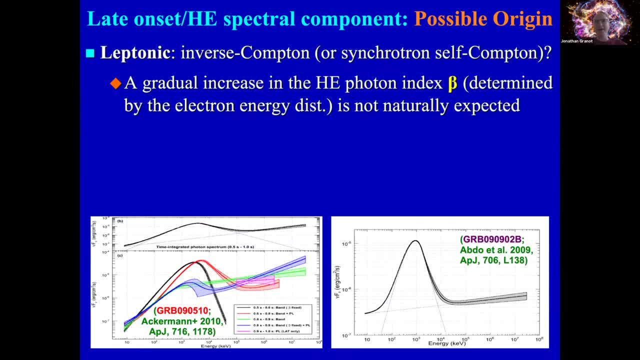 Okay, it was too quiet, Thanks, Okay. so what can we learn from the theoretical perspective? So, first of all, if we consider the tonic process, inverse Compton or SSE for the high-energy component, then the gradual increase in the high-energy photon index beta. 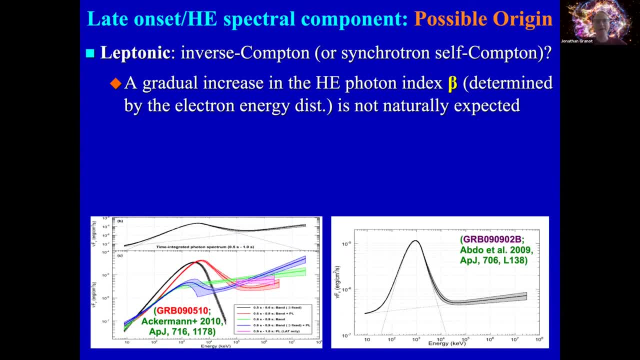 which, in this case, would be determined by the electron energy distribution power law index. it's not naturally expected to become harder throughout the duration of the burst. It's possible, but it's not very natural. It's hard to account for the different photon indexes. 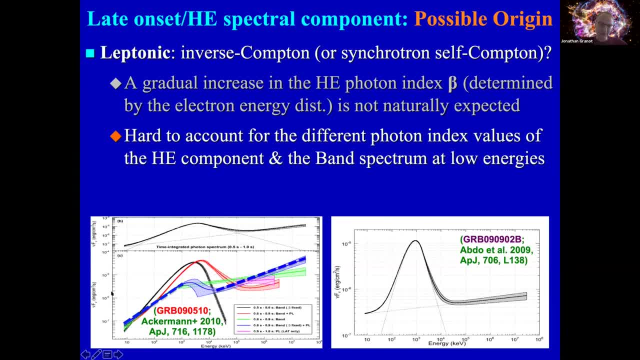 on the one hand here in the high-energy component, on the other hand the low-energy component of the band, because they're expected to be the same in this synchrotron SSE combined model. And finally, it's hard to produce the extension of this power law component. 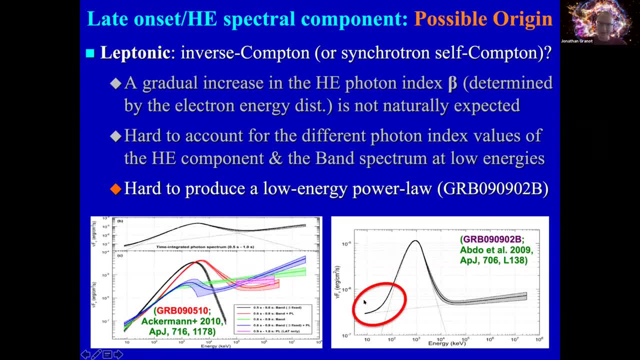 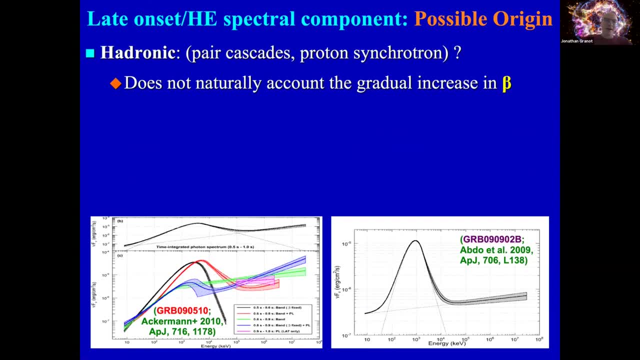 to lower energies below the band component, which is seen in many cases. So that's kind of a drawback of that. And for hydronic models you could have a Pertus case, proton synchrotron, and again you don't naturally expect a gradual increase in beta. 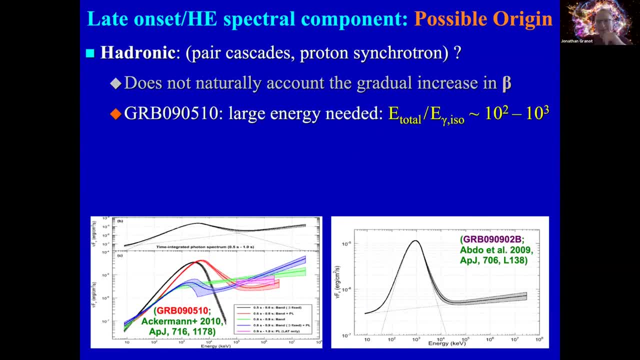 though it's possible. One drawback is that in many cases, energy requirements are fairly extreme. It could be two to three orders of magnitude above what you see in gamma rays, And what you see in gamma rays is already pretty demanding energetically. 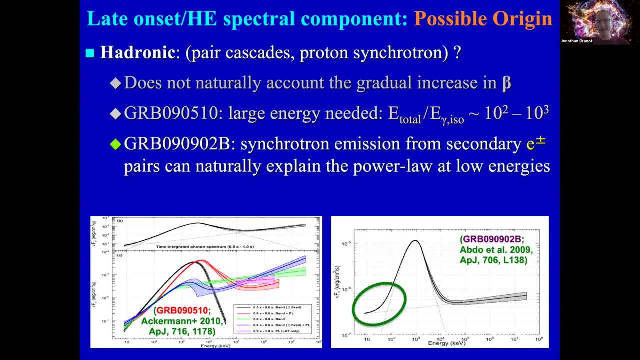 So you need huge amounts of energy. On the other hand, you do naturally produce an extension of the power law component at the lower energies from synchrotron emission, from secondary pairs, that are produced in such scenarios. So each of these interpretations has some pros and cons. 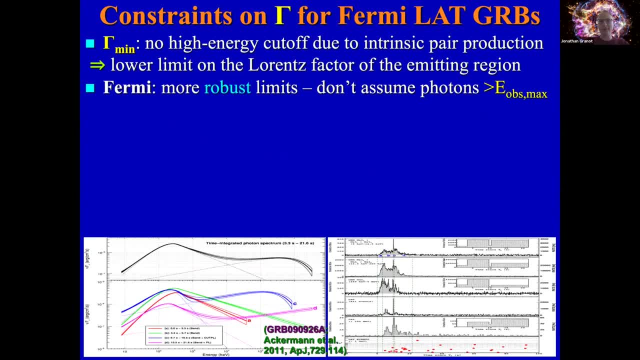 Now we can learn about the bulk variance factor of the emitting region from seeing such a high energy spectral component. In particular, if there is no cutoff in this power law, one can put a lower limit on the bulk variance factor: gamma min. 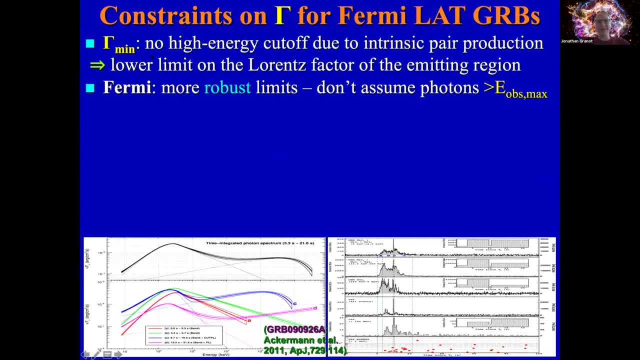 And this is from compactness arguments, opacity to gamma, gamma- gamma pair production within the source. The limits put by Fermilat are more robust than previous ones because they do not assume the existence of photons above the highest energy photon that is actually observed. 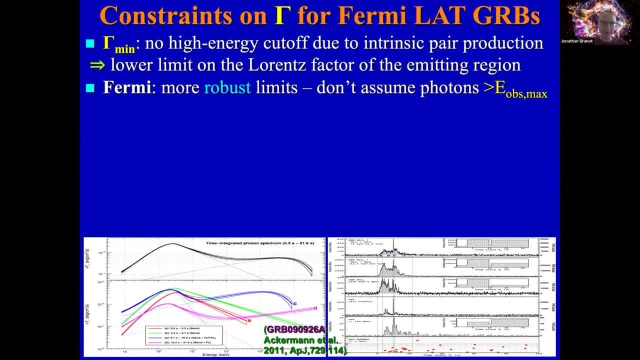 compared to previous limits of that kind. One caveat is that tau-gamma-gamma within the source depends both on the bulk variance factor gamma and emission radius R, And in order to get to that gamma min, you need to assume some relation between r and gamma, the usual assumed relation that you 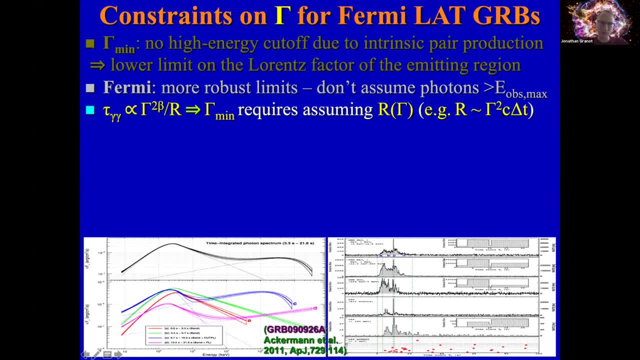 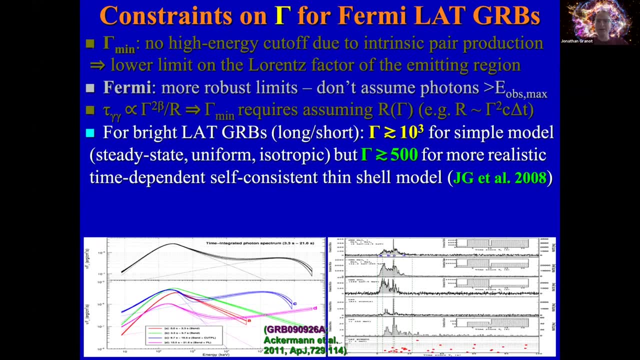 see here holds in many models but not all of them. so that's one slight caveat. now for the brightest lat grb is both long and short. you get the gamma min order of 1000 for a simple model, assuming steady state uniform isotropic photon field within the source. however, if you do a more careful, 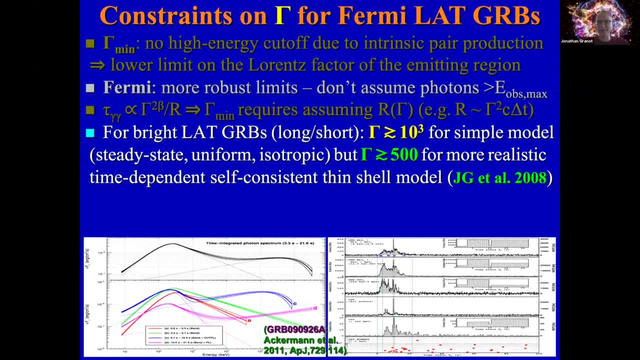 analysis you get about the factor of two lower gamma min order 500. that's our more realistic time dependent, self consistent thin shell model. now, in cases where you actually see a cutoff, you can estimate the rents factor itself. and for these two types of models, in this case grbo9926a. 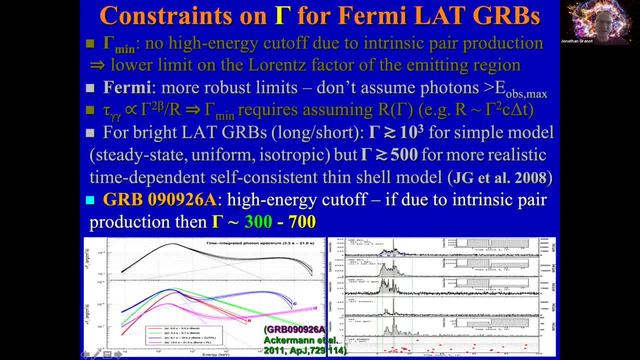 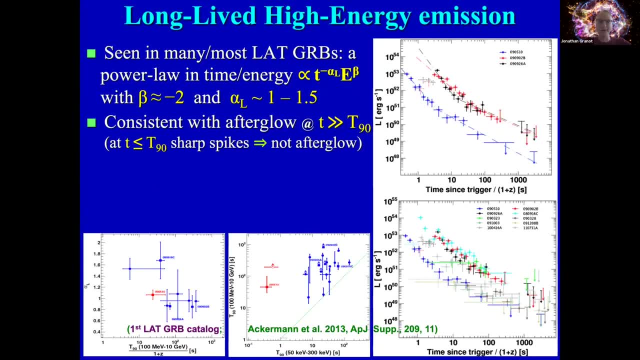 you get an estimate of 700 or 300 respectively. the 300 is probably the more realistic number. okay, now for the long-lived component. as was shown very nicely by beta, you see in many grbs that the gb emission lasts well. after the nev emission it typically decays as a powerline time. 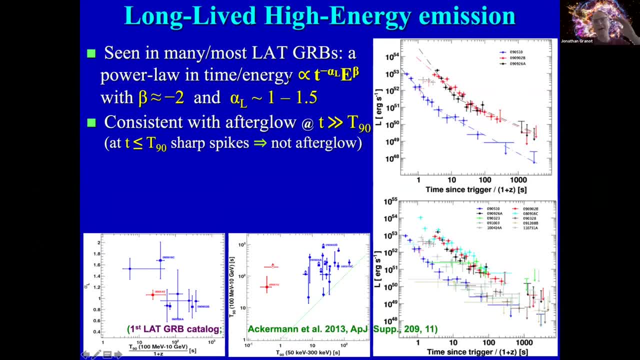 t to the minus one to one point five roughly, whereas the spectrum is a parallel, flatish new beta close to minus two and well above the t90 of the nev emission. it's almost certainly the same as the afterglow emission, but when you see sharp spikes initially it's part of the 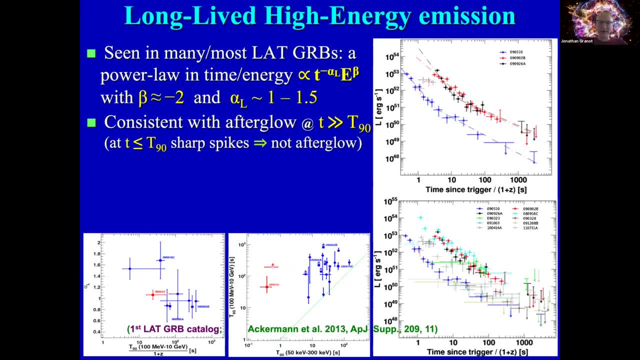 prompt emission. you can't get such high temporal variability from the afterglow emission. there are other possible explanations etc. and sometimes you might even see the transition. probably it was seen. one of the best cases is grb190114c. it was discussed extensively. there are other possible explanations. maybe it's associated with extinct layers. maybe 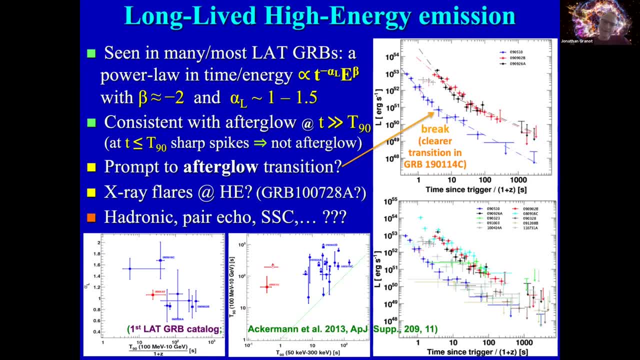 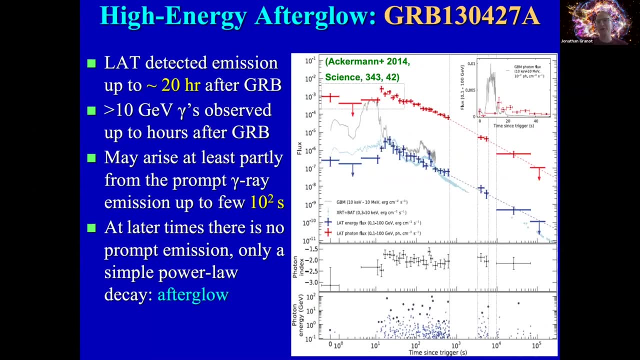 it's associated with very high energies like lystor and pyracos, etc. etc. in most cases, this does not seem to be the case. in some cases, especially very high energies, it could be ssc, but that was already discussed quite extensively. okay, now i'll switch to high energy afterglow from grb130427a. 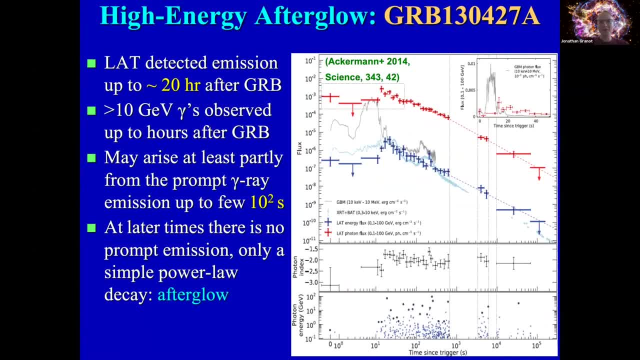 monster burst. it was discussed extensively, so i'll just briefly remind you that it was detected up to about 20 hours after the grb and gb energies afterglow was detected, and then, in this case, it's with many high energy photons above 10 GeV up to hours. 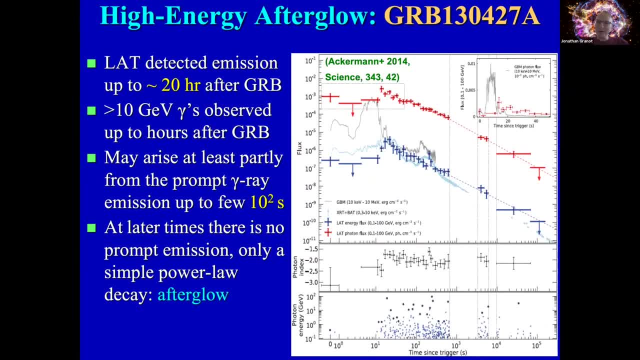 after the GRB. It may partly arise due to prompt emission in the first 200 seconds, but it's much longer at times. You see just a very smooth parallel decay, parallel spectrum. Everything tells us it has to be afterglow at late times. 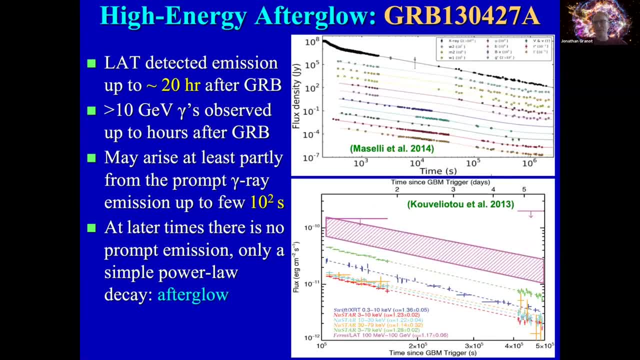 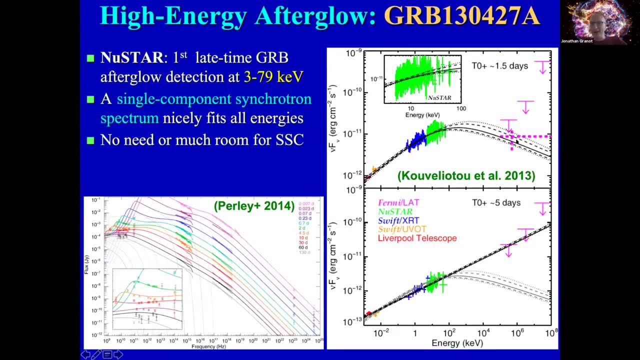 And here you see again from optical through X-rays to gamma rays. you can see the nice parallel behavior. So at late times it's clearly afterglow, And if you look here at the spectrum in particular lasting from optical through X-rays, 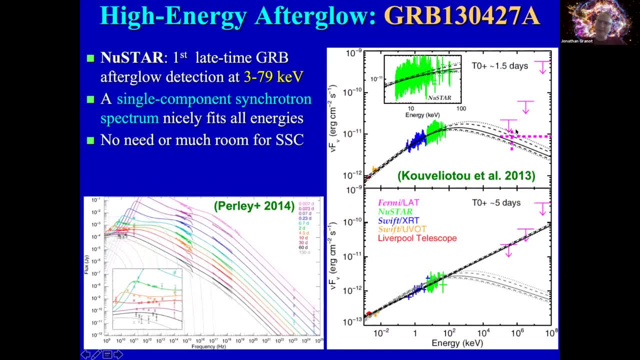 all the way to GeV. it's consistent with a single synchrotron spectral component And in particular, the upper limit by Veritas leaves very little room for any SSE component appearing at the highest energies, So it appears to be dominated by a single synchrotron component. 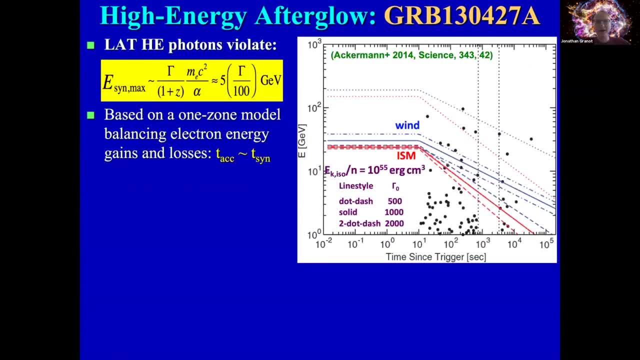 in this case. And why is this so interesting? Because it clearly violates the famous maximum synchrotron photon energy limit. Now, this limit, so-called burn-off limit, is based on a one-zone model balancing electron energy gains and losses, equating acceleration time to a synchrotron energy. 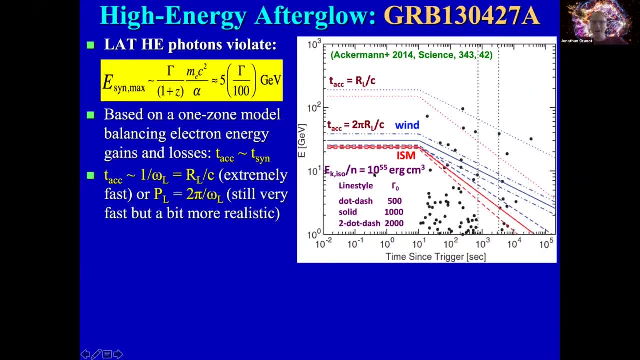 loss time And you can see the two lines here where even the lower lines are very conservative. They assume the electron essentially doubles its energy in a single Larmor gyration time, which is extremely optimistic. It's probably accelerating slower than that. The upper lines are crazily optimistic. 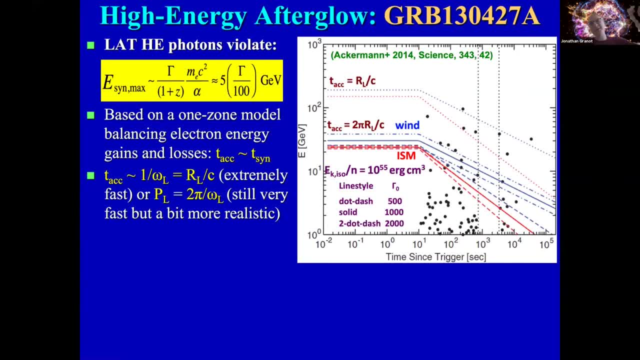 assuming it doubles its energy, doing only one radian out of this Larmor gyration, which is unphysical in my view, But still, You know, it clearly violates this limit by about an order of magnitude. Now, what does it mean? 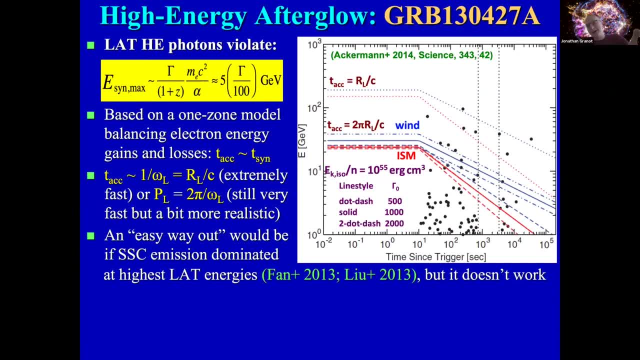 An easy way out would have been if it was dominated by SSE, but it doesn't seem to work in this particular case. It might work in other cases, So there really appears to be a true violation of this limit here, which means at least one of our assumptions must break. 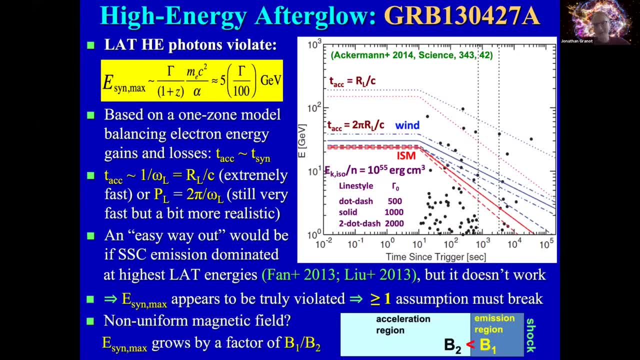 Now what might break? The best candidate is the assumption of a uniform magnetic field in the acceleration, in the emission region. So you could in principle have just behind the shock that accelerates the particle a high magnetic field region And well downstream of the shock. 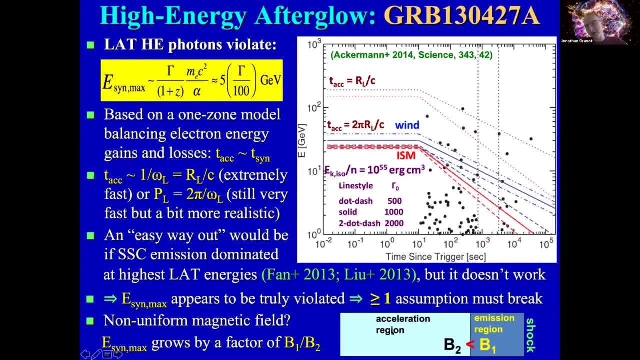 the magnetic field could decay and become lower, in which case the bulk of the acceleration would be in a lower magnetic field B2.. And the highest energy photons may be emitted when these high energy electrons reach the higher magnetic field region B1,. 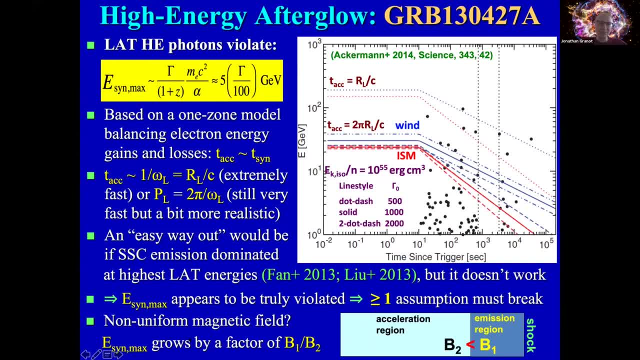 and emit these photons, in which case you can exceed this limit by the ratio of these two magnetic fields. In this case, it has to be about an order of magnitude. Seems to be potentially plausible. Now we can use high energy emission from GRBs. 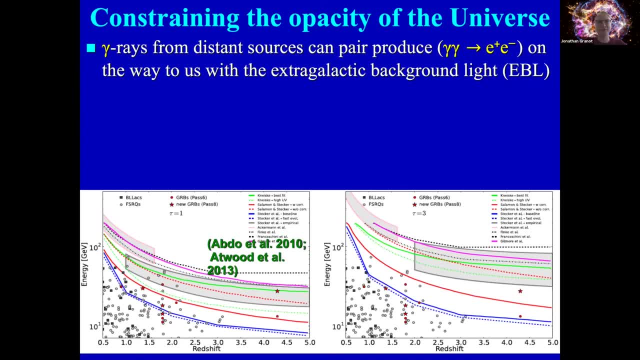 to also constrain other physics, not only intrinsic physics of GRBs. One example is constraining the extragalactic background light, because the gamma rays from the source and the GRB on the way to us can interact with this EBL radiation field. 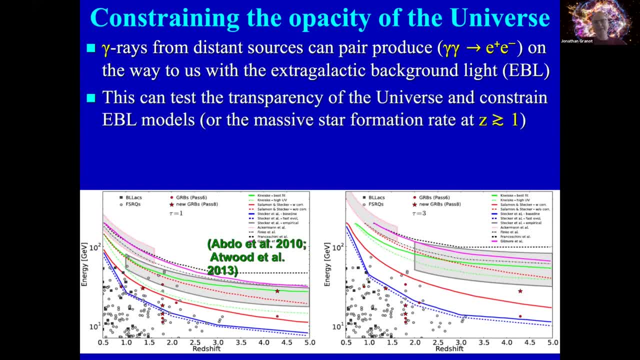 And produce electron positron pairs. Now this can test the transparency of the universe. An EBL model is essentially a massive star formation of cosmological redshifts. GRBs are competitive with AGN and probe higher redshifts And in particular using lasers. it 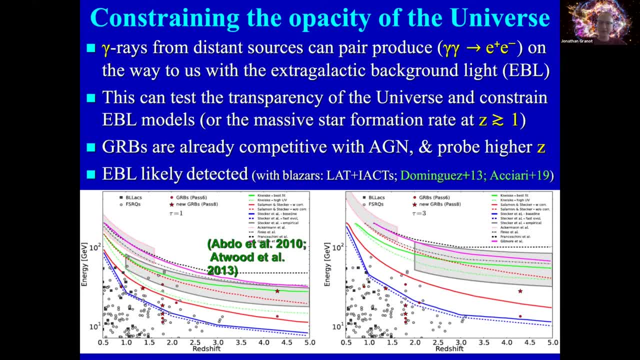 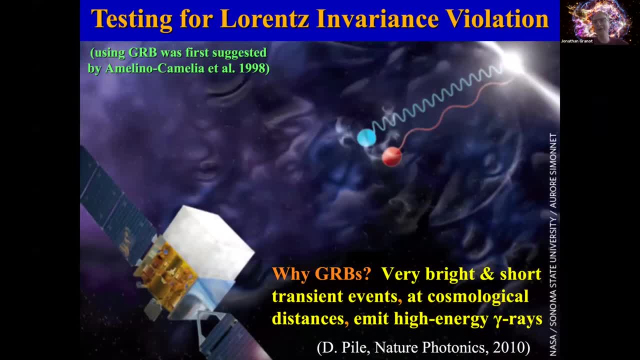 was probably already detected. So GRBs are interesting in that respect. And finally, they can test Lorentz invariance violation, where the idea here is that GRBs are thought of as a short pulse of radiation at cosmological distance, So they emit high energy photons of various energies. 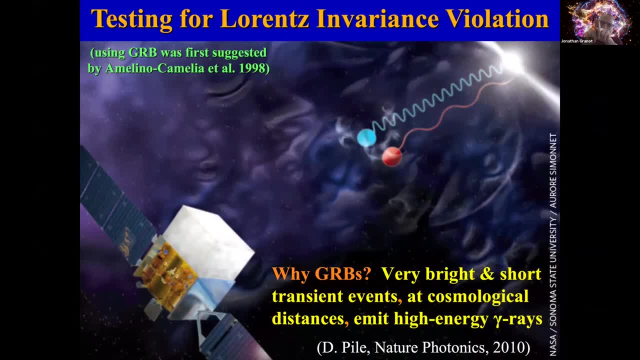 And if you had an even very slight difference in the propagation speed of photons as a function of their energy- some vacuum dispersion so-called- then they would reach us at different times, even if they were emitted at exactly the same time and place in the source. 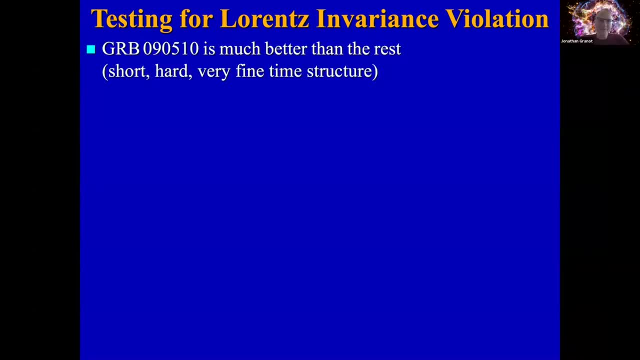 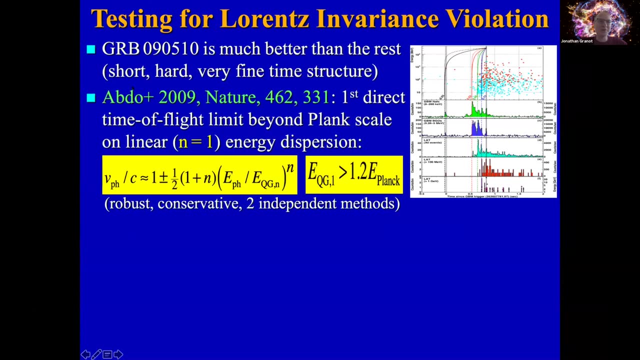 Now the best way to test this, the best source so far, was a short test, GRB 090510.. It is much better than all the rest, simply because it was short. So it was a very short pulse, It was very hard spectrum and had very fine time structure. 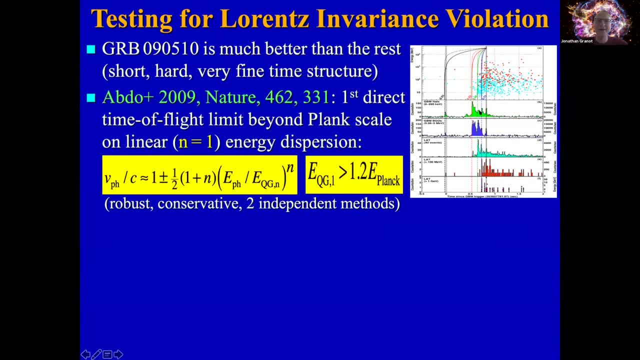 with the spikes lasting 5 or 10 milliseconds. So it was extremely useful And we used it in 2009 in a Nature paper to set the first direct time of light limit on linear Lorentz invariance violation or vacuum energy. 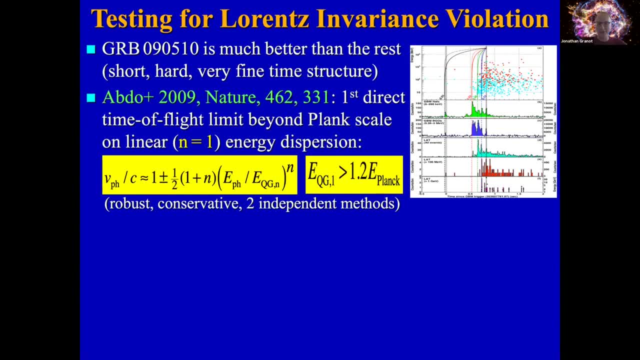 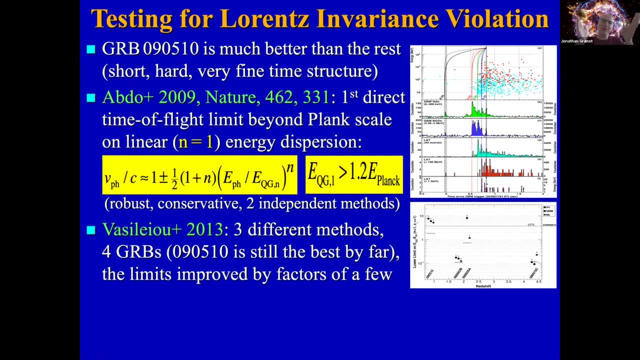 dispersion. It is above the Planck scale or Planck energy. It is robust, conservative, using two independent methods. So that really made a lot of noise. This was improved four years later using three different methods. Well, we used four GRBs, but still by far. 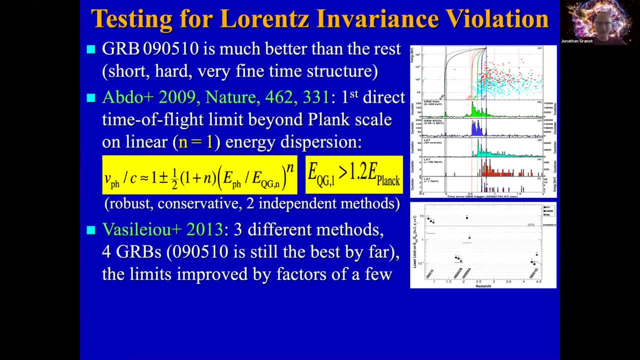 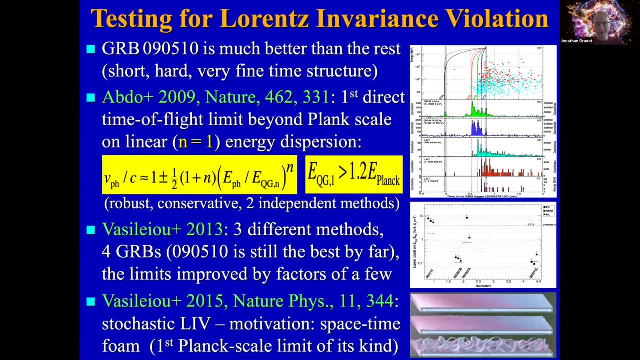 this one short GRB gave the most strict limits, So we were able to improve the limits by a factor of a few. And finally, in 2015,, we put the first Planck scale limit on stochastic, Stochastic LIV, motivated by spacetime foam models. 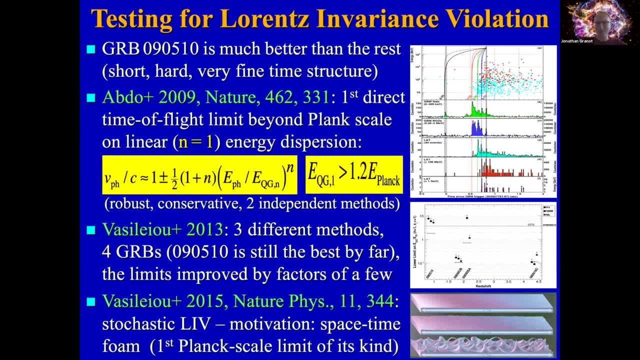 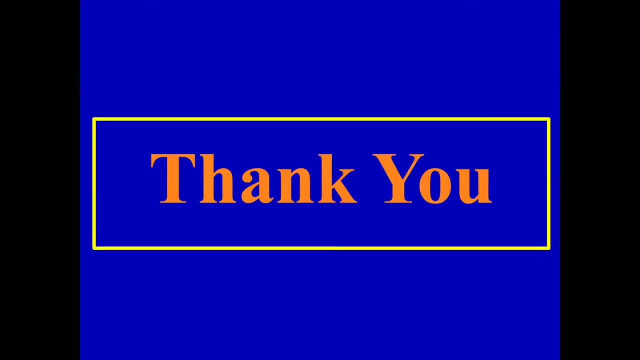 Again, this is the first limit of its type above the Planck scale, which is the only natural scale in this problem. So two minutes, Yoni. OK, perfect in time. I was just giving you two minutes, Perfect, Yoni. 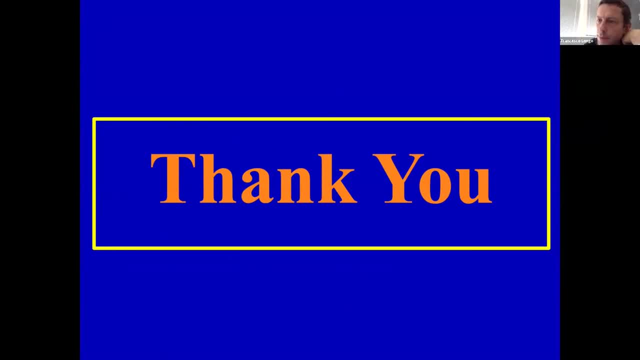 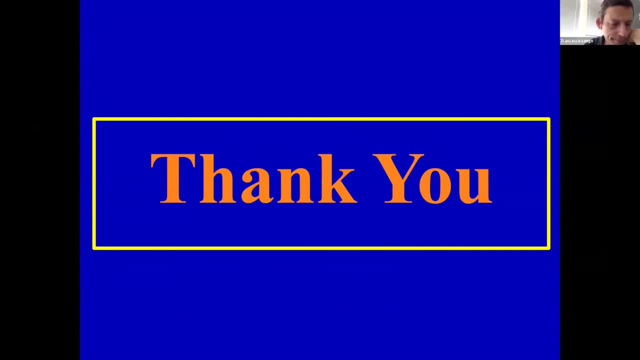 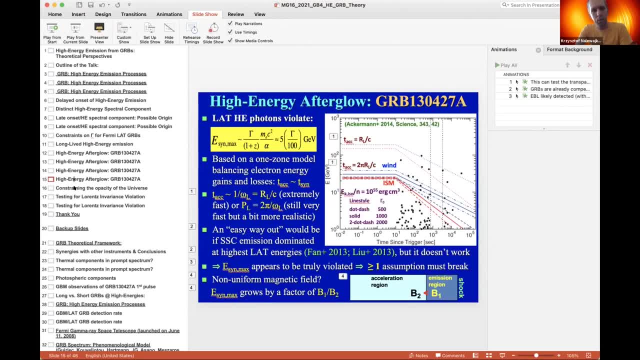 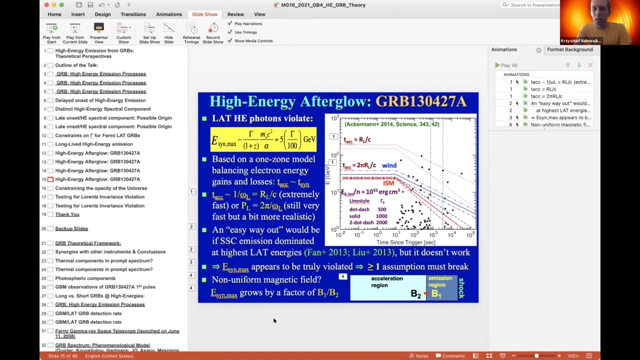 mentioned magnetic field compression by shock as a possibility, But other possibility that has been discussed in other contexts was magnetic reconnection, which allows to have E greater than B and accelerates particles beyond the limits. Is that possible in this context or not? Well, in principle, you know, it's a nice idea. 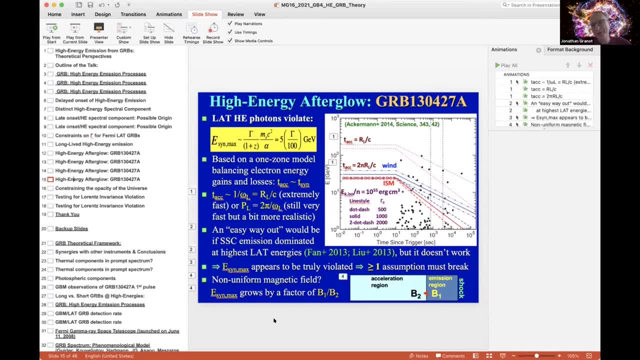 but the question is: how well can this work in practice? So when- I guess the question is the sigma. if it can be high, Well, let's put it this way, It could work in, potentially in the prompt emission, since we're talking in this particular case about 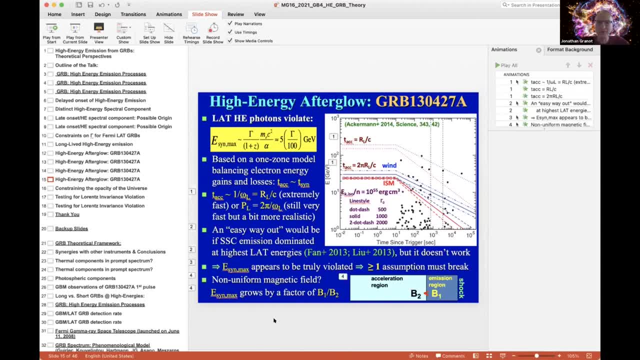 you know hours after the GRB and it's clearly afterglow. the answer is no. it can't work in the afterglow, Because in the afterglow you're talking about, the collision is shot, going into the external medium. 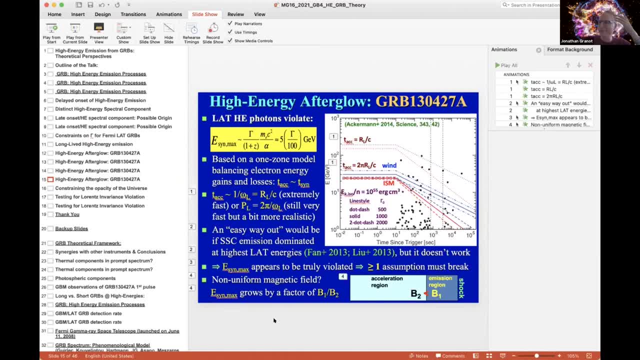 You expect there, you know, to have the upstream sigma negligibly small. you know order of 10 to the minus eight, 10 to the minus 10.. And it's hard to see how you can have acceleration by magnetic deconnection in the afterglow. 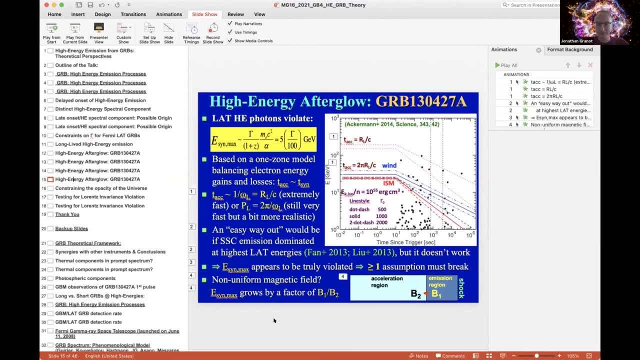 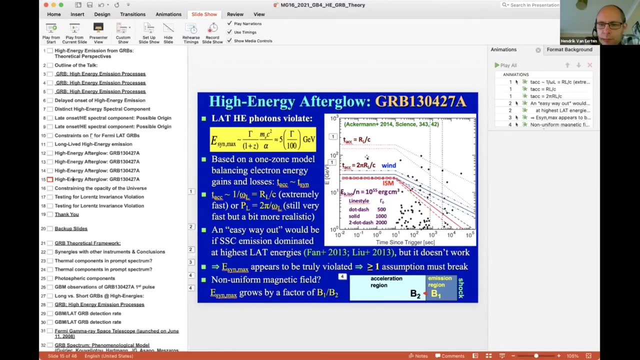 So it's potentially relevant for prompt GRB emission. Okay, thanks, Okay, thanks. So I see another question by Enrique, please, While you have that slide. I have a question, While you have that slide up, on the magnetic field. 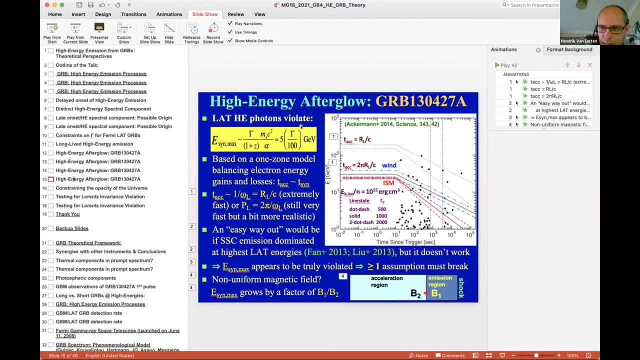 So I was just wondering: does this require anything peculiar for that to work, the B2B1 ration- or is this sort of a general recipe that provides a way out? Is this easy to achieve in practice, or does it require tuning of some form? 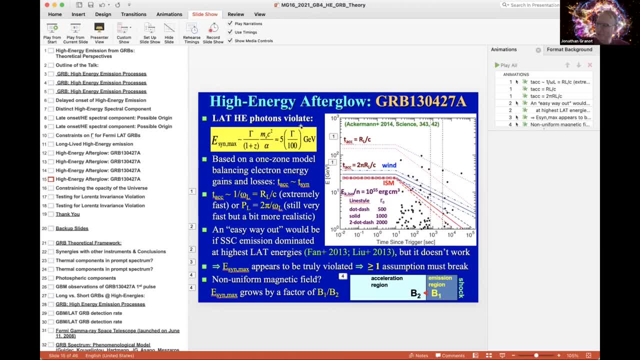 Well, there is still a lot of room for more quantitative study of this. So it has been put out, you know, as a toy model. basically so far. So if you have such a configuration it's possible, But how to get it in practice it's less clear. 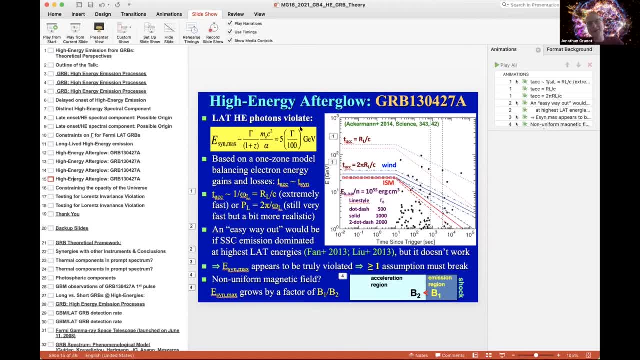 So we expect, you know, in the afterglow to have some initial amplification or generation of magnetic field just behind the shock. But then you expect it probably to decay over a certain scale. you know, maybe hundreds, two thousands of plasma skin depth beyond the shock. 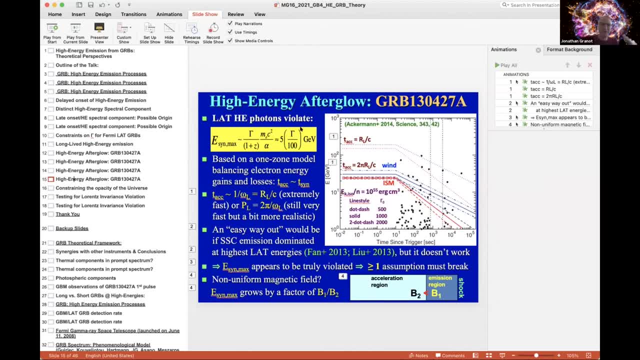 And then it could potentially saturate. it needs to saturate and not completely decay in order to in order to explain afterglow observations. but then again this layer would be fairly thin. so, even you know, a thousand or ten to the four plasma skin depths compared to the whole afterglow. 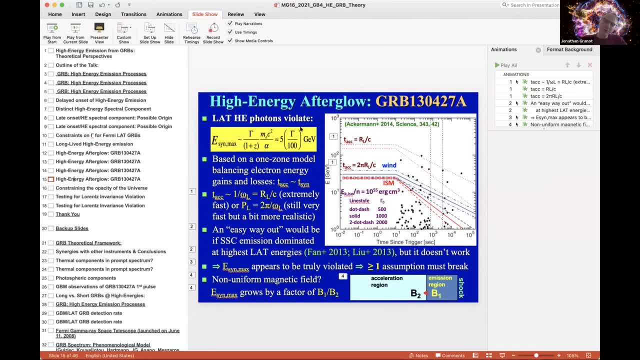 emitting region. it's a small fraction, so to have enough photons emitted there. it's not clear how well you can explain it quantitatively, even if qualitatively it might work. so that's a caveat and still needs to be explored in my mind. okay, thank you. 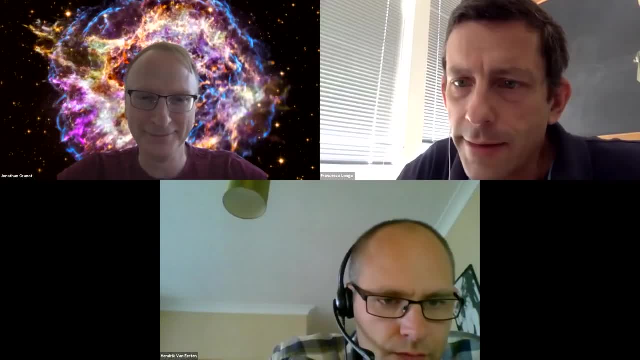 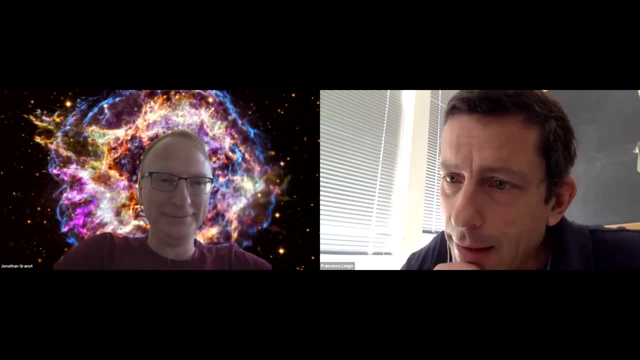 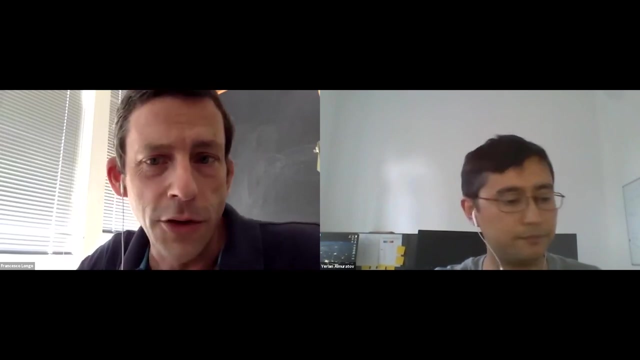 okay, thanks yoni and all the other that, let's say, participated to the discussion of this very first talk. so on the theory talking, and let's move now to the fourth contribution of the session, which is by: yeah, umar, out of. so, please, the airline is your turn. 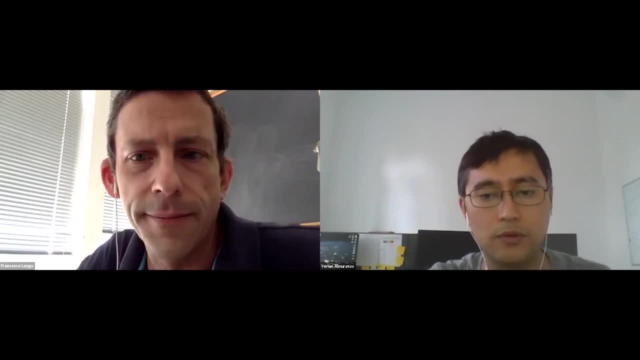 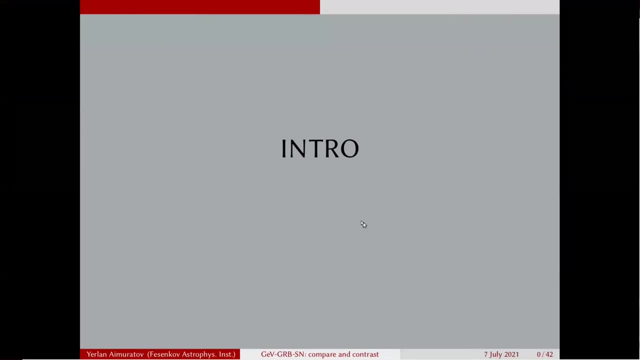 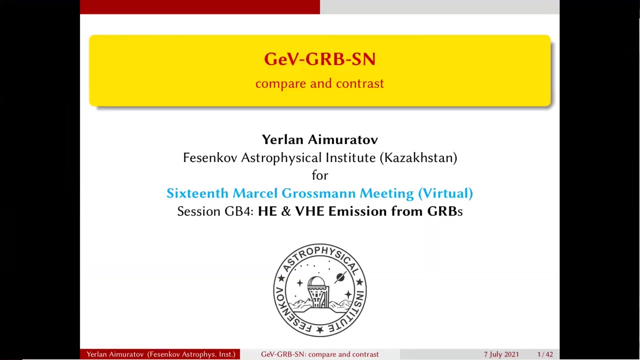 hello, do you hear me well? yes, yes, okay, let me share my screen first. do you see my screen correctly? yes, sir, yes, is. is it moving correctly? it is moving correctly, please go ahead, okay. so, hello, and thank you for inviting me to join this conference. today. i will talk about the gamma ray burst with high energy photons and associated with the supernova. 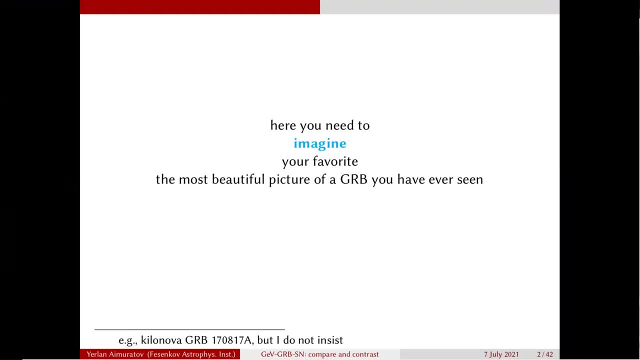 this is a talk which is based on a very fresh, new and maybe raw results still, but it's. it works to be mentioned and maybe we can discuss after all the details of other steps. okay, so we will talk about the main part. i will revise the main part of the grb supernova association and 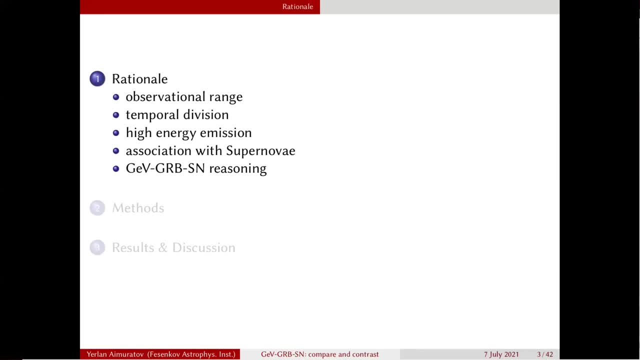 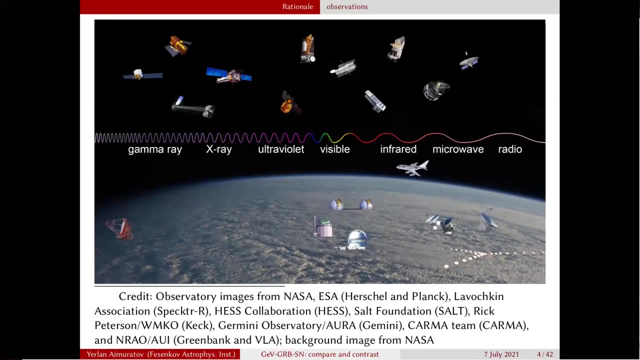 the grb- jeff photons association. then i will move to the methods and the results in discussion, the small discussion i have. so, as you already know that grb exhibits his behavior in all the electromagnetic spectrum, not only all but also the gravitational waves and we hope to be neutrino and 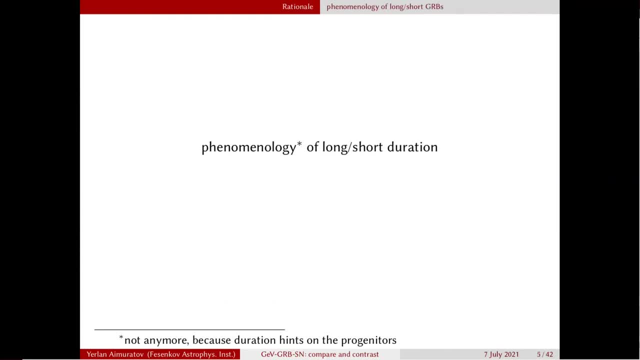 to come soon, and the first part to be mentioned is also is the phenomenology of the long-short duration. it is not more the phenomenology because, as you might heard also the, the progerentus, is hinted by the duration itself, but the but, the very, in the very beginning it was a really 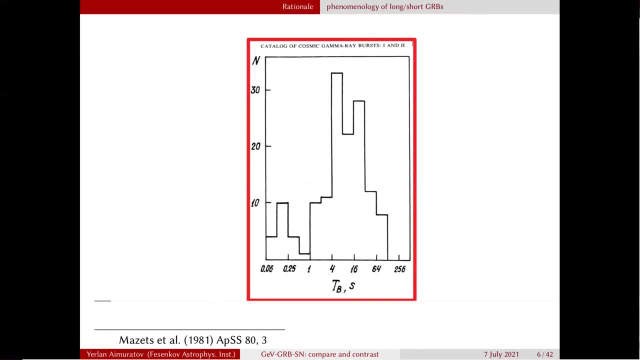 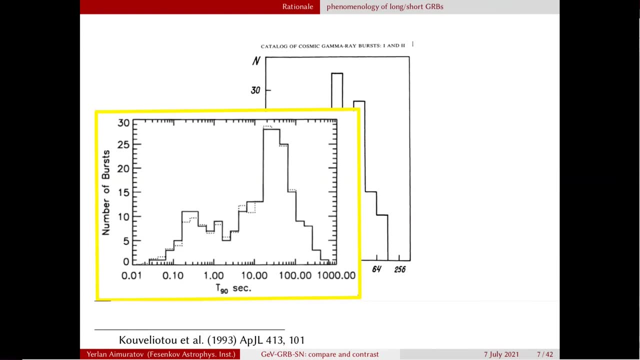 phenomenology. so people were observing grb duration and they they have seen that there was some behavior as well. but next, in very normal situation might appear natural. there is a very behavior dividing and showing the B-model distribution. The first hard proof for that was done by work in 1993. 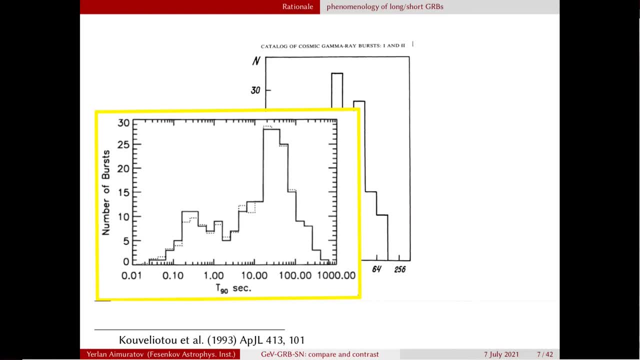 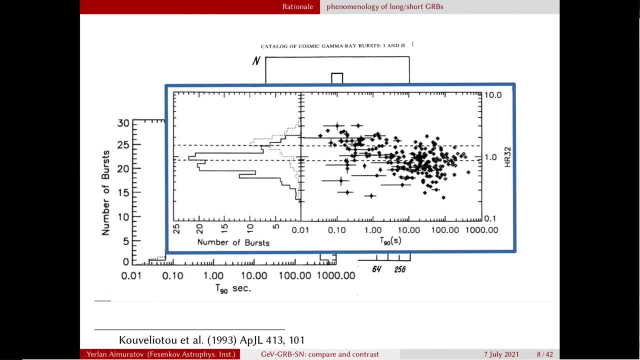 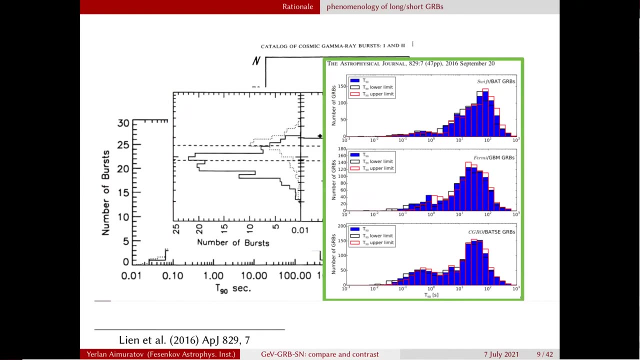 by Covigliato, which was then stood as the true, And then people started to look at this phenomenology from the other side and starting to search and to look for the theoretical models as well Further. by the way, this was done by the BATSI telescope. 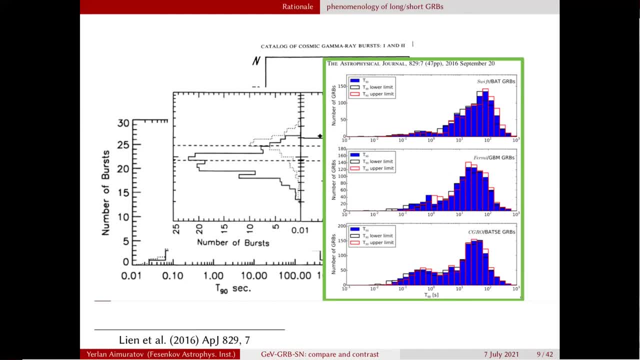 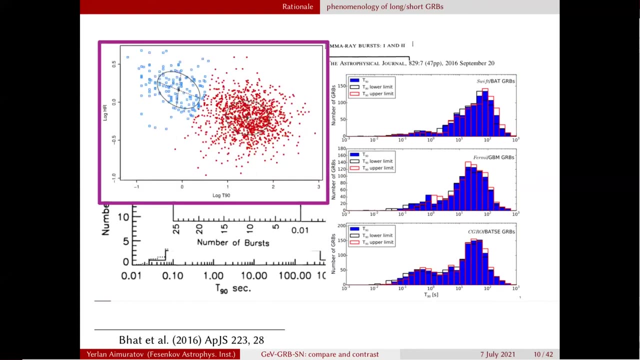 dedicated to the GRB study. Further missions like Fermi, GBM and the SWIFT-BAT missions also were observing the T90 distribution and also confirmed the B-model distribution. So also the hardness ratio shows that the emission from the GRB comes in two parts. 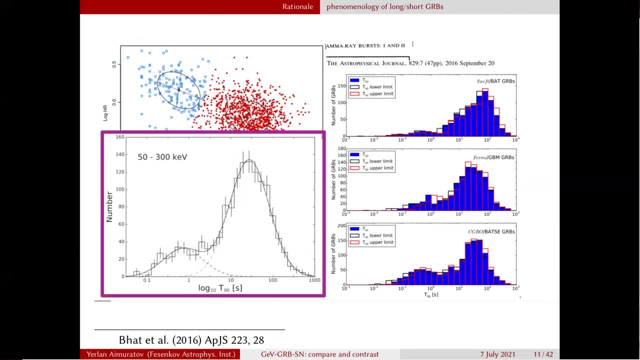 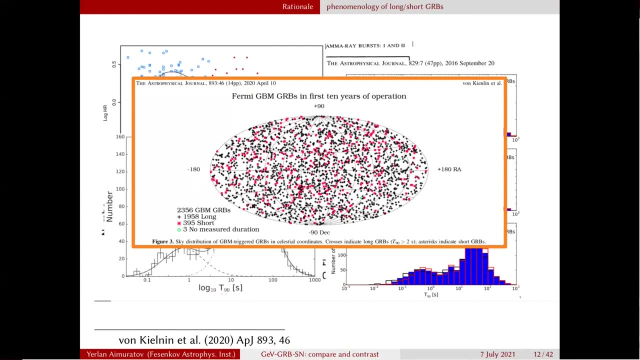 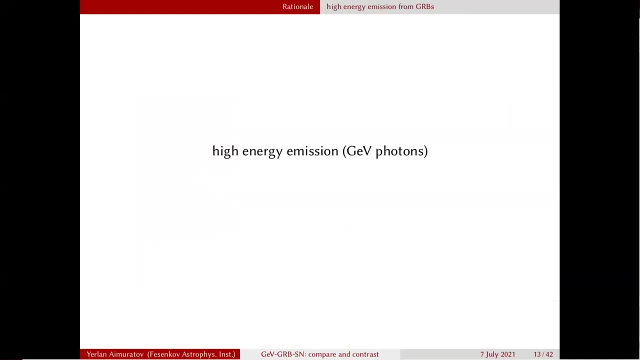 showing the distinct relation for that. So here's the recent results by paper 2016,. and here the Fermi results showing that the distribution of the GRB is, by the way, cosmological and comes from the outer universe. So another part. 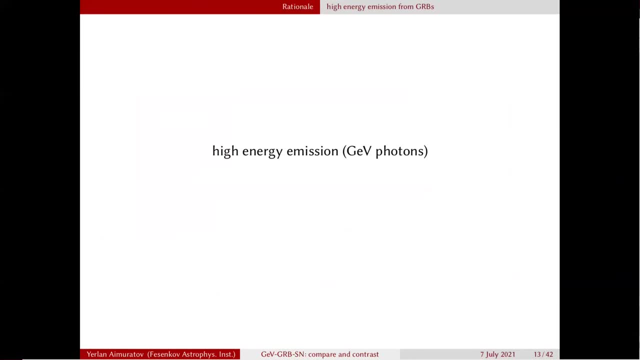 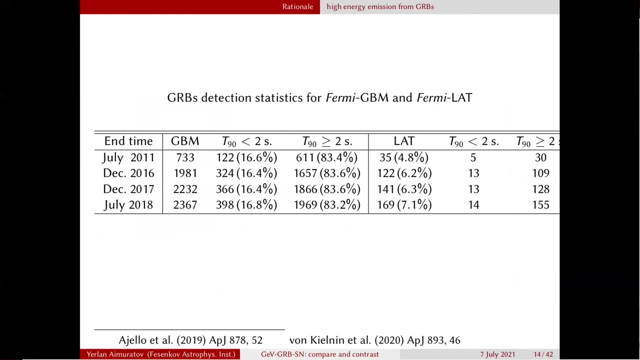 Which I would like to talk today is the high-energy emissions of the GEV photons from the gamma-ray burst, which was discussed also today by previous speakers And here we analyzed, here we showed the statistics And for the time of release of the second catalogue, 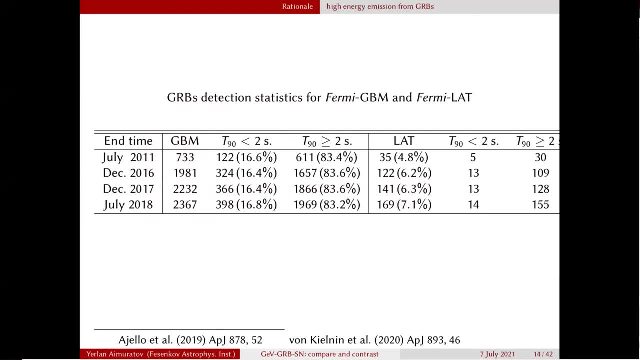 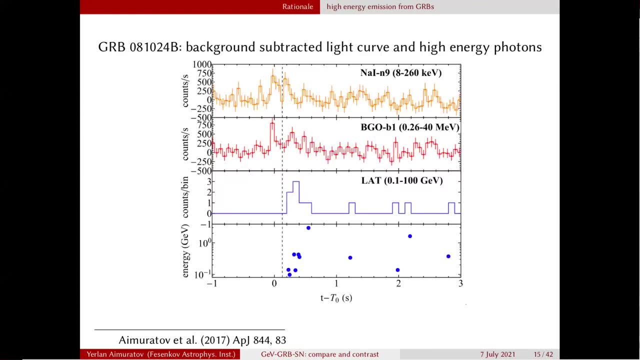 by Fermilab. it was around 169 LAT detections by the GRBs. And what is the high-energy photons? They are shown in the blue dots here and it shows that there's like a emissions count-like experiment of photons coming from the GRB part. 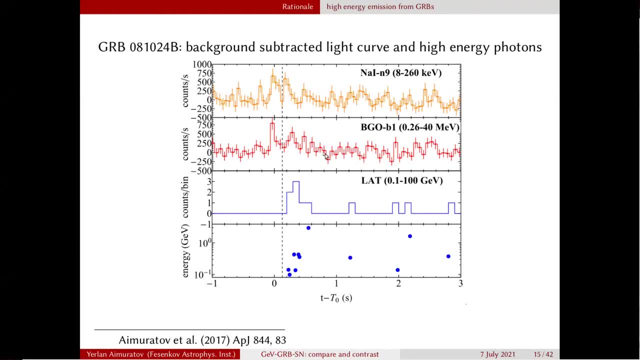 which has a random distribution actually and does not strongly correlate with the prompt emission in the key V-part as well. And then it was named after the GRB part, and it was named after the key V-part as well, And then it was named after the key V-part as well. 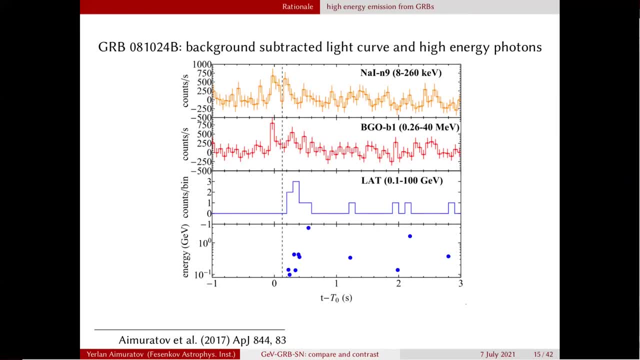 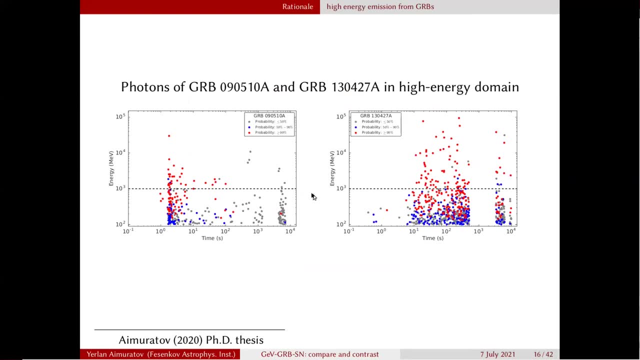 And then it was named after the key V-part as well, And then it was named after the key V-part as well, Which, because it happens for a long, extended time after the burst itself. So, and they are different in behavior and duration as well. 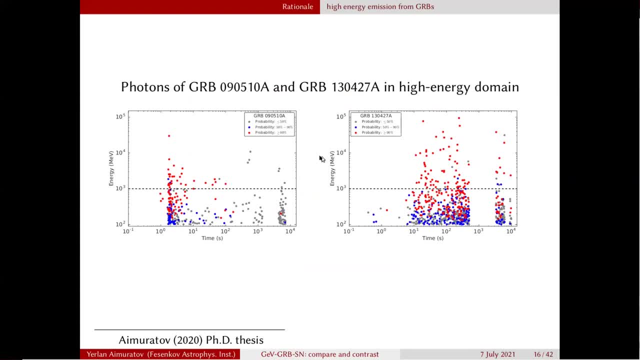 So, and they are different in behavior and duration as well, And they're present in the short GRBs and the long GRBs. Here I show the most prominent, like the most prominent iconic GRBs, from the short one and from the long distribution one. 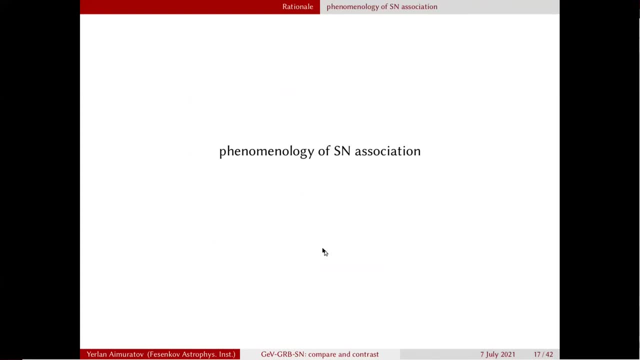 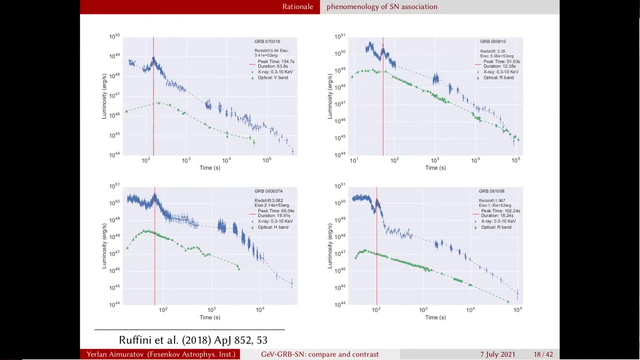 And from the long distribution one And from the long distribution one. Another part is the phenomenology of supernova association. By the time of the first redshift discovery, the first supernova association was found, and it is still be found by photometric. 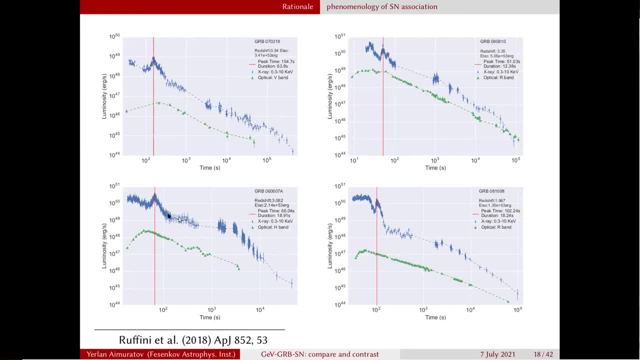 and spectral observations And the photometric observations here, usually in the GRB. here's the X-ray afterglow and here's the optical afterglow. And the photometric observations here, usually in the GRB. here's the X-ray afterglow. 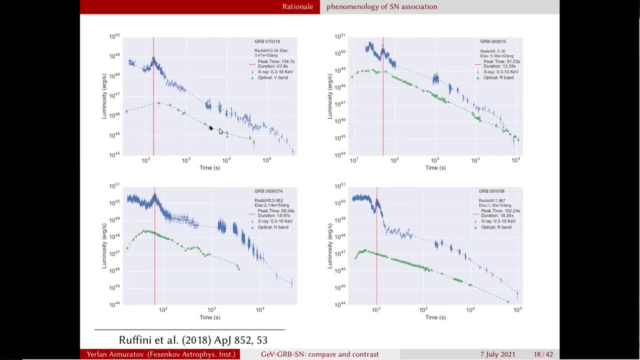 for example, The optical afterglow has the simple power law behavior. The optical afterglow has the simple power law behavior. The optical afterglow has the simple power law behavior during the time And when we see the, when we associate the supernova with the GRB. 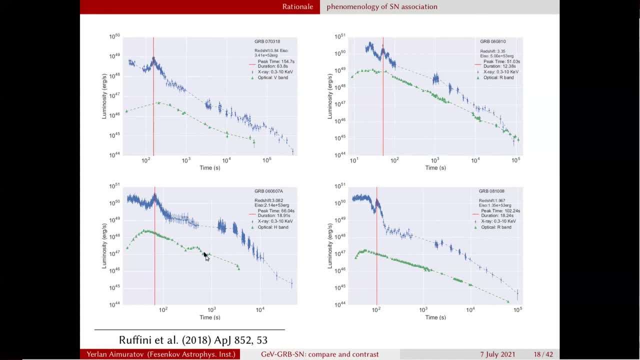 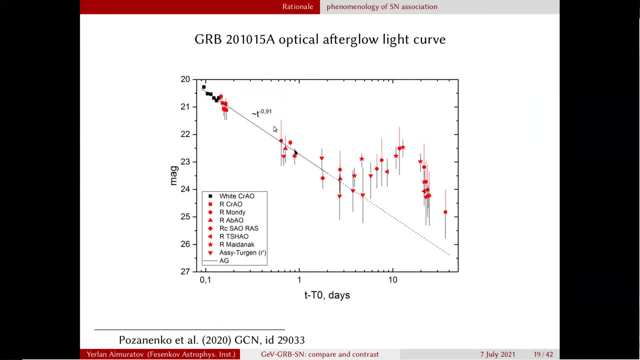 we say that there is like a bump behavior. By the way, this bump- I checked- is not about the supernova as well, this one. So the bump is shown like here: it's faster, brighter. So the bump is shown like here, it's faster, brighter. 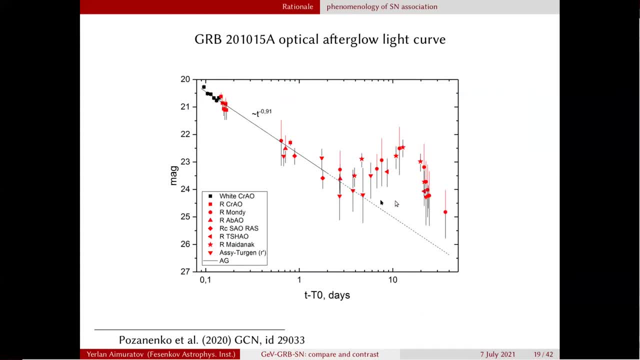 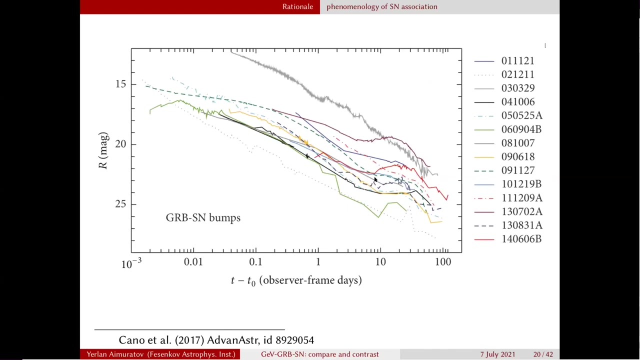 and it's brightening in the magnitude, like within days. It usually happens at 10 days. So the first 10 days, depending on the evolution of the burst And the increase, could rise even like three, four magnitudes And the bump behavior present in all GRB. 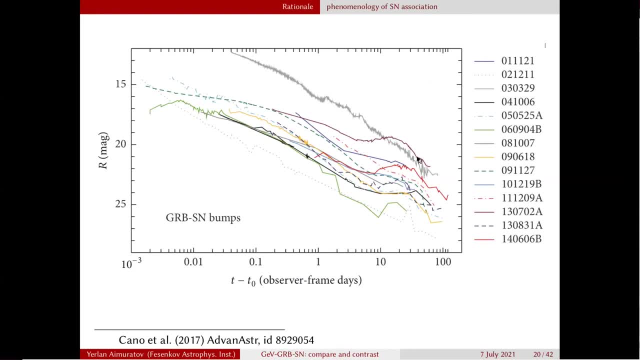 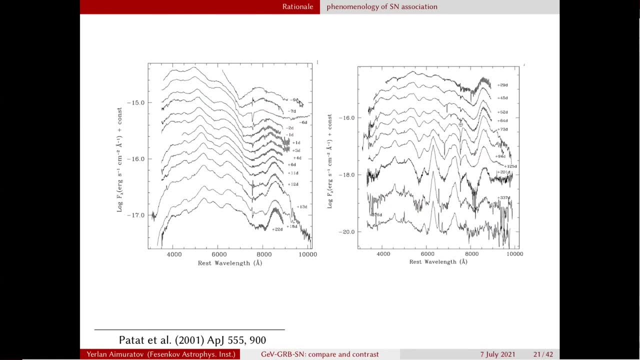 associated with the supernova photometrically, but as well we have spectroscopic evidence for the association. we have spectroscopic evidence for the association with the supernova. So when the big telescopes look at the position of the GRB after and follow up for several days, even months, like here, 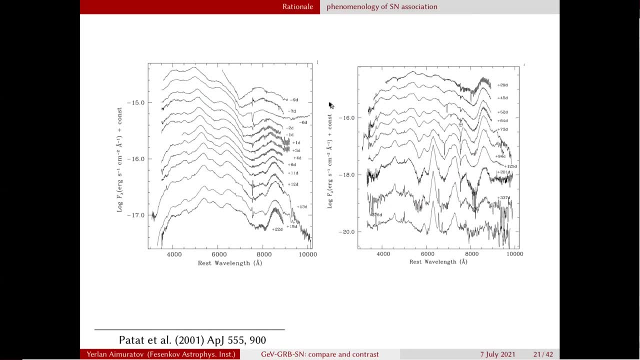 they see that the emission, the spectrum, evolves towards the broadening of the absorption lines And it shows- here is the, the spectrum, the absorption lines. And it shows- here is the, the absorption lines. Here are some of the prominent lines. 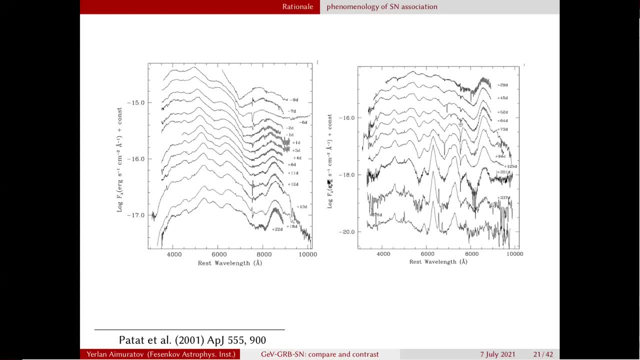 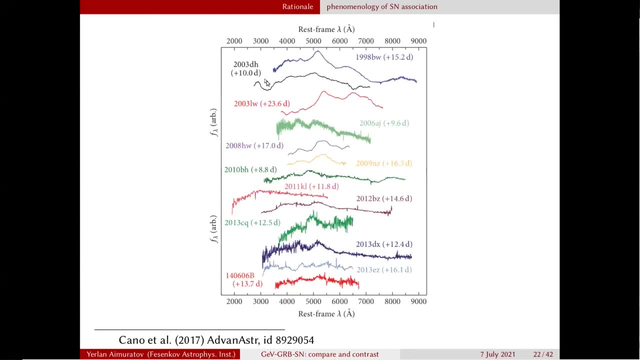 by which it is identified as a supernovae, And it evolves drastically, So the supernova itself. Here's a collection of the. here is a collection of the several supernovae associated with the GRB And you can see that the spectral behavior. 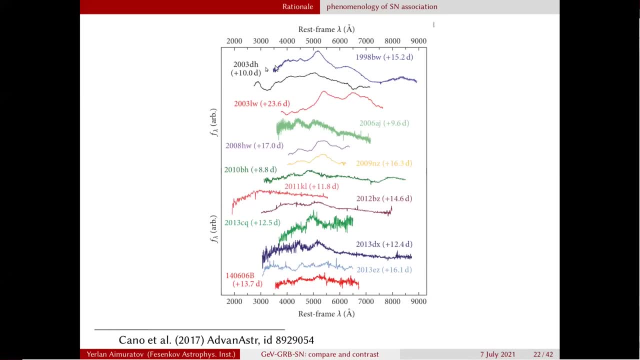 is somehow random. to be honest, this is dichonic 1998 BW. here's a collection of the several supernovae associated with the GRB and you can see that the spectral behavior is somehow random, to be honest. the first one of its kind, GRB-associated supernovae. 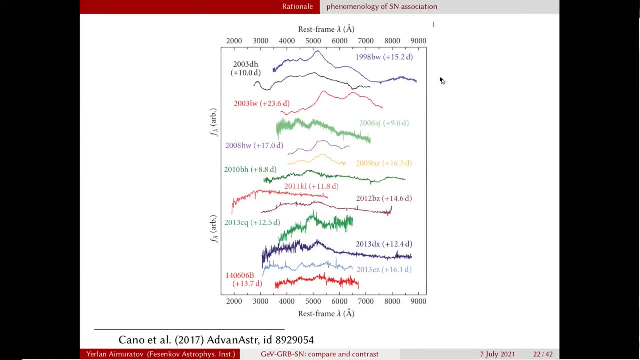 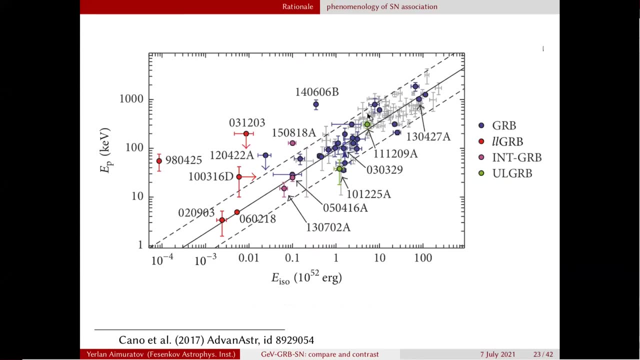 And it's like a standard ruler to be measured with the new candidates And looking at the energetics of the GRB-associated supernovae, one can say that there is not so much behavior showing that they are located separately from the rest of the long GRBs. 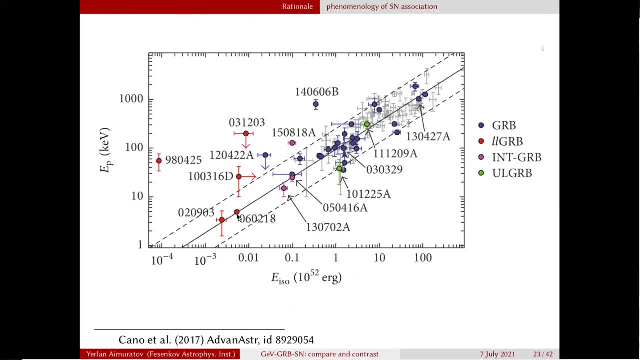 By the way, they are associated with the long GRBs- because there is enough time to detect, probably, I mean from the observational point of view, And here in the colored dots you can see the population of the GRB supernovae. 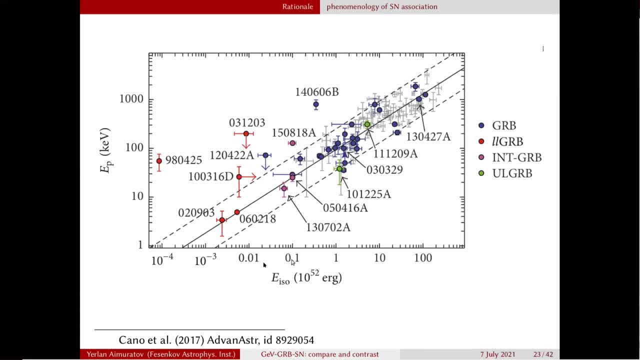 And you can see as well that the energetics of the prompt emission of the GRB spans from like 10 to the 54 Erg to the 10 to the 40, even 10 to the 48 Erg energies And the peak energy in the spectrum on the prompt emission also. 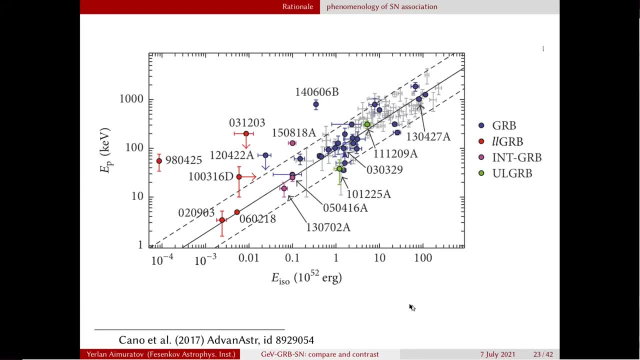 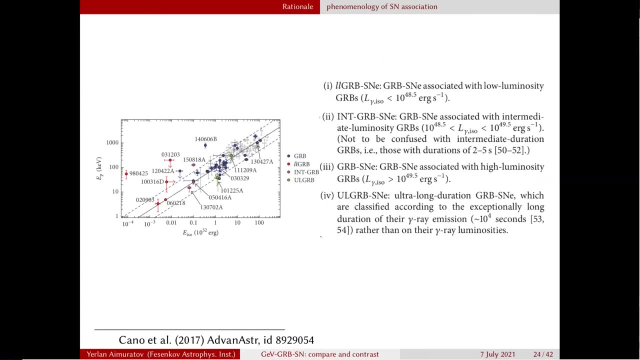 scatters like three orders of magnitude. So by having the first, reliable and like quite enough number of GRB supernovae, there were attempts to classify them And mostly they are classified, as you can see, by the luminosity, So the brighter they are. they are collected in one sample, in one group. 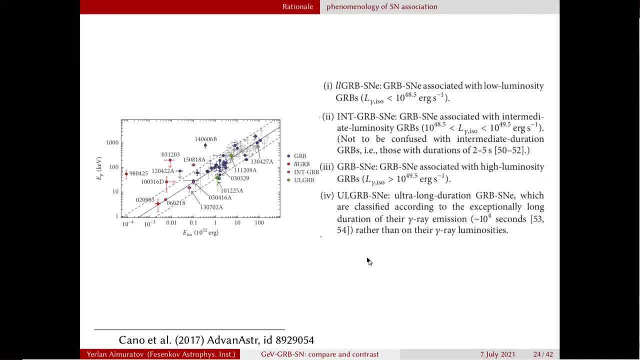 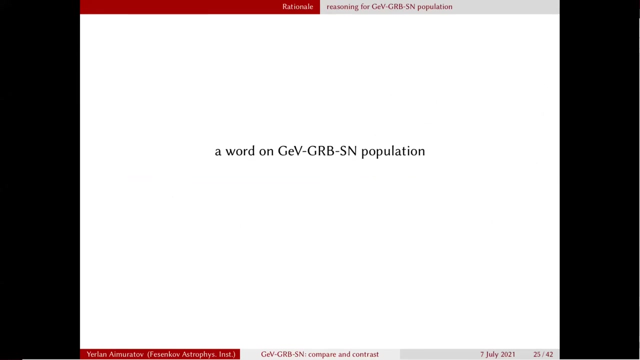 And the dimmer. they are collected in another group. Another category is to look for the duration, So it's like ultra long duration GRB supernovae. So they are responsible for the different mechanism of anything also. So we now want to focus on both the collection of the GRB with the Jeff photons. 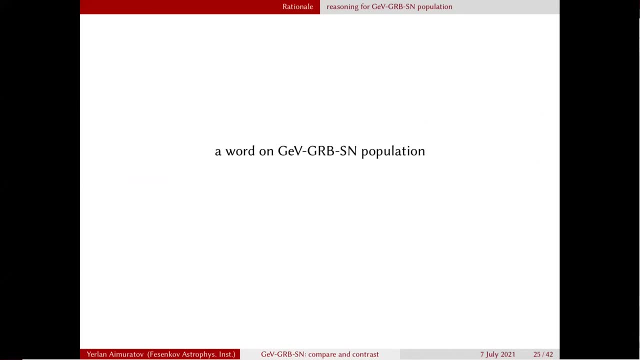 and GRBs with the supernovae. So it's like a kind of intersection of these two groups And the reason you can expect that this sample is very small, And indeed it is very small. But let's try to look at them. 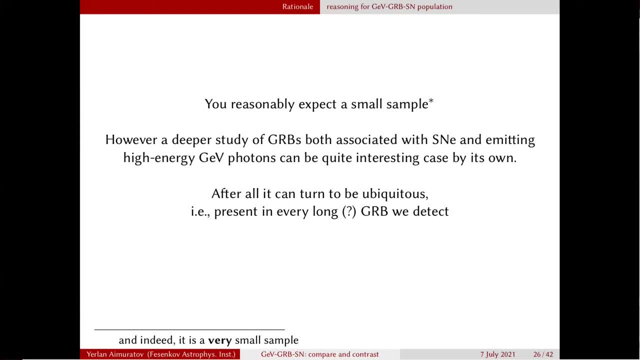 And maybe we can see something interesting for us. So the method is very simple: We just intersect two populations And, of course, due to the possibility of Jeff detection only by Fermi, we focus on the era of Fermi-Lath operation. 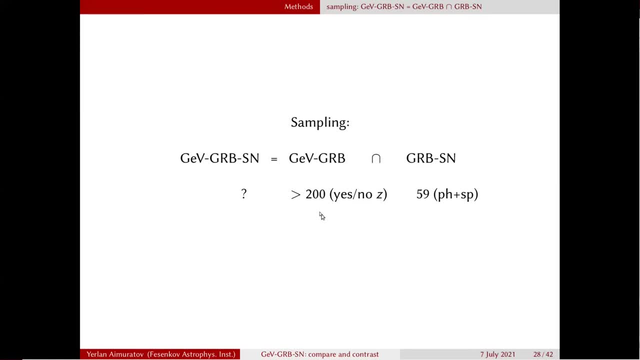 To the moment, to this year, there are more than 200 or so GRBs with the high-energy photons, both with and without blood shift, And there are around 59 GRB supernovae. Half of them happened before Fermi era. 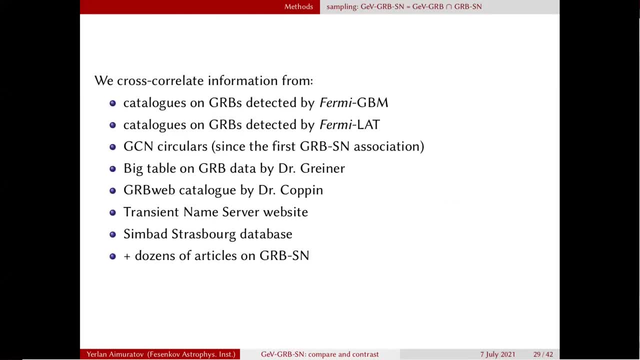 So we just throw them out And we just look for the and cross-correlate the information from different catalogs of the Fermi, the GCN circulars and the Big Table By Dr Greiner, Dr Kopin. 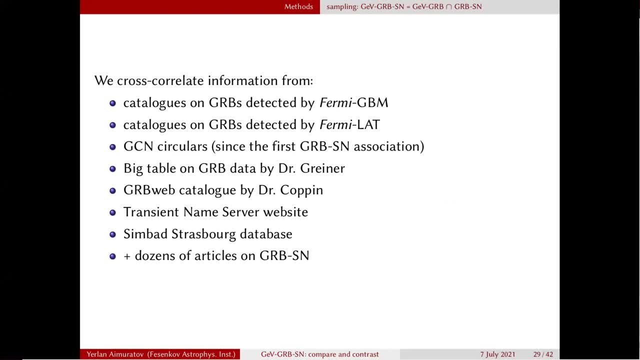 and also research for the information of the supernovae, because there are many transients happening And the supernovae are obtained like in the usual way now, not like 10 years ago. So it is reflected also in the naming of the supernovae. 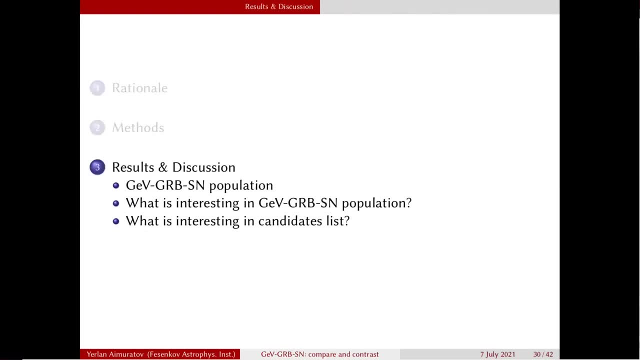 We can see later And by collecting this information, we have only five GRB, GFGRB, supernovae population to the time. We have 25 more candidates for that And we are checking now, then, And you can see that from the first glance. 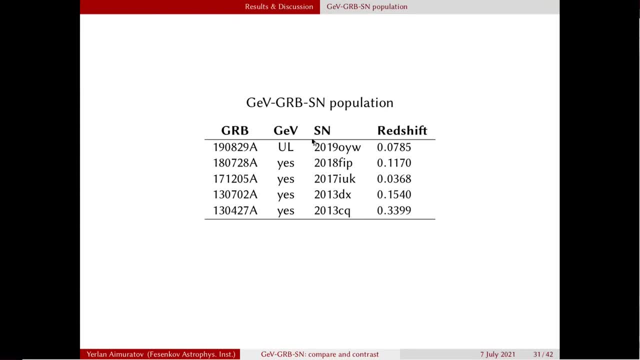 if you cover the GE part, you can see that the GRB supernovae properties for the redshift are more or less standard, Usual Less than redshift two. It's obvious, And their behavior. their behavior is also standardized to the supernova 1998 BW. 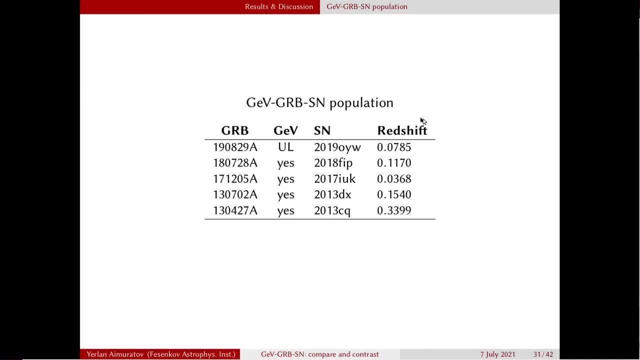 So in the energetics they are different- I can show it later- And all of them have the GEV present. This is puzzling because GEV photons is believed to happen in the energetic GRBs. As we know, the supernova happens in GRBs. 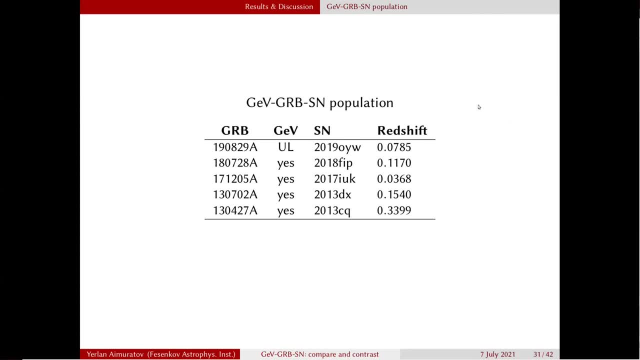 which is less energetic. So this could puzzle a bit, but it tends to be. it tends to be true that the GRB, GFGRB- supernovae is less energetic in most, but this is not the ultimate case. So there are 25 more candidates. 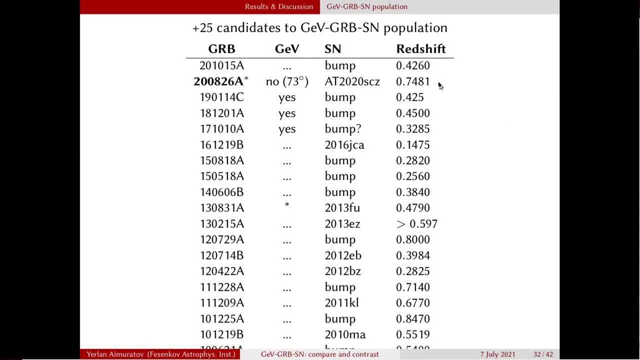 to be checked, And one of them I will discuss later. This is actually 2008,. 2068.. Actually, the reason I have studied this population in detail, like you know, three, three weeks ago, months ago, 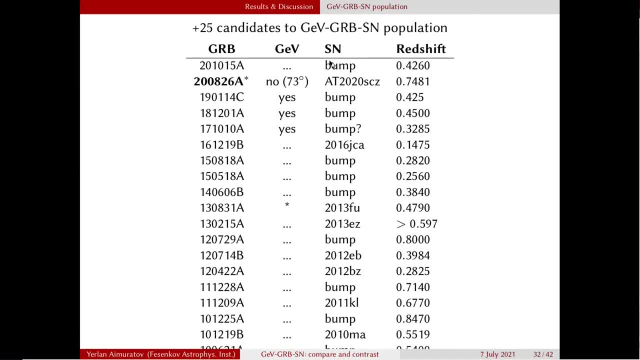 I started this work, So the the the results are very preliminary. So, as I told you, you can see the bump in the light curve or you can spectroscopically identify them- the supernova, after all. So they are identified. 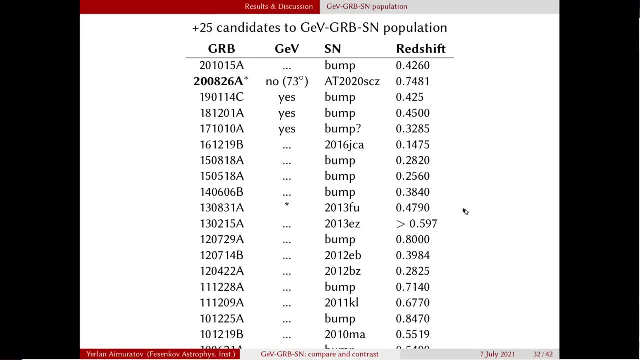 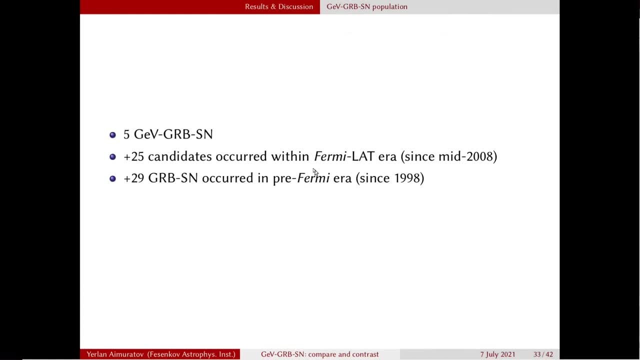 and for the, for the rest of the GRBs you can see here without GEV it needs to be checked, like for the upper limit also. We're we're still doing this work. You have a few minutes, Two minutes. 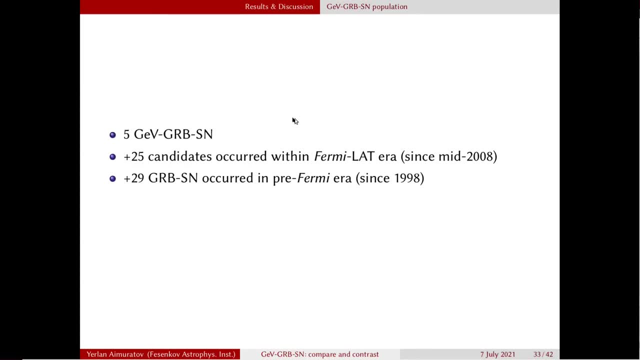 Okay, Okay. So, as I told, there is like a five population, five objects of the population, 25 candidates to be checked and 29,. unfortunately, we cannot check because it happened pre Fermi era. So let's move on. 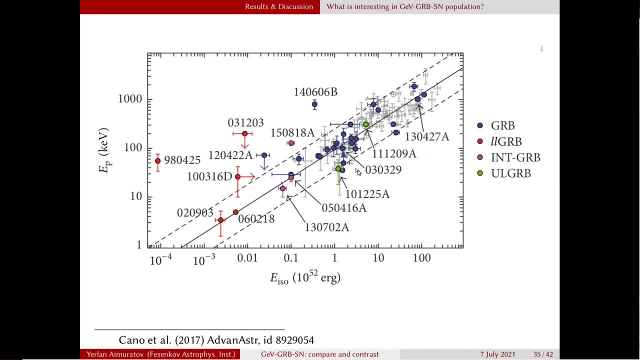 What is interesting in our population. So, as in, as in previous result, this GRB 130427, and this GRB 130702, GEV GRB supernova residence. So you can see that the energy spans, the tropic energy spans a lot. 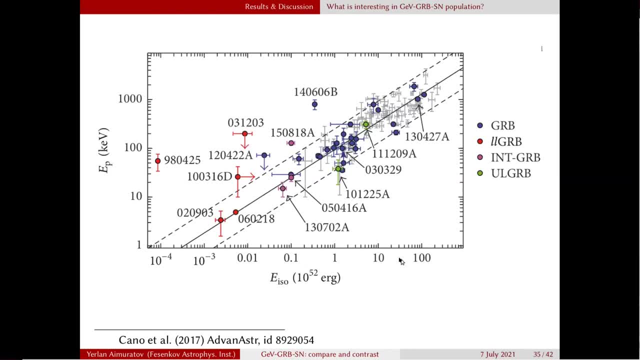 This is a, by the way, the EPTI is a matter. relation for the for the spectral harmless. also Another two, another three candidates happening, also showing the diverse behavior on this plot. For example, 17,, 12 or five is a two to the 24.. 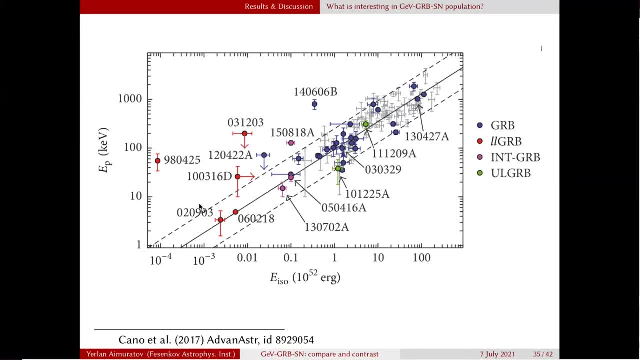 Eric is up to here. This dot, this dot here. So the, the, the peak energy, less than 100.. And another two is a 10 to the 51. So is around here up And 10 to the 50.. 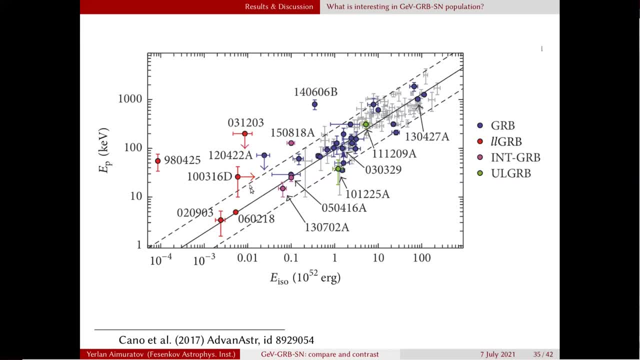 And also around around here up. So you can see that the energetics is in diverse but it. but it could hint us that maybe, maybe also the, the, the GRB, with the supernova lacking, the GEV mission can also emit. 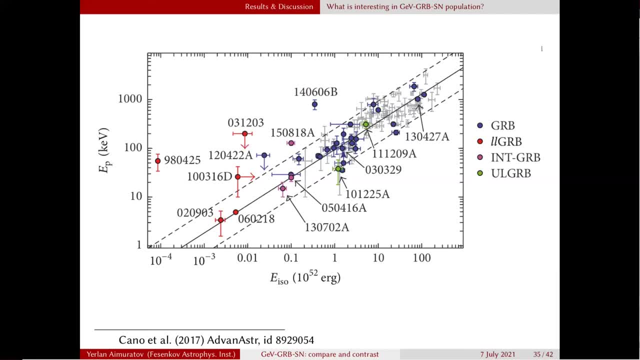 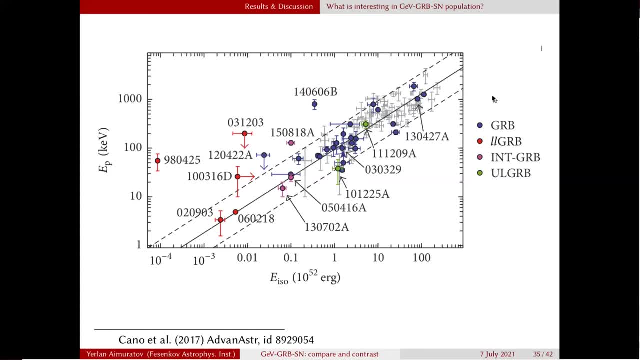 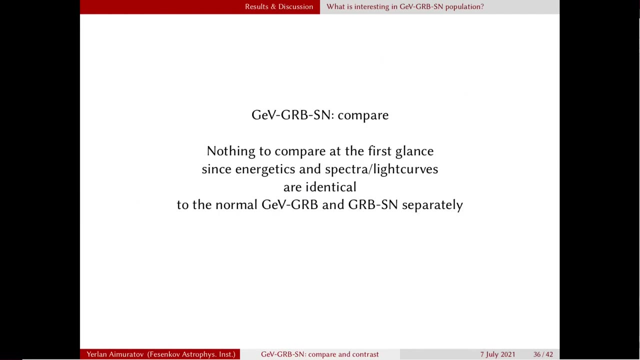 it could be it could, it could also tell about. it could also tell a lot about the, the energy level, Or can it have a lot to do with the? denken gives something. It can hint us that it could also emit geographical. 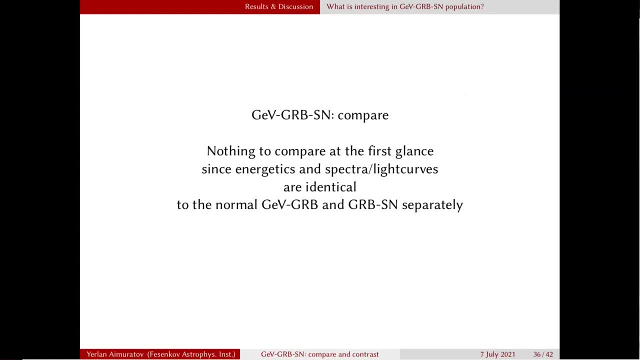 We lack due to the, The line of sight Properties, or due to the sensitivity of, Which is discussed many times in the papers. So, at the first glance, stone for this is a candidate which we are still analyzing of the is the 2008 26a the, the grb. 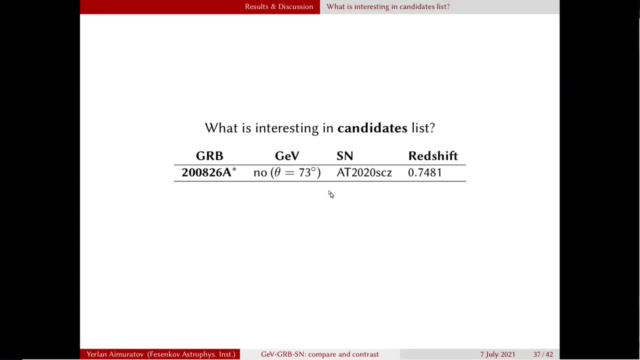 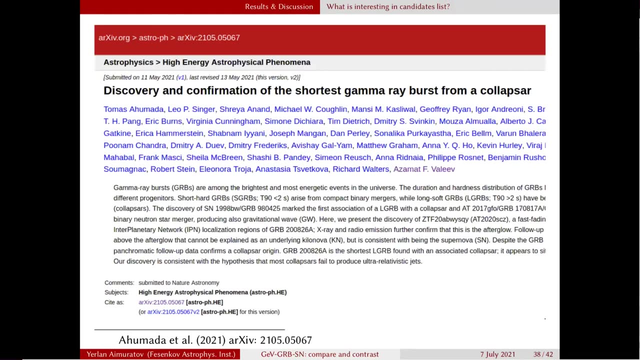 associated with the supernova. fortunately, the the boresight of the fermilat is 2073, so we can calculate the upper limit for that later. and this grb is something new because its duration. this is the grb associated with the supernova and it's and it's like the mechanism for that. 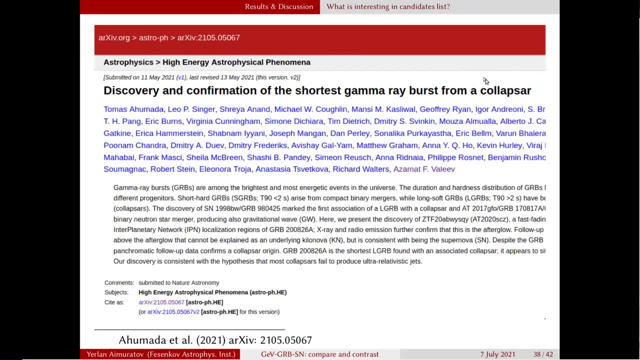 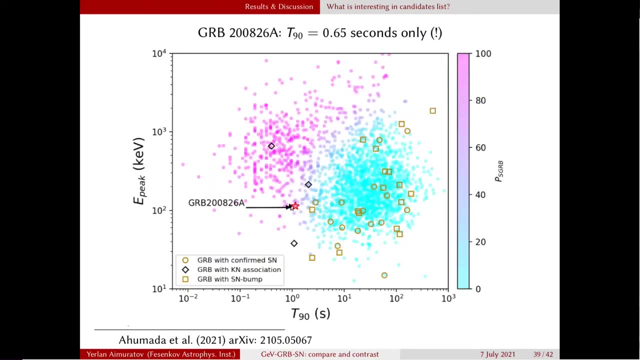 is like a collapse is discussed in this paper. it's a very fresh paper of like two months ago published, but it's a short gamma ray burst and for uh, surprisingly it's t90 duration is 0.65 seconds and the location on the epic t90 diagrams are on here, but probability of the analysis shows 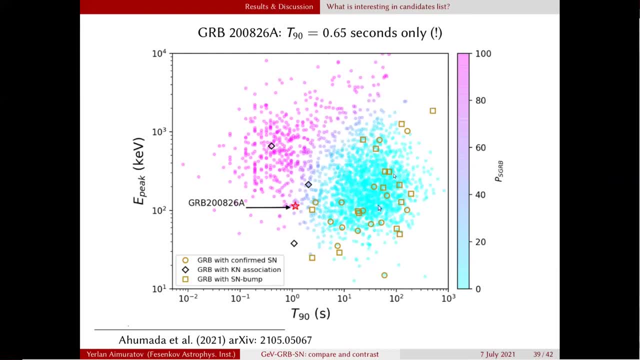 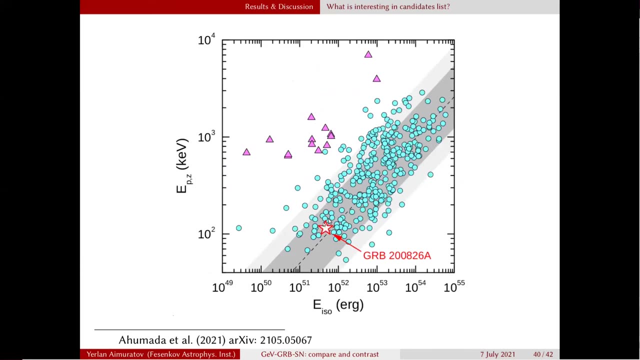 that it most likely to happen in in to belong for the long population in first, but nevertheless okay. gamma ray duration is 0.65 seconds only and you can see and compare with the previous epi, kiazo, so it happens as well in within the amati relation with the good correlation. 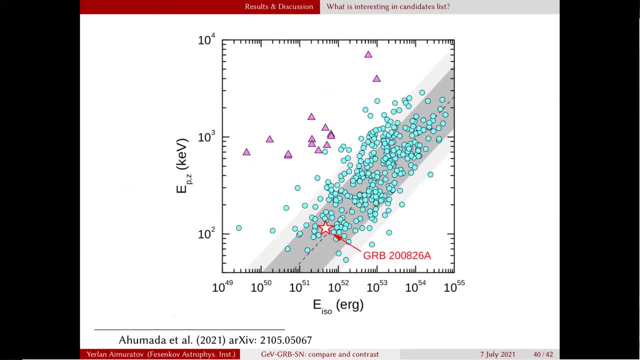 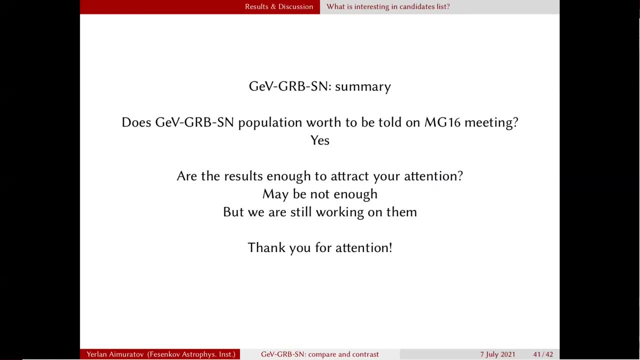 so does it mean? does it mean that uh jr population worse to the mentioning on this meeting? definitely yes, because you can see it is puzzling by energetics, because it spans for five orders of magnitude on e isa and there is as well short duration, uh prompt emission, which also occurs to be a collapse star in the end. 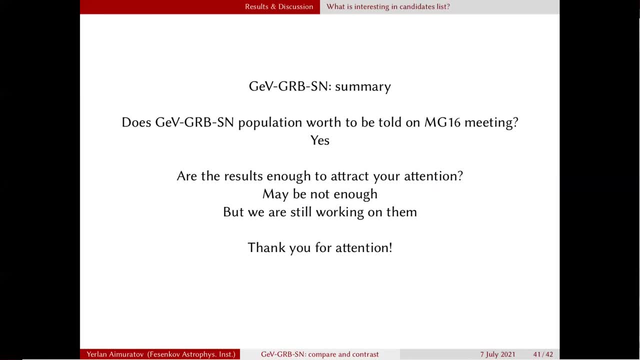 by identified by, by panchromatic behavior of the collapse of origin and as well, it happens at close redshifts, at close distances, so we can study them in more detail and maybe in the future we can prove, show that more grbs with the supernovae or more grb with the high 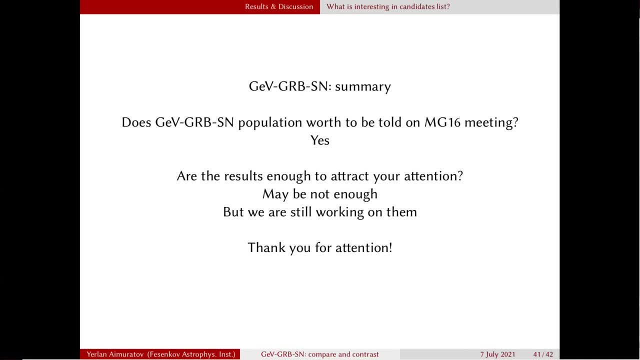 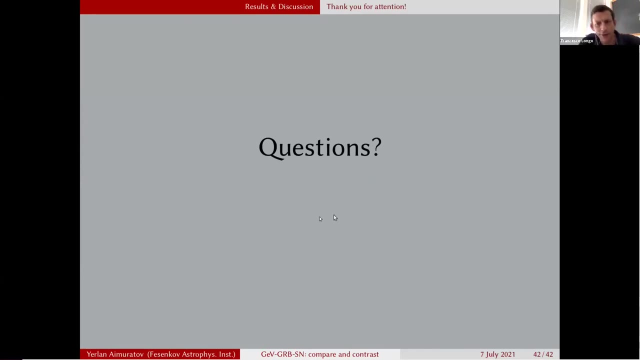 energy emission can be unified and show both behavior, maybe with the instruments with more sensitivity as well. thank you, thanks for your questions. thanks, yerland, for also the nice talk and the nice topic that you raised. so there is time for one question only, unfortunately so. is there someone that who wants to ask something to yearland? 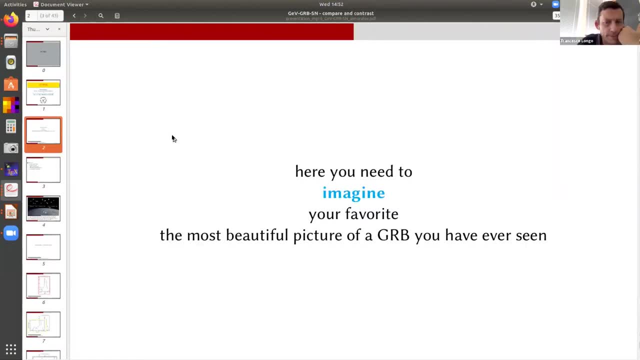 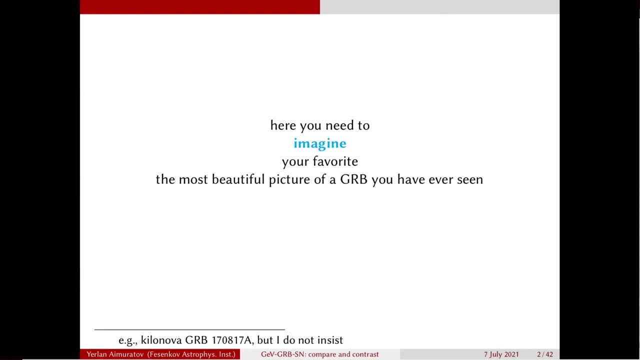 otherwise i have one small, okay, ionic, please. what is so special about this event? if it appears to be, you know, on the borderline between long and short grbs, so it naturally is intrinsically the long, hard class of grbs and therefore shows a super long and short grb, which is an increase in the 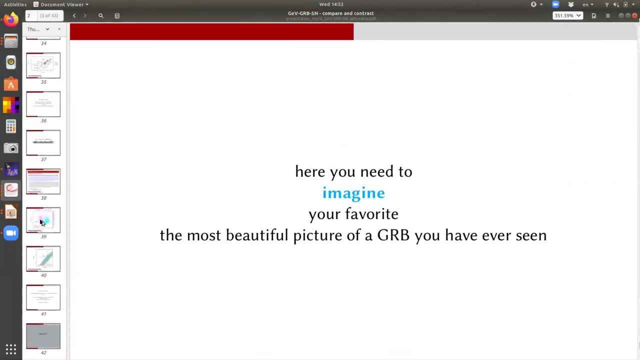 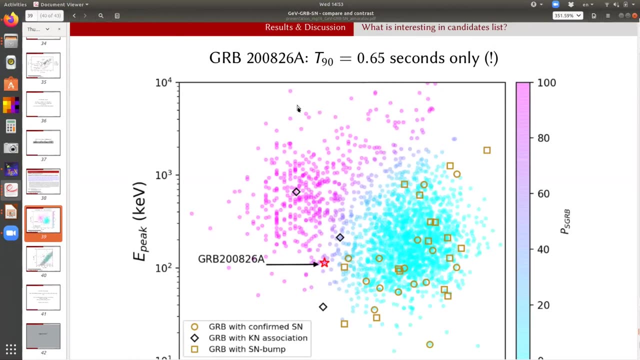 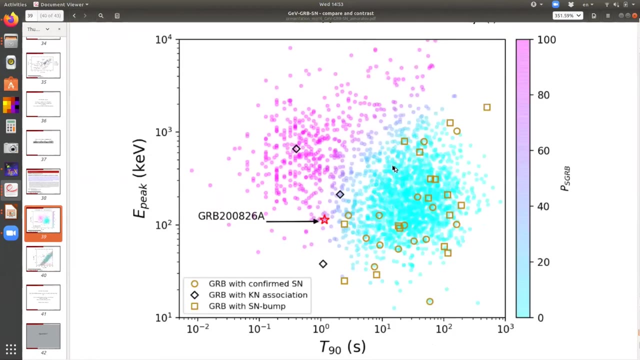 shows a supernova. what's so special about it that it made it to nature astronomy? yeah, in sorry. yes, indeed, it goes to the nature astronomy under the revision, but uh, it's surprisingly short. it's 0.65 for my, for my experience, uh, this borderline uh short, long, actually long duration, GRBs happens. 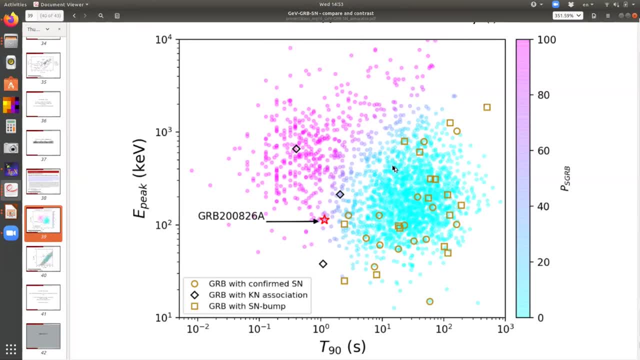 close to the to the two seconds and in most cases I have seen that uh, short GRBs happening, crossing the border of the long population. but it could hint us that, uh, maybe the behavior which we see through the prompt emission and we identify them as long and short. 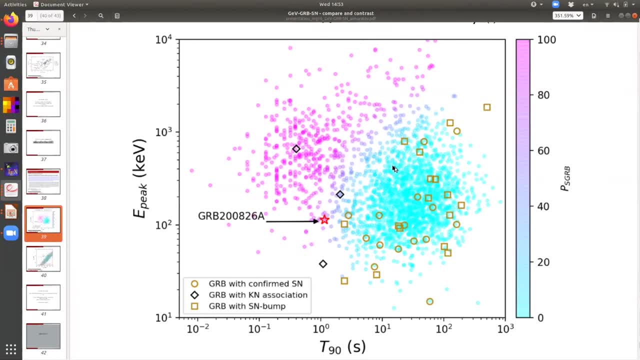 with and without supernova, or with or without GEV, photons could actually be hidden due to the circumverse area or the, the geometry of the burst. so, yeah, what I wanted to say, that maybe they all show the presence of GEV emission as well, if they are, and, and, the, the, the energetics. 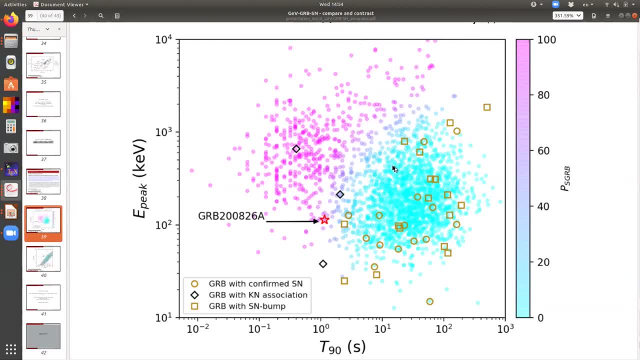 is not a matter for them. as you can see, the uh, the span of energy in four, five points. okay, see another. raise a hand by bim bim. please go ahead. yes, uh, this is actually a comments on the GRB遊戲と of the question. uh from uh, uh, Jonathan, so basically, uh, if we 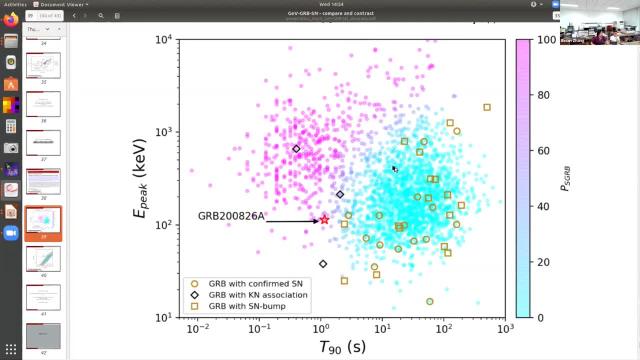 look at the paper. we have another paper. uh, uh, this is like a code submitter to a neutral astronomy. the point is that this burst is definitely a short near me. uh, in terms of the duration is very sharp spike. you cannot claim there's a tip of iceberg. uh, GRBs and uh GRBs like. 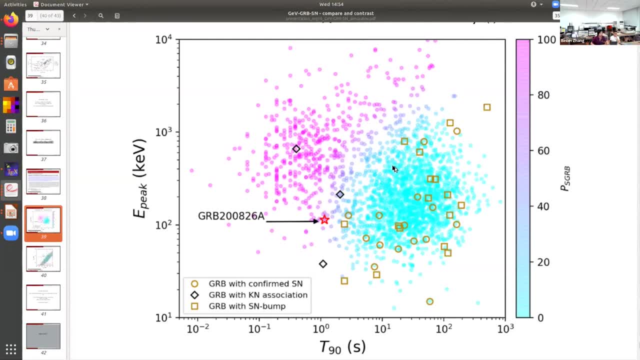 this is sharing an trochę quickly. um yeah, as we go to another slide, so anotherurf, sim�d bmgis, which has shown before we have a short GRB associated with a simple NOA, but you can claim that's a typical iceberg. intrinsically it is long. 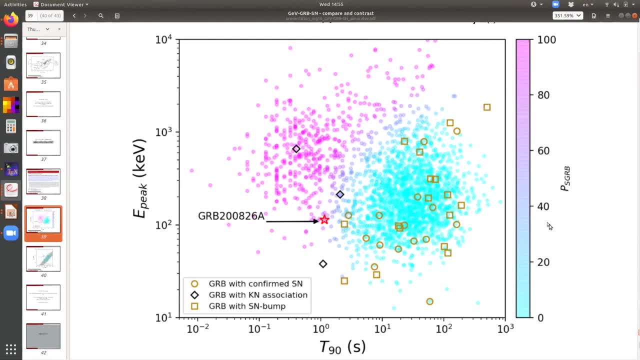 But this one it's definitely short. Rating wise, it is definitely consistent with being long. You can see here that it's exactly on the borderline between long and short GRBs, and there are long GRBs that show very sharp spikes as well. 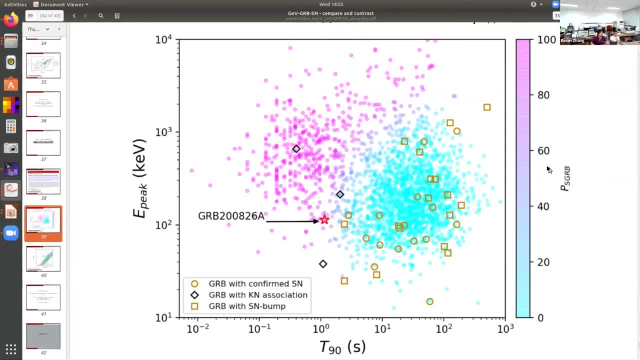 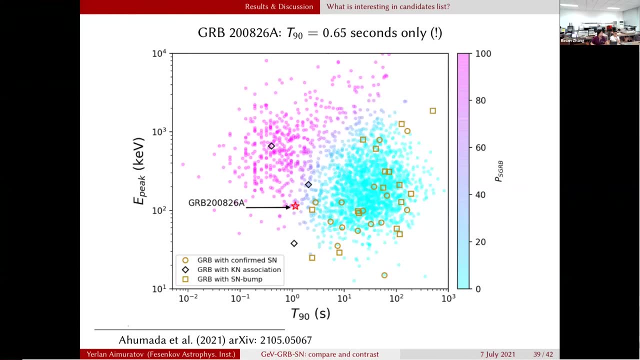 If you really look at the light curve, this is actually the most spiky one among all the short GRBs. So that's the key points. We didn't see the light curve here, but you look at the light curve, you actually can get this point. 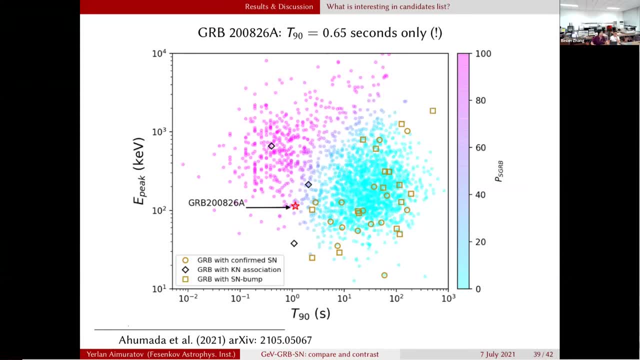 Yeah, that's just my comments, Thank you. Okay, sorry for interrupting because we need to go ahead, but this, let's say, topic is very interesting. So, if you want to, as I said last time, if you want that, we can create a breakout room. 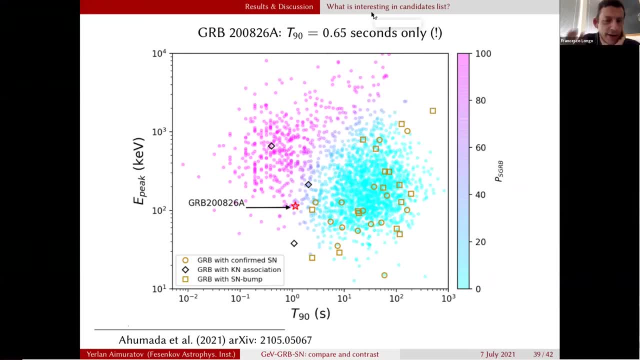 so any of you who want to discuss privately about, let's say, continuing to discuss as it was in a real congress during the coffee break, you can do that, And let me, or Fabian do, to create a breakout room for you. 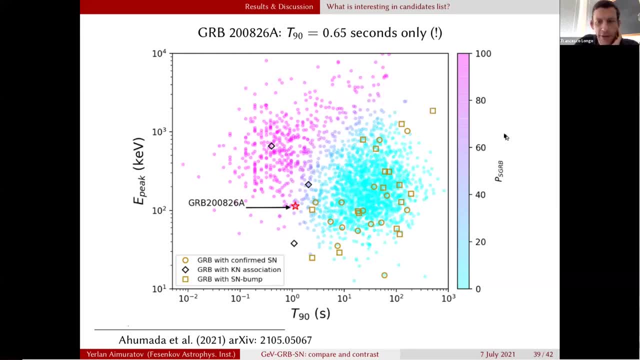 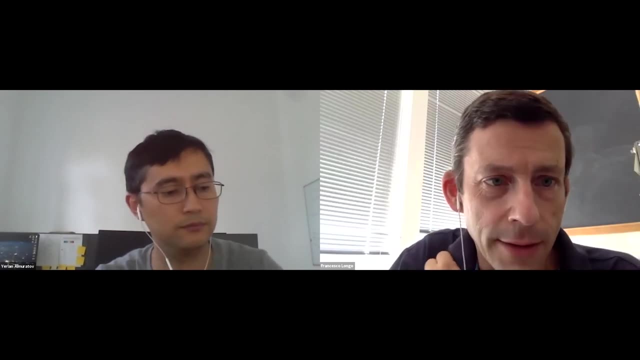 So now let's thanks again, Jarlan, for the nice and stimulating talk. And then let's move to the second theory talk for today, And we have heard about the, let's say the interpretation of the GV part mostly. Now we will ask- we have asked Jelica Bosniak to discuss. 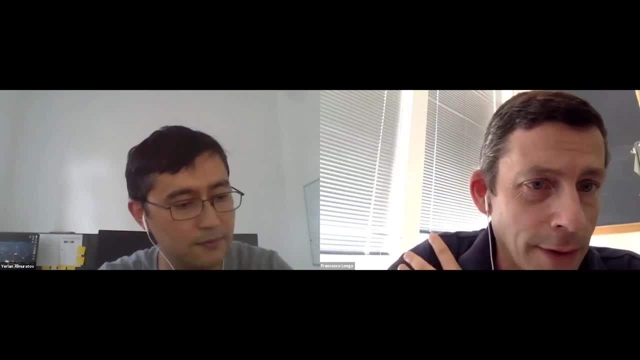 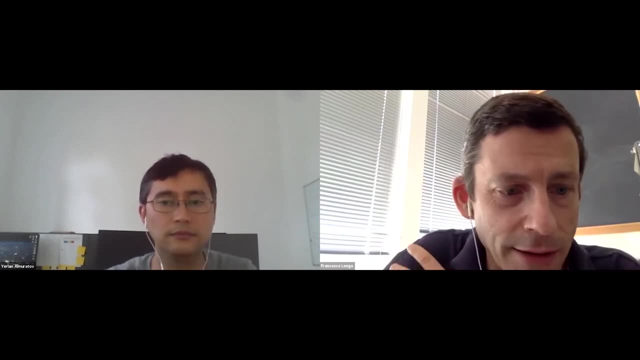 about the prompt emission, especially for in the view of the possible future detection of such component in the energy part. So, Jelica, it is your turn, Please, if you want to start sharing your screen. Can you see my screen? 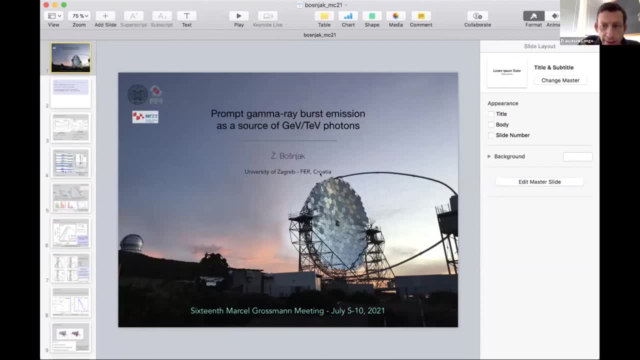 Yes, and we can hear you very well. And while you start sharing, I'd remind every of you: if you want to share your slides on the Indico, please do so so that we can have access to them also later on. 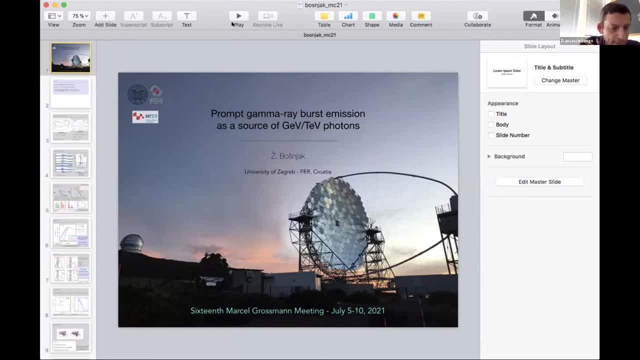 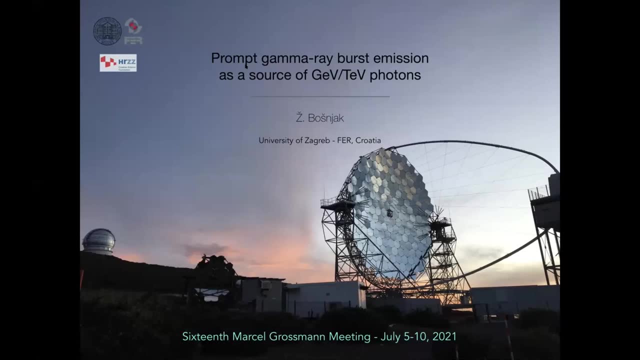 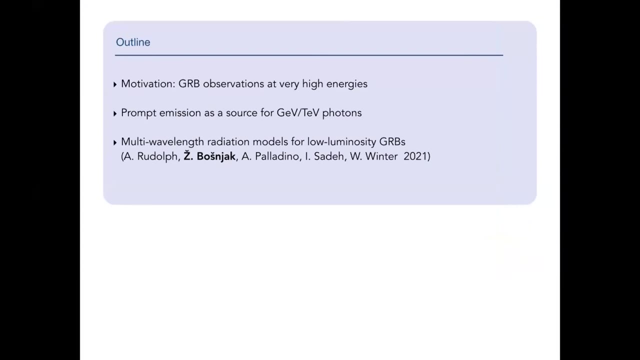 if you want that, Okay. so please, Jelica, go ahead. So first I would like to thank the organizers for inviting me to present my work. This is the outline of my talk. I will briefly present some observations at high energies. 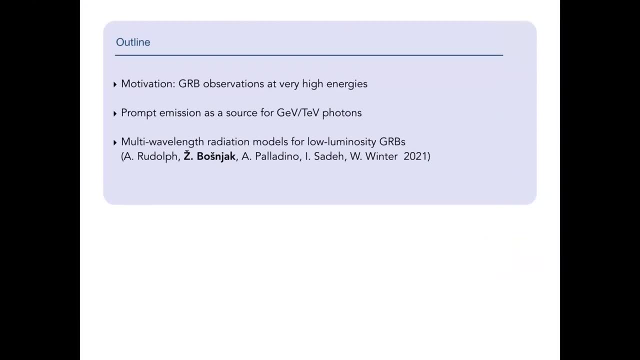 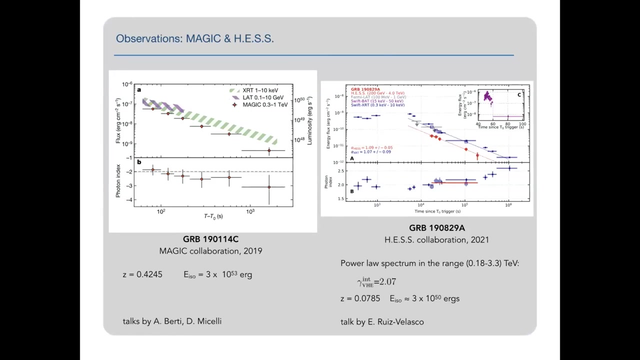 Then I will discuss radiative models for prompt emission, And finally I will present the multivalent radiation models for low-luminosity gamma-reverse in framework of the internal shock model. So radiation at high energy is expected, for example, from electrons accelerated by internal. 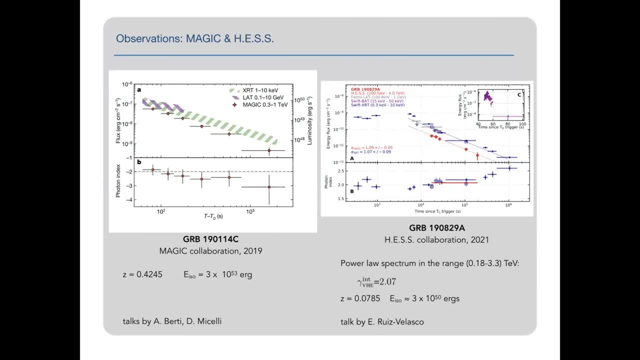 and external shocks via Fermi mechanism to a parallel energy distribution leading to electron synchrotron radiation which, in the observer frame, extends beyond 100 MeV. Inverse quantum scatterings of such synchrotron photons leads to GeV to TeV spectral components. 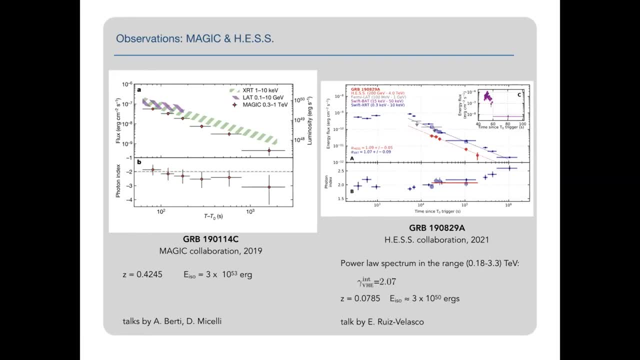 While the emission can extend to TeV energies, such photons are likely to be degraded to lower energies by pair production, either in the source itself or in the intervening intergalactic medium. unless the GRB is at very low, redshift Photons of GeV and TeV energies were observed. 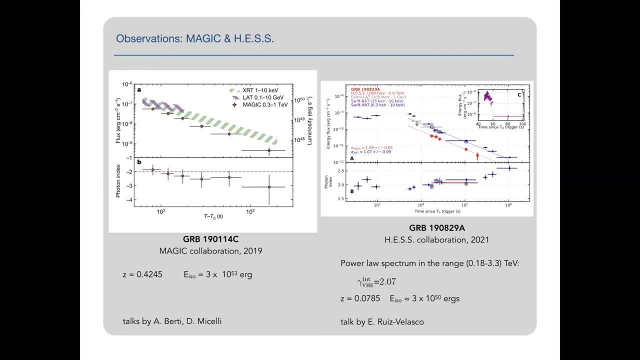 with the Fermi, MAGIC and HESS experiments. The MAGIC collaboration detected photons in the TeV range from GRB 1901-14c, and the multivalent observations obtained by the MAGIC collaboration have formally established for the first time the existence of the SST component. 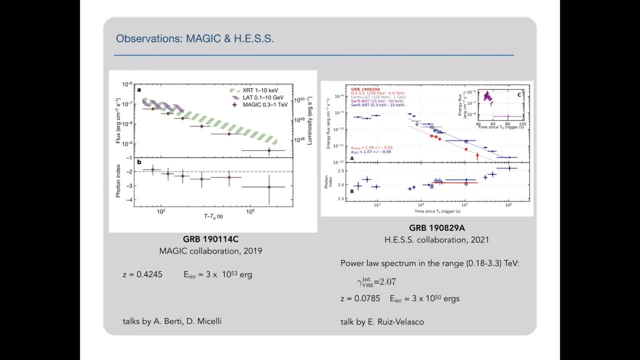 in a GRB afterworld. HESS collaboration reported recently the detection of very high-energy gamma rays from the afterglow of GRB 1908-29a. Synchrotron components describing the spectrum of this event would need to extend more than three orders. 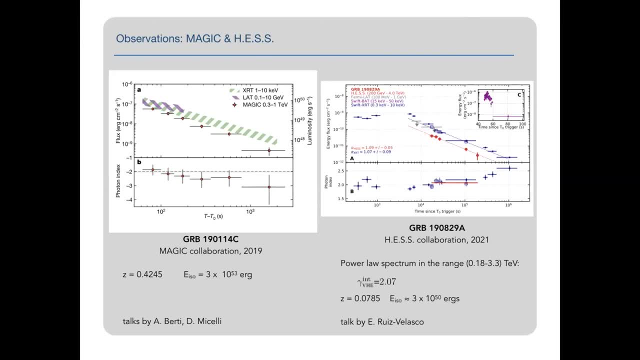 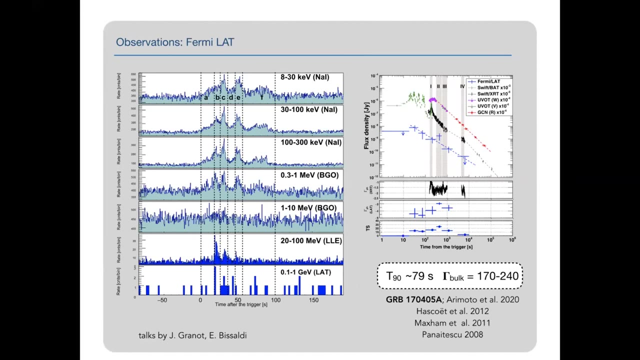 of magnitude beyond the synchrotron limiting energy. This would require an unknown high-efficiency process to accelerate electrons. An example of GRB observed by Fermi-Latins is the long-term B170405a. It showed gamma-ray emission about 20 MeV delayed. 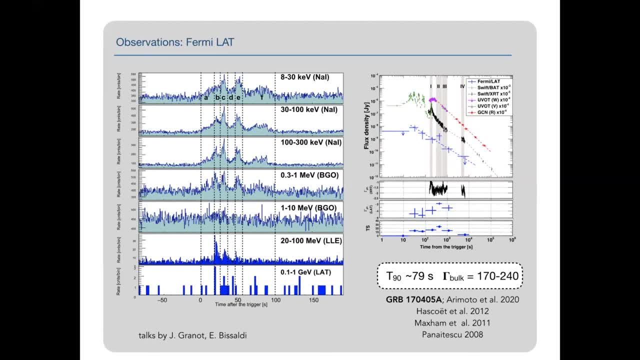 for 20 seconds with respect to the emission below 1 MeV, after which temporarily extended emission lasting for about 1,000 seconds in the GeV band was detected. In addition, 200 seconds after the prompt emission started, an optical onset was observed by SWIFT. 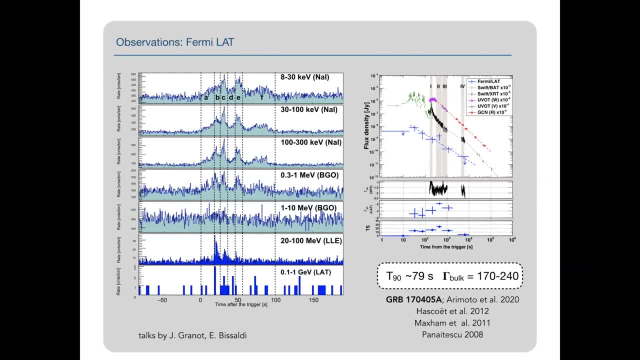 So the multivalent observations revealed different temporal onsets in the optical and GeV bands at 200 seconds and 20 seconds, and the authors suggested that the GeV and optical emissions may have different physical origins. A plausible scenario could be synchrotron emission. 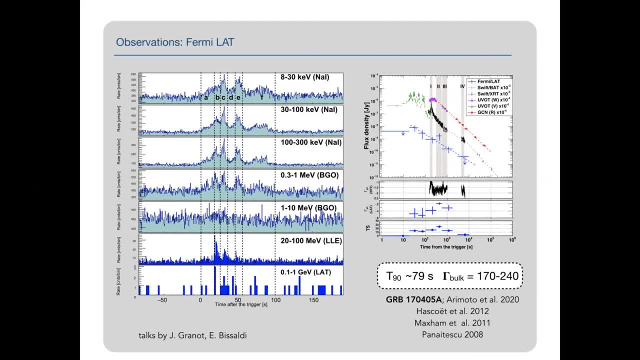 from an internal shock, which can naturally explain temporal variability in the GeV band. The delayed onset can be interpreted as strong temporal dependence of the pair production opacity, which can also be longer than the variability timescale. So this was considered in the paper by Askoet et al in 2012.. 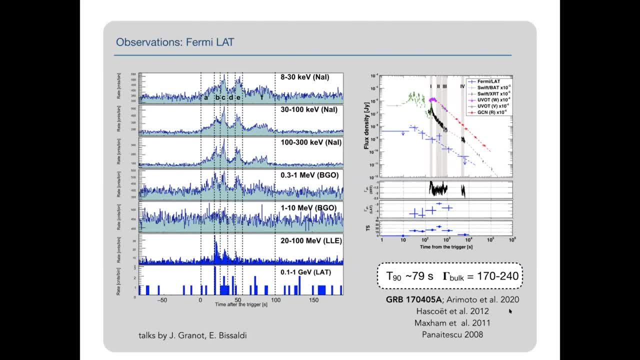 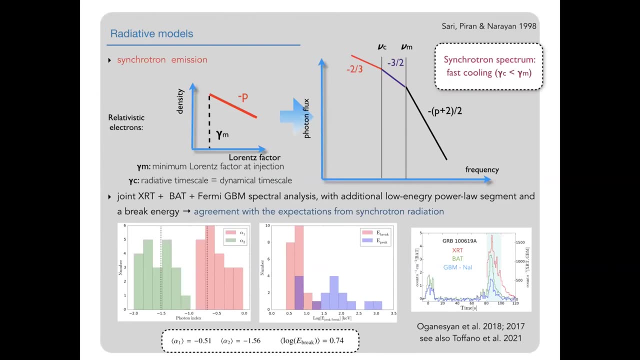 The preference of an internal shock scenario over other models was suggested also by Maxim et al in 2011 to explain the observed behaviors in the GeV band. for other LAT GRBs, Gamma-ray burst non-terminal spectrum has lead to the suggestion that both 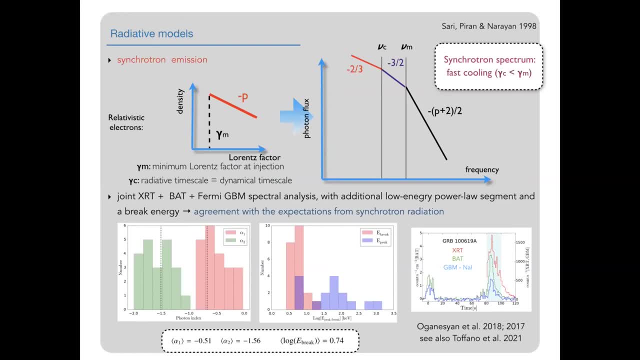 the prompt and the afterglow are produced by synchrotron emission of relativistic electrons. There is a reasonable agreement between the prediction of the synchrotron model and the afterglow observations. However, the observed spectral shape of the prompt emission 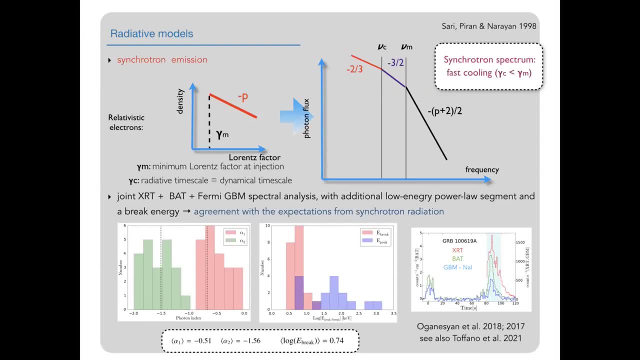 is in disagreement with the synchrotron predictions. Recently, Oganesi et al have analyzed a sample of few tons of GRBs and performed joint spectral analysis of prompt radiation In the sample. Oganesi et al was able to determine the spectral shape of the prompt emission. 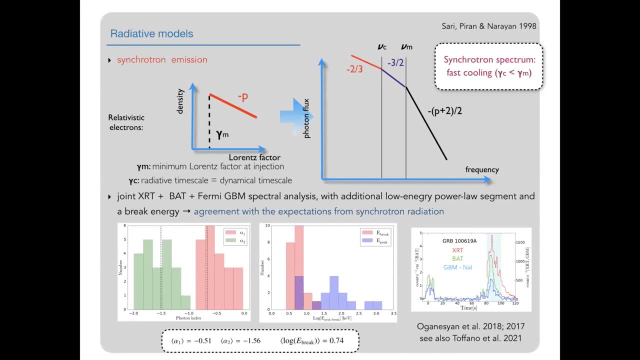 by using a large energy coverage. The inclusion of soft X-ray data revealed a hardening of the spectral shape towards low energies- A break, and then additional parallel segments were added to the fitting function. So the average values of the photon indices below and above the break energy. 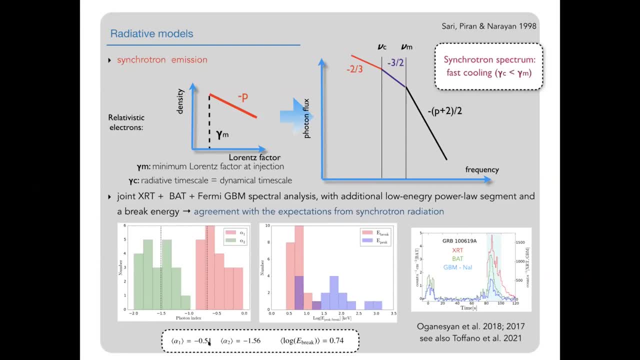 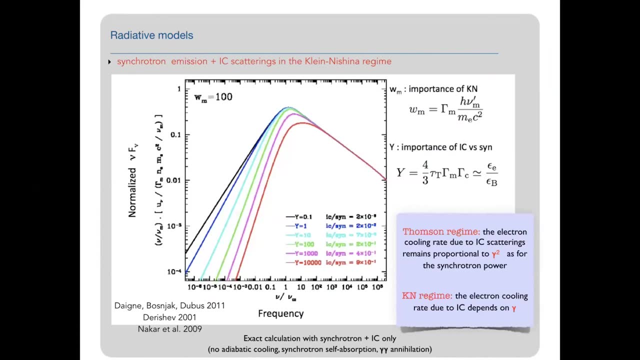 were found to be very close in a scenario where the break energy corresponds to cooling break. From the theoretical point of view, we have shown that inverse Compton scattering in a regime affect the spectral shape of the synchrotron component due to a better efficiency. 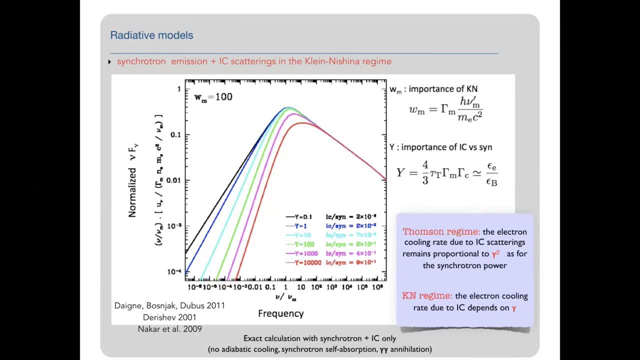 for low frequency photons. This resulted in a steepening of the low energy photon index alpha, and we found that it can approach to minus one. We also identified a regime of marginally fast cooling synchrotron radiation where gamma C is very close to gamma M. 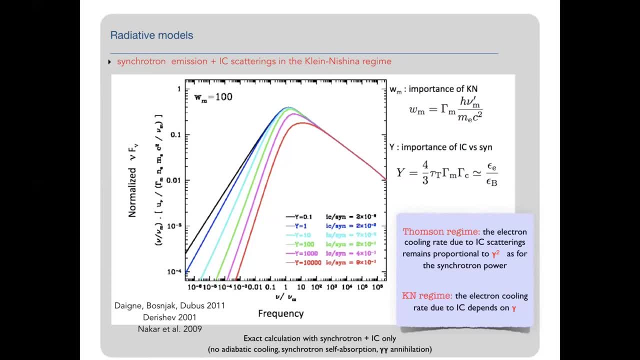 which leads to even steeper slopes, so closer to minus two thirds. I'm showing here the two parameters that define this effect. One is the WN, which tells us how deep in Klein-Ishina regime the scatterings occur, And the other is Y factor. 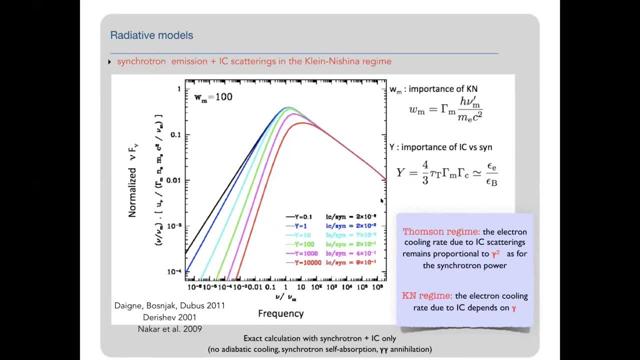 that tells us about the importance of inverse Compton versus synchrotron component. So here I'm showing the spectrum how it changes for value of WN is 100 and for different values of Y. Here I'm showing the spectra in the co-moving frame. 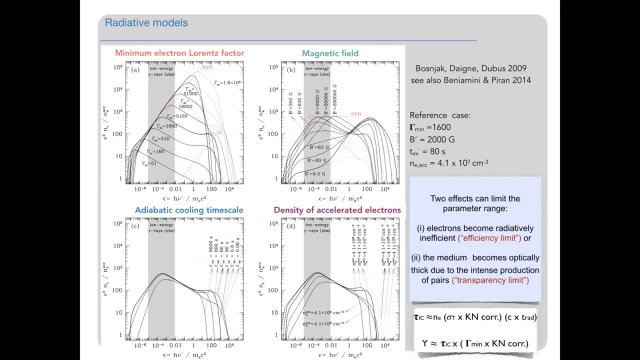 Radiative code included synchrotron emission, inverse Compton scattering, photon-photon annihilation, synchrotron self-absorption and lodiabatic cooling. There are four parameters that shape the spectrum. The first one is the minimum electron Lorentz factor. 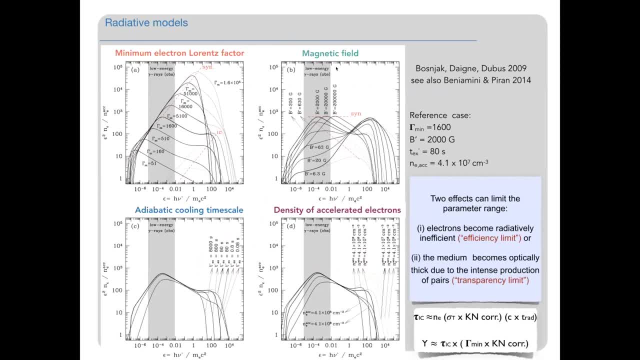 of electron distribution, magnetic field, adiabatic cooling timescale and density of accelerated electrons. So each panel here shows the evolution of the spectrum when one parameter is varied while all other parameters are maintained constant. So a strong inverse Compton component. 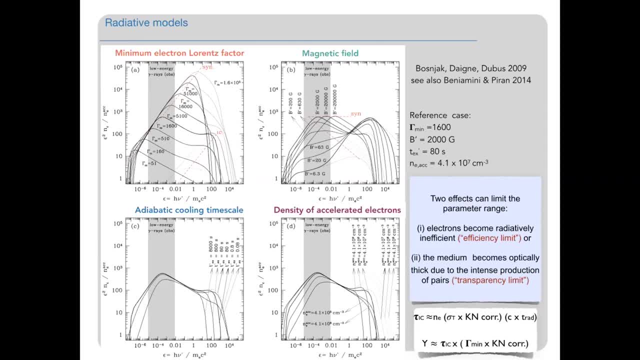 is obtained when relativistic electrons survive long enough for scatterings to occur. So it means that radiative timescale is approaching to expansion timescale and the efficient inverse Compton scattering still occur for low values of gamma, min, low magnetic fields and low Tx. 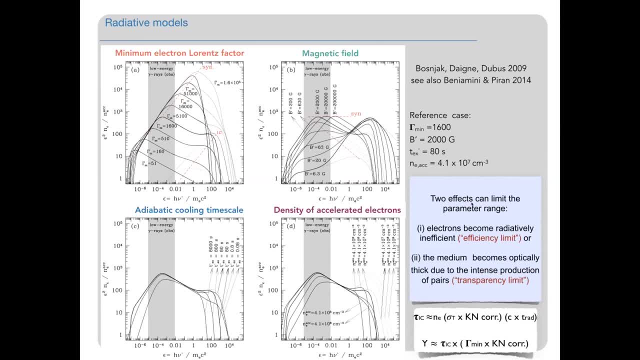 Low density Ne does not favor inverse Compton emission, but the large densities would increase photon density and then also photon-photon annihilation. Inverse Compton components is then strongest for intermediate values of Ne. I would like also to mention a very interesting work. 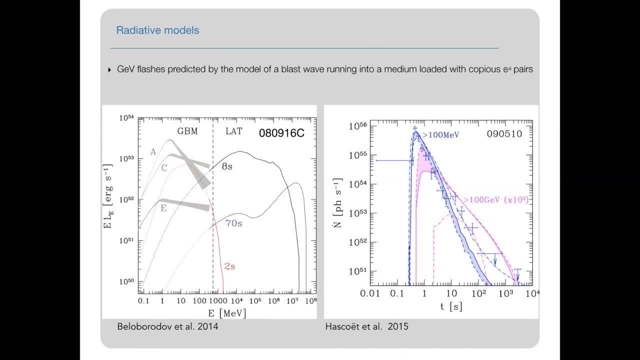 by the laboratory and collaborators, because the observed prompt MeV radiation is taken as input of the simulations. So the mechanism is the following one: The prompt MeV radiation propagates in the external medium ahead of the blast wave and the external medium becomes pair loaded. 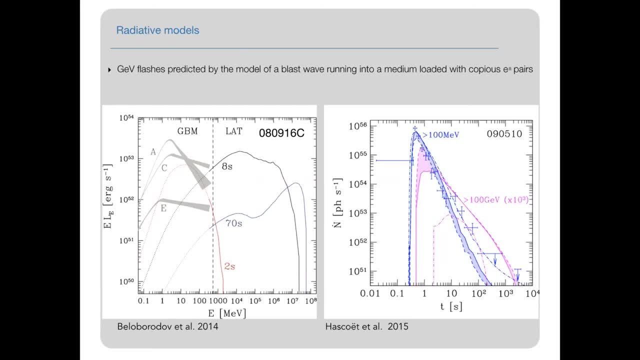 The blast wave has a high Lorentz factor and heats the pair loaded external medium. The medium is cooled behind the shock via inverse Compton and syncretron emission, And when the prompt GRB radiation decouples from the blast wave, the shock-heated plasma is also cooled. 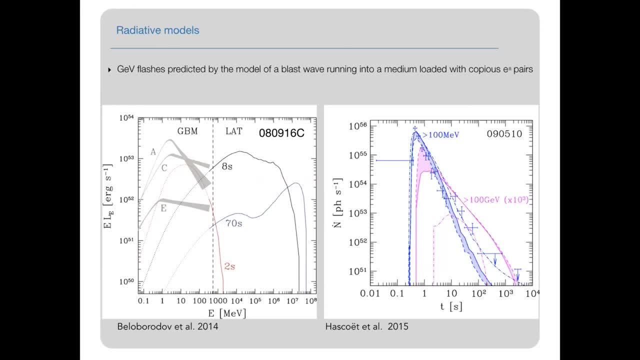 via the slower SSE emission. So the SSE regime occurs in the far tail of the GUI flash. So this plot here shows model light curves and data, for short, GRB 090510.. And this plot shows the spectrum of 080916C in three time windows. 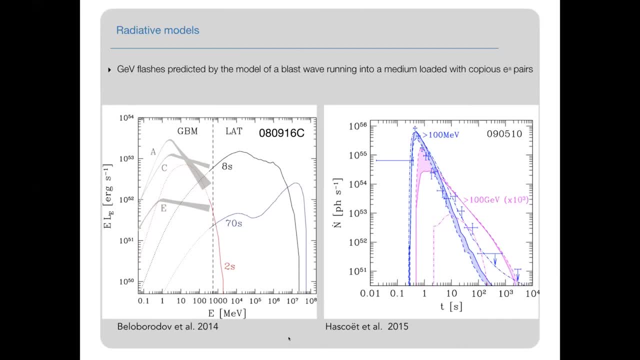 The curves show inverse Compton emission from the blast wave. The prediction of bright emission- about 100 GVs- can be tested with ground-based telescopes like CTA In the internal shock scenario, initial inhomogeneities and the distribution of Lorentz factors. 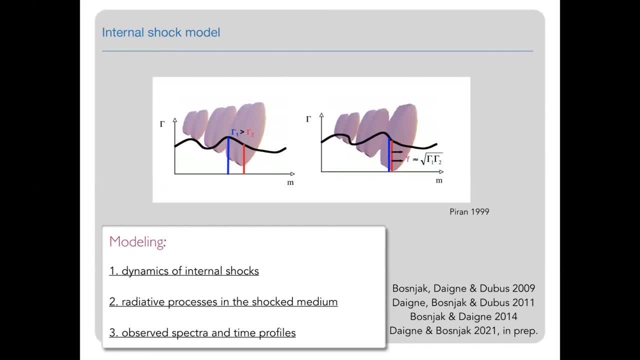 lead to the formation of shock waves that propagate within the relativistic outflow. The shock waves dissipate kinetic energy and accelerate the population of relativistic electrons, which in turn emit syncretron photons. The acceleration of particles in the internal shocks is accompanied. 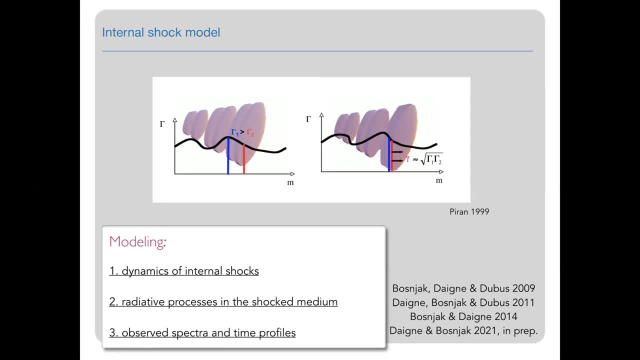 by time-dependent radiative processes which are coupled to each other, And in order to follow the evolution of the emergent spectrum, we combined a model for the dynamics of internal shocks within a relativistic flow with a detailed calculation of the radiative processes occurring. 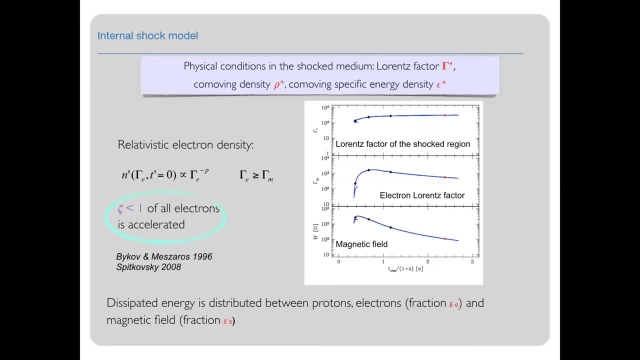 in the shocked medium. So for each collision the physical conditions in the shocked medium are computed And I'm showing here the Lorentz factor of the shocked region, minimum Lorentz factor of the electron distribution and the magnetic field. We have developed a code. 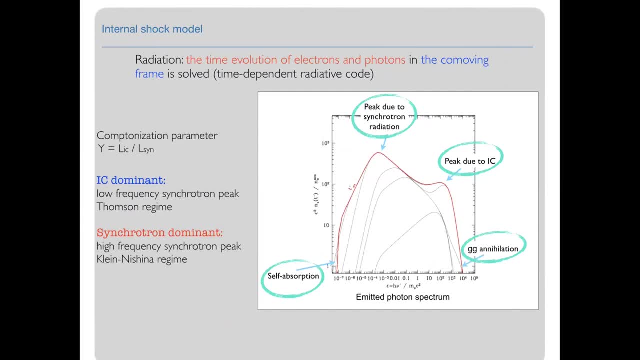 to compute the emission from the shocked material. The calculation is done for all the collisions occurring during the dynamical evolution of the relativistic outflow. The calculation of the emission is done in the co-moving frame and the code follows the time evolution of electron density and the photon density. 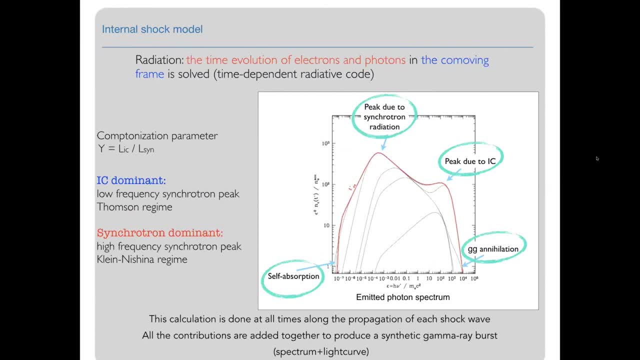 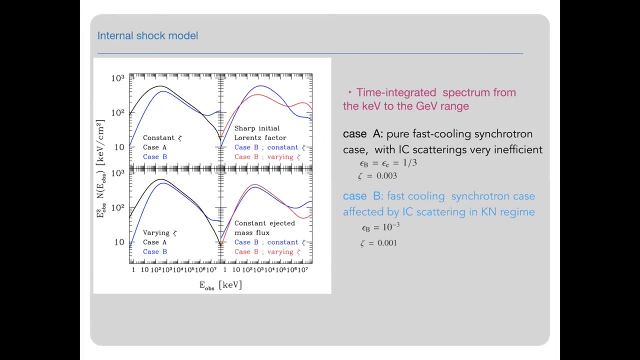 including the processes that are shown here. Here I'm showing the time-integrated spectra from KeV to GeV range that are resulting from the simulations. The inverse Compton component is negligible in case A, while it creates a well-defined additional component at high energy. 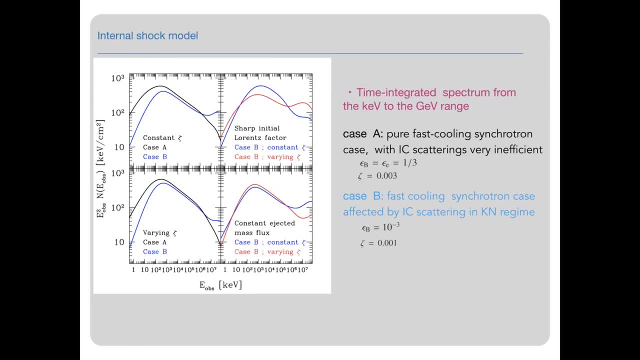 in case B We examine different assumptions on microphysics. So zeta here is the fraction of relativistic electrons that are accelerated to relativistic velocities and on dynamics such as the initial Lorentz factor shape or the case where the ejected mass flux is constant. 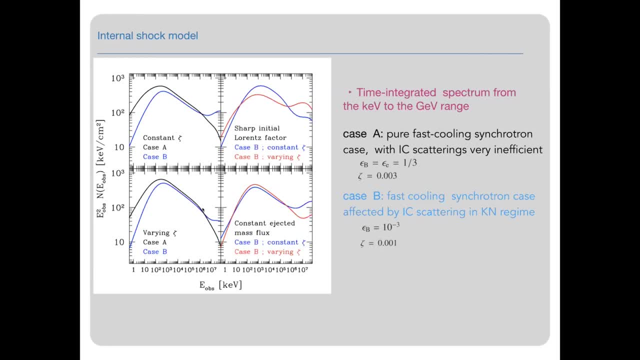 It is interesting to note here that the additional component in the GeV range is very flat in the new FNU spectrum and would probably be fitted by a parallel with the photon index close to minus two, as observed in several lat GeVs. These are the light curves. 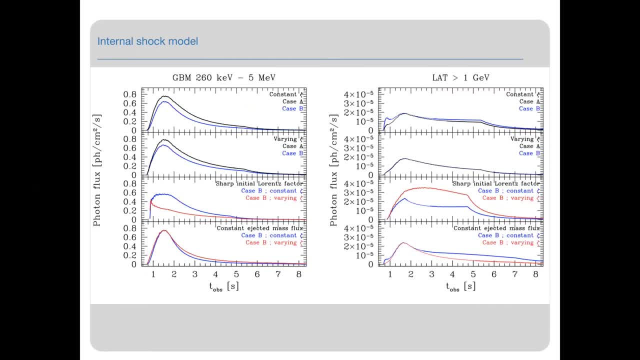 in the soft gamma-ray range and in the high-energy gamma-ray range, plotted for different cases as shown in the previous slide. The assumption for the dynamics have a strong impact on the high-energy emission. The case where the initial distribution of the Lorentz factor 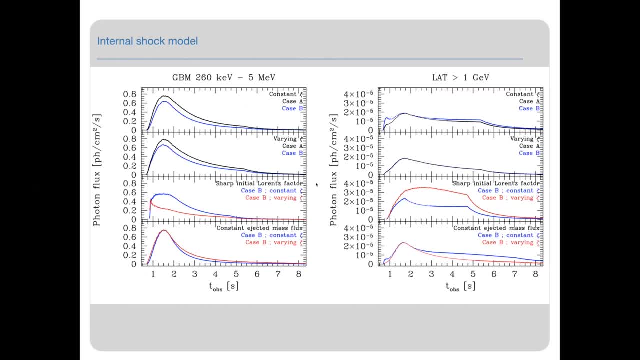 has a sharp transition from minimum to maximum in Lorentz factor is particularly interesting. Here the shocks are immediately violent, so that the inverse quantum emission is suppressed by Klein-Ishina corrections. It is only at late times that inverse quantum emission becomes bright, when more scatterings. 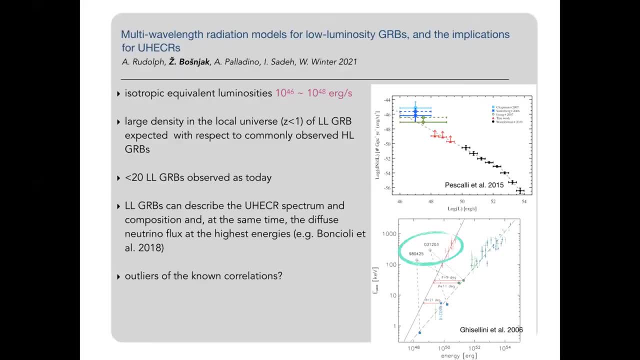 occur in Thomson regime. We studied also the prompt phase of low luminosity gamma-ray burst as potential source of very high energy gamma-rays. This paper is just about to be submitted. Low luminosity gamma-ray burst exhibits substantially lower luminosities and in some cases, 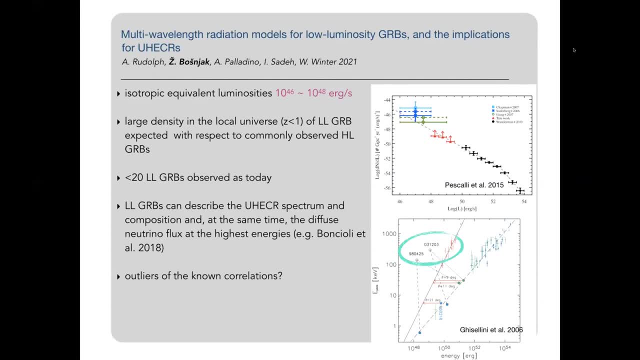 longer durations than commonly observed gamma-ray bursts. Additionally, these events are characterized by relatively low Lorentz factor and lower peak energies Due to their low luminosity, they are mostly detected at low redshins. Only a small number of low luminosity: GRBs. 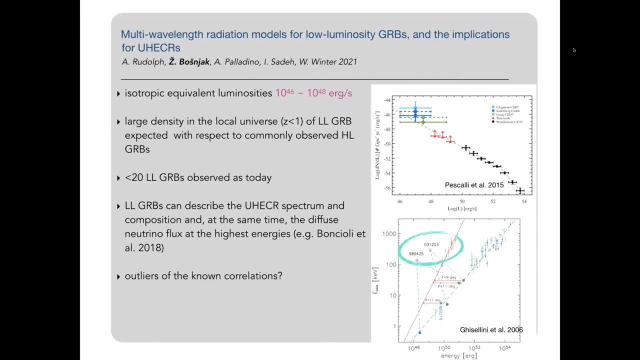 have been detected at low redshins. In this case, only a small number of low luminosity GRBs have been detected at low redshins. In this case, the low luminosity gamma-ray burst and the low luminosity GRBs have been observed to date. 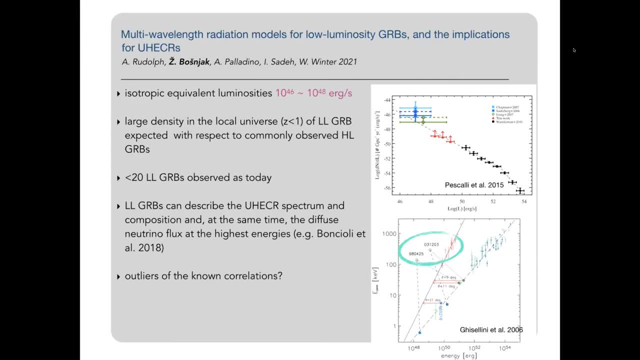 due to the limited sensitivity of currently running X-ray instruments to low EPIC events. Observations by instruments with the ability to detect very faint GRBs showed that the population of low luminosity GRBs may be distinct from high luminosity events and thus dominate. 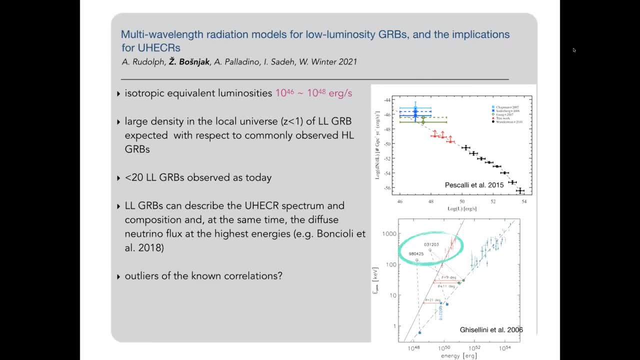 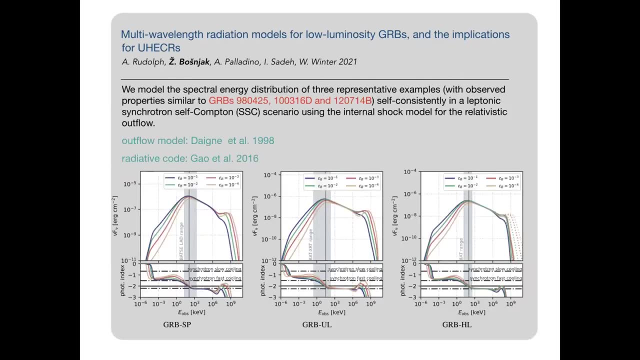 the local GRB population. We modeled the spectral energy distribution of three representatives of low luminosity GRBs at low redshins and at low redshins. In this example, we can see that low luminosity GRBs have been detected at low redshins. 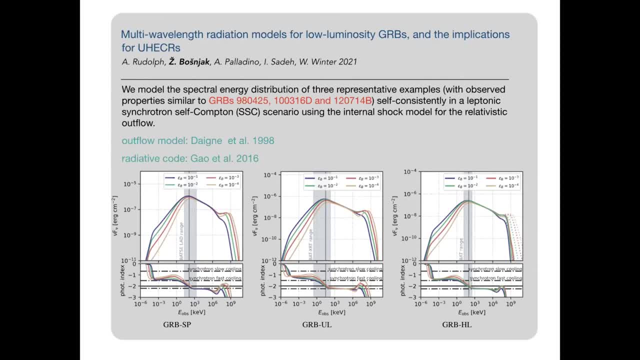 at low redshins and at low redshins with relative resilience and the relative resilience of some of the GRBs as shown here In this example we can observe a number of parallels with the relative strength of the GRBs, A number of 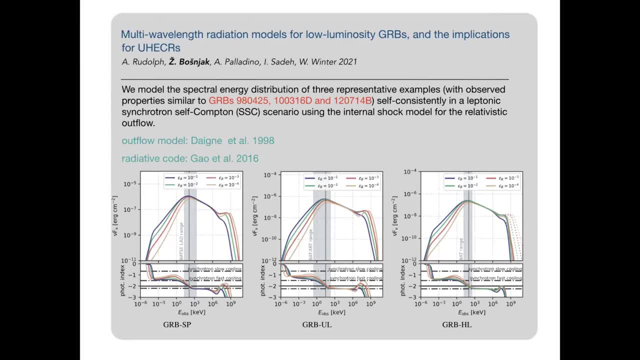 collaborative examples with observed properties similar to GRBs 98,0425,, 1003,16d and 1207,14b. We modeled them in a leptonic SSC scenario using the internal shock model for the relativistic outflow, and we refer. 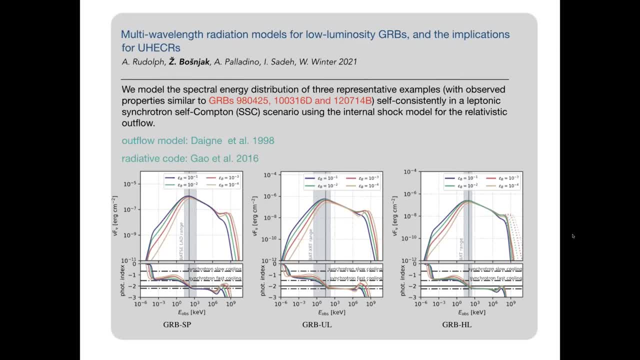 to these examples as GRB single peak, GRB ultra long and GRB comparing to other GRBs To investigate the conditions under which inverse content radiation may lead to potentially observable peak in the GeV and TeV range. we vary the fraction of the 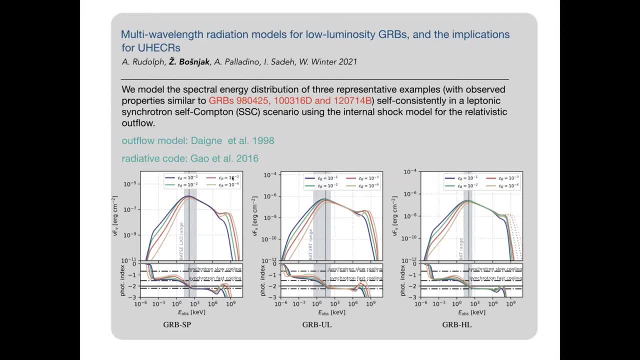 energy budget supplying for the magnetic field. For comparable sub-MeV emission and similar jet properties, the multi-wavelength predictions show a strong dependence on the magnetic field. Weak magnetic fields induce high fluxes in the very high energy regime and low fluxes in the optical, and the opposite. However, very high energy emission might be suppressed by 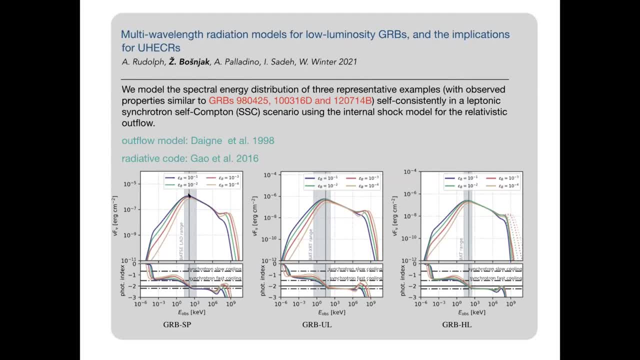 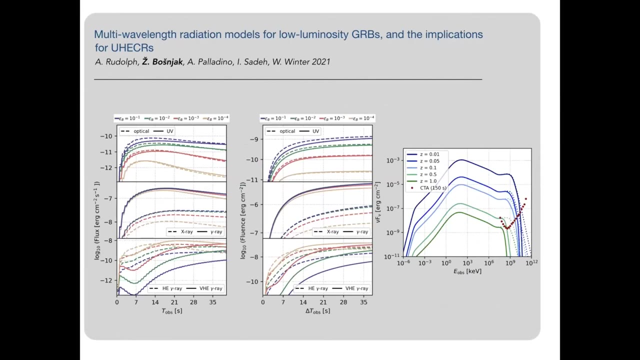 photon-photon absorption or interactions with the extragalactic background lights for redshifts larger than open blind. Here I'm showing the flux and flux lengths as a function of observation duration for different GVs. Also, the predicted observed spectra is shown for high luminosity gamma-ray bursts placed at 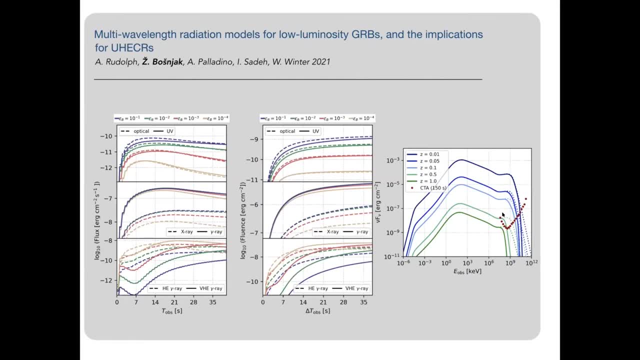 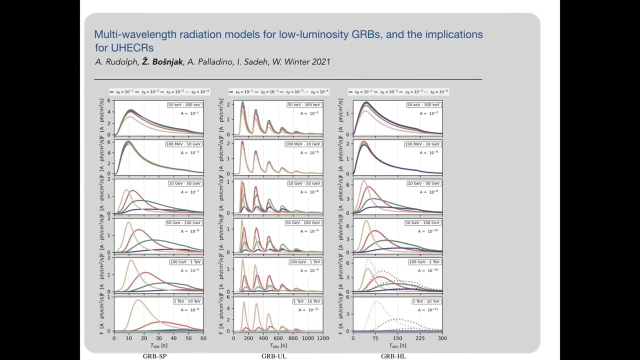 different redshifts. Dotted lines represent the spectra with EBL absorption and the red markers show the minimal fluence nominally detectable by CTA for an observation duration of 150 seconds. These balls show the light curves for different high-energy regimes. We show the results for different choices of Epsilon-b. 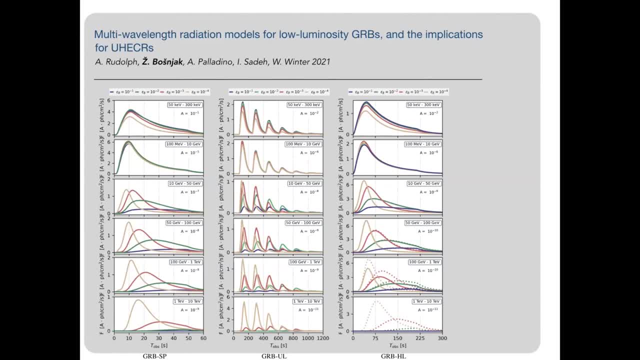 It is interesting to note that high-energy emission shows a delayed onset with increasing Epsilon-b in all scenarios. This is an example of how the different observed light curves may be used to constrain the physical process. The early signal in a single peak light curve. 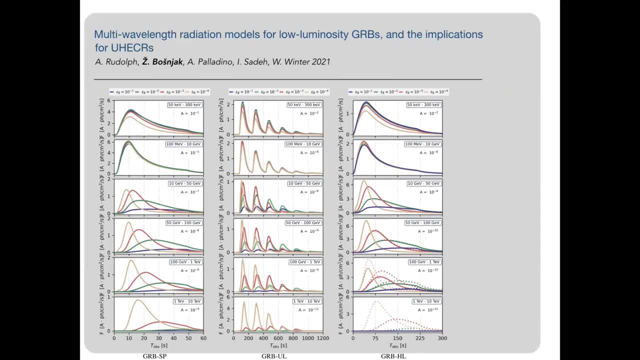 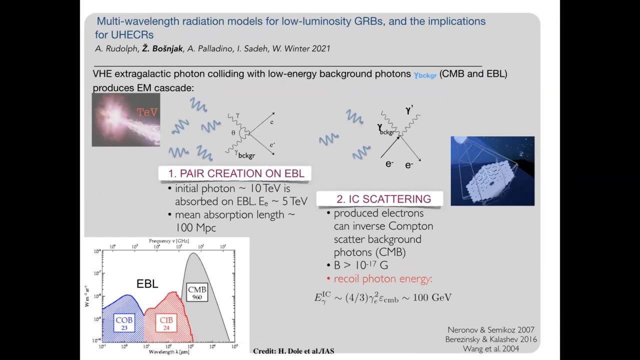 is related to collisions close to the source and these are subject to strong photon-photon absorption- expresses the high energy component- This is the last subject I would like to address. So the photon-photon interactions between primary gamma rays from the gamma ray burst and low. 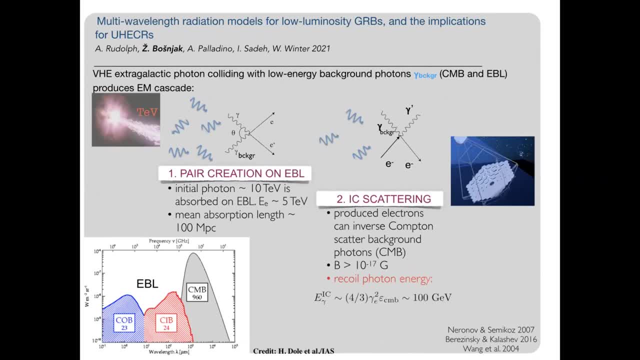 energy photons. Five minutes, Angelica, to the end, Thank you. And so the photon-photon interactions between primary gamma rays from the GRB and low energy photons of the EBL generate electron-positron pairs far away from the source. 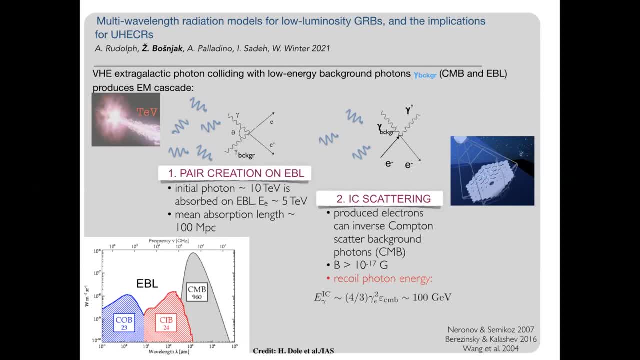 The pairs can be deflected by weak intergalactic magnetic fields for a short period before giving rise to secondary GUI and TEV components by upscattering ambient CMB photons. They would arrive with a characteristic time delay relative to the primary emission. that depends on the properties of the intergalactic magnetic fields. 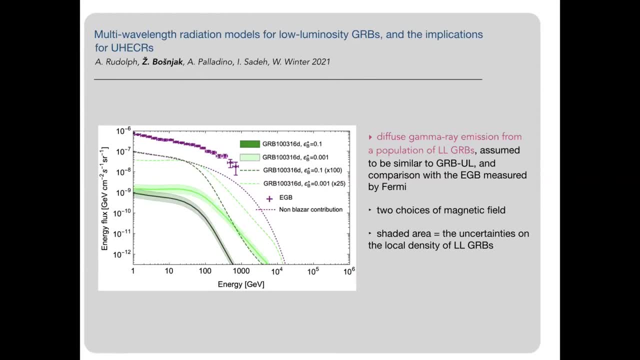 We have Calculated the contribution to the extragalactic diffuse gamma ray background from low luminosity gamma ray bursts. We show in this figure the expected contribution from a population of low luminosity GRBs If all of them were described by a prototype. 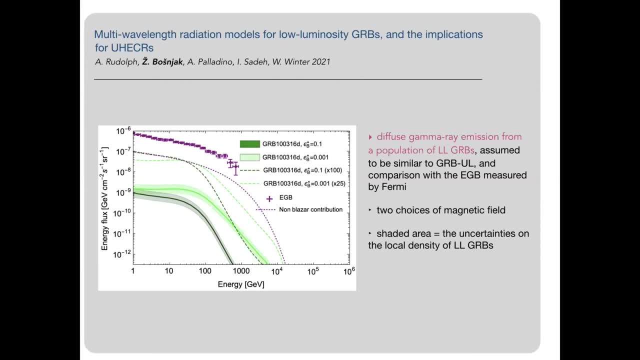 we called ultra-long gamma ray burst And we compare it with the extragalactic gamma ray background measured by Fermi. Note that extragalactic gamma ray background, which again is expected to be driven by active galactic nuclei, And the expected contribution from other source classes. 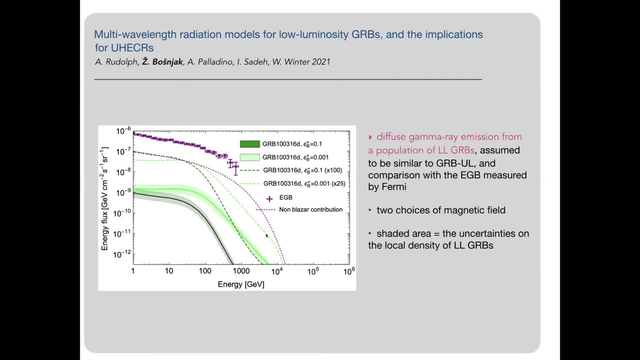 is small. So we show here in the dotted purple curve the 14% of the extragalactic gamma ray background flux. since blazers already provide 86% of contribution, We show this as the possible maximal contribution from low luminosity GRBs to the extragalactic gamma ray. 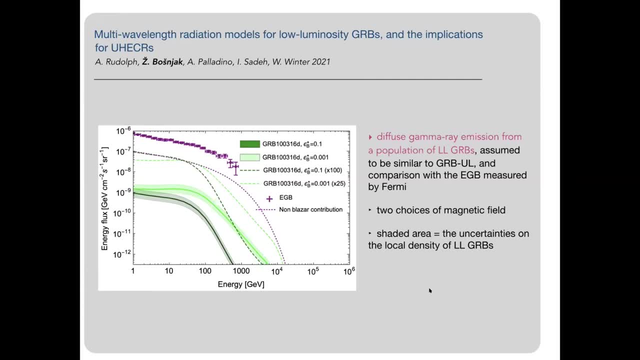 So we can see that the extragalactic gamma ray background we are showing here. so the case is for two choices of magnetic field And also just to show how much this low luminosity GRBs contribute to non-blazer contribution, we multiply this two distributions by factor 125.. 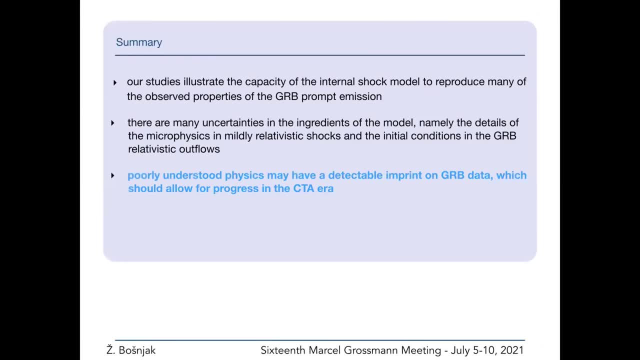 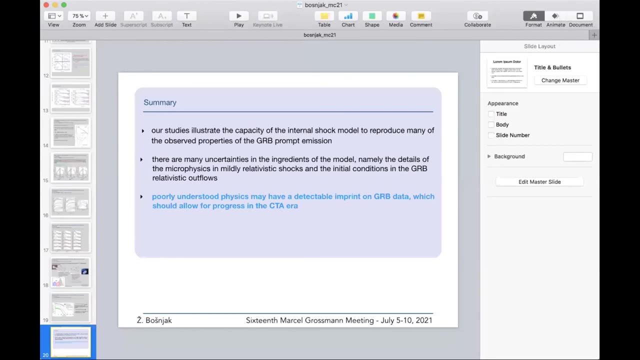 And this is my summary. So thank you, And I'm ready to answer any questions if there are any. OK, Thanks, Jelica. So I see already one question by Yoni, please, And then one by Giovanni, Hi. 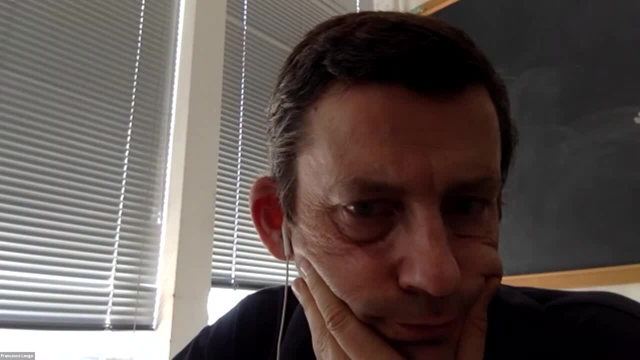 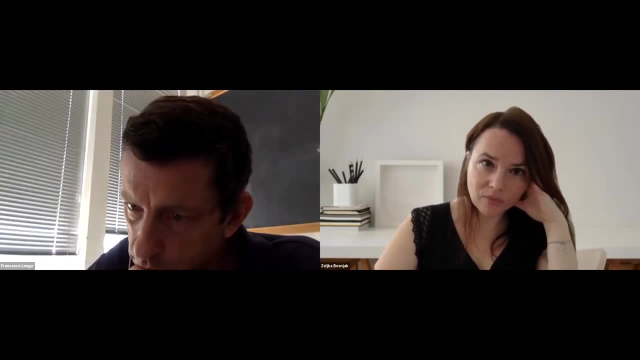 Thank you for the nice talk. You mentioned that you can get the delayed onset of the high energy emission. My question is: is this a matter of tuning the parameters, And could you get, for a different choice of parameters, the opposite trend? Do you really get it naturally? 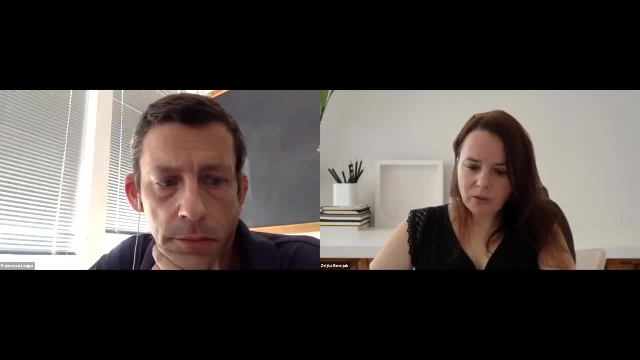 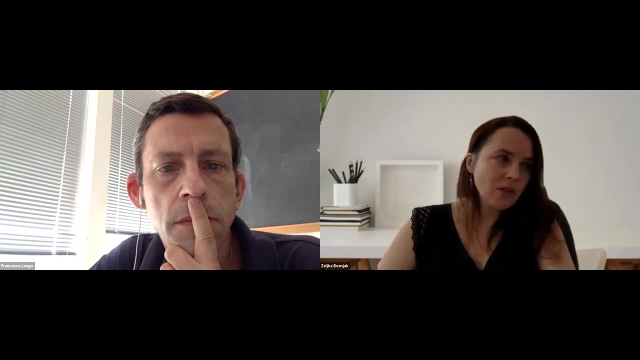 Well, there are two effects. First, we are following the evolution of the relativistic jet. So since we have the evolution of the microphysics parameters, you would expect also the evolution of the dominance of different components. What do you mean? you have 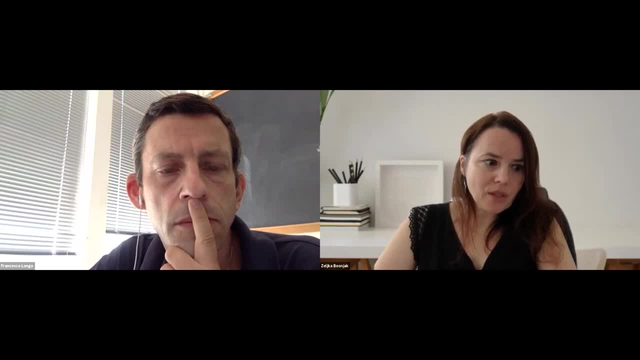 Do you assume them, Or where do you get this evolution from? Well, actually, it is determined, very much so, by the initial assumption. OK, OK, So the first one is the distribution of the Lorentz factors of the relativistic jet. 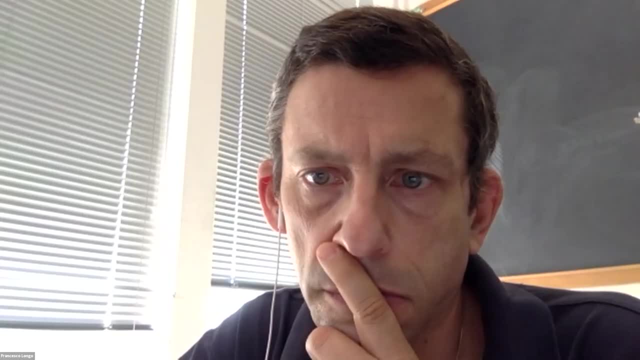 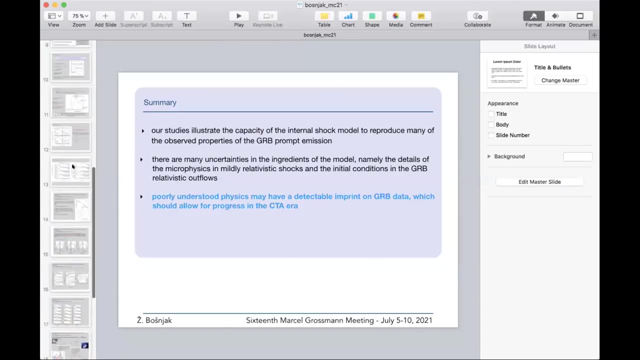 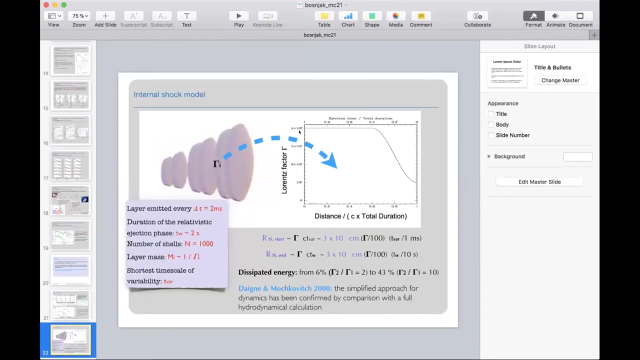 So, for example, let me just show you the again the. This may give the dynamics, but how do you get the microphysics parameters from there? So, for example, the examples that I've shown, we have assumed such distribution of Lorentz factors, which would produce us. 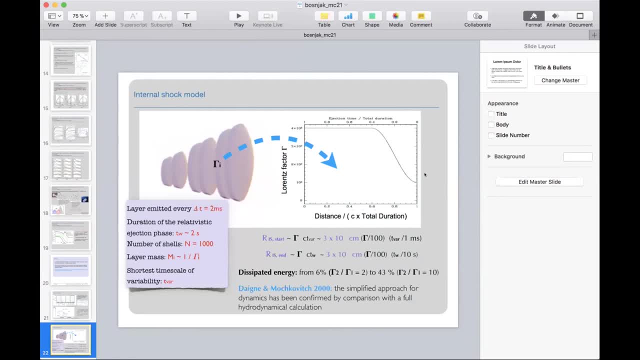 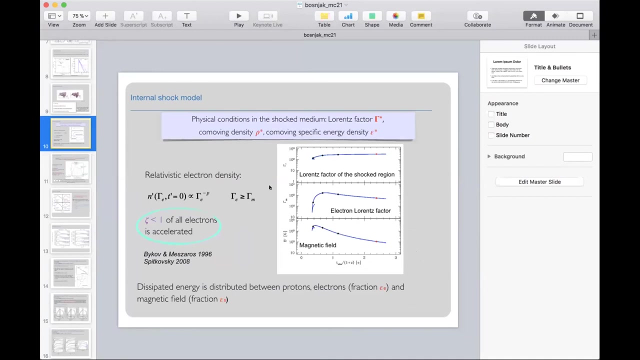 a single peak GRB whose light curve has initially fast rise and then exponential decay, And then also. so this distribution is going to determine how this evolution of physical conditions in the shocked medium is evolving. So there are the assumptions on dynamics and the assumption on microphysics that finally determine. 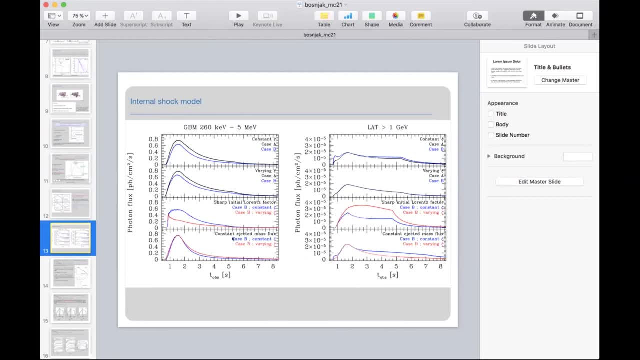 what you're going to see in the light curve or in the spectra, For example. here I'm showing what happens when we assume just like a step function for initial Lorentz factor distribution And you can see that we obtain completely different evolution. 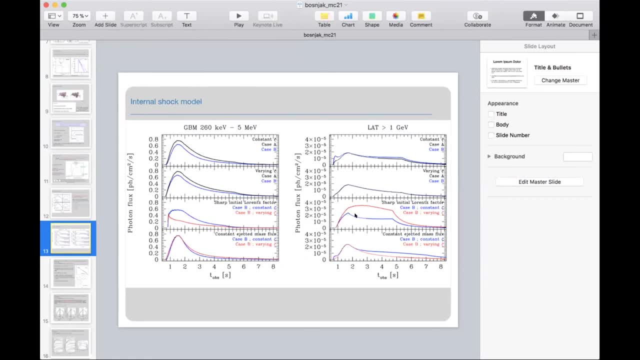 And so you can see the signatures in the light curves. Also. see, you can notice here that there are two cases for constant zeta and varying zeta. Zeta is the microphysics parameters that tells us what is the number, fraction of electrons that are accelerated to relativistic velocities. 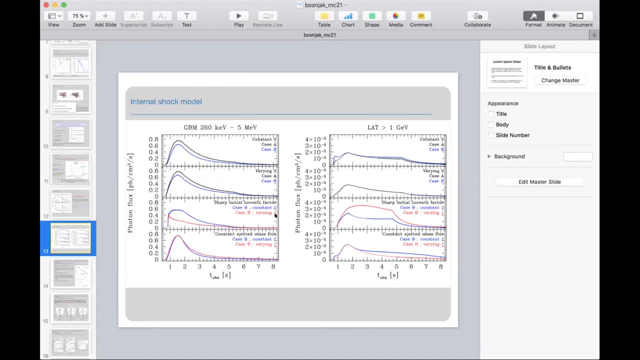 And so varying zeta case means that we put it to be proportional to dissipated energy in the collision. So you see that there are both assumptions on dynamics and microphysics that are going to affect the final shape of the collision. So you see that there are both assumptions on dynamics and microphysics that are going 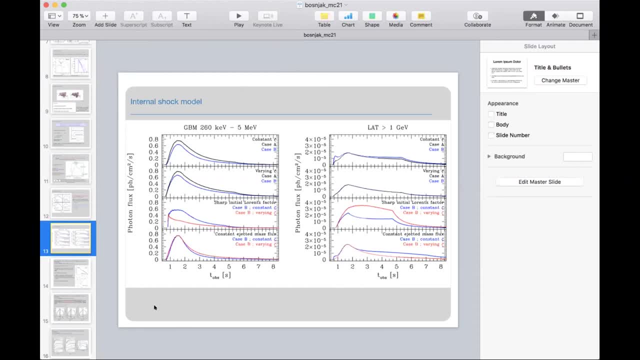 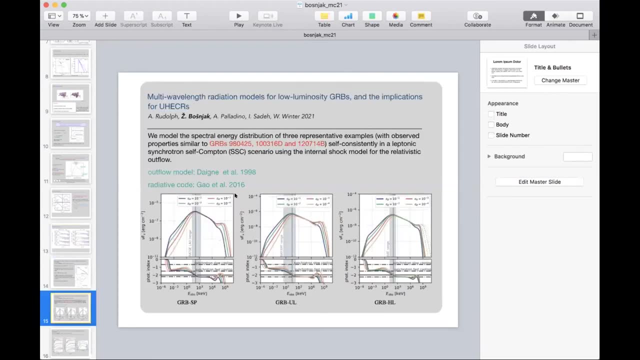 to affect the final shape of the collision. It's gonna depend, you know, on the spectrum and the light curves. Yes, so the difference is also here. for the second work I presented On low luminosity, J embraces, we are using a different radiative code. 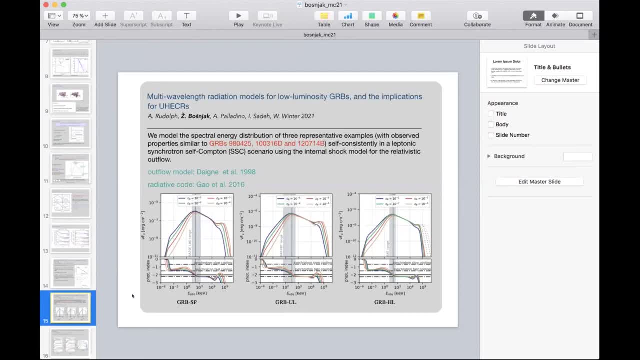 And it is improved with respect to all simulations as it a used to include the effect of the secondaries. Thank you, I see the second question by a person in the audience. Yes, please Again- sorry, giovanni, quite fast because we are mostly out of time. so, please, giovanni. yes, my question is very. 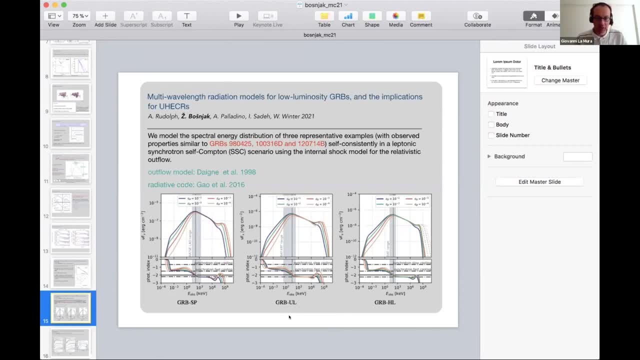 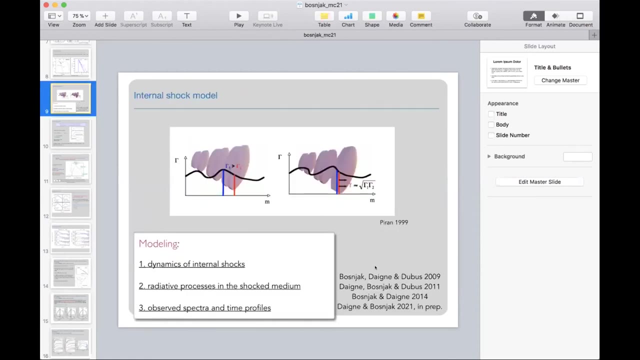 fast and basically it was concerning the code that you use and i wanted just to ask whether it can be available for groups who are interested to model the very high energy emission of gamma rebirth. so these are the papers in which we describe the code and we are currently finishing. 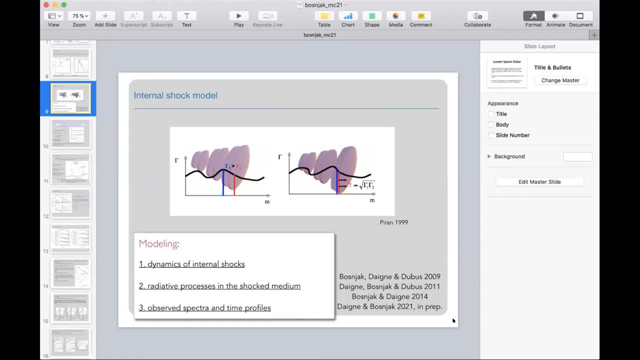 a paper where we are updating some assumptions on microphysics. so the code has never been made publicly available and i don't know. this is something we can think of, think about in the future, certainly, okay. okay, thanks again, angelica, for the very nice, comprehensive presentation about this very nice physics. now we'll we thank the speaker again and 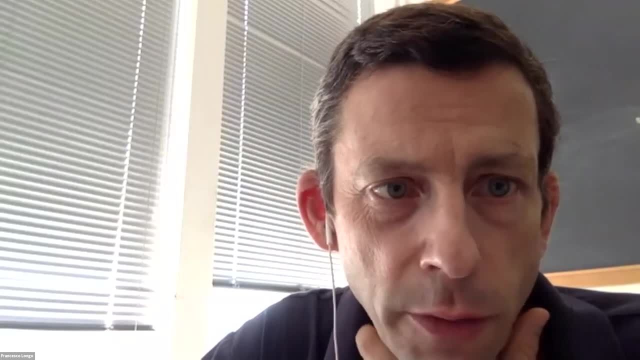 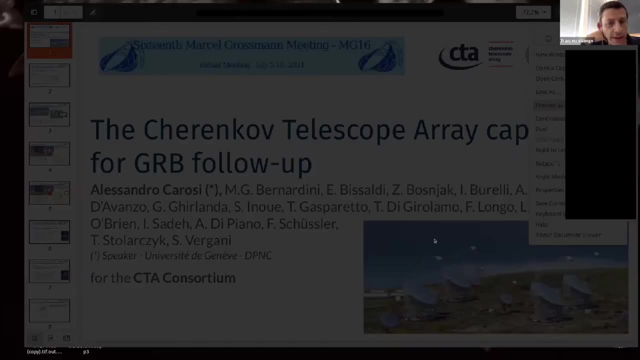 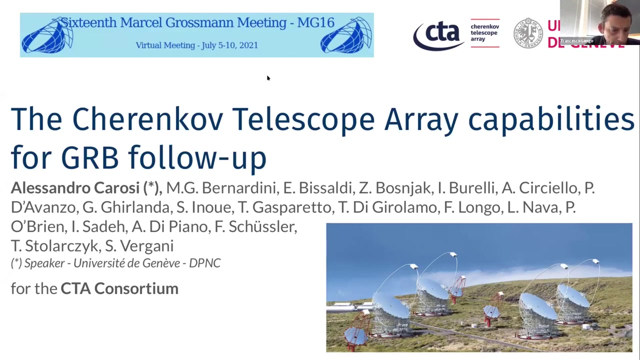 we move to the current and future telescope. we'll complete the presentation of the eict telescope that we started on monday with the presentation of the possibilities of for gamma rebirth, follow-up by cta. so please, alessandro, it is your turn. uh, good morning everyone. can you hear me? can you see my slide? 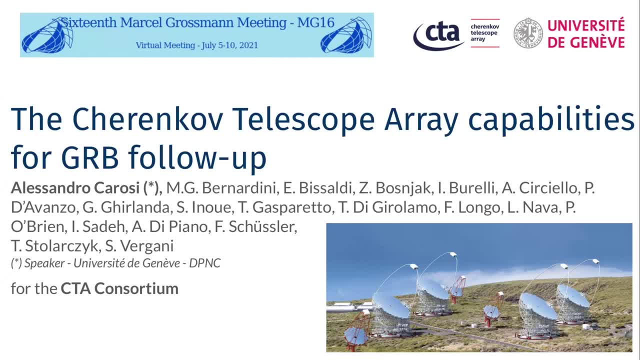 okay, so thanks first of all to the organizer of this session and thanks for inviting me in joining this. uh, this, this meeting i'm going to report about the, the charon telescope array capability in gamma: reverse the follow-up. uh, this presentation or, as you may imagine, is on: 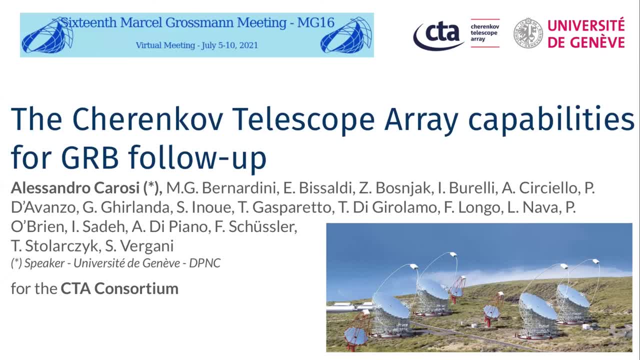 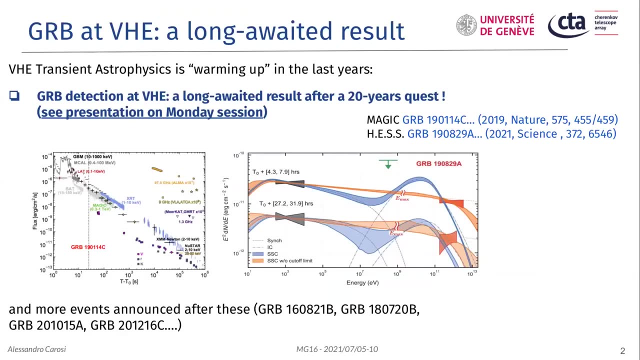 behalf of a larger, our larger team, in particular the gamma reber's team, and belonging to the, to the cta transit working group, and, in particular, the, the people that you, you can see listed in the this table. so, to sum it up, so i have the first, the first slide. uh, the first slide is, uh, going to 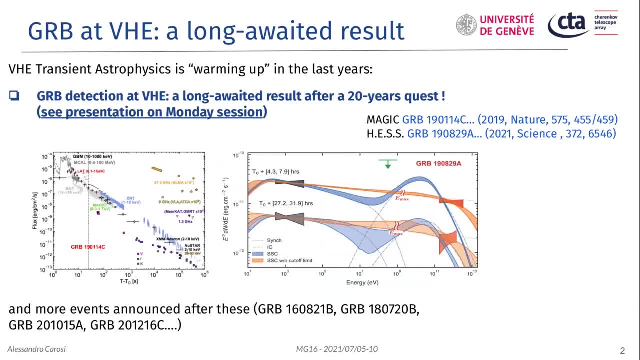 be uh, one of the first slides uh i used here on this, uh, on this in first, uh first slide, uh. so of course, i don't want to spend much time on on this topic. as you definitely already know and, moreover, you already heard about about these hot topics in the in the interesting session of 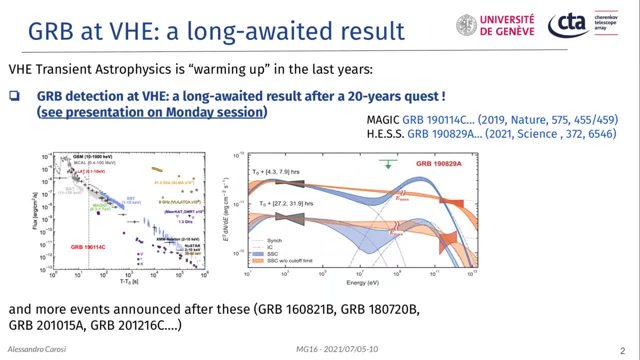 of monday afternoon. just let me, just let me remind that, uh, gamma-ray burst using the current generation of imaging atmospheric Cherenkov telescopes. So you know, of course, that some of these results have been already published, like in the case of 1901-14 scene. 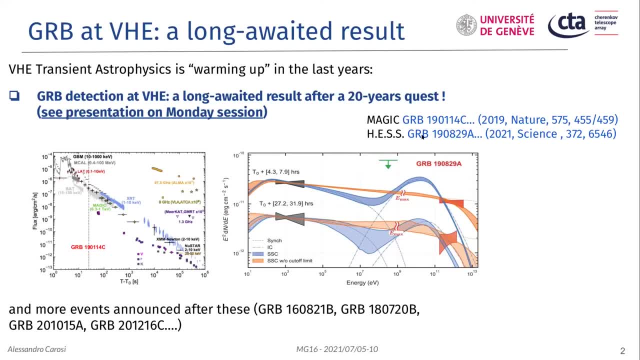 for the GRB detected by MAGIC And in the case of 1908-29,, this GRB detected by one of the GRB detected by ESS, And so you have seen this. the results showed in the presentation of Monday. 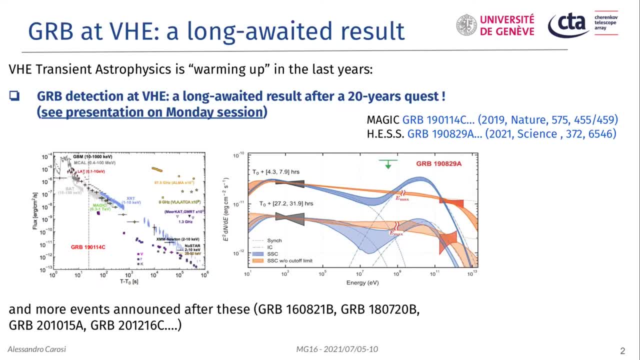 And some other events have been announced to have been detected, but the publication are not yet available. So just to mention some of them: the GRB, the short GRB- 1608-21B, 1807-20B, 2010-15A. 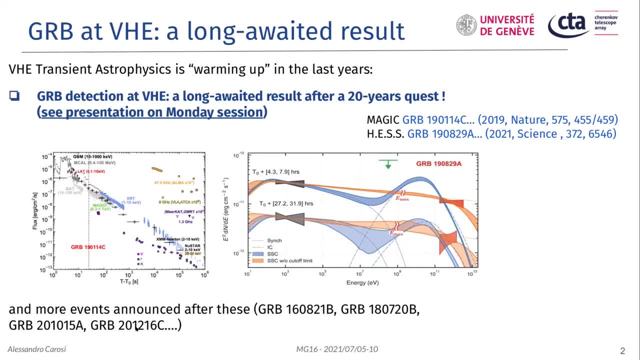 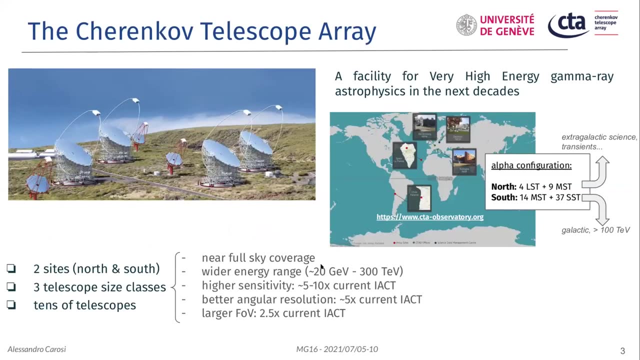 and the most recent, the GRB at the end of the 2020-2012-16C. So these are already the sample of events that have been detected by current generation of Cherenkov telescope. So what about the next generation? 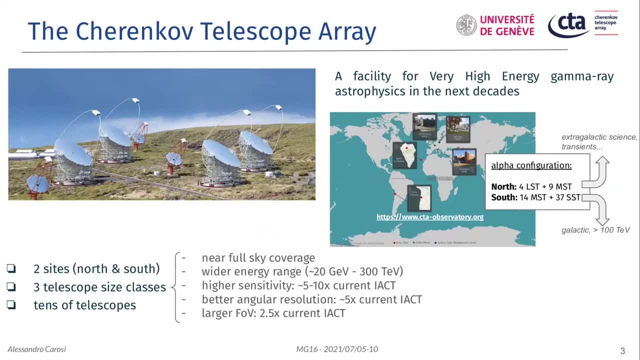 Of course, the next generation, for people that are not familiar with this kind of instrumentation, would be the Cherenkov telescope array, So CTA. indeed, that will represent one of the main infrastructure for the very energy astrophysics in the near future. 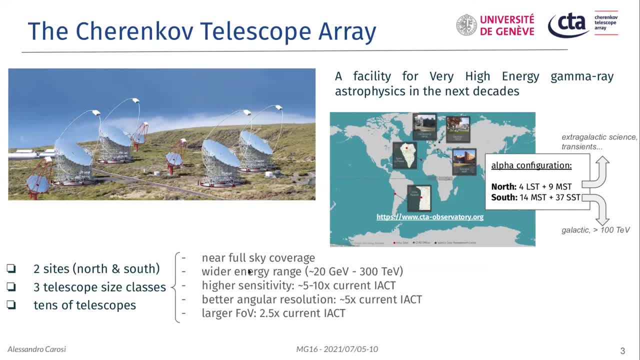 So, in particular, it will be composed. it will be formed by two array of imaging atmospheric Cherenkov telescope, located in the Northern Hemisphere, in the Canary Island of La Palma, and in the Southern Hemisphere, in the Atacama Desert. 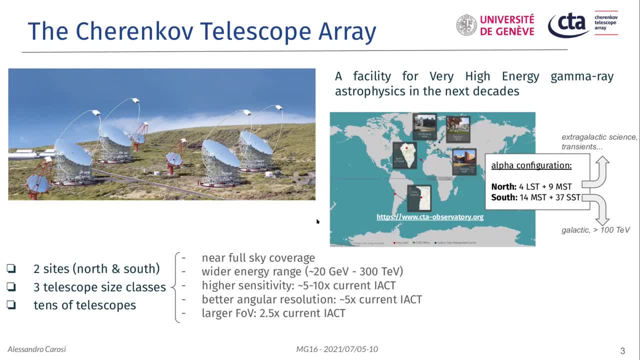 So, within the array, we will have three different type of telescope: the so-called large size telescope with a diameter of 23 meters, the medium-sized telescope with a diameter of 12 meters and a small size telescope that will have an optical diameter. 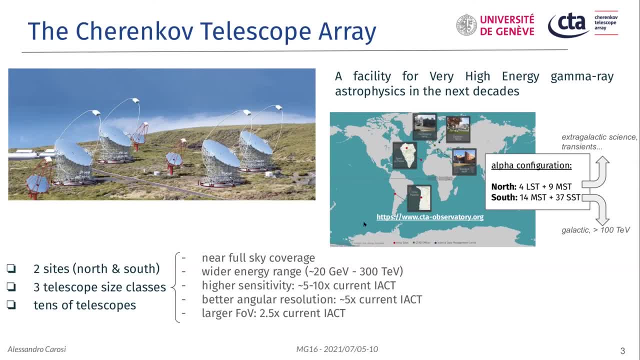 a primary mirror with an optical diameter of 4 meters. So in the first phase, these two array will follow the so-called alpha configuration, that is, a configuration that imply the presence of 4 LST and 9 MST in the north array. 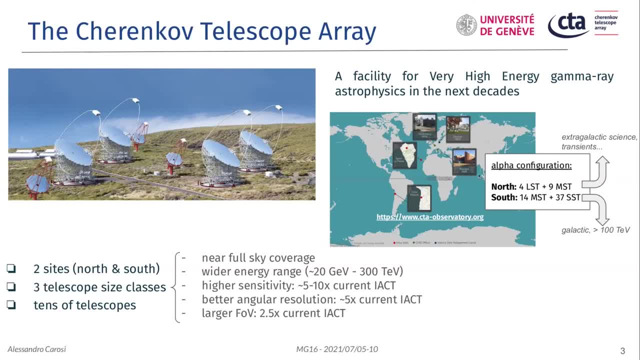 and 14 MST and 37 Professor Ckinesh on- antibiotics, SST in the south. This will allow, of course, an investigation on some kind of complementary science, in the sense that the north array will be mainly dedicated to extragalactic. 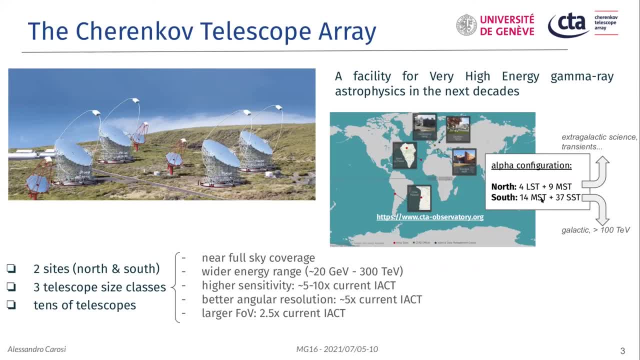 science and to transience follow-up, while the south, at least in this first phase, will be mainly devoted to galactic observation and observation at very high energy, that means above 100 TV. In general, this characteristic of the two array will make CTA of course. 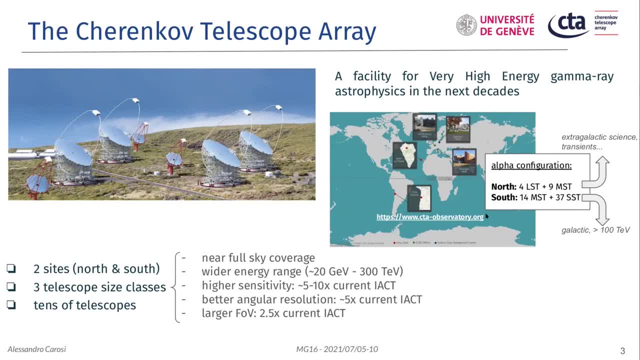 an important step forward with respect to the current generation of ESCT in terms of, in particular, the wider energy range that will cover, roughly speaking, from the 20 GV up to above 300 TV And this wide energy range. it can be covered with a sensitivity. 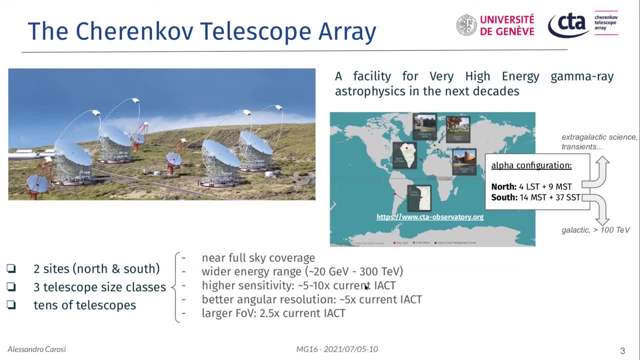 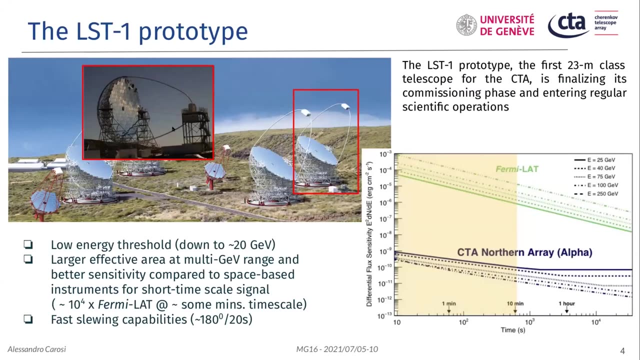 that is from 5 to 10 times better than the current generation of Cherenkov telescope, And on top of that, of course, we have also a better angular resolution and a larger field of view. Let me briefly mention which is the first CTA telescope that will start operation. So 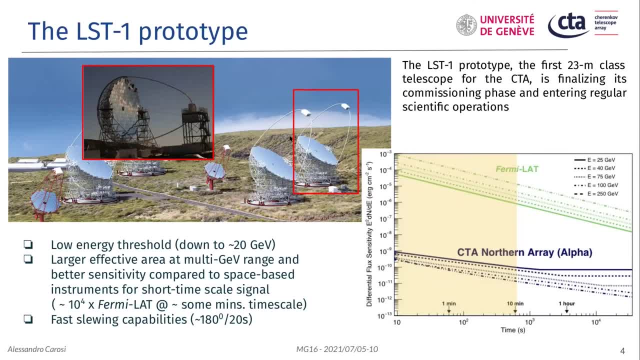 you can see here in this picture that is on the background is a rendering, so it's a computer picture, but in the inner plot it's an actual picture. That is the first one, a picture of the LST-1.. That is the first prototype of the 23 meters class diameter telescope for CTA. And this 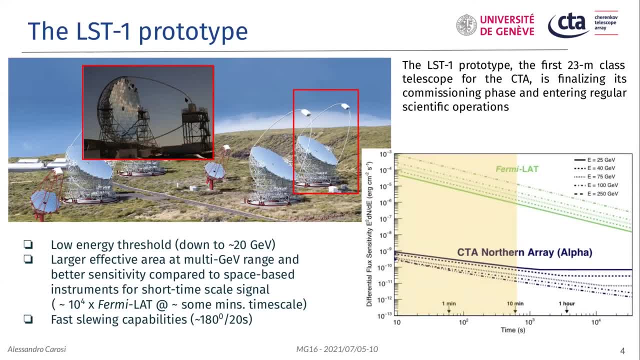 is a telescope that we have in Trans-End Follow-Up and, in particular, gamma ray burst, it's main scientific case because, thanks to its diameter, this telescope will be the one covering the lower energy, the lower energy range between, roughly speaking, 20 GV and 200 GV, And this 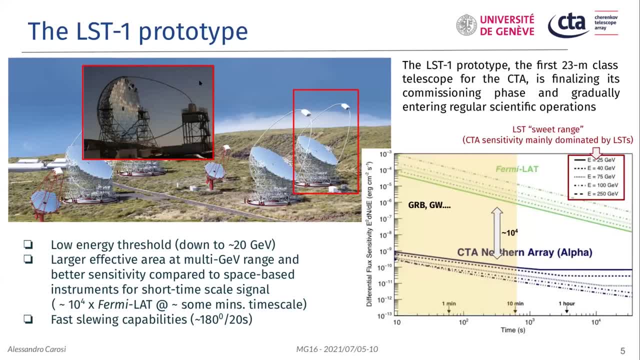 is, of course, particularly important for seusses like gamma ray bursts that are located usually at high redshift, and so their observation might be negatively affected by the EBL absorption. Moreover, within the three telescope classes that I mentioned before, this LST is built to be light. 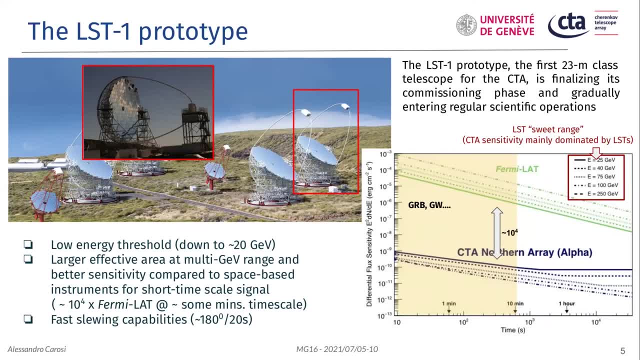 so, even if it's the largest telescope, it weights only around 100 tons, and this will allow a fast repositioning with a speed of the order of 180 degrees in 20 seconds. In general, it is important to remember that this in terms of sensitivity with respect to space-based satellite, as you can. 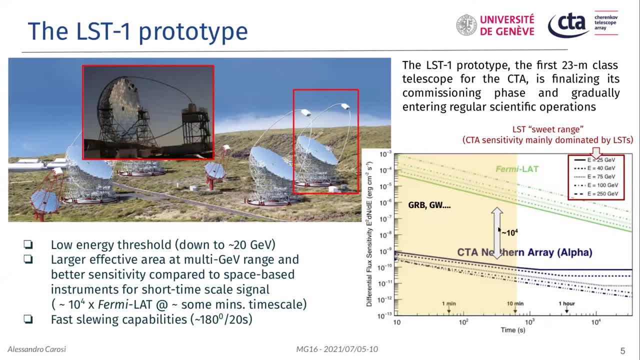 see here in this plot, we will have a sensitivity for a time scale of the order of 10 minutes, that is, of the order of 10 to the 4 times better than space-based satellite in this energy range. So this will this, of course, will. it stands as a very advanced characteristic to perform. 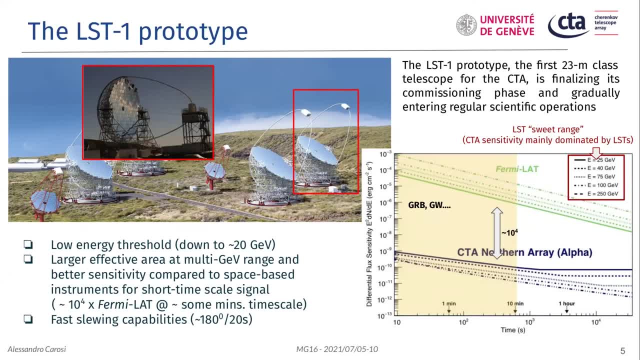 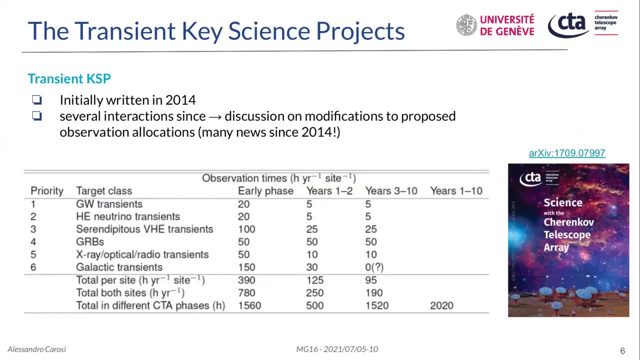 better with respect to satellite is short time scale signal detection. Of course, the price to pay is that this is a ground-based facility with a reduced duty cycle of the order of 10 percent. Within CTA, TransCent represents a key science project. that means CTA, one of the CTA science. 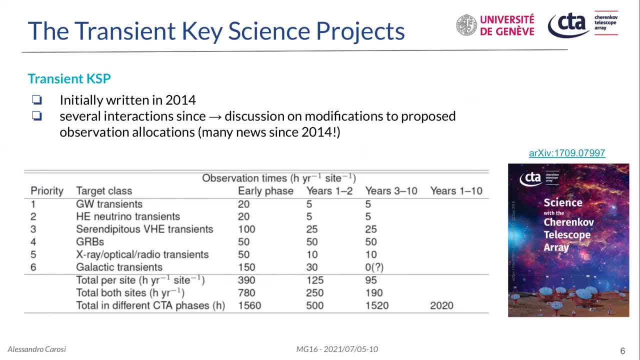 core program and the main goal, of course, is to prepare to the response of CTA to a wide range of multi-wavelength and multi-messenger alerts, including, of course, gamma-ray bursts. So a list of the possible transients that are under investigation. 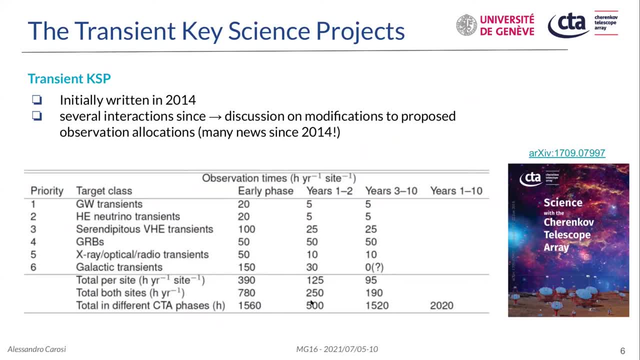 inside the TransCent working group of CTA are presented in this table that is published in this big collaboration paper, Science with the Cherenkov Telescope Array, in which we reported the foreseen and the proposed observation time allocation for each of the GRB. 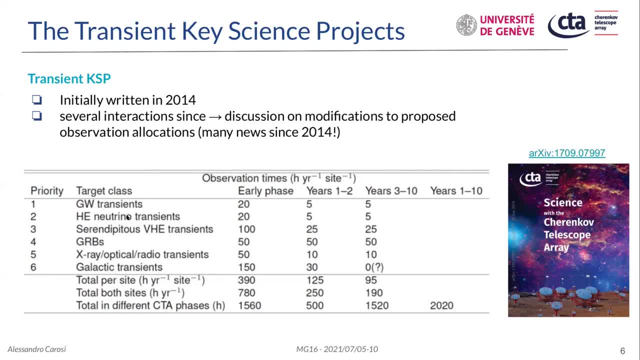 sorry for each of the TransCent that we are thinking as a possible science case for CTA. Of course, this table has been initially written in 2014 and of course, before so the new discovery. so this number has to be revised somehow in the near future, taking care and taking into account that the new discoveries. 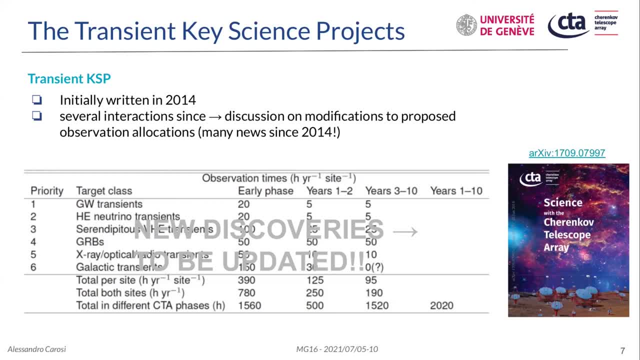 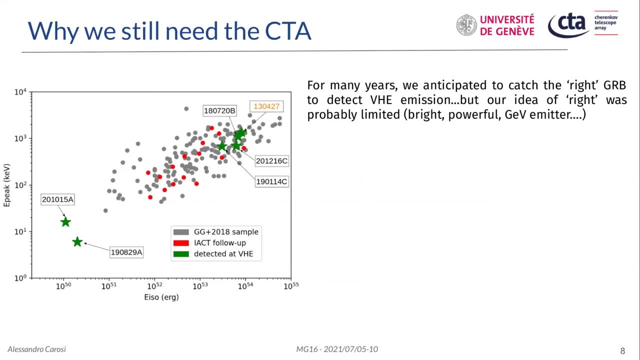 since 20 that we had since 2014.. So actually we can argue if we still need the CTA observation of gamma-ray bursts now that we finally catch the very energy emission. And of course, I don't want to go into the details about the theory that we 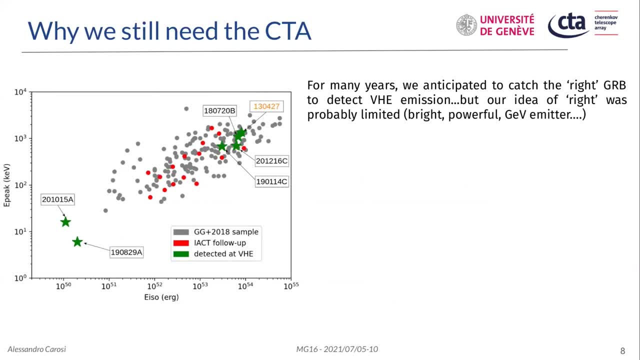 heard from the previous speaker. But of course, as a matter of fact, as it happens sometimes these new observation bring also some new questions And it's now not always easy right now to account all pieces of the puzzle. So in particularly, let me just mention that for many 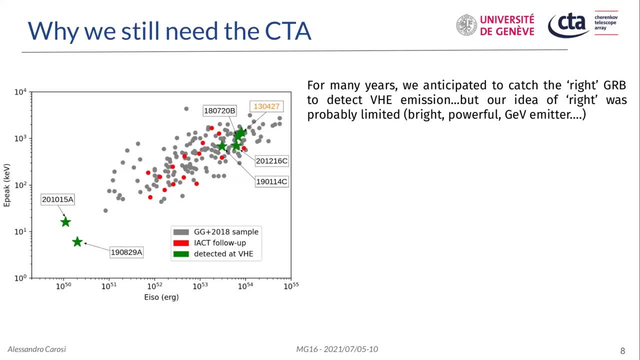 here we anticipated that we were going to have a very, very large number of new observations. So to capture the right GRB to detect very high energy emission component. And this right GRB in our mind was somehow a limited idea in the sense that, of course, in 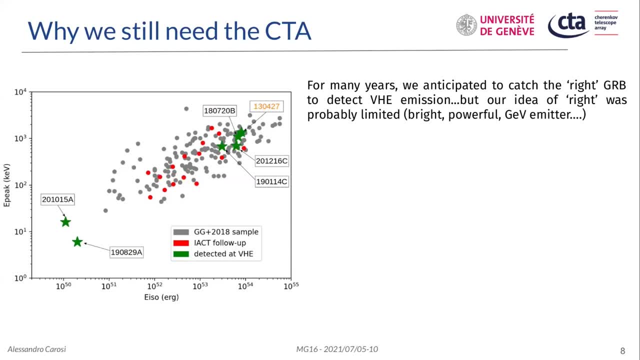 our mind, we wanted to have a bright GRB, a powerful GRB, a GAV emitter and possibly also a low redshift. So this characteristic, of course, makes an ideal candidate for very high energy emission. But, especially with all this data, we thought that this was a very good idea. So we 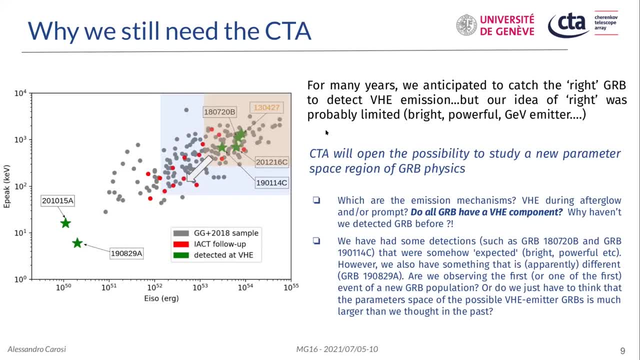 Today, now we know that the things are probably more complicated than what we previously thought, And, in particular, we need CTA to expand, to open the possibility to start to study a new parameter space region for GRB physics, not only the one that you can see here in this plot, that is, the so-called Adamati relation. 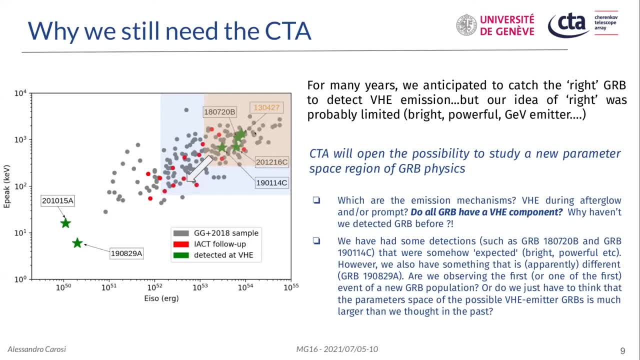 So in the top right of the plot, where we have of course the brightest events that of course we will have the possibility to catch with CTA. But as you can see already from the discovery from S and Magic that we have also some outsider events that stand a little bit out of what we previously thought as an ideal candidate for GRB at very high energy. 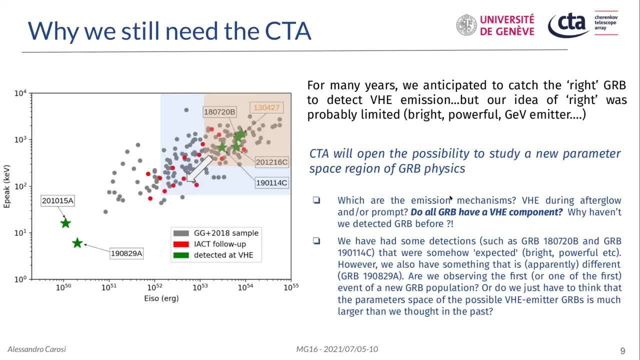 So the question that we want to ask is, of course, if we have, if all the GRB has a very high energy component, and why we haven't detected so far- I mean before at least, And in particular we want to answer to this question- that why we have some detection that somehow are expected. 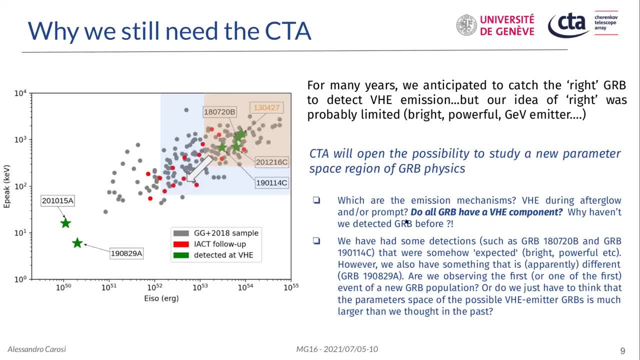 like 1901-14-SIM, for instance, or 1807-20B that are bright, powerful and very luminous GRB. But we also have some very energy detection that are somehow apparently different, Like in the case of 1908-29-28.. 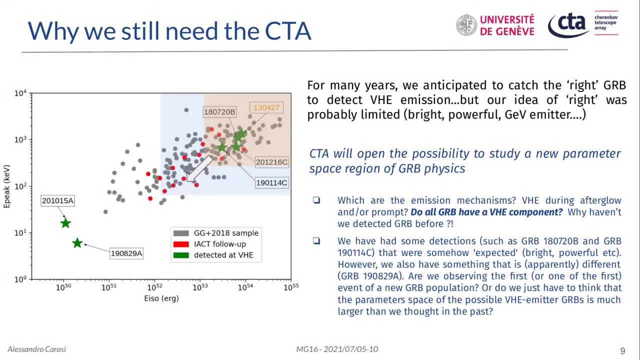 So the question is: we have to think that the parameter space of the possible very energy emitter, GRB, is much larger than we thought in the past, Or there are some different population of gamma-ray bursts that can give a very energy signal. So these are the questions that CTA is intent to answer. 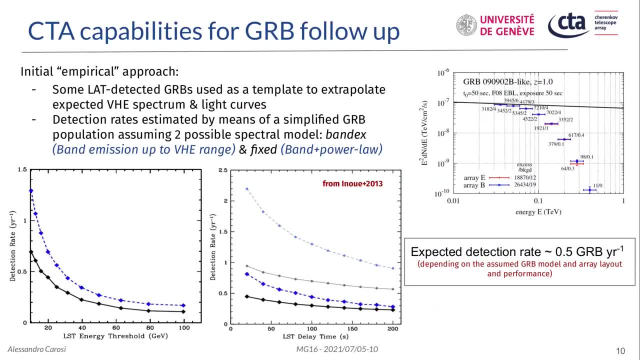 So what we can do with CTA. There was already some some work in 2013 in which in which we use some LUT-detected, we use some kind of empirical approach in which some LUT-detected GRB were used as a kind of a template. 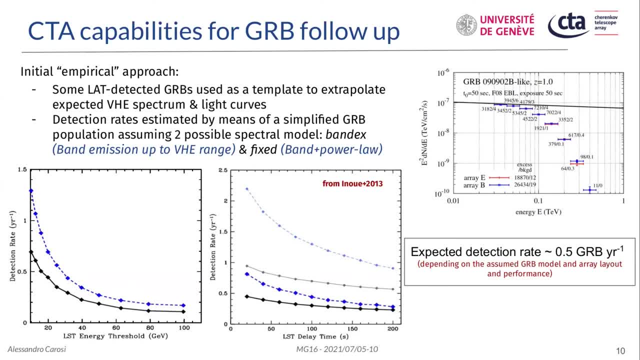 to extrapolate the expected very high energy spectrum and light curve in the very high energy band, So in particularly the detection rates that we estimate in 2013, was following two possible spectral model for this, for this simplified GRB, So the two possibilities of using this so-called BANDEX model. 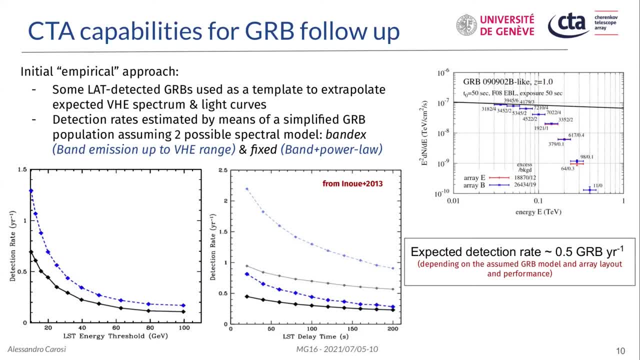 that means an extrapolation of the band emission to the very high energy range, or the so-called fixed spectral model that foreseen, on top of the band function a power log contribution with a power index of two. So in a new FNU plot to something that is relatively flat. 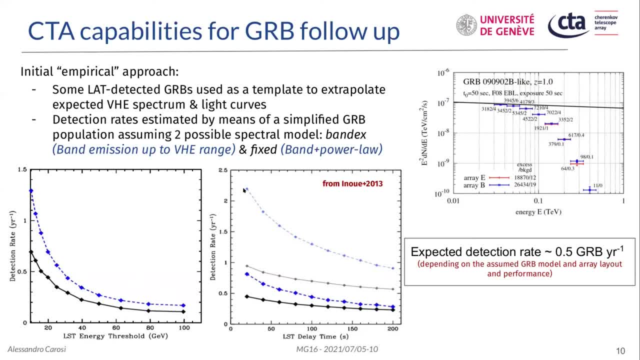 And here you can see the, the, the preliminary plot that we published in in 20, in 20, in 2013,, in which we reported the expected detection rate as a function of one of the of the characteristic that we. 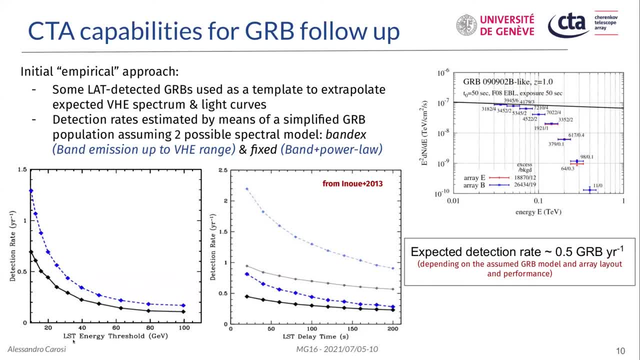 at that time we we were foreseen for, for CTA and particularly for for LST, like in this case, on the on the left plot, the, the energy threshold or the response time to, to, to the. 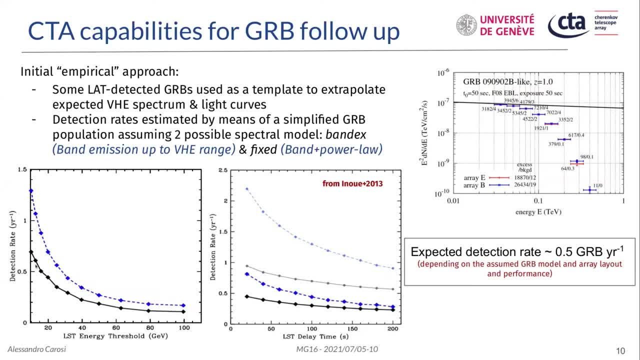 to the trigger for different, for the, for the band emission, that is the black curve, and the fixed scenario, that is somehow more optimistic. for the GRB emission, That is the blue, the blue line. So, depending on the assumed spectral model and the array characteristic, 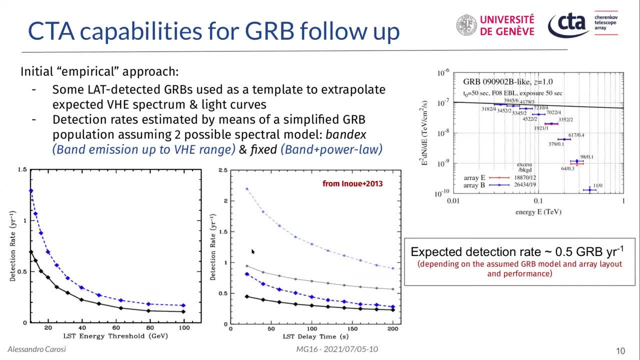 of course. in any case, you can see that the number were very somehow limited of the order of of one event per per year, per array, depending on the assumed GRB model and the array layout and performance. But this was then in. 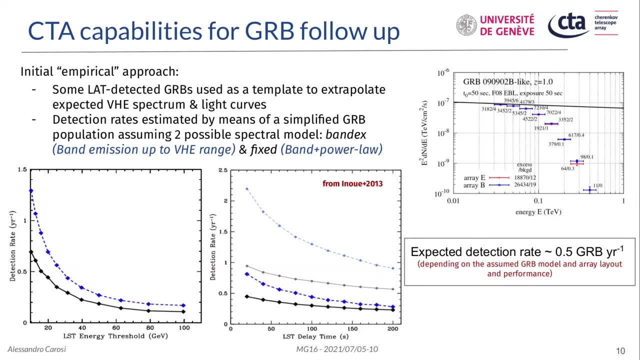 in 2013.. So where we didn't know about, about the current Miller-Bloom energy detection, And if we didn't know about the characteristic of a CTA array, that now we know much better. So right now there is. 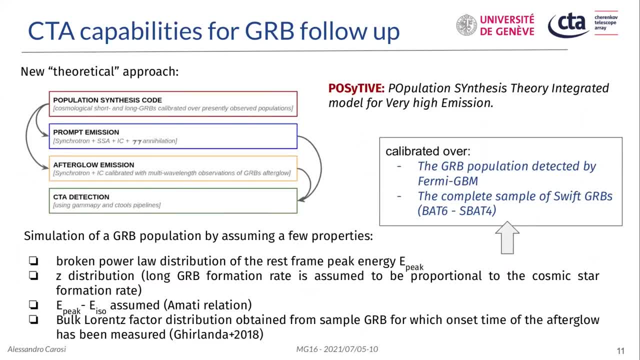 there is a new theoretical approach that is under development, in which we are stimulating a GRB population that, by assuming few intrinsic properties, like the distribution of the peak energy, of the, of the events, the redshift distribution then, and the the we assume, of course we assume that this grb population will follow the so-called 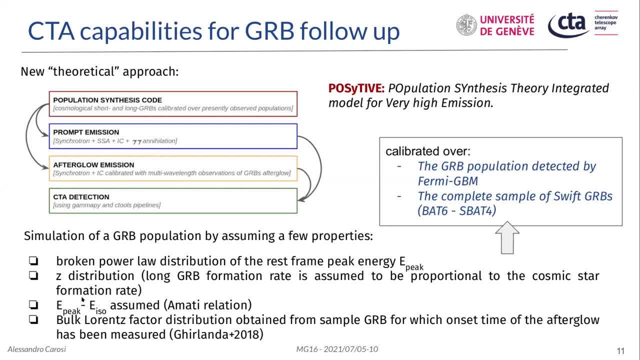 amati relation. so the, the release, the relation between the the peak energy and the equivalent isotropic energy, and the distribution of this, uh grb, this population, uh, these events will have a bulk lawrence factor, that is, uh follow a distribution that is obtained by, by a sample. 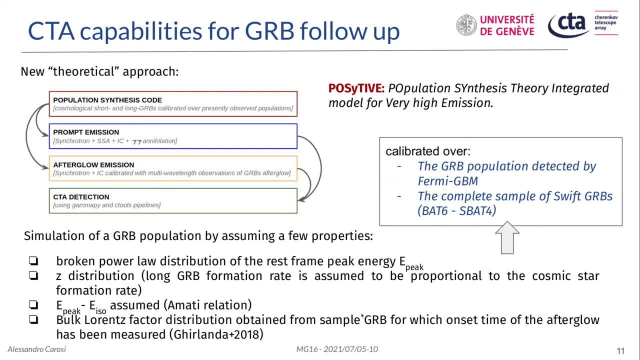 of g of real grb. so um, uh distribution for the bulk lawrence factor, that is obtained by measuring the onset time of the afterglow for uh, for uh, for uh, the grb population. so all these uh intrinsic property are calibrated over the, the um, the real sample of grb, in particular using the the. 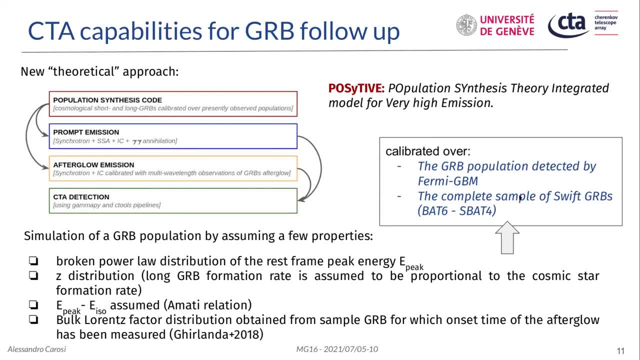 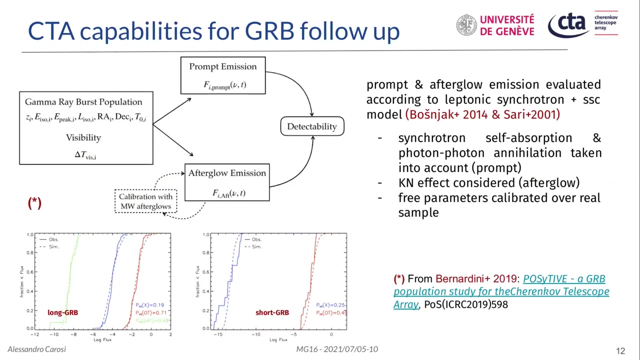 the catalog for from, from fermi, gbm and from swift, for both the long and the short grb and the name of this, uh synth. this population model is called positive, that stands for population synthesis theory, integrated model for various energy emission. and so once we have our grb population calibrated over the, the real sample of of observable grb, we can account. 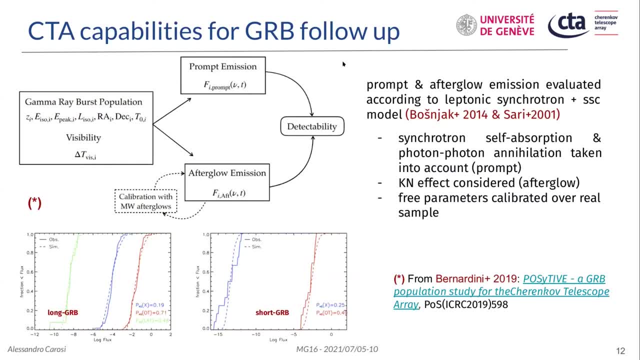 for the uh um nature of theradas drawing. So also 막net, or dried rigor um get the grb truly narrow tight. the group of uh 지만 isson, yeah, amount that mf is either much uh high or uh yeah, I like you American. uh, yes, let's. 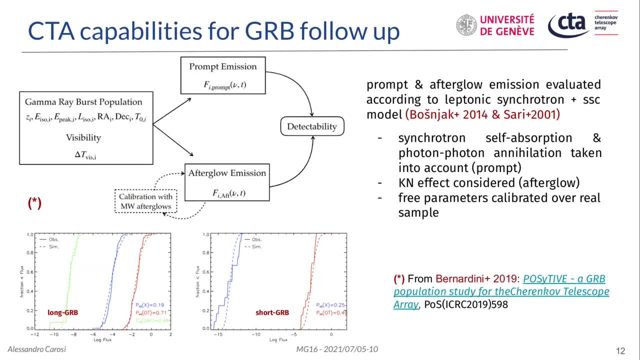 try uh. introduction to of ijke model, so uh uh, how uh? and Public Theory. So here this kind of emission models are taken into account. so everything is feed with the distribution of AISO, redshift, EPIC and the duration of the GRB. 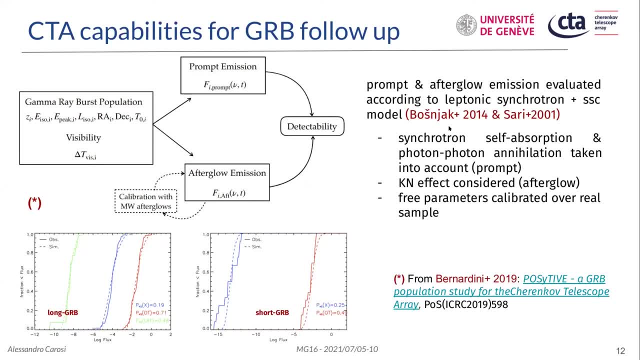 And this model are used to calculate the very high energy emission for expected in the CTA band. So some correction are taking into account, in particular the synchrotron self-absorption and the photon-photon annihilation for the prompt emission and also the Klein-Eschin 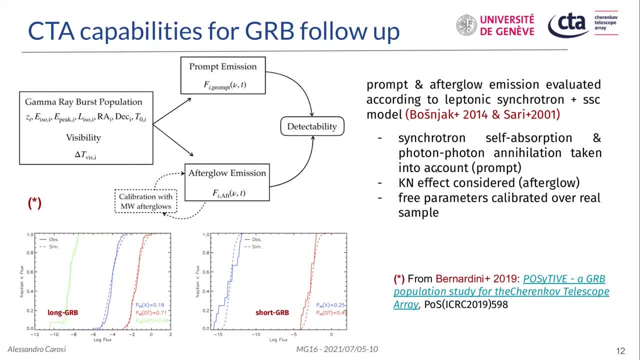 effect that are considered also in the afterglow. The remaining three parameters, like the micro-physical parameters, Five minutes, Alessandro. five minutes. Okay, thank you, Francesco. So the remaining three parameters are calibrated again using the full sample. 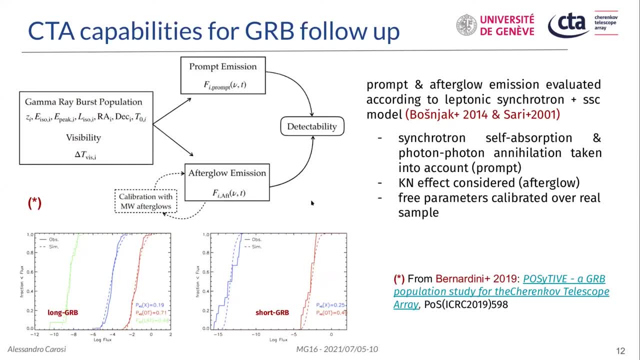 So this is a sample of GRB observed in another wave band and here in the bottom plot you can see the- let's call it the luminosity function in different wavelengths, so in the X optical and in the LAT energy band. for the simulation population that is the dashed line. 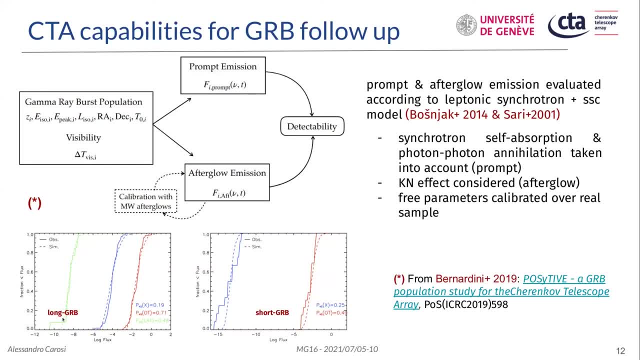 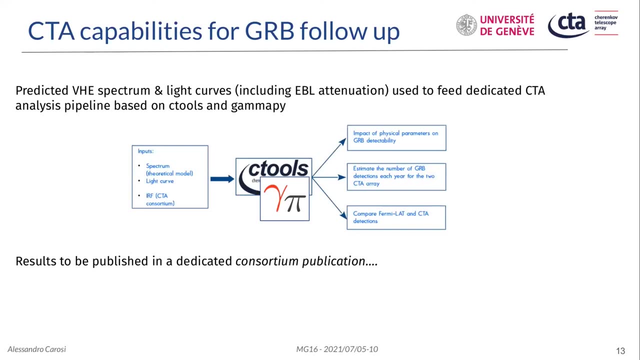 and the observed population. that is the solid line. So you can see the match of the Between the simulated and the observed population. So once we have the simulated spectrum, the simulated light curve, we of course have the instrument response, the appropriate and the latest version of the instrument response. 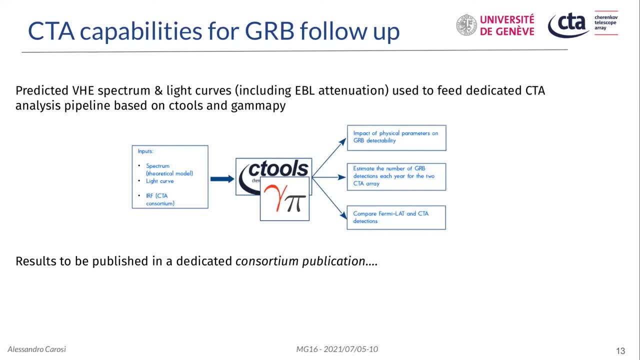 function for the CTA. All these ingredients are used to feed the dedicated analysis pipeline that are developed by the CTA collaborators, so using different tools, in particularly the C tools and the gamma pi, So we have two different pipelines, Okay, And this will allow us to determine in a robust way the expected number of GRB that we can. 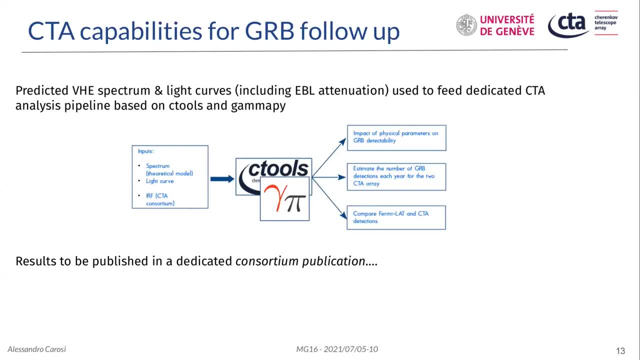 expect by a possible detection by the tool array and also to optimize the possible strategy in follow up for the future observation. So these kind of numbers I cannot still provide it because we are still discussing. I can anticipate that in terms of, In terms of detection rate. we are not talking about, of course, tens of event per year. 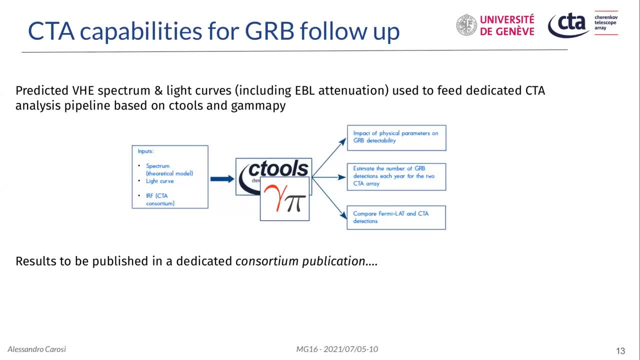 We are always talking about some events per year, per array, So this will depend, of course, by the characteristics of the array and by the strategy that we are going to follow, And these results will be published in a dedicated consortium publication that will probably 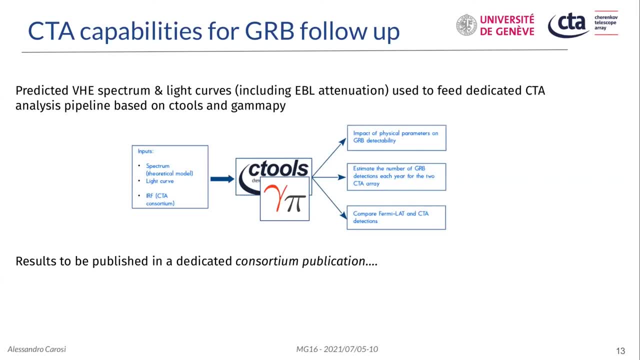 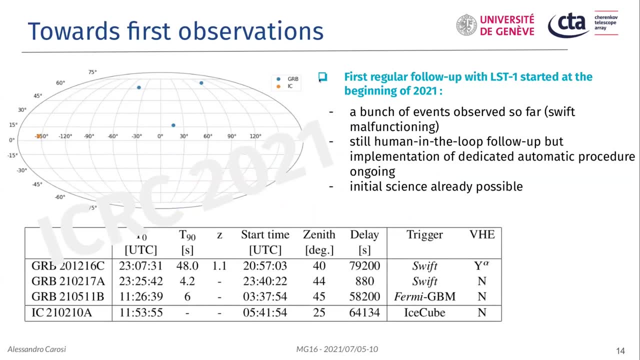 came out, I hope by the end of this year, But most likely for the beginning of the year. Okay, So this will be the end of 2022.. Just to conclude that what we are doing so far is a work on prospect, but we are finally. 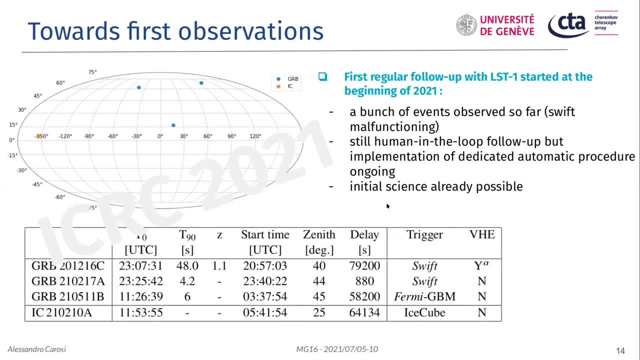 moving also to real observation, And here is just a slide that I grabbed from my contribution- the next forthcoming ICRC 2021, in which we will report about the first observation, the first follow-up of transient event, in particular GRB and neutrino alerts with with LST1.. 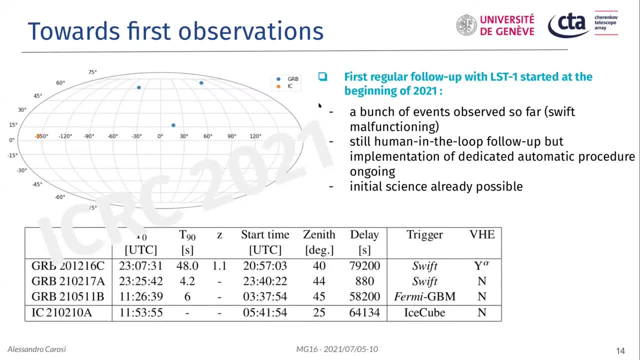 So with the prototype of the 2023 LST1.. Okay, of the 23 meters telescope in La Palma. So the telescope it's sending is commissioning phase, but we are gradually entering in regular scientific operations. So an initial science phase, it's the starting. 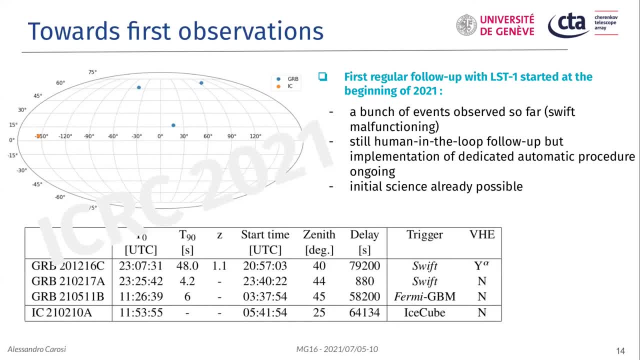 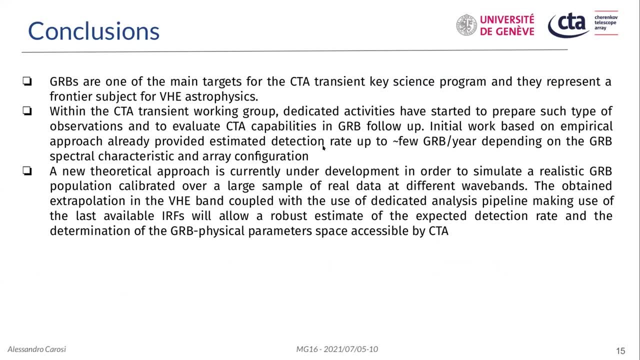 and we are producing already some follow-up and some results. So I leave here my conclusion, because otherwise I guess I'm out of time, and thank you for your attention. Yes, thanks quite a lot, Alessandro, for the nice presentation and the nice out. 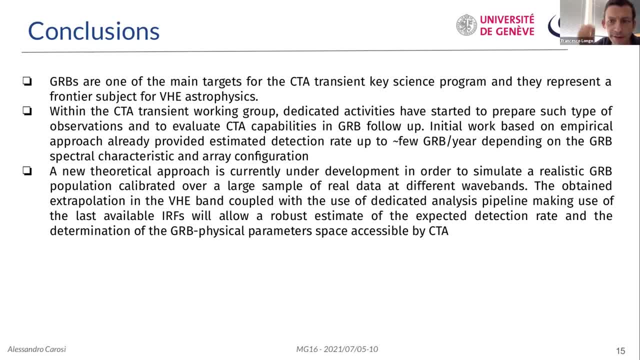 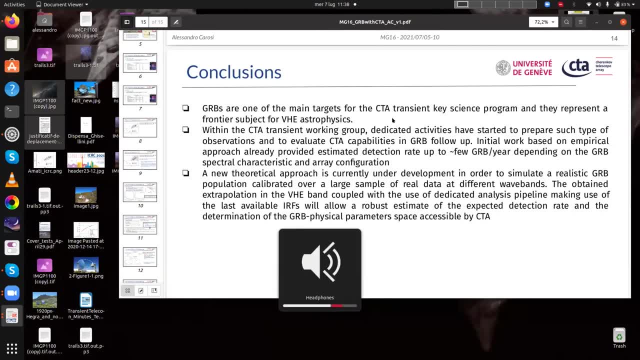 let's say for coming results by CTA. So Ioni, please. Hi, thank you very much for the nice talk. I wanted to ask essentially: in your model there are many model parameters that enter and so on. It is very nice that you calibrate. 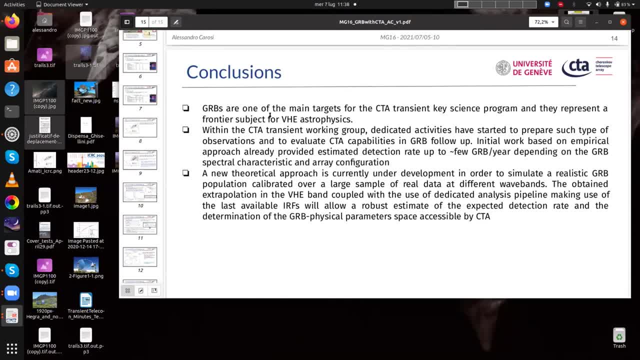 according to current observations, However, probably you still cannot determine all of the model parameters uniquely, and some freedom probably still remains. So, in light of this, might it not make more sense instead of aiming at the one final number for the rate that you would expect? 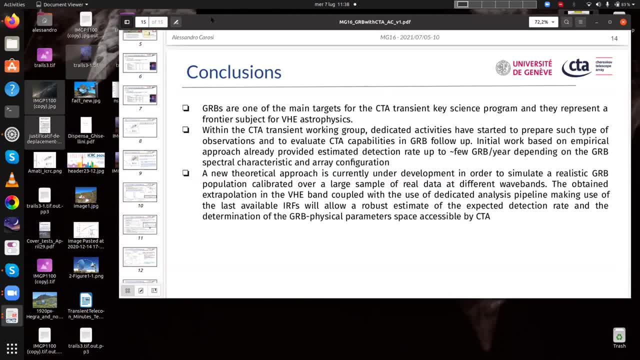 to instead determine the probability distribution, or what is a plausible range of event rates that you might expect? Yes, definitely. This is actually a very great, great, great suggestion. So I definitely agree. So I really think that this suggestion can be implemented. 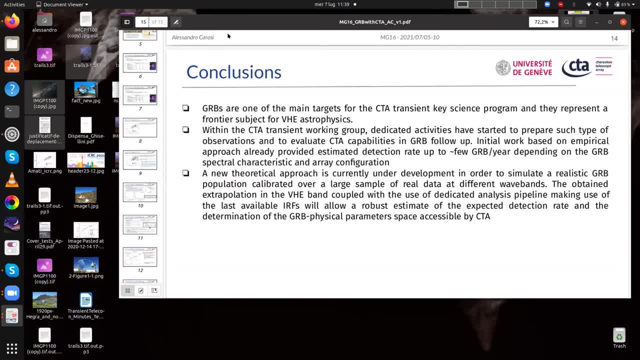 in the sense that the detection rate that, given as a number like this, it might be, of course, bias by all the uncertainty and all the freedom parameters that are used to model this kind of population. I definitely will take into account this suggestion, Thanks. 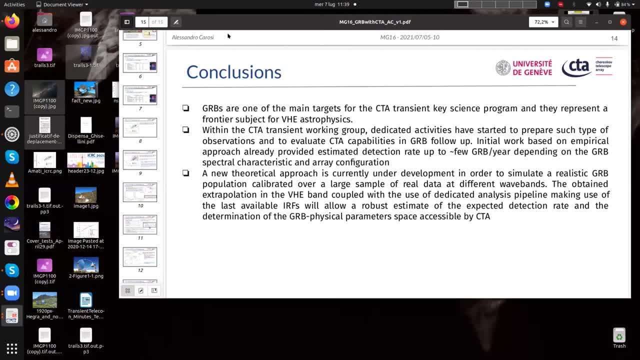 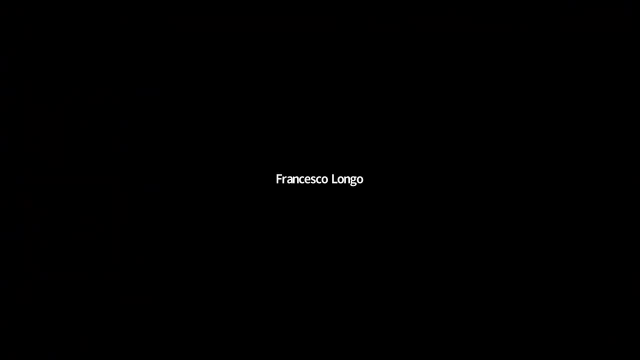 Okay, So if there are no other question, we thank Alessandro again for his nice talk, And then we'll go back to the S-hour array and we discuss about all results on Monday And today. instead, we have a very nice presentation on the LASO approach to GRB. 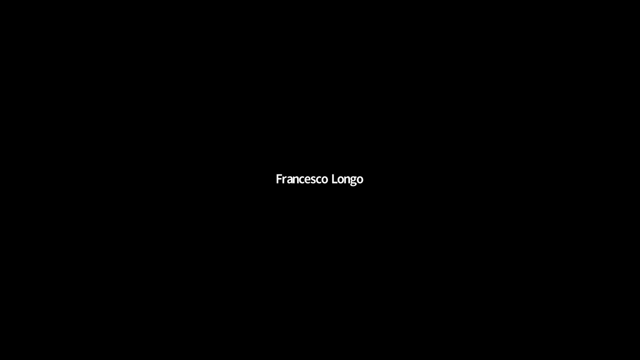 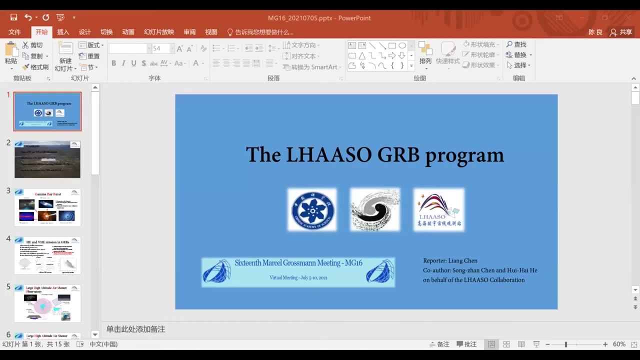 So please, Liang, it is your turn. now, Dr Chen, it is your turn. Okay, can you hear me? Yes, there are some noise in the background, but I can see at least your screen. I'm sorry about that, but I 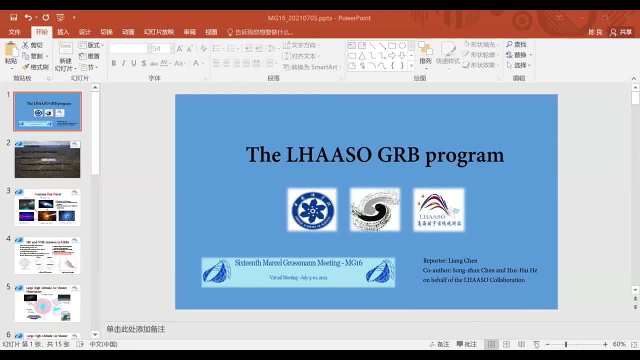 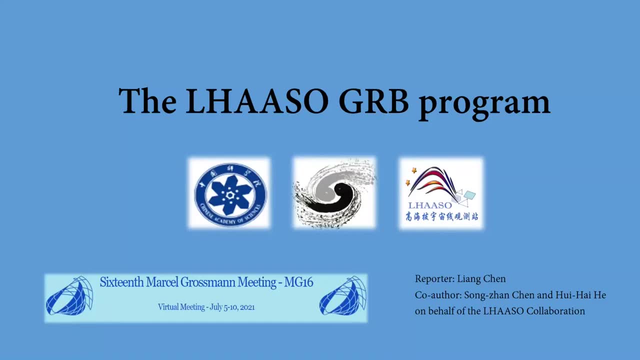 Now better, now better. If you are close to the mic, I think it's better. Can you see my screen? No, Can you see my screen? Yes, Hello, Can you see my screen? Yes, Yes, Yes, Yes. 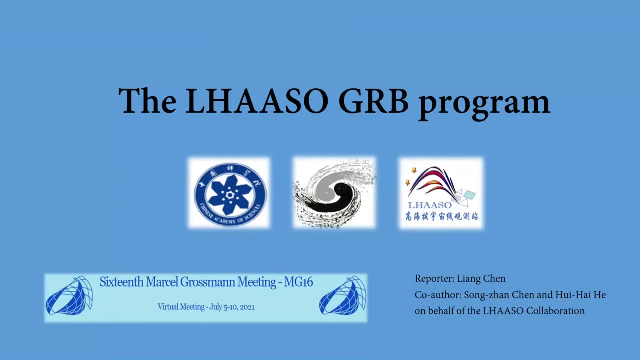 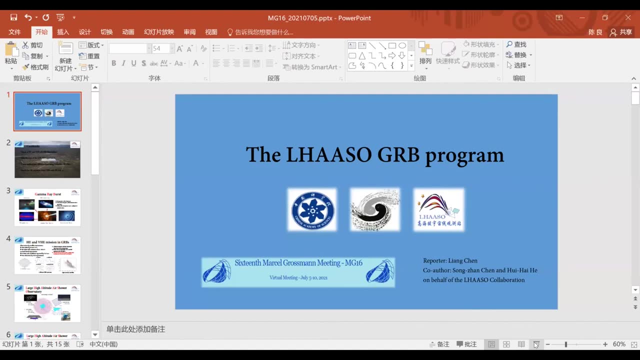 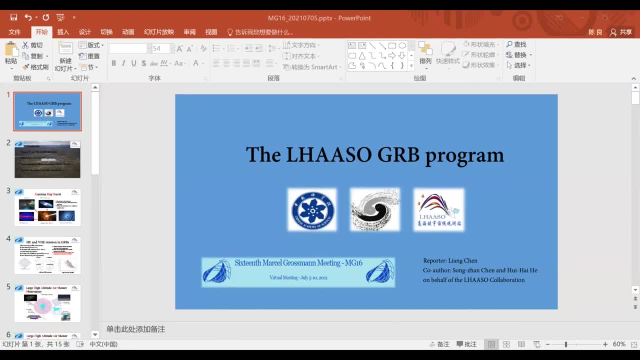 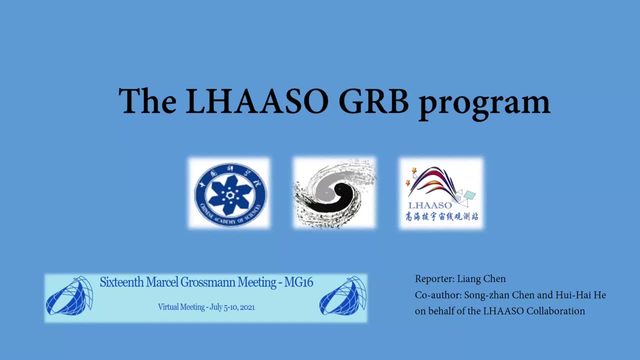 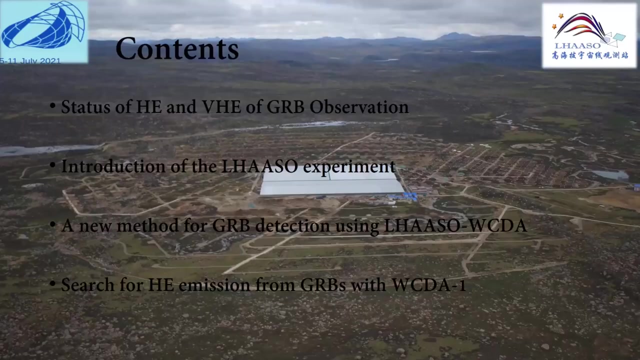 Okay, Okay, I will start my talk. Hello everyone, my name is Liang Chen, a PhD graduate from the Dassault Corporation. It is my pleasure to share my work here with you, And the report will be conducted by the Holy War Parts and major content of this report. 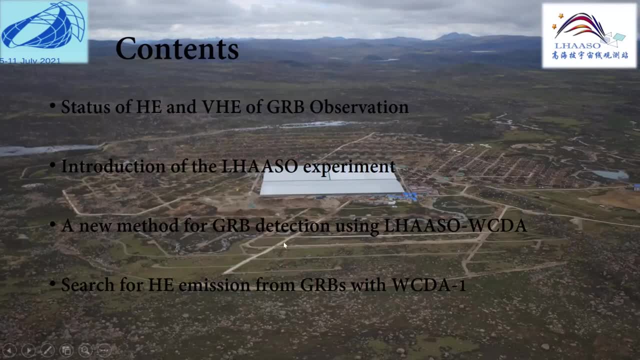 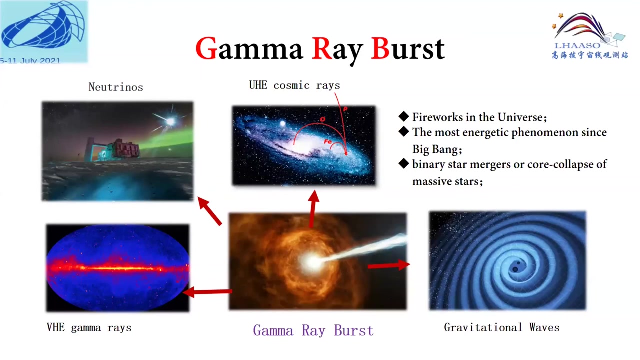 is a new method for GRV observation by Dassault- WCDA- Okay- And also share our preliminary data analysis and results on the quarter WCDA. Okay, Let's begin my talk. As we now know, GRVs are the most energetic phenomena with the Big Bang. 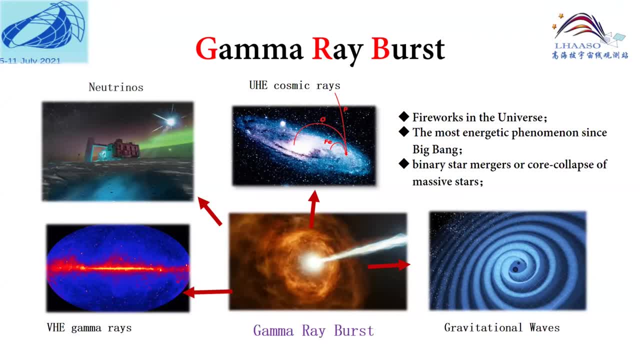 They are originated from binary star markers or core clefts of massive stars. Okay, Presupposing two short GRVs and long GRVs- And GRVs are popular objects since they are highly-reliable objects. They are highly correlated with very high-energy gamma rays, high-energy neutrinos and also 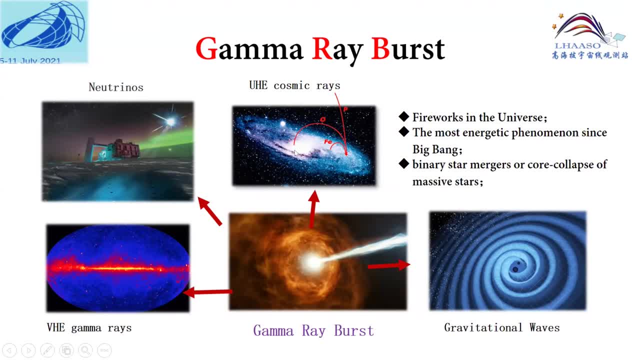 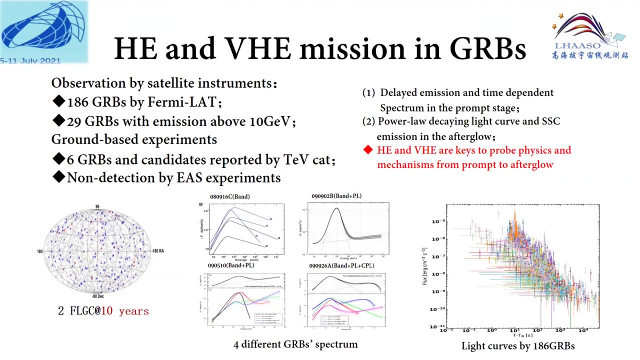 high-energy Huffington rays Multi-messenger observation gives strong association with the gravitational waves About high-energy and very high-energy emission in GRVs. Thanks to the rare performance of Fermilabs, it opened the high-energy emission of GRVs from 2009 to 2018.. 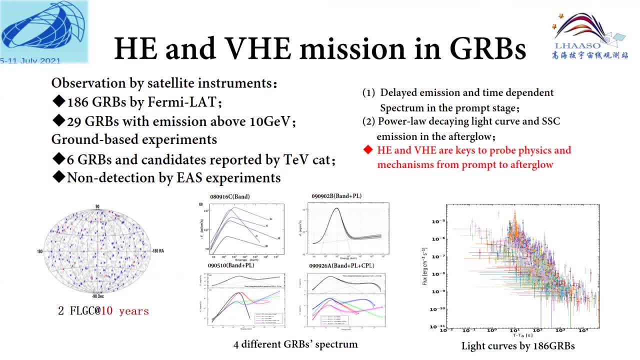 186 GRVs were observed by LAT and 29 of them were observed with emission above 10 G-eV. Results showed delayed emission and external components above G-eV In the prompt state. in the prompt emission there exists complex time-dependent evolution. 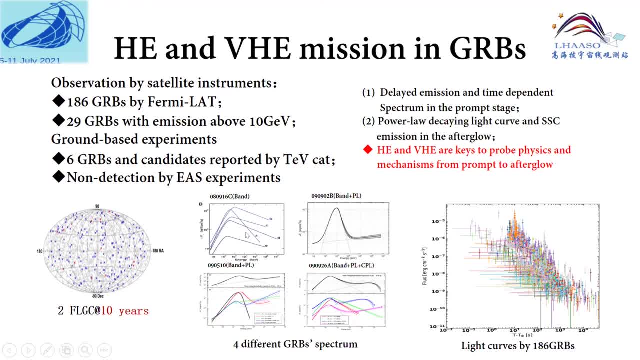 of energy spectrum, As you can see in GRV, the four GRVs. As you can see in the four GRVs For the ground-based experiments, the IACGs first opened very high-energy emission in GRV 1901-14C and up to now six GRVs. 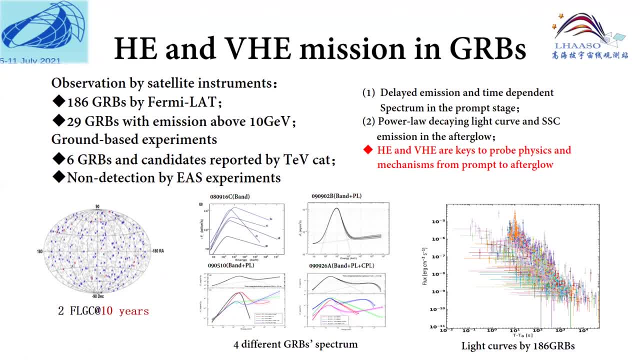 Six GRVs and candidates were reported at the IACGs. Observation showed similar signature with the X-ray afterglow, Since high-energy and very high-energy emission were observed both in the prompt stage and the afterglow. there are keys to probe physics and magnetics from prompt to afterglow. 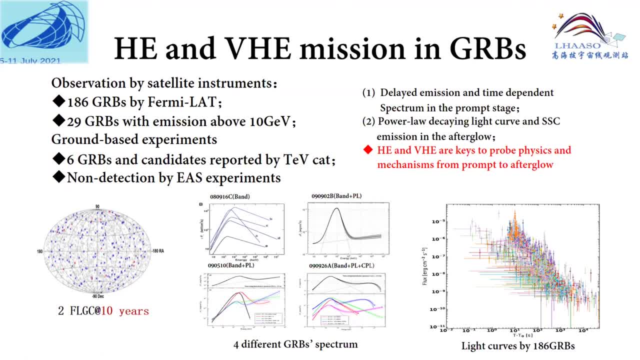 However, for IACGs, the narrow field of view and strict observing condition makes them difficult to catch probes. Therefore, a large field of view and all-day 43 instruments is better for GRV prompt emission. Therefore, a large field of view and all-day 43 instruments is better for GRV prompt emission. 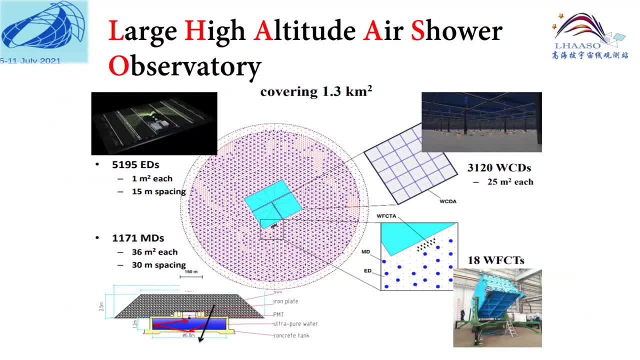 I will introduce the Large High-Edge-to-the-Air Shower Observatory. The Large High-Edge-to-the-Air Shower Observatory, also named LASSO, is a new generation observatory built in Daocheng, Sichuan Province. It is a very beautiful place. 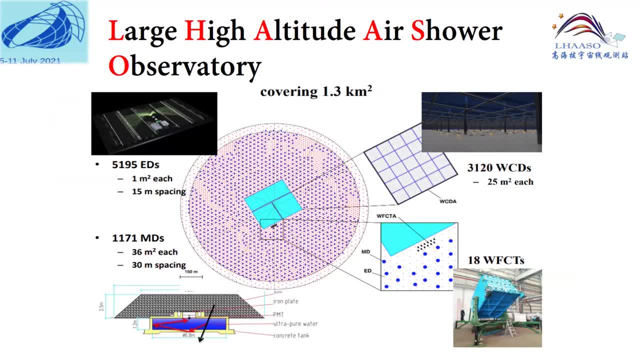 The LASSO is one of the most important observatories in the world. The LASSO is one of the most important observatories. It is the second largest observatory in the world for objective objectization and constitutive cosmic-ray and gamma-ray experiments in the world. 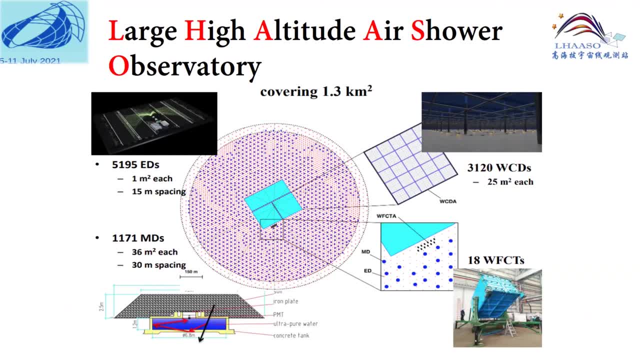 It contains 4 parts, 5- motor電. 할게요 from resignes 5.195 electromagnetic particles, also named EDE, which measure electromagnetic particles. It is also a very small observatory for group modes of measurement or which isn't. 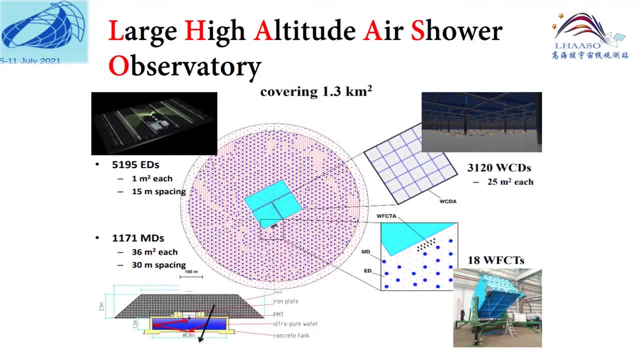 Visible to many people, like from larger subjects. 1,171 neuron detectors with mirror neuron components in the shower. This means that the radio, the dimミー of tick� voyager, can monitor the объセائろう capac arguments, and also recorded implic―機시. 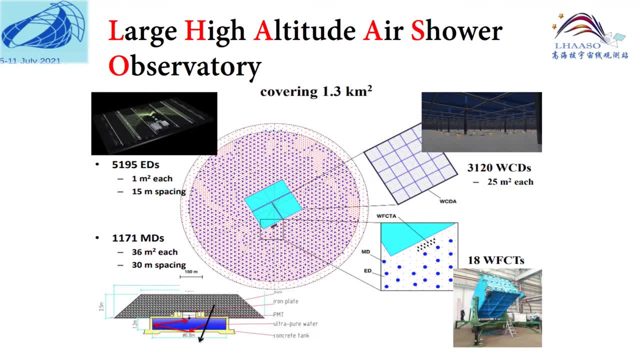 It is a very small observatory in Daocheng, The Св escrəбеº в propre. InShawers is a small observatory called InShawers economically and grilled exhibiti. gern pit ум. Also, we call it MD, EDS and MDS of the KM2A, which is focusing on ultra-high-energy gamma-ray astronomy. 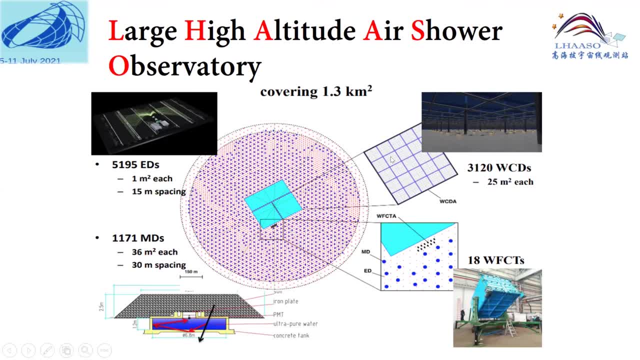 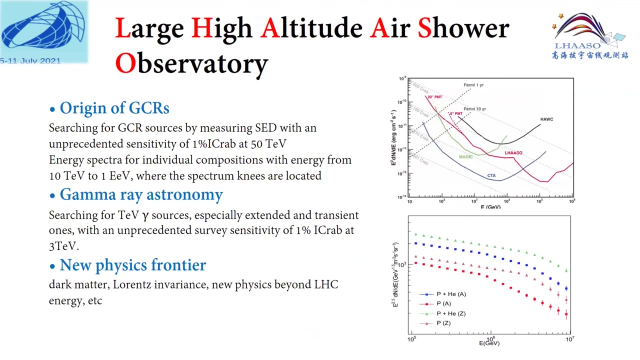 And on the center is the WCDA, which mirrors Cherenkov types of secondary particles. We will introduce it next And also shown here is the WCDA- ambient cosmic-ray measurements. The main scientific goal of NASA's Context-3, the Origin of Galactic Cosmic Rays. 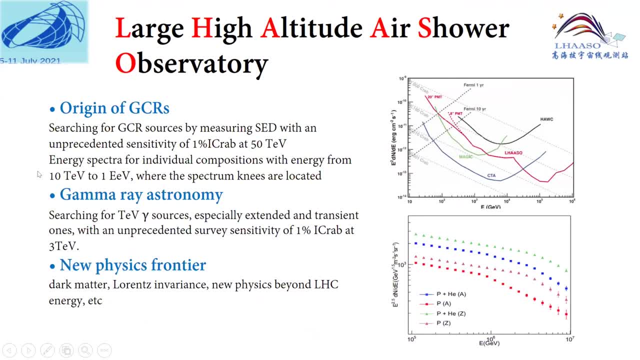 mainly for searching for galactic cosmic-ray sources by measuring the energy spectrum within an unpredictable sensitivity of one percent, But perhaps as 100 TeV we find for particles in the galactic world And the energy spectrum for individual components, with energy from 10 TeV to 1 TeV. 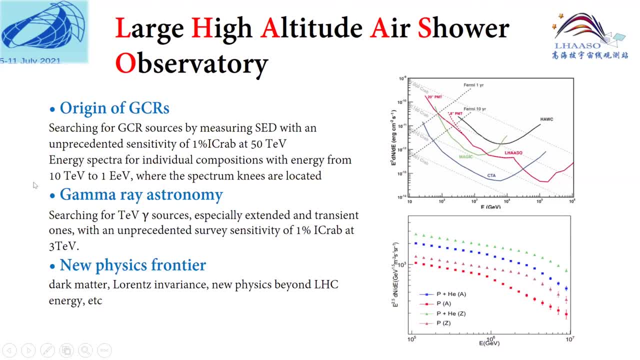 is to find the cosmic-ray physics, For example the knee, And for gamma-ray astronomy, mainly focusing on northern TeV. gamma-ray sources is fairly extended and transitive ones, With an average extended survey: the training of one-person crab at 3 TeV. 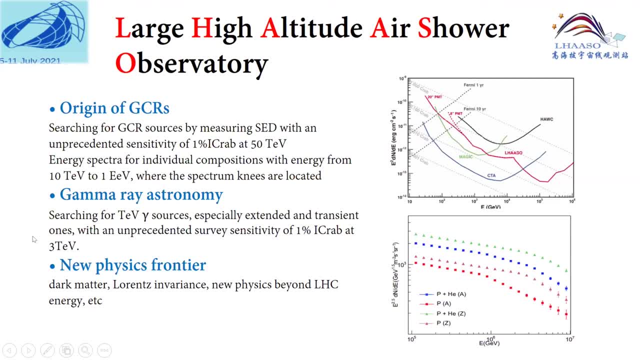 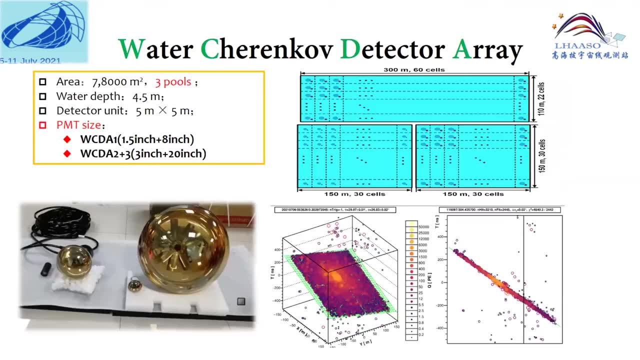 And the first is new physics frontier, such as black matter, Lorentz, invariance violation, new physics beyond LHC and so on For GRB program. the last one is mainly The array, mainly the WCDA. it covers an area of 78,000 square meters. 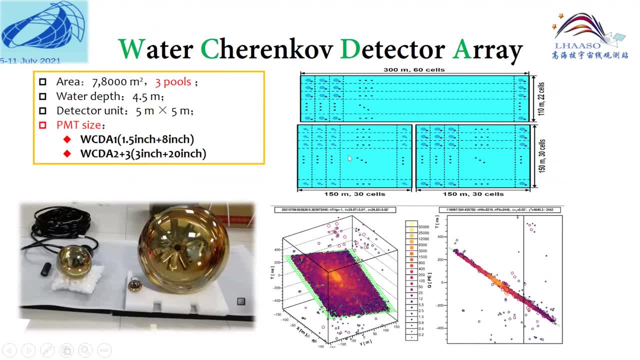 And we have three pools. The first pool uses 1.5-inch and 8-inch PMPs to receive signals, And the second and the third pool use more sensitive 3-inch and 20-inch PMPs, Which can reduce threshold energy and improve the sensitivity. 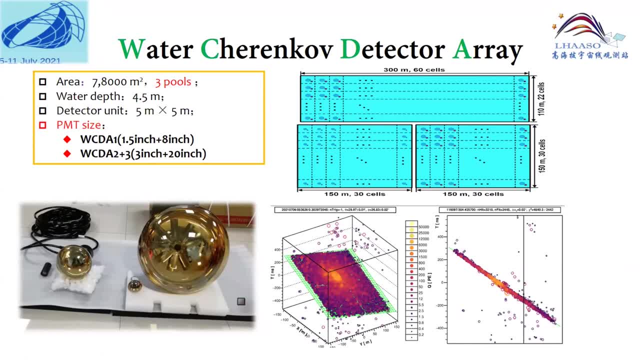 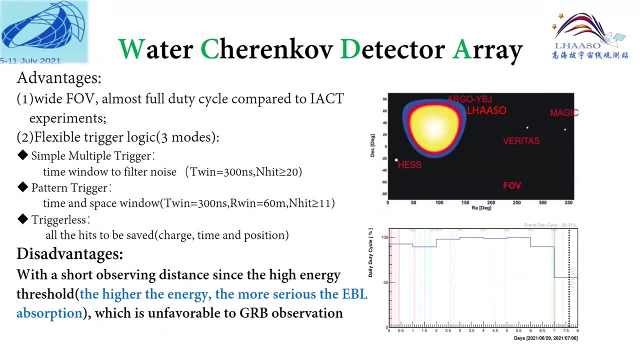 And for now the whole WCDA array is in operation showing a good performance. Here I show one event in the WCDA array Very useful WCDA has advantages of wide field of view and almost a broad duty cycle. And whatever the powerful DAQ makes, 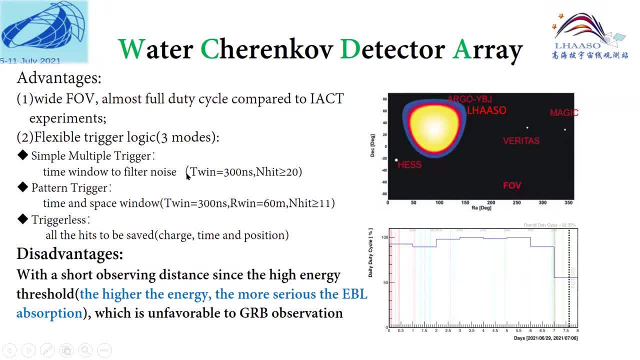 it is easy for WCDA to develop flexible trigger logic focusing on different physics, And for now it has three trigger modes: Simple particle trigger, pattern trigger and triggerless trigger. The triggerless mode stores all the keys, including time, charge and position. 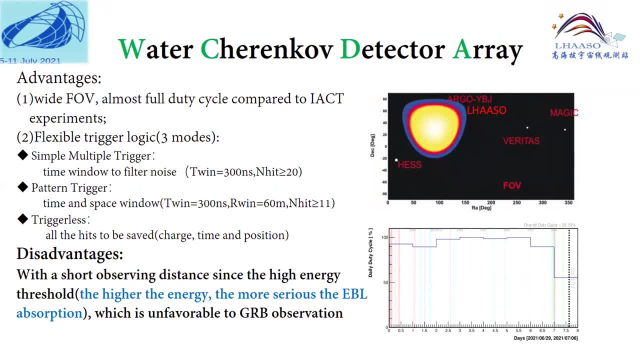 making it possible for us to develop offline triggers. However, the high energy threshold is the most difficult thing to detect GRB. with WCDA, The typical energy is about T, which is unfavorable to GRB observation since the EDR absorption, as we know. 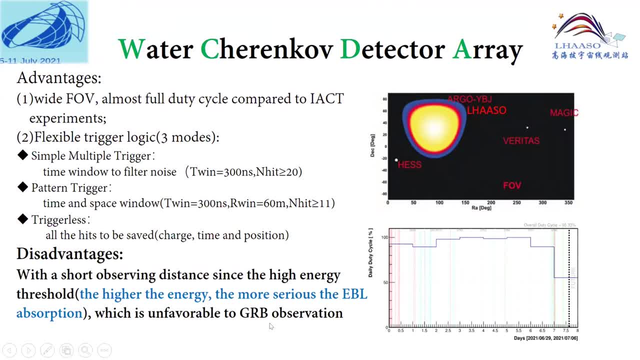 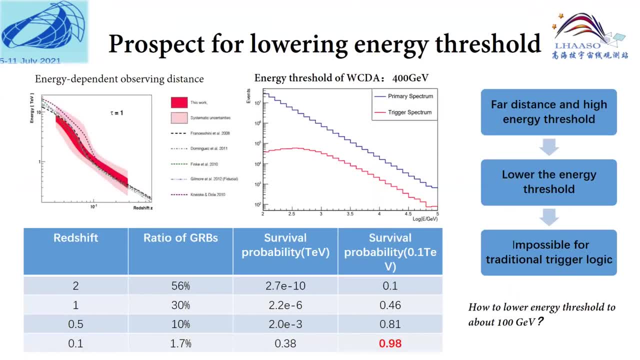 the higher the energy, the more serious the EDR absorption. What we want to do is to reduce the threshold energy of WCDA And you can see in this table that in the red shift of 0.1, the GRB only covers a percent of 1.7.. 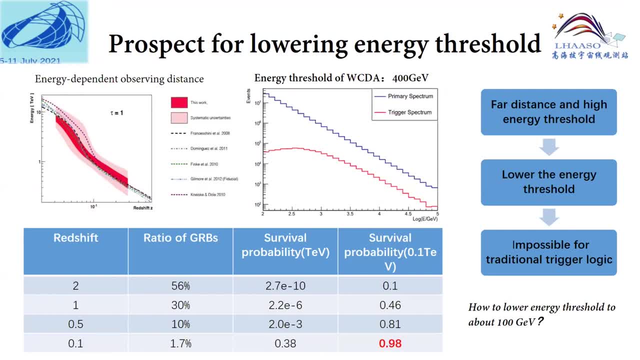 And even at such a close distance, the survival probability at T is only 38%. Only at about 100 G the EDR absorption can be ignored, And therefore we want to reduce the energy threshold to below 100 G, And this is very hard to accomplish. 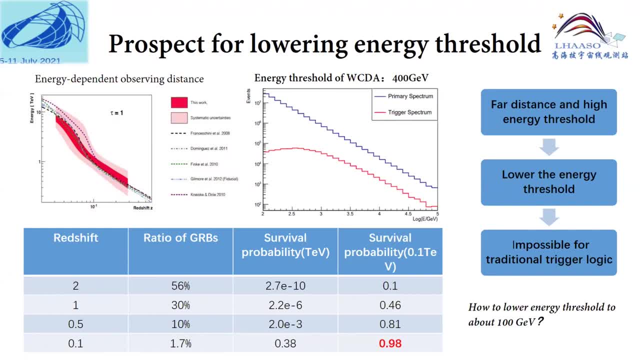 for a higher noise detector such as WCDA. The main problem is that we have a wide field of view. This was due to the large trigger window, about 100 nanoseconds. If we reduce the trigger window, we can filter more noise, But at the same time, 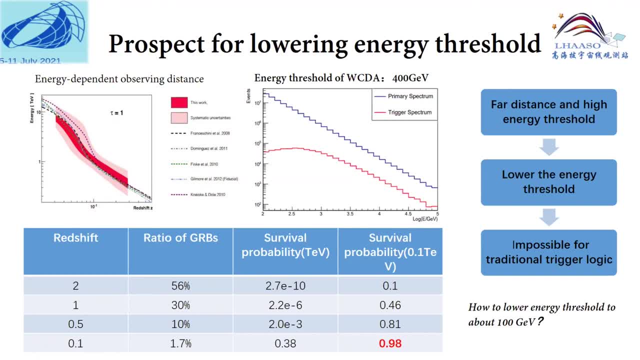 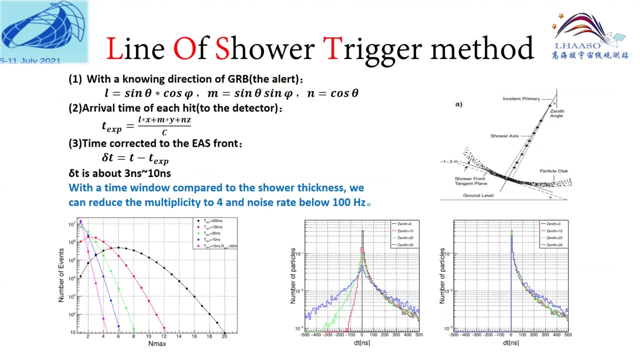 we will lose largely the sample events And therefore how can we lower the energy threshold to about 100 G? And here we propose a new method named the line-of-saw-trigger method, And the time and the position of secondary particles follows a planar formula. 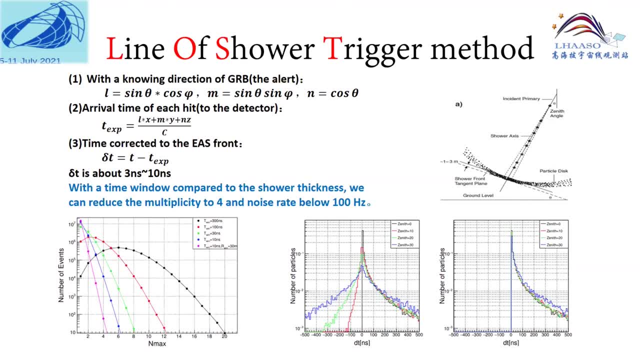 For the no-direction sorting, such as GRBs, we can get the direction vector and then calculate the expected arrival time of each heat, And after that we can correct this and change the time. to the shower front. The shower front is also about 1 to 3 meters. 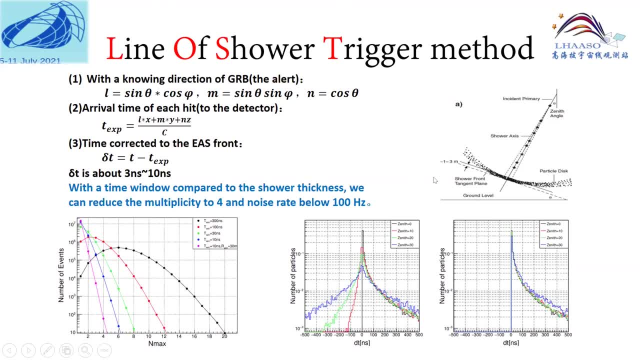 corresponding to the time range of about 3 nanoseconds to 10 nanoseconds, And with a small time like this, with a small lifetime like this, we can filter more noise and we won't lose largely the sample of GRBs With the time window. 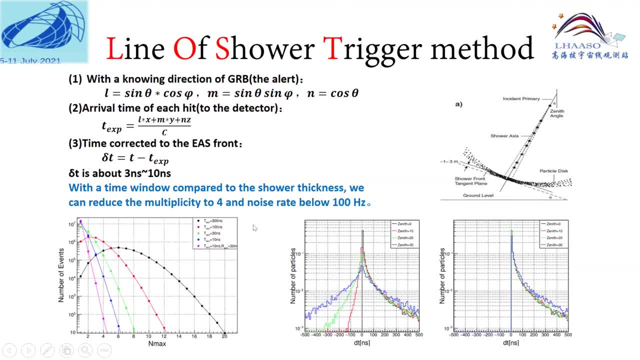 compared to the shower thickness, we can reduce the mass velocity to 4 and the noise rate to below 100.. You can see in the right, in the bottom of the right picture, after the time correction, the arrival time, the time risk is significantly. 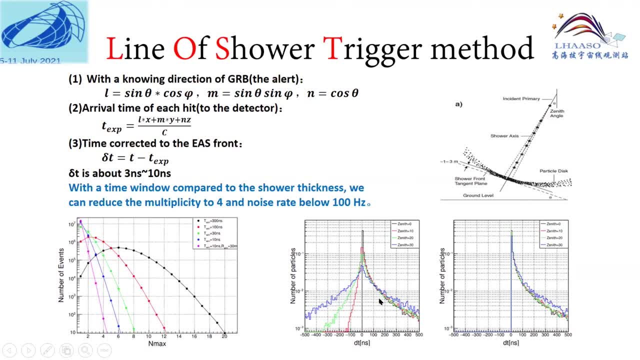 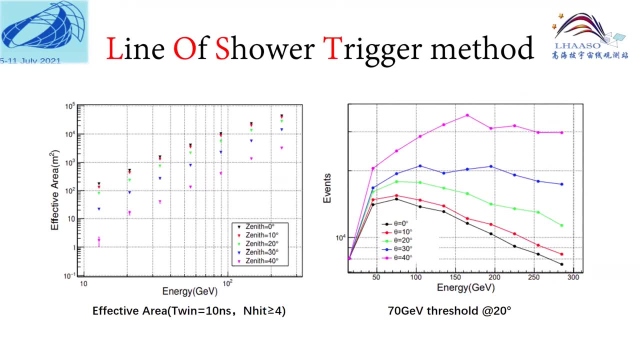 is significantly smaller than than before. We use the last method to simulate the effective area and then calculate the energy spread show after about 4 days, giving our promising results With the effective area of several thousand square meters at an angle below 20 degrees. 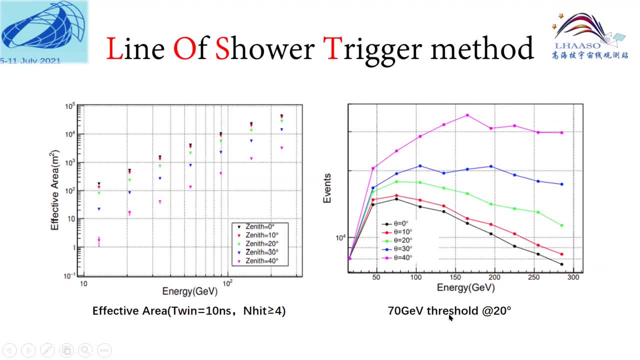 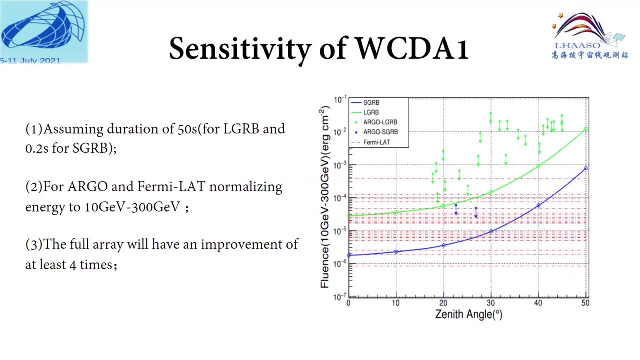 and the energy spread showed of 70 GeV. And next we estimated the sensitivity of the quarter WCVA array. In the right picture also shown is the Argos upper limit and the 29 GRBs with photo energy above 20 GeV. 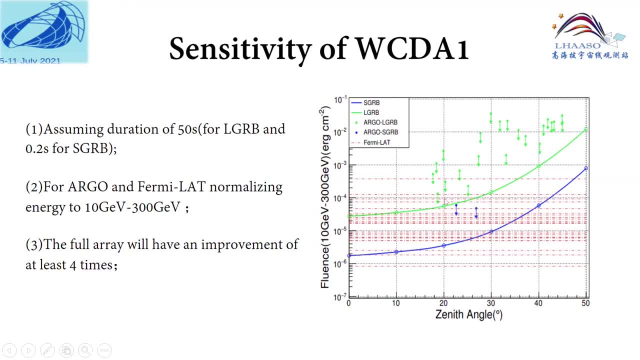 You can see that for the for the short, for short GRBs, the quarter WCVA has better sensitivity than most of the last samples. And even for long GRBs, 7 of them can be detected by WCVA. Very promising results. 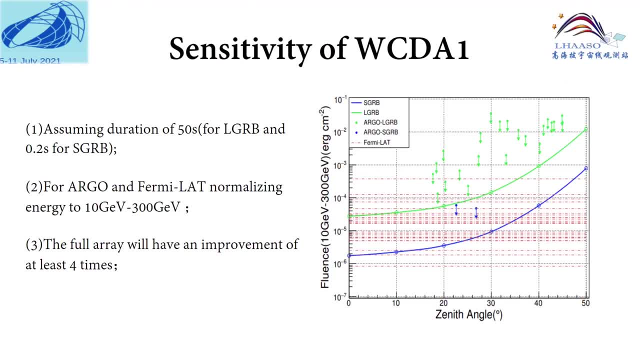 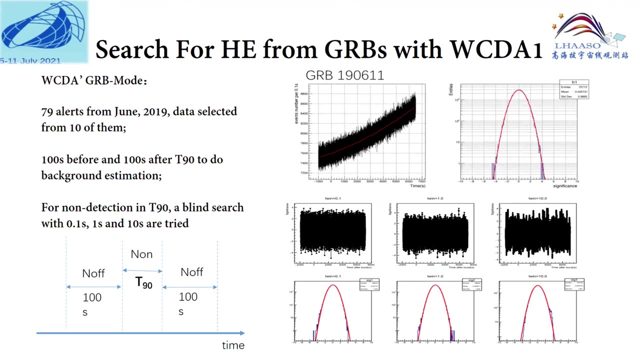 And the. the full array will have an improvement of at least 4 times since the, since the physical area will be larger at least 4 times. On the other side we analyzed 10 GRBs of 79 GRB samples got by WCVA. 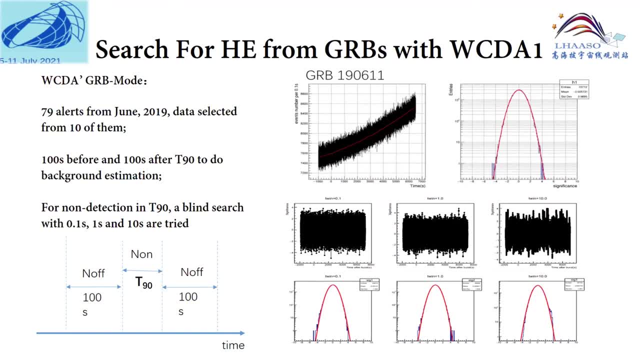 And none of them were observed. significant excess in the duration of T: 19 times. And we used also three different time windows to search to: to search for signal in: in 2.5 hours before and after the burst. After the burst: 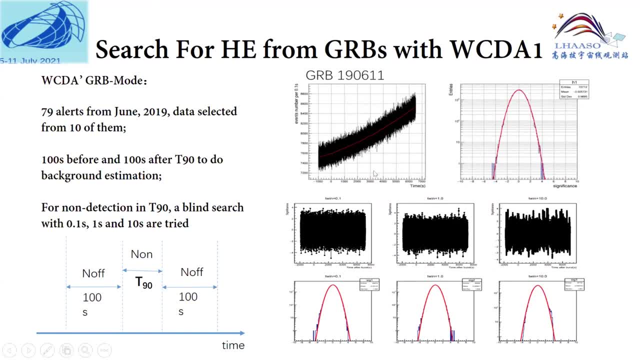 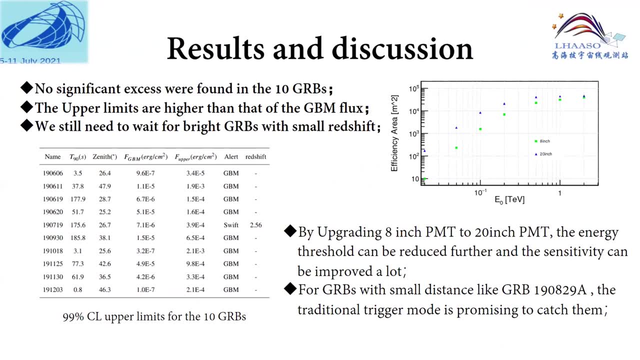 also no excess. Here is one of the examples. And last, we give 99% upper limit set by WCVA1.. You can see that for the upper limit, for the upper limit in the energy range of WCVA, the upper limit, 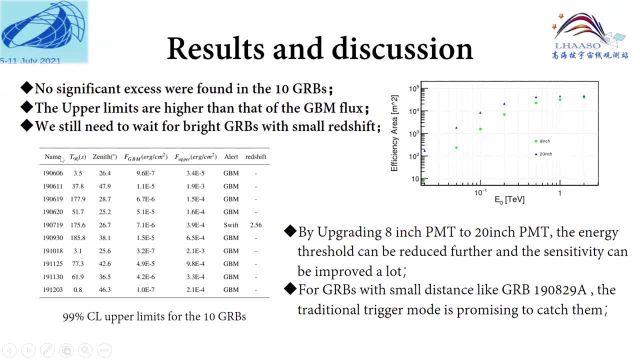 were higher than 10 of the GBM flux. It means that for most, for the for most of the GRB samples, WCVA has both a constant pathway and we can't constrain the flux well, Which means that we still need bright and small distance. 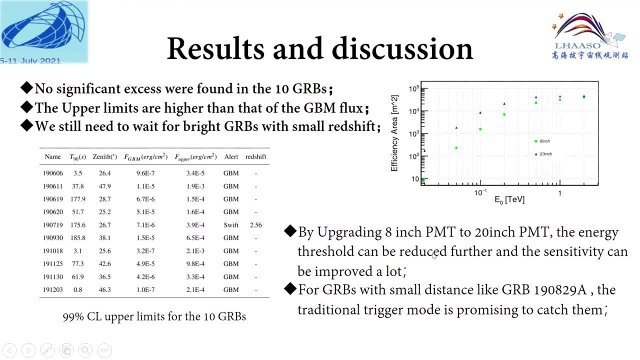 GRB samples And by a friendly 18-inch EMT to 20-inch EMT the energy threshold can be reduced further and the can be improved a lot, And for GRBs with small distance like 19,, 0,, 8,. 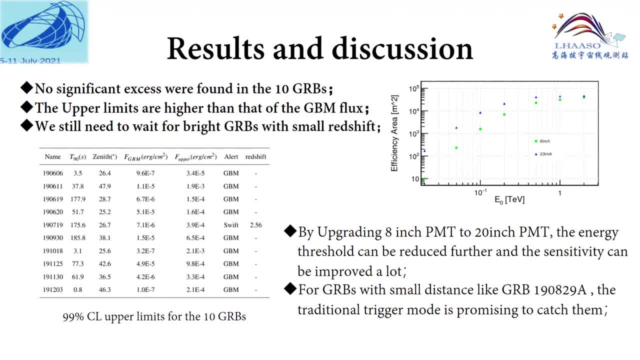 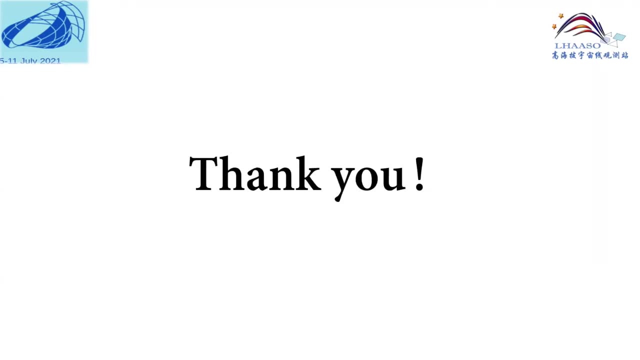 29,, 8,. the traditional trigger mode is promising to catch them And the WCVA array will have a promising result for future GRB observation. Okay, I will stop here. Okay, thank you, Okay, thanks Liang also for staying. 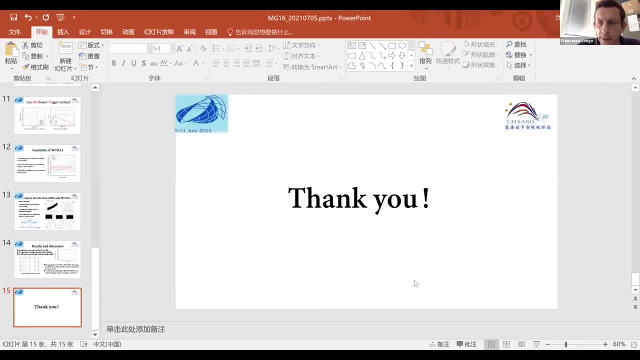 perfectly in time within your allocated minutes. So very also interesting results and hopefully, let's say, with your sensitivity we can. either you or Oak will catch GRB from the ground which is currently awaited at this largest energy. So 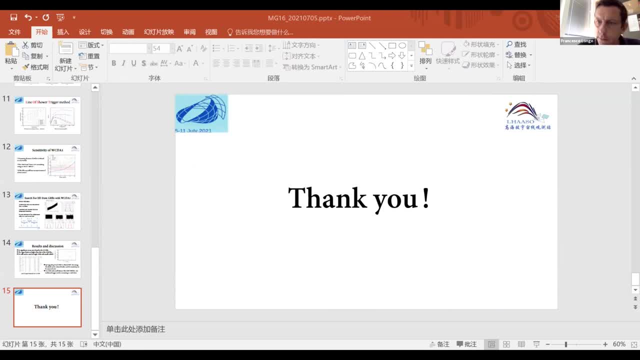 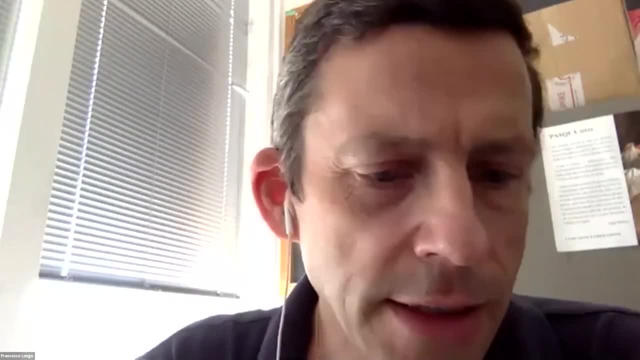 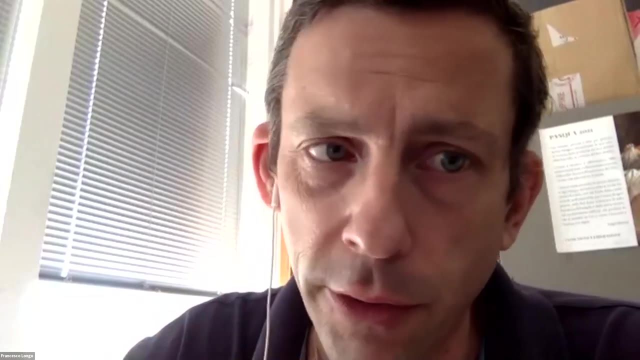 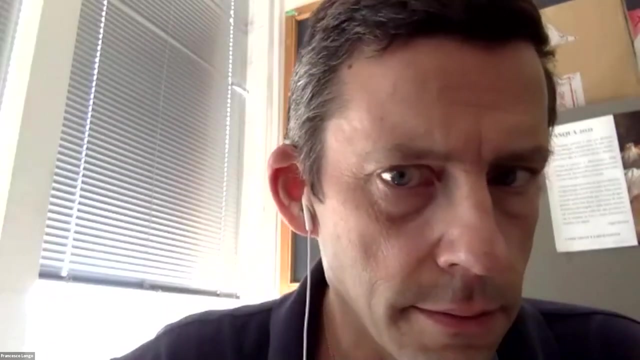 are there questions to Liang? I have one small question: These upper limits that you obtained are obtained in which timeframe? On the prompt phase or on the time scale? It was on the prompt phase and we also. we also do blind search with. 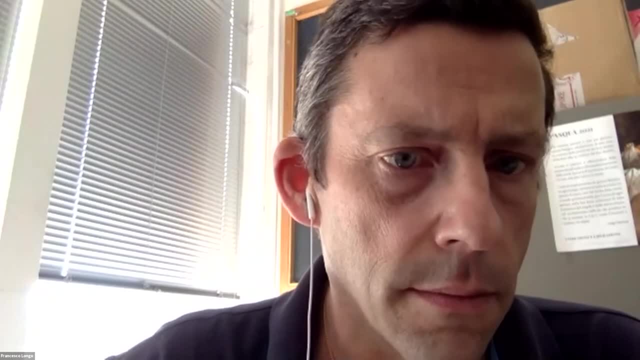 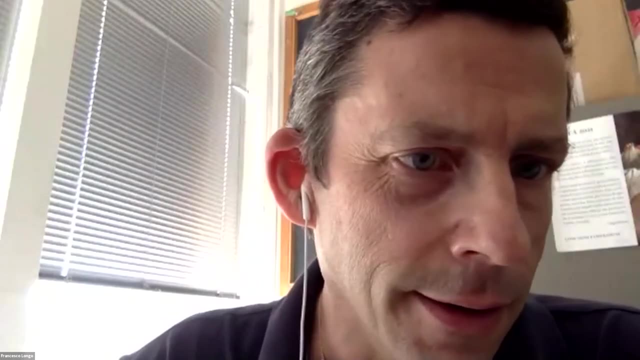 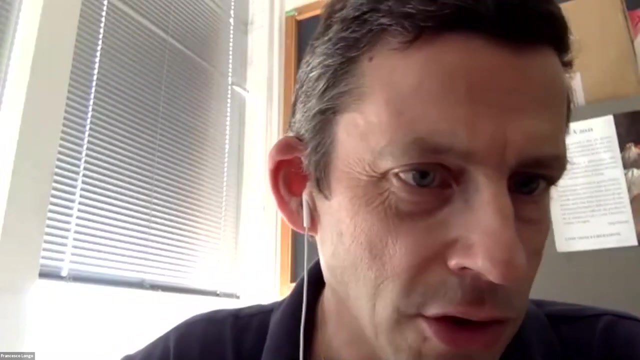 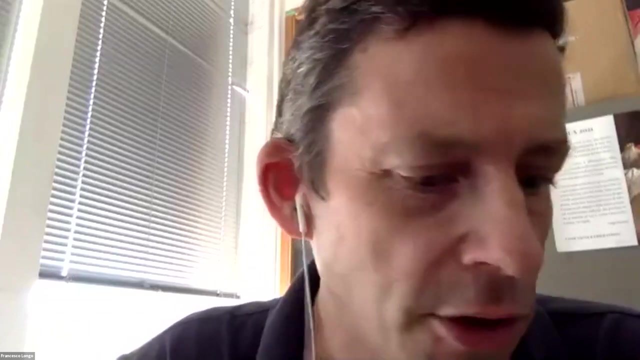 with different time window, but there have no exit now. Okay, because this might be a very nice opportunity for the shower array that can catch, say, the prompt, while the, but also since we know that the afterglow phase is the one emitting very high energy. 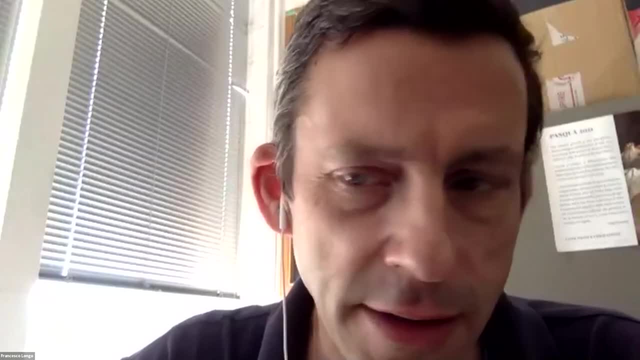 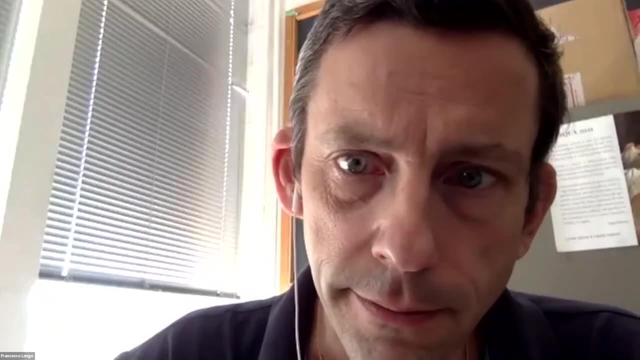 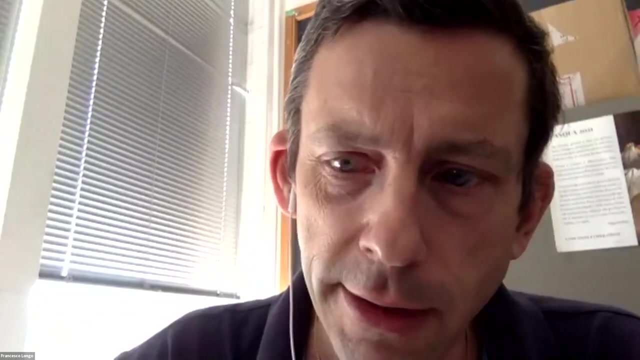 you can search for also for longer duration, to see if something is there. Okay. so thanks quite a lot for the presentation. Are there other questions to Liang? If not, we move then to the last talk for this session, from Giovanni Again. 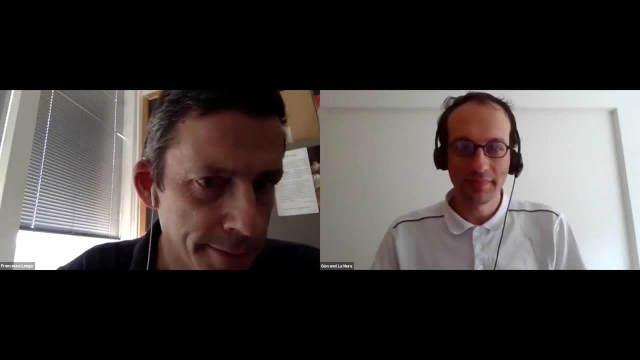 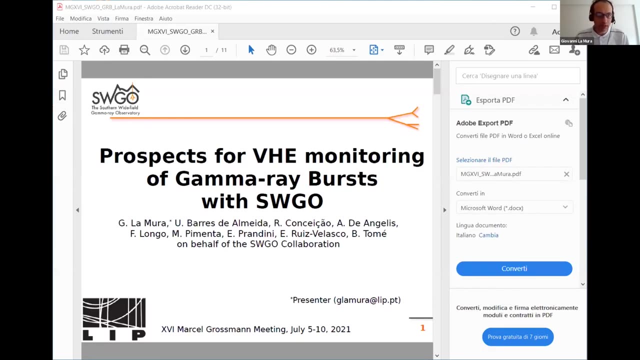 on future, in this case, future shower array detector. Please, Giovanni. Yes, I'm going to start my screen now. Can you hear me? Yes, very well, Okay, and I just need to send the slides full screen. So I guess. 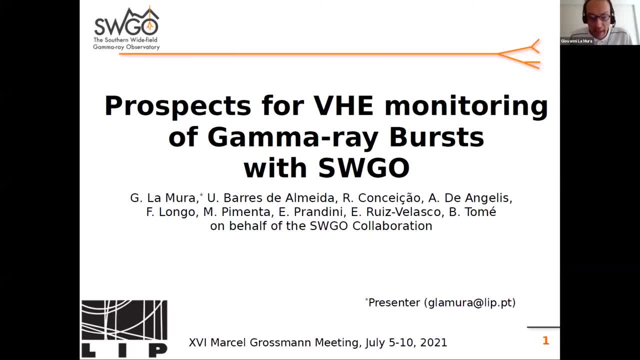 you see the slides so I can, Yes, go ahead. Yeah, First of all, let me thank you for your attention. I'm going to present the prospects for a very high energy monitoring of gamma ray bursts with the Southern Wide Field Gamma Ray Observatory. 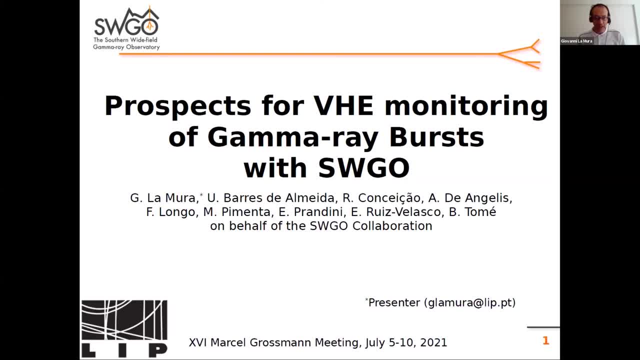 which is a new facility that is currently under research to be installed in the southern hemisphere. We already talked about the southern Wide Field Gamma Ray Observatory that is planned to be delivered by Jim Hinton on Saturday, So in this case I am just focusing. 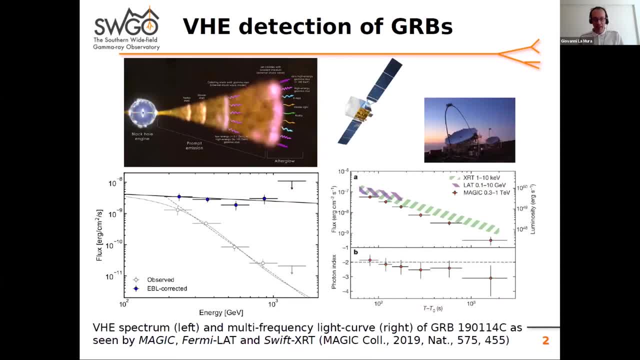 on the details of the study that we are carrying out for the scientific topic of gamma ray bursts. Now for sure, this is going to be a very high energy discovery, because several theoretical models predicted that gamma ray bursts should be intrinsically able to. 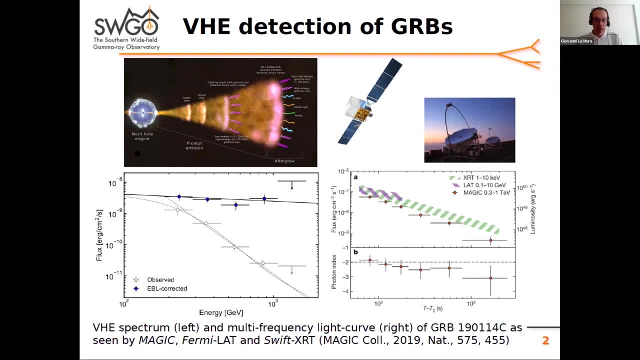 radiate in the very high energy regime And in particular, we expected different type of processes that, both during the very high energy signals and in the best cases, also be good candidates of multi messenger signals, especially for the association with the gravitational wave and possibly 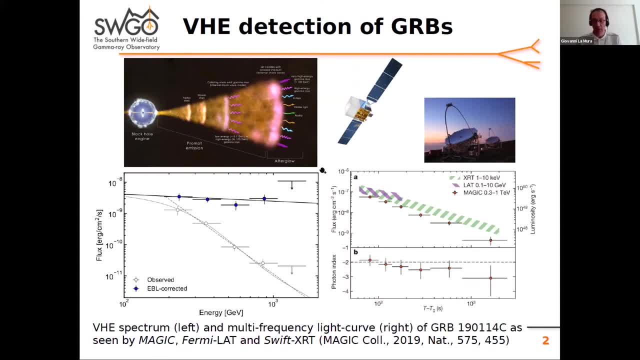 neutrino detection. What we know from the observations that were carried out in the past is that gamma ray bursts can radiate in the very high energy domain without the appearance of intrinsic cutoffs. The photons that were detected in this component appear to be possibly. 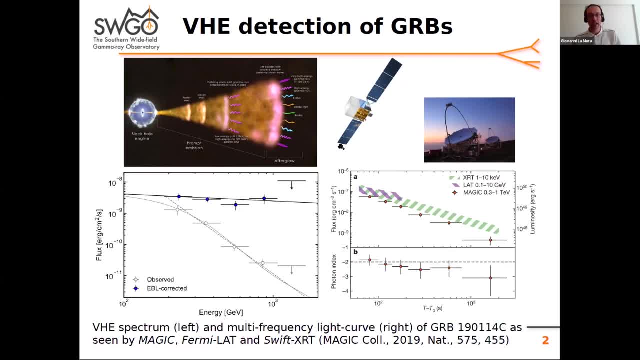 associated both with the prompt emission and with the afterglow. In the case of the afterglow, finally, MAGIC and HESS observations were able to actually detect the extension of this component up to almost the light opacity, which produce a severe absorption. 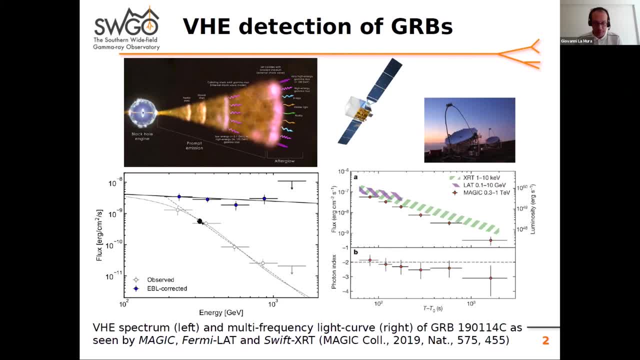 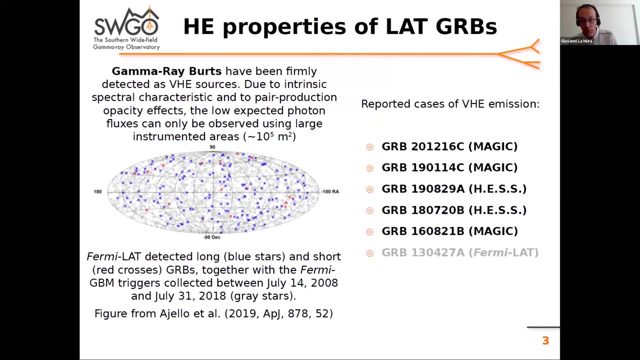 of the most energetic photons. The intrinsic spectra interestingly appear to be a power low of a spectral index close to minus 2, which leads to a very low energy spectrum. The flux which is detected in the very high energy domain appears to be something. 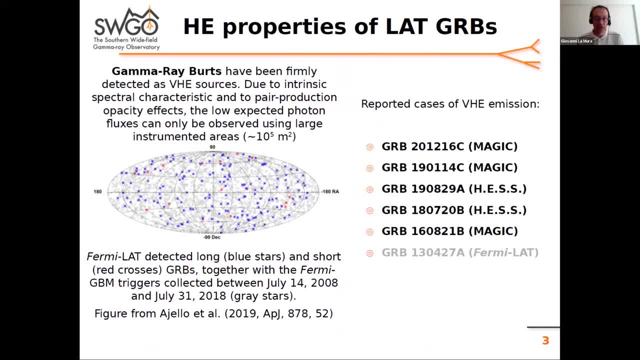 that exceeds the extrapolation of the low energy spectrum. So the idea is that we may use this monitoring campaign to extrapolate the expectations in the very high energy domain and compare with what we know from the currently available observations. Here we have a set. 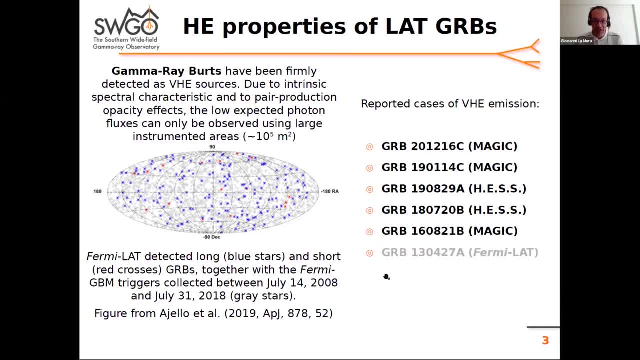 of the most recent results from the last year, And I'm putting also in gray shade the detection of this classic GRB1304-27A by Fermilab, which went up to the famous 95 giga electron, and the lack of previous 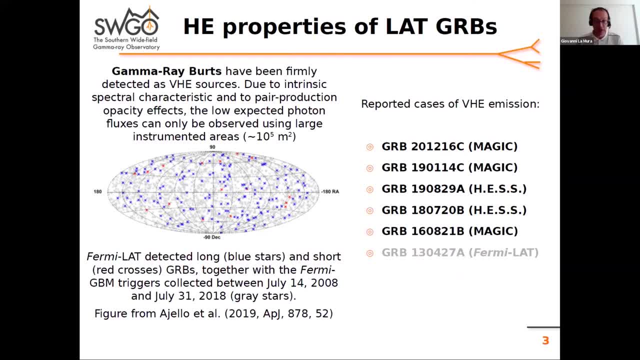 detection is due to the fact that the expected fluxes at these energies are very low and therefore we need instruments with large effective areas sensitive to this domain range. If we use the GBM and other triggering instruments, we can estimate what is the fraction of gamma ray. 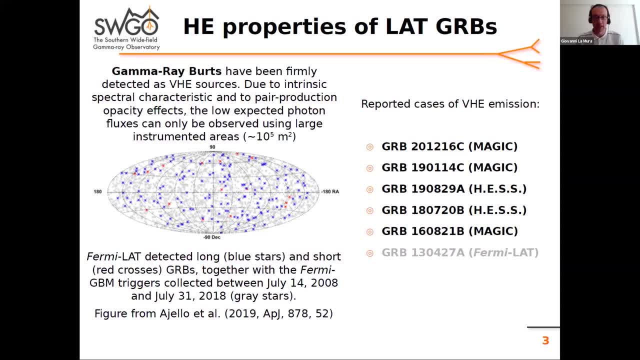 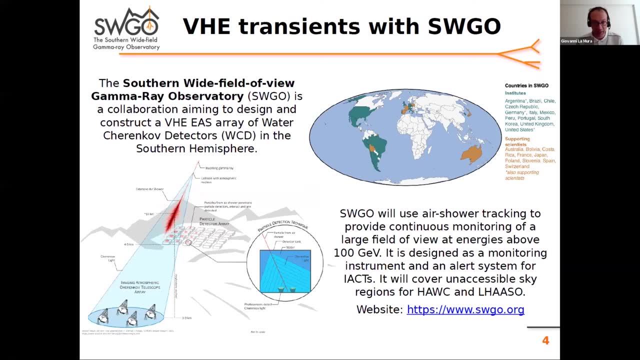 bursts that are associated to an energetic component and try to attempt to extend this population to the very high energy domain. Okay, Here is where the data has been formed in order to install a monitoring instrument based on water challenge detector arrays that should survey the southern 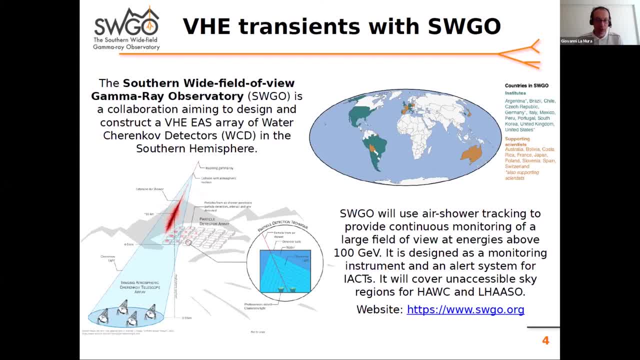 part of the sky, therefore providing a complement to the northern part of the sky. So this is the data that we have collected from the data that we have collected from the data that we have collected from the data with the quickest estimated response There is. 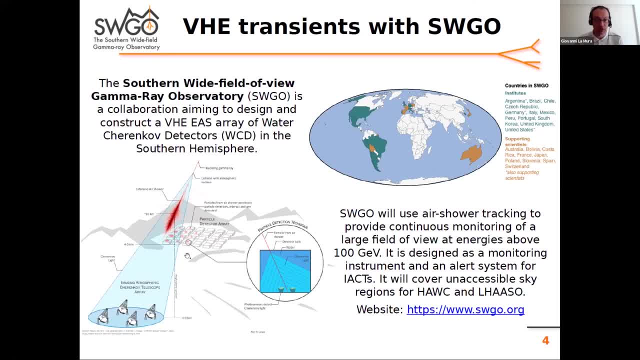 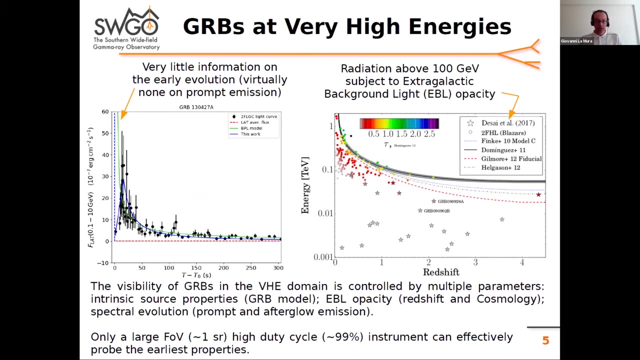 some fundamental information that we are not able to collect concerning the spectral evolution, especially in the earliest stage and possibly in the prompt emission of the event. Both of these data are very important for the interpretation. Our idea is that we can use the observations carried out. 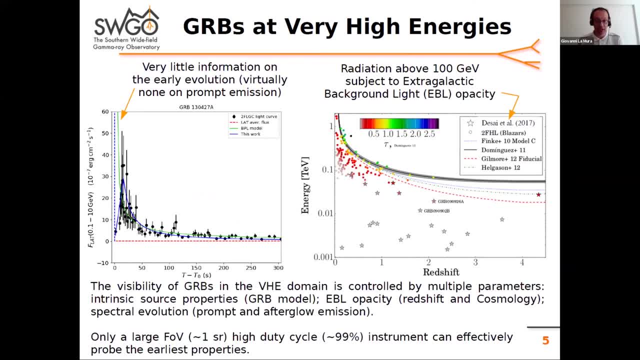 by Fermilat in 10 years and collected in the second Fermilat gamma rebirth catalog to try to estimate the evolution of spectral shape duration and redshift In particular. the redshift is playing an important role because of the expected separation of 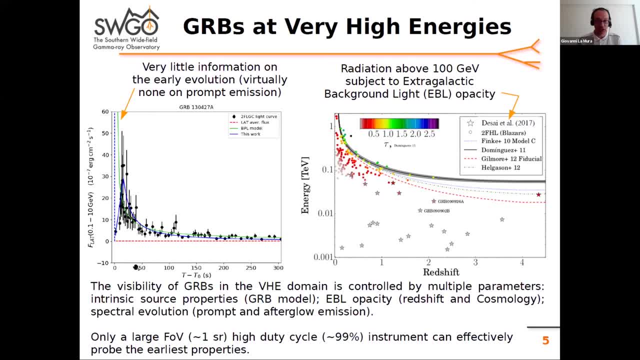 very high energy photons. Our idea is that we can, in principle, estimate what are the instrumental characteristics that are required in order to optimally follow the triggers related to gamma ray bursts, Of course, given the information that has been observed in gamma ray bursts. 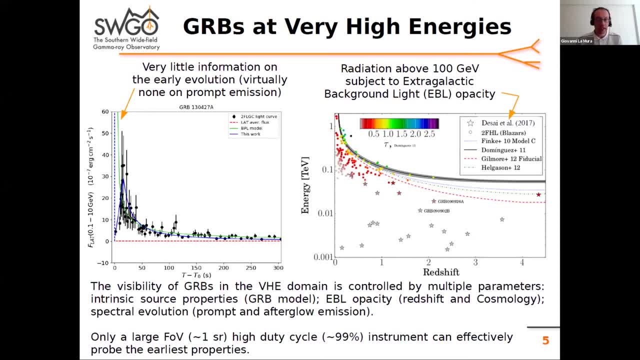 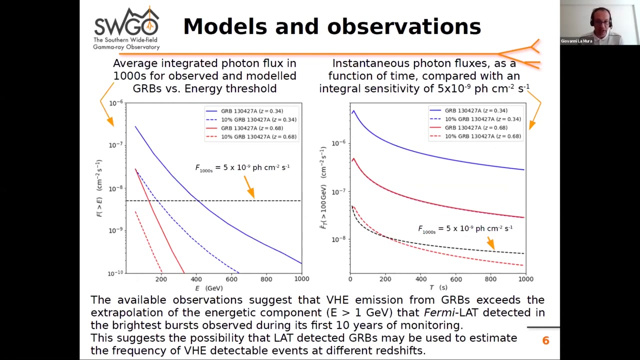 we know that very little information is currently available in the earliest phase of the evolution And only in a field-of-view instrument with a very high duty cycle can monitor in the sky. in order to probe this domain of the emission, Our approach has been to: 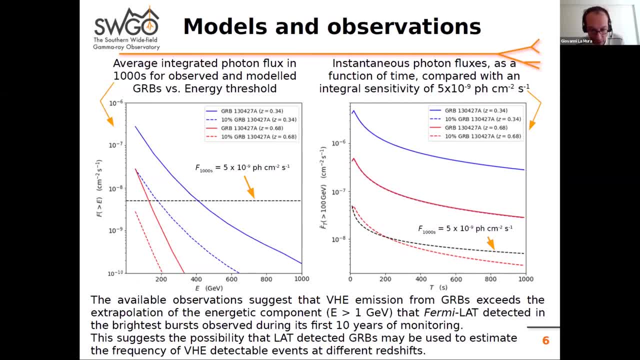 take the spectral and temporal characteristics of gamma rays and to attempt estimating the fluxes available above different energy thresholds and the evolution of these fluxes with the shape of the light curve observed by Fermilat. Our idea is to simulate an ideal requirement of an 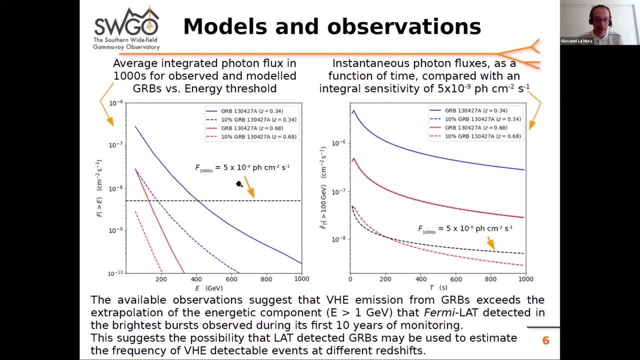 instrument able to react to a flux of some 5 times 10, raised to minus 9 photons per square centimeter per second, in an observing time of 1000 seconds, and compare it with the expected flux of real flux that are fainter than this. 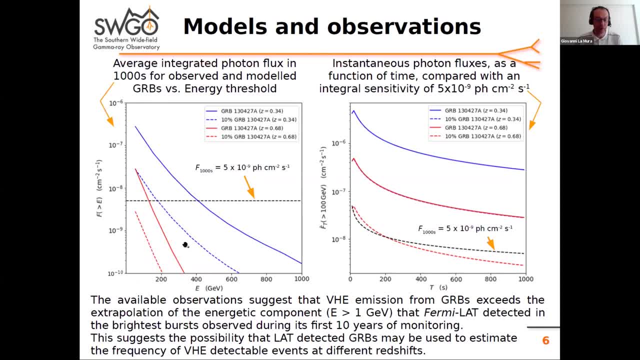 one, but located at the same red shift or at the same bar, simulated at a larger red shift, with the effects of 1,000 seconds, And if we assume a specific evolution of the sensitivity of the instrument close to the square root of the available time. 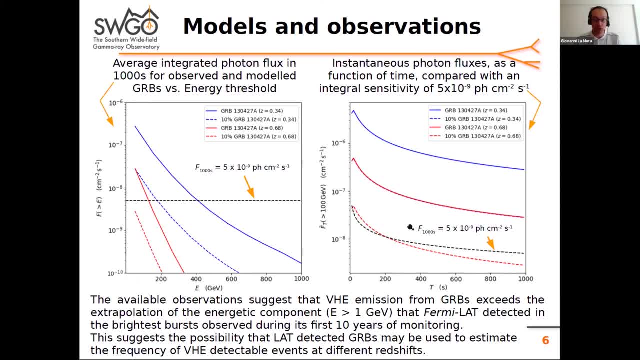 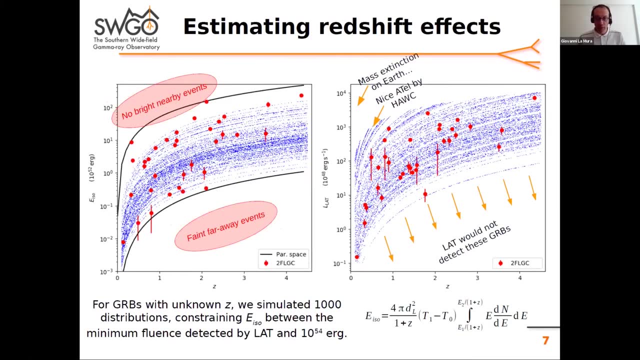 we see that the instrument is able to reach the expected flux emission from all the other elements of the instrument And we can see that there is a very small fraction of event, in particular, 34 LAT detected event out of a sample of the source and therefore 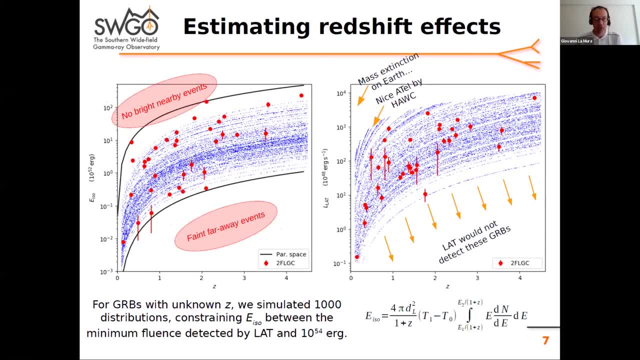 we know the intrinsic emitted power and the luminosity. There is a huge sample of events for which we don't know the actual red shift distribution, but we can use this population in order to extract an extension. To do this, we took the fluence. 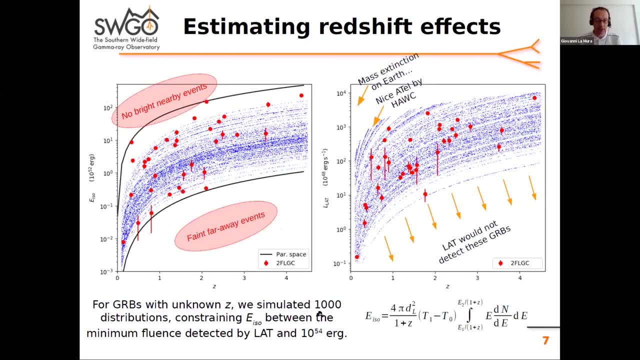 of the observed gamma ray bursts and we simulated 1,000 distributions of bursts having this fluence distributed over the same red shift range observed by Fermi LAT. This shows the specific luminosity on a specific luminosity range, which is actually consistent. 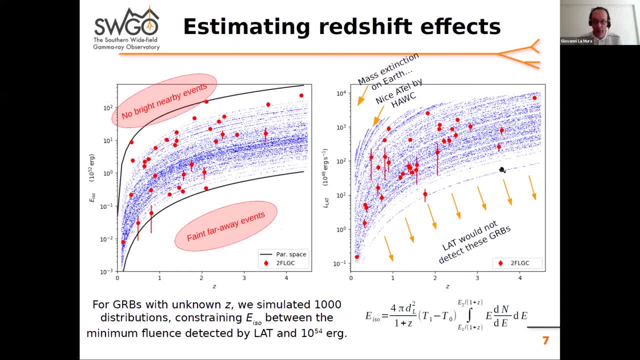 to the one observed and takes into account the fact that there we should not predict bursts to be distributed in a range larger than 1,000 distributions, And the simulation needs also to cover what we know from the currently existing observation, In particular, 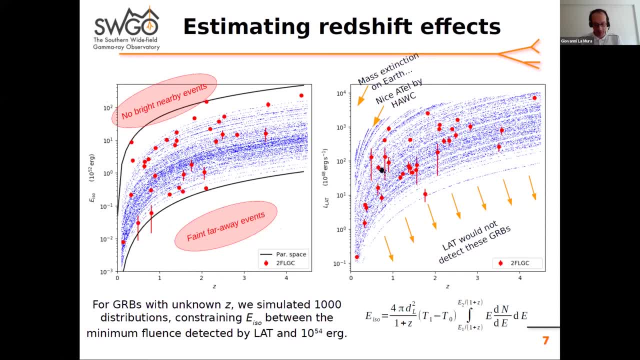 we see that the simulation comes to a region where we have much more dramatic consequences on the Earth. So the reason to use this approach is that the simulations calibrated over the isotropic energy emission take into account all the signal which is recorded in the population. 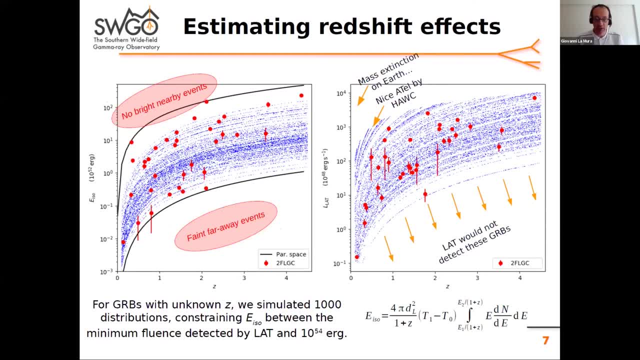 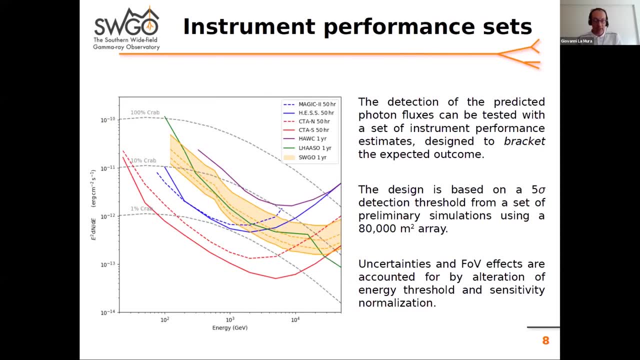 for bursts that were covered only for a very short time of loud signal duration. Our purpose, once we have a distribution of real and realistic simulated performance with a set of instruments, performances that basically bracket what we expect to be the final performance of the SWIGO array. 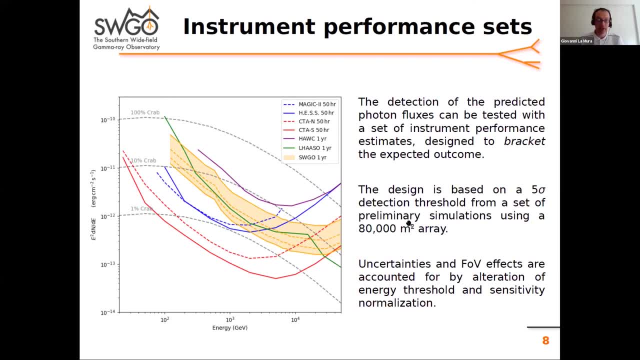 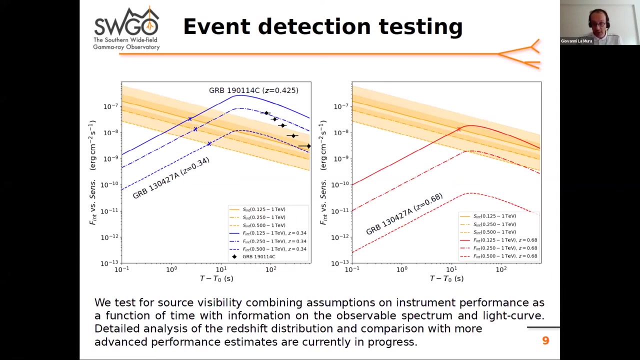 We base our simulation on a reference performance which simulates the field of view, and we account for uncertainties due to variations of sensitivity in different positions of the field of view by alterating this reference sensitivity and the energy threshold above which we can simulate the fluxes. 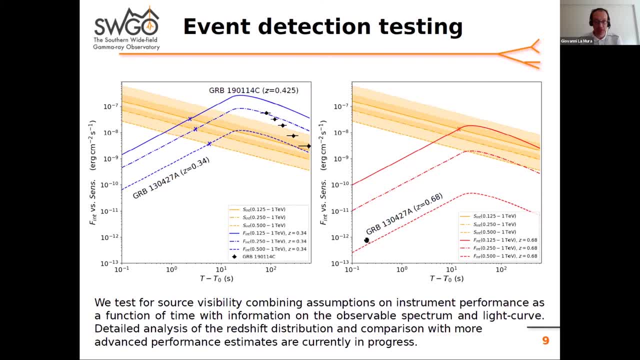 that we expect with the corresponding instrument, sensitivities adopted as a function of time and, in particular, we can evaluate, once we know the spectrum, the light curve and the different adopted array, with the different energy threshold, checking in which amount of time we get the detection in the 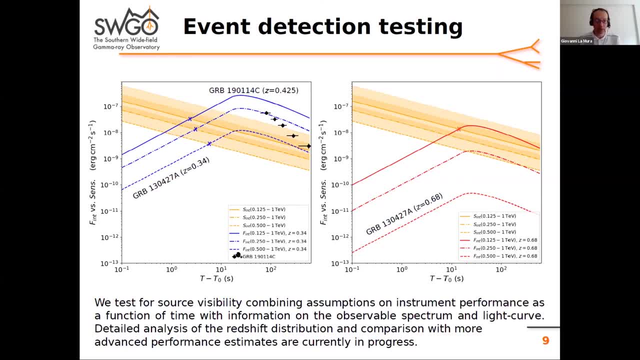 sense that we accumulate more flux than the one which is required by the corresponding instrument configuration and we are able to simulate less optimistic cases. but we see that an array which is able to perform down to at least 125 giga electron volt is still able to. 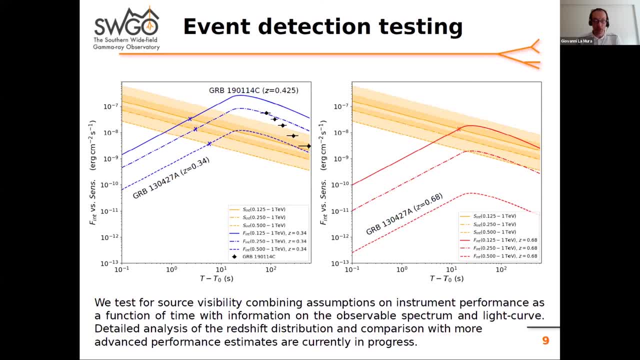 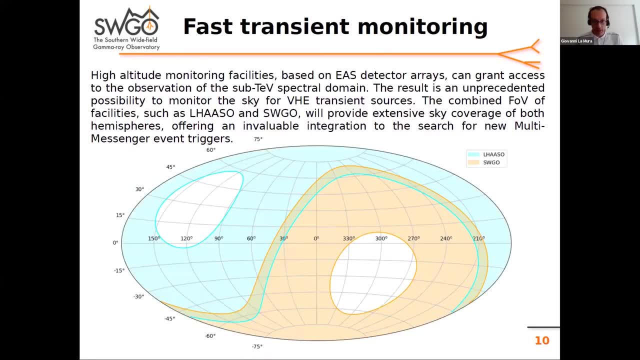 access simulation with simulated faint GRBs and therefore increase the detection rate possibilities. as a final remark, we can conclude that the combined operation of LASO and SWIGO will therefore result in an nearly zero emission, which will represent a fundamental way to improve our knowledge of the 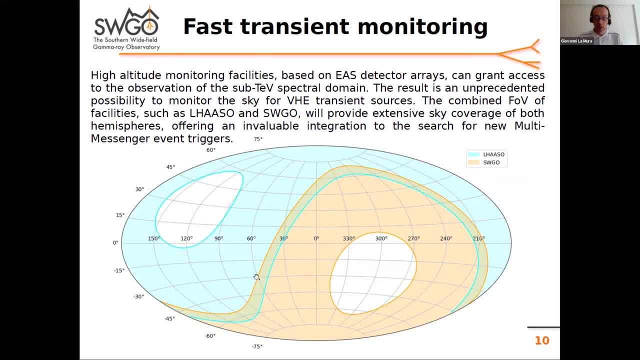 very early and possible prompt very high energy properties of gamma ray bursts, leading also to plug a fundamental additional piece in the search for very high energy emission and to provide reliable locations towards the source, will definitely help the search of potential association with other alerts coming, for example: 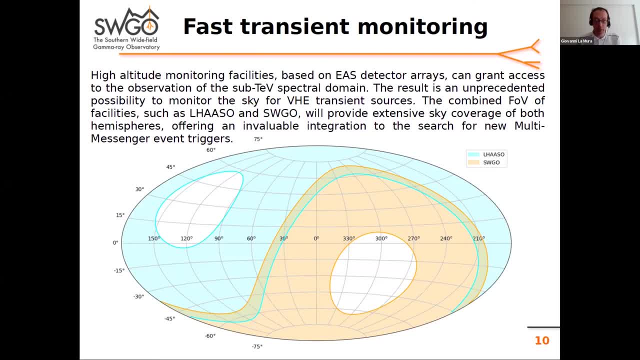 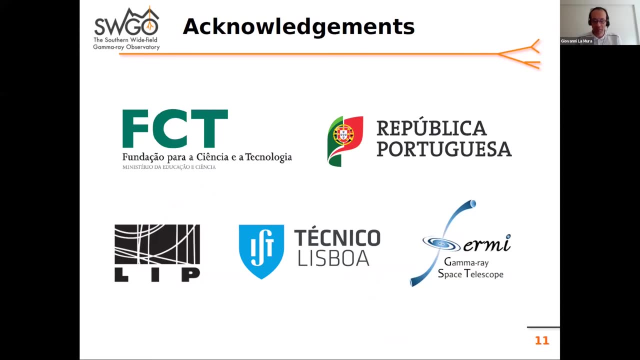 from particle and gravitational wave detector and further drive the follow-up that will need to point to the region in order to collect all the required information. with this I am over. I will be happy to answer your questions and listen your comments, if you have any and if 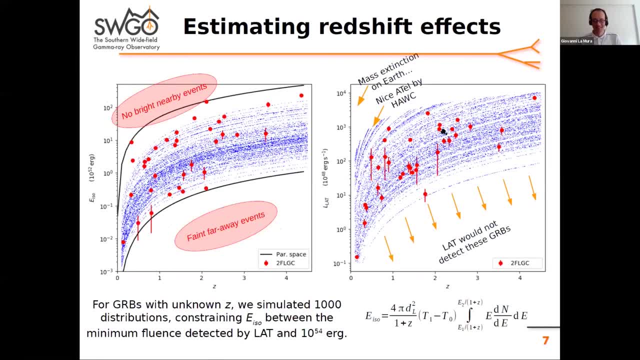 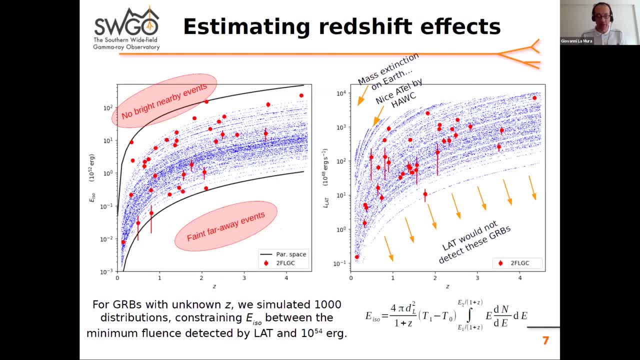 the, the, the of the sky which Hawk is observing. they should potentially be detected, And this is in agreement with what has been stated elsewhere. So this one is not really a scientific, But the point is that in this region we expect that Hawk should be able to react. 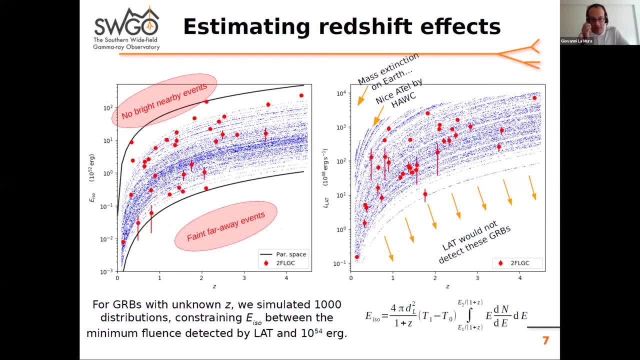 But these bursts are so rare. let's say, according to our estimate, that this is consistent with the fact that Hawk has not yet detected any No And OK. in this plot, the red dots are not the one expected to be detected by Zwiegel. 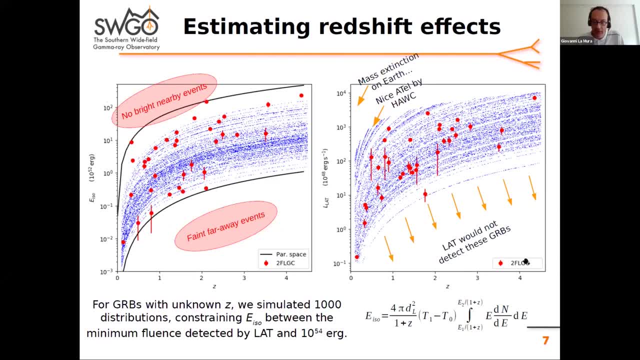 but they are the one detected by Hawk. No, no, This one are the ones with the known red shift, And the request that I have is that I might have missed it. Have you said something when Zwiegel can be starting to take operation? 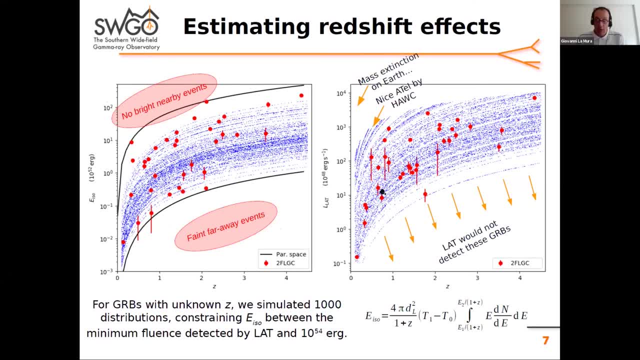 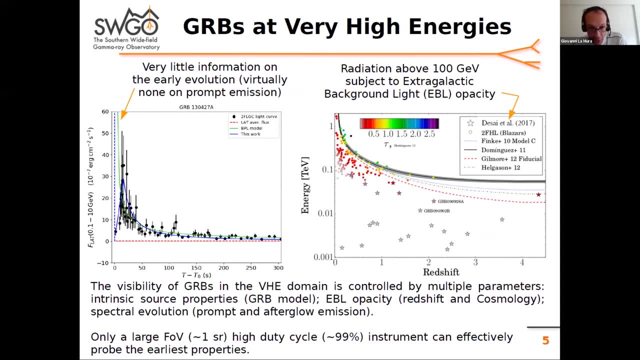 Or this will be. we have to wait until. Oh OK, I think that the correct answer will come from the full Zwiegel presentation, But we have some orders of magnitude concerning the current stage, which should come with a final design with all details proposed. 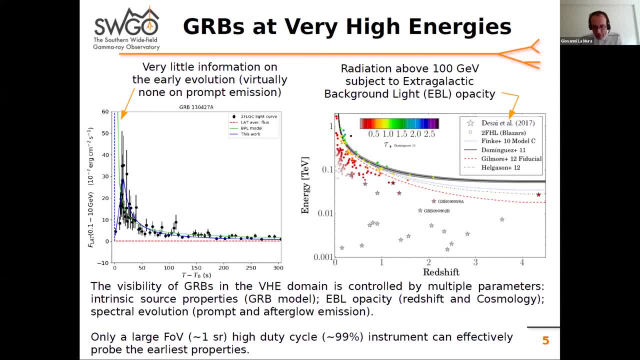 by the 2000.. Then the- And the instrument should be in the best of all possible words, I think, because we need to take into account that not everything is under our control. The instrument should be operating and taking data by 2030,, more or less.